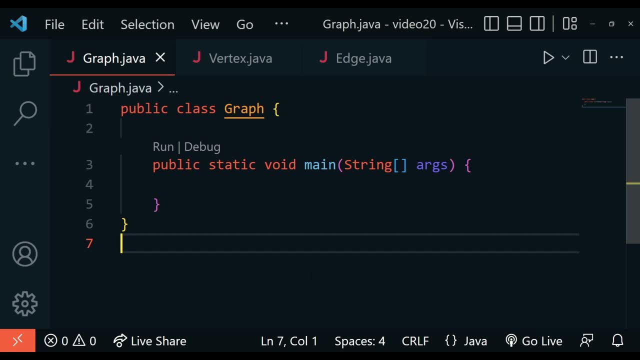 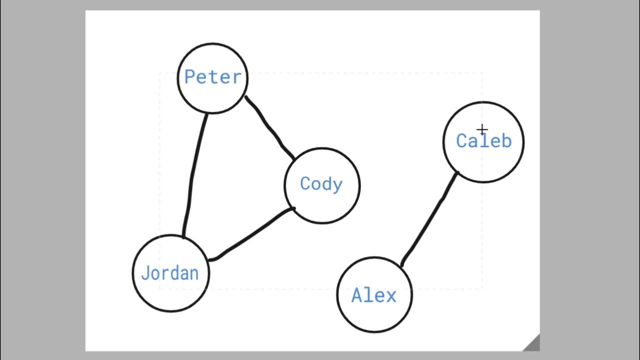 or vertices which hold data and edges which connect to vertices. A vertex is a single node. Now all of this will be explained through the diagram. Here's a sample of a graph that I created. These circles everywhere are actually vertices and they're holding data and edges which connect to vertices. So these lines over here are known. 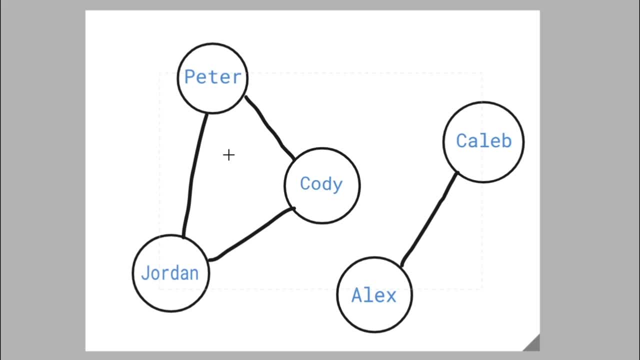 as edges These things. Now I want to give an example. Consider a map of your neighborhood As a graph. we could represent bus stops as vertices and bus routes between stops as edges. So how about the internet? Web pages can be thought of as vertices and the hyperlinks that 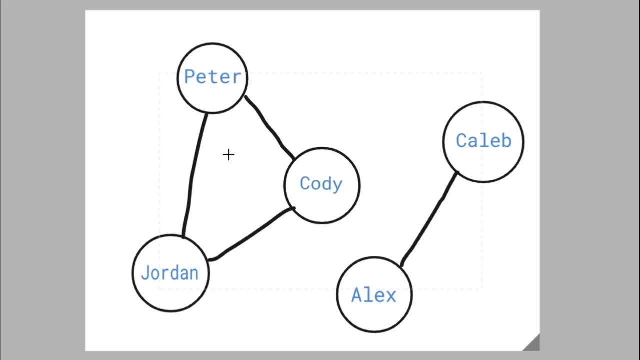 connect them as edges Real world relationships represent, as graphs are numerous, making them an important concept to grasp. The graph which you could see over here is actually representing a social network. People are vertices and edges are friendships, So these lines are friendships. 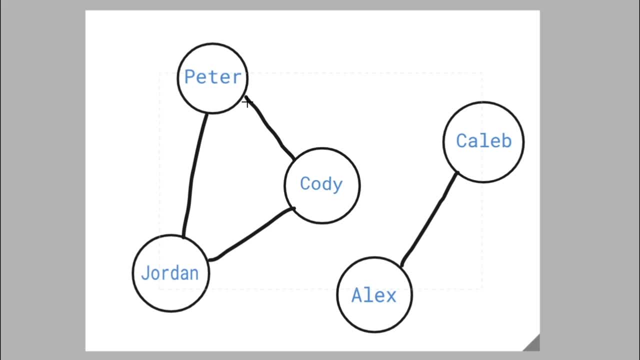 These circles are the people. Peter, Cody and Jordan are all friends. Peter and Cody are friends, and the same goes for Cody and Peter. Peter and Jordan are also friends, and Jordan and Peter are friends as well, So this bi-directional pattern is also existing here. Jordan and Cody are friends. 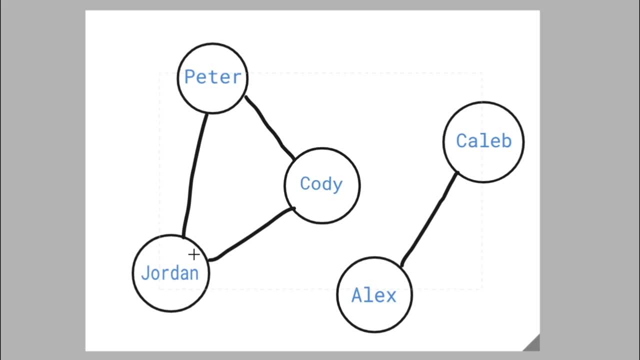 and Cody and Jordan are friends. One other thing that we see here is this thing, which is Caleb and Alex. Now, these are friends, but these are not linked with these people over here. Interesting A path is made up of vertices connected by any number of intermediate edges, From Peter to 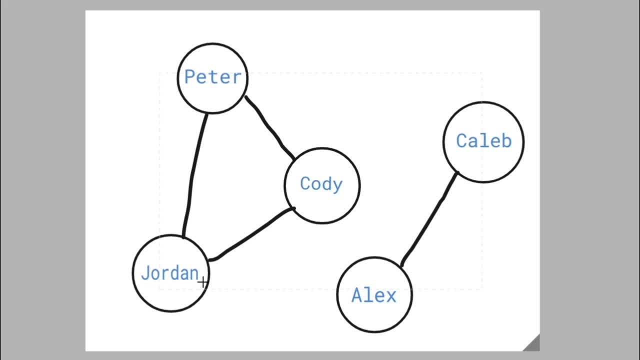 Cody. the paths could be Peter to Jordan, to Cody or Peter to Cody. There is no way between Peter and Caleb. A graph is disconnected when no path exists between two vertices. So this here is a disconnected graph because not all of these vertices are connected with each other. It's 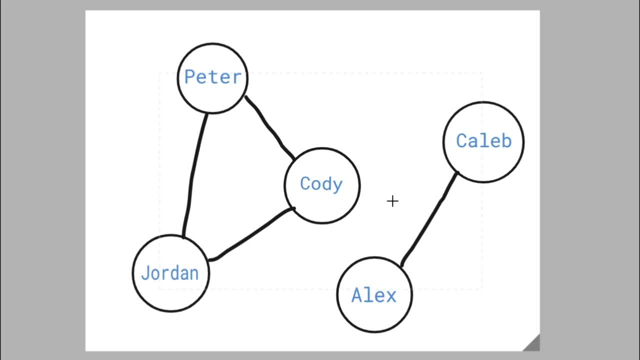 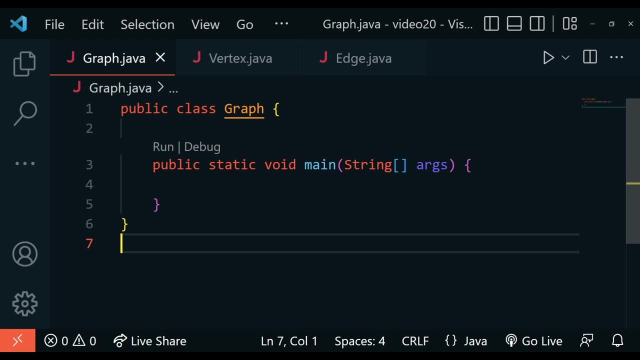 impossible to reach here. so this is the reason why this graph is a disconnected graph. All right, so now let's map out this concept in our code. Now what we want to do is we want to create a graph class that could be flexible enough to support directed, undirected, weighted and unweighted. 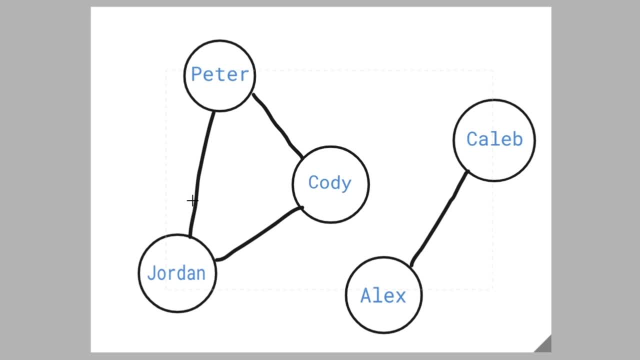 Now, the difference between a directed and undirected graph is that for directed graphs, which is so, this is an undirected, disconnected graph, because there's no link here and you can't reach here, so this is disconnected. the reason why it's undirected is the reason that 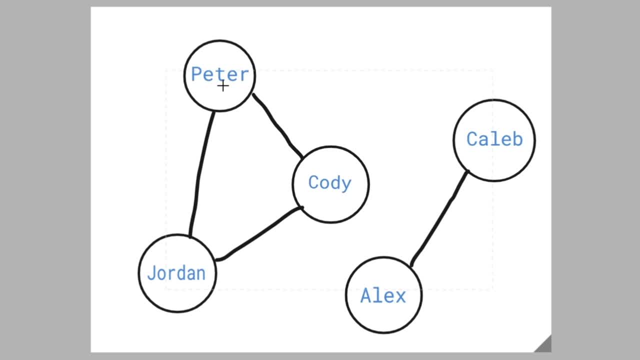 both of these paths are like bi-directional. so over here, Peter and Jordan is Peter's friends to Jordan and also Jordan's friends to Peter. so this is bi-directional. so, and this is undirected. if it's directed, it would have arrows here, so it would point. 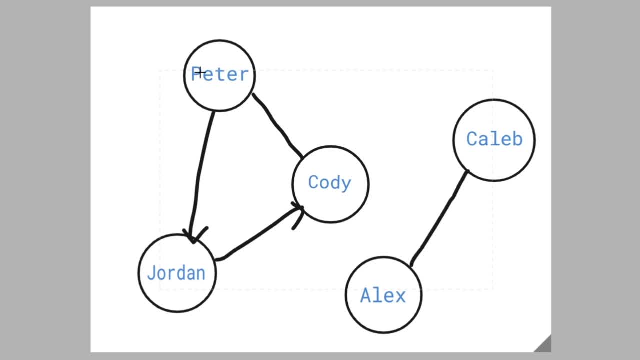 that Peter is only friends to Jordan, but Jordan doesn't like him back, and Jordan is friends to Cody and Cody doesn't like him back. so something like that is going to be directed. in case of weighted graphs, you'd have weights on top of each, so I know it doesn't make sense over here. 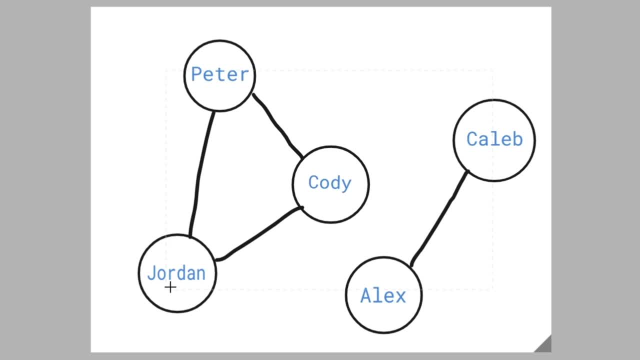 but if we had like um stop bus stops and then their um routes, it would have been easier and easy to map out. but here if I say Peter and then Jordan, it takes like um, let's say five. so it's something like this, and then we have 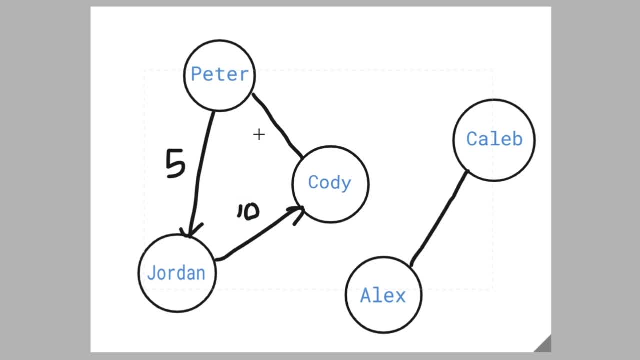 um, over here we have, let's say, 10, and over here, let's say it's 12.. so over here now we got weights on top of the edges, and these are just going to indicate the number or the expense that we're going to take here. so, Peter, um, I know it's not a good example. like I said, we could have done with. 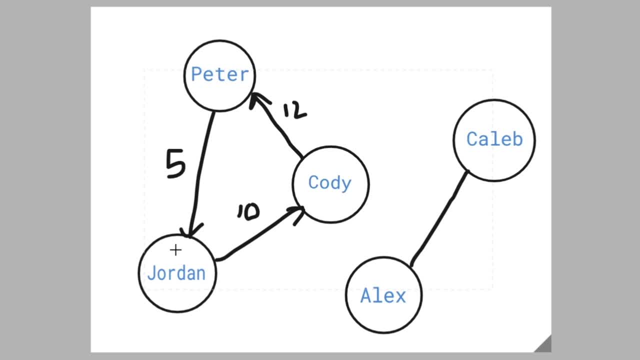 weights, but here we're taking. Peter is friends with Jordan and I don't say five times, uh, he, he likes him five times. this Jordan likes Cody 10 times and Cody likes Peter 12 times. I'm not sure if that was a good example, but uh, you, you got my point there, something like that. it with which. 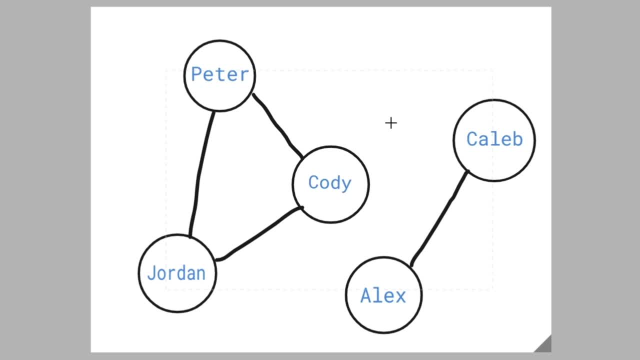 associates um the numbers as their expenses. with this in mind, we will create our graph with the following requirements: a vertex can store any data. so if you have a vertex, you can store any data. you can store any data. if you're not sure, yeah, if you're not sure which one to use, you can um share. 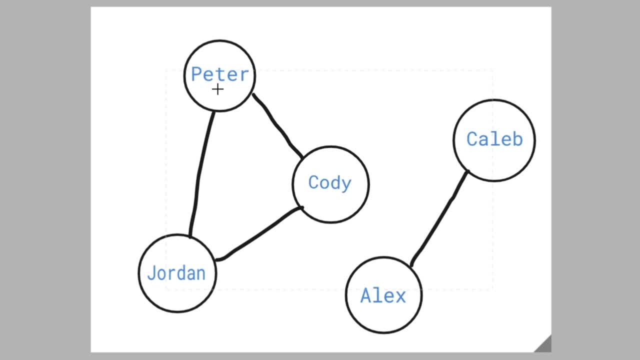 the data ourselves and then just figure out the difference between the color gradient, Wennstorm and thelandstand, the 영화 gradient. but sometimes you don't want to consider them as twoIL values and people are gonna go and hit them in the seabed, so it's part of their 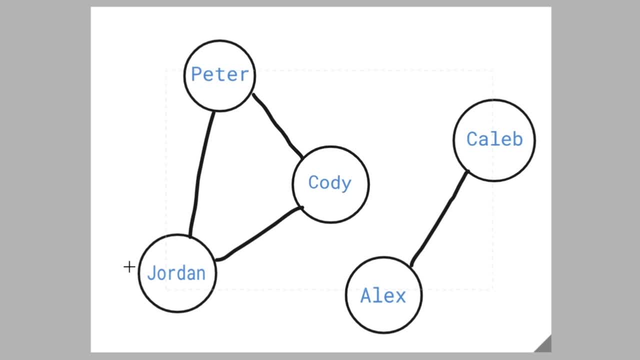 business and they can um, when they show if they are um, you know, 155, you know, commented maybe 505, why don't they use the same value, which is a lot more okay? somebody is asking who wants to be on the seabed. I think you want to go to this. 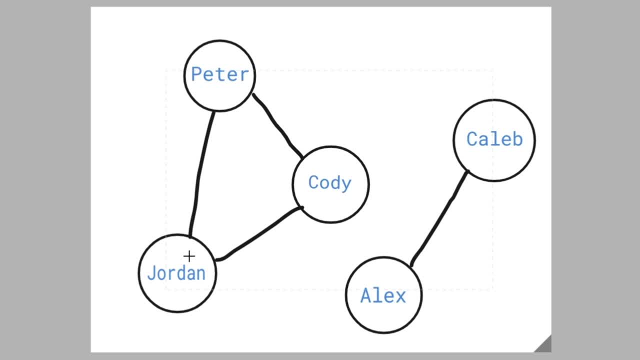 yeah, that was the first thing I was going to have to answer. so many times we're talking about, for example, many times we give you a to link to this line, about these together. really well, pretty much, you're going to learn literally the outcome structure here. So it's going to be in a list of edges, So they're going to be represented by a. 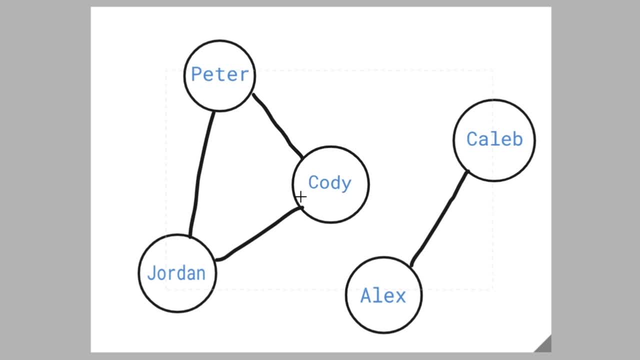 list of edge instances. A vertex can add and remove edges going to another vertex. A graph stores all of this, all of its vertices, represented by a list of vertex instances. So all of these vertices, you see, are just going to be stored in that graph structure. A graph knows if it is. 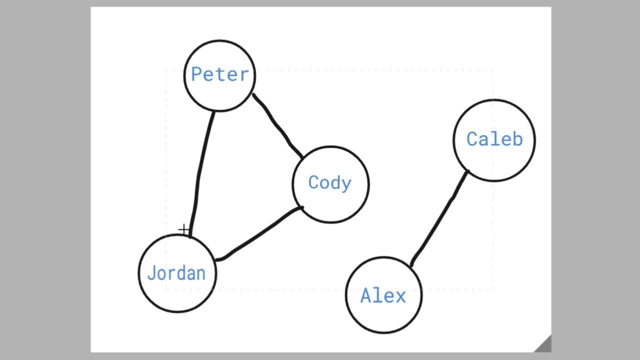 directed or undirected. Like I said, this is undirected And if it had some kind of direction it would have been directed. A graph can add and remove its own vertices. Graph can add and remove edges between stored vertices. With all of that out of the way, let's write the code. 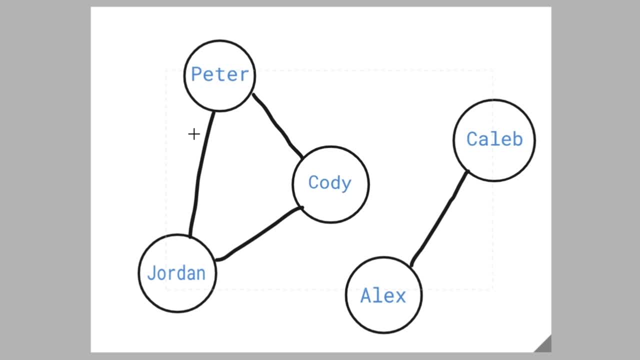 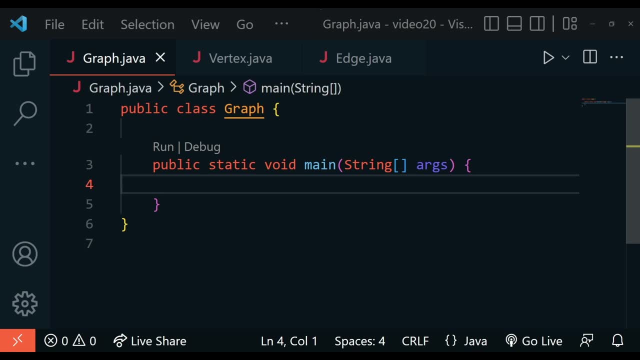 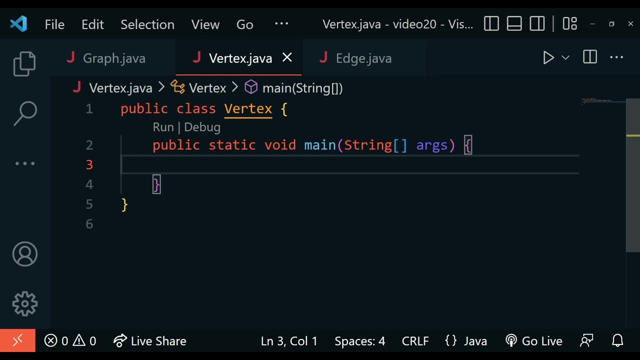 So, to keep the concepts grounded in a real world application, we'll build a transportation network of bus stops as we go. What I want to do first thing is actually look into my vertex class And because I know this is a circle which has the data and it's also going to have the edges. 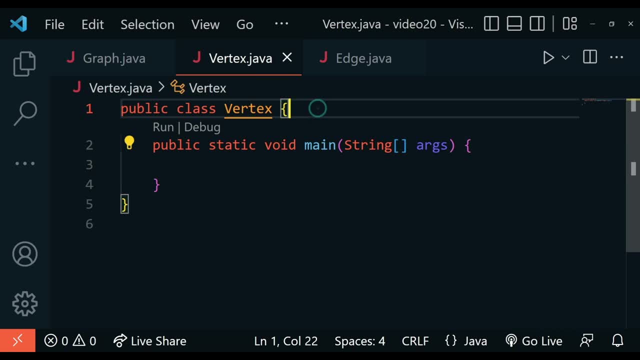 so we're going to start from this one Here, we're going to go into this class vertex here And we're just going to create some instance variables. So the first thing that I am saying is the private string data. The second thing that comes to the mind is private array list. 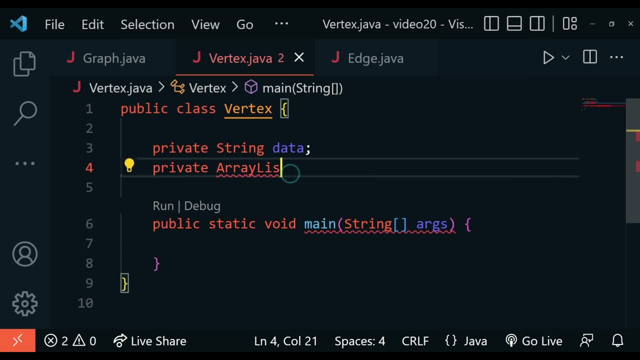 because we want to store the edges right. So we say array list, we put the type of the array list and we put the type of the array list. And we put the type of the array list And we put the type of the array list here. So we're going to store edges, So it's an array list of edges. 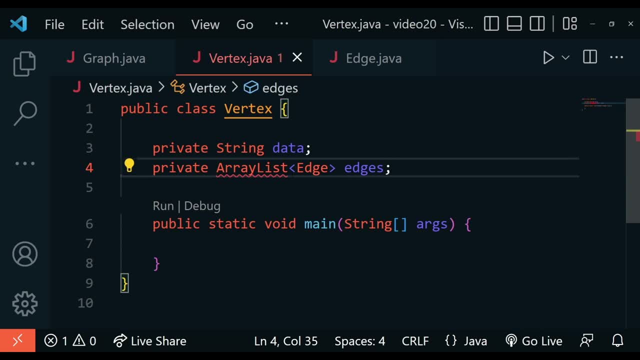 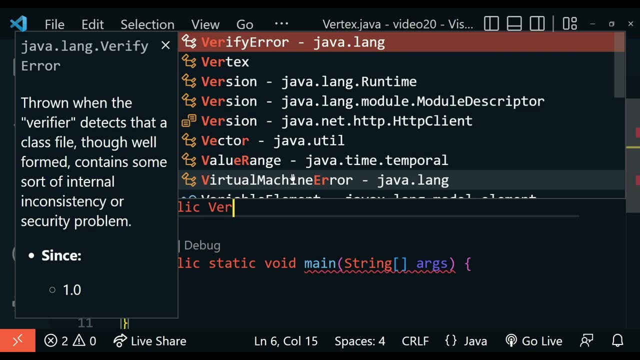 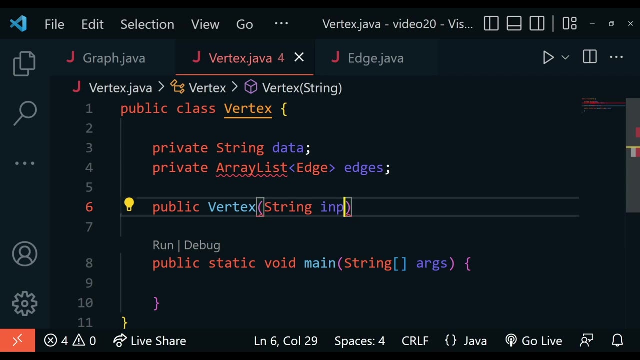 And we're going to call this as edges. All right, so now we're done with that. Let's add a constructor. here we're going to say public And we're going to say vertex. Here we're going to have a string And we'll say input data, the data that the user will provide. And then for that, 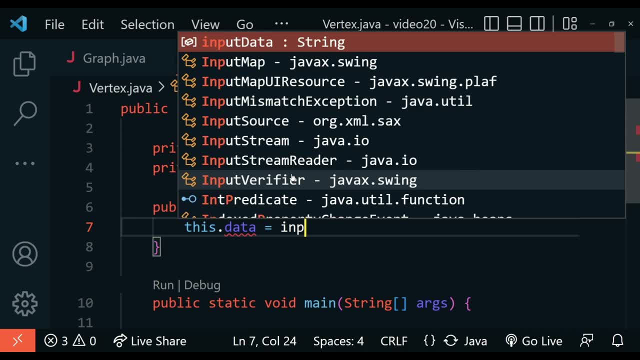 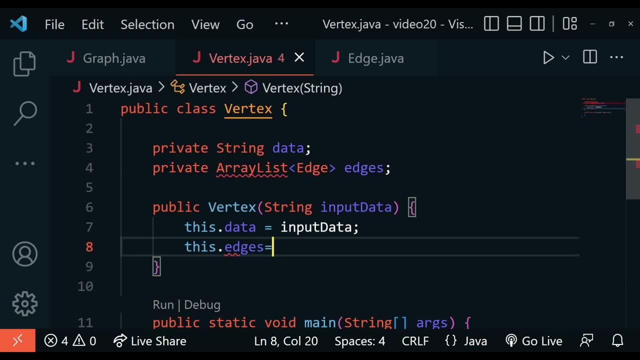 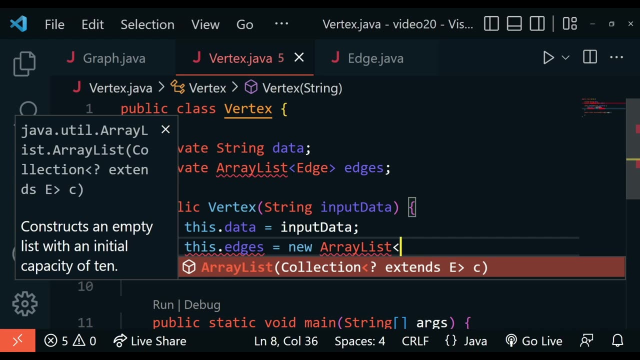 we'll say the class variable is equal to the input parameter, And then we have this dot edges, which is the edges, And that would equal to the new array list. And here we want the edge And we also want this. So 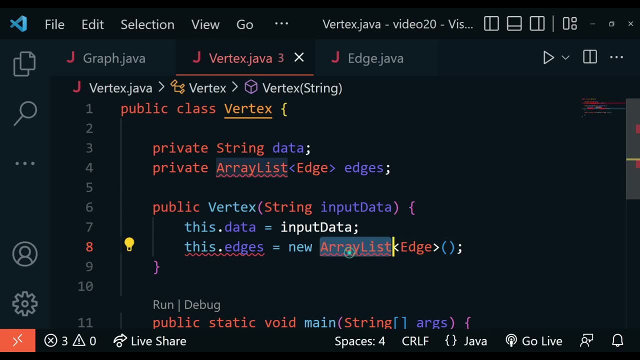 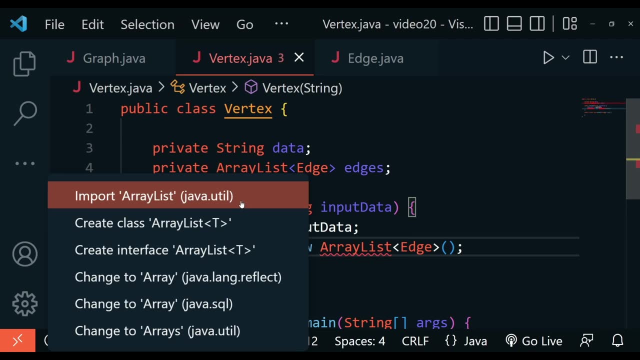 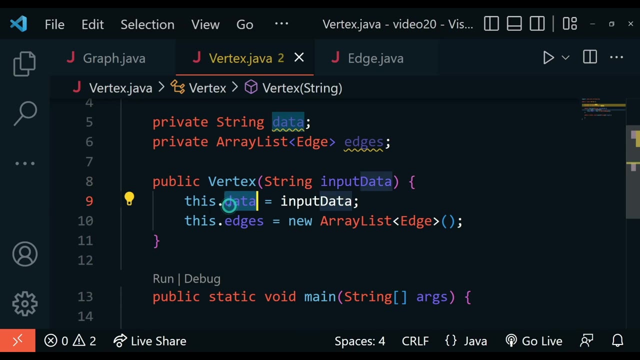 here we instantiated the array list, which was this edges one. Now I know this is giving us problems because it's not allowing us to have this, So let's just import this. import Java utility array list and the errors are gone. Here we have a vertex constructor that assigns the data with the input data and also. 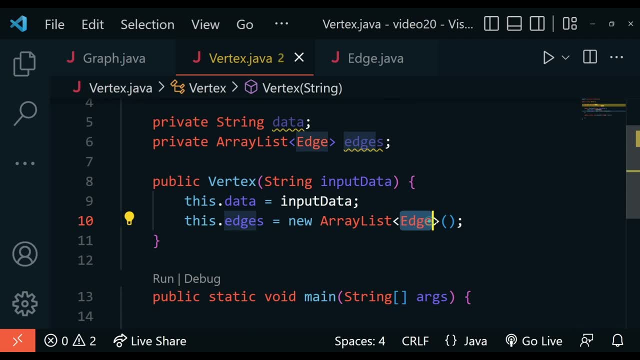 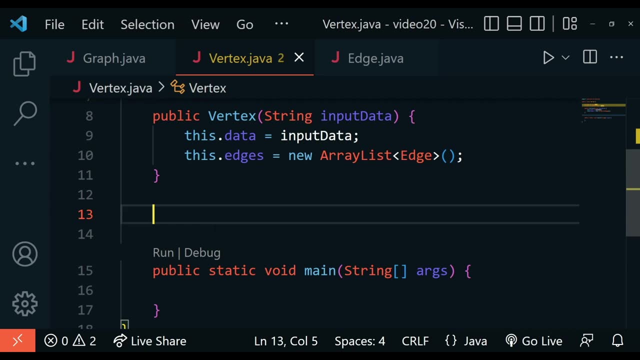 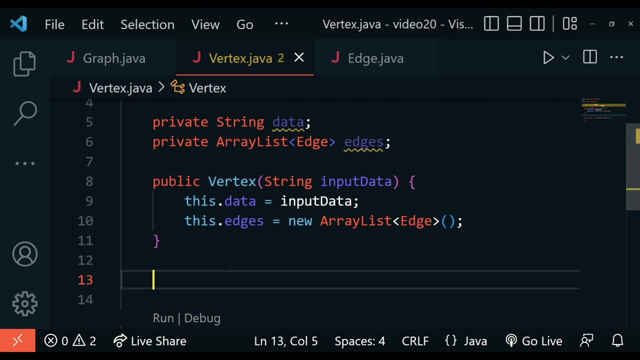 instantiates the edges list with a new array list of type edge. Now we got these vertices right. now we want to have a mechanism that will allow us to see these edges in live action right. The other thing that I want to go through this is that I'm going to create this as a directed graph, So 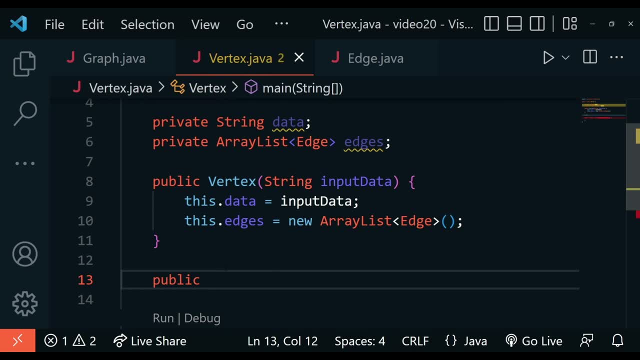 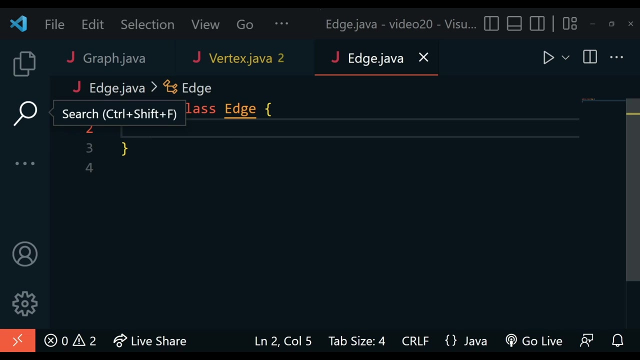 there's gonna be arrows here, a method called public void, add edge, And over here we're going to add in the vertex And vertex And integer: Wait, because the right thing here and the order over here is going to tell you you can see this right here. So here, you're going to add this node here And here. ween just goes over here. Now I'm going to, if you're coming over, say ng once. in two, this will work out, And if it's energy, these two mean a lot. 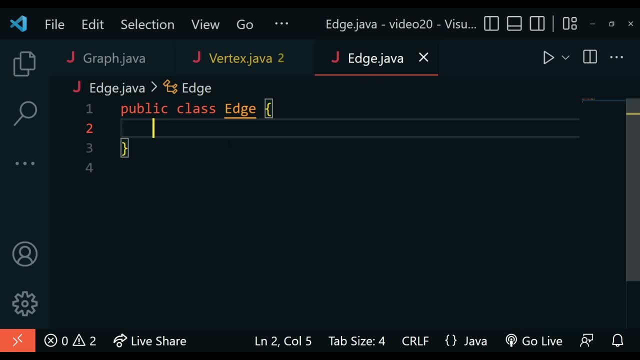 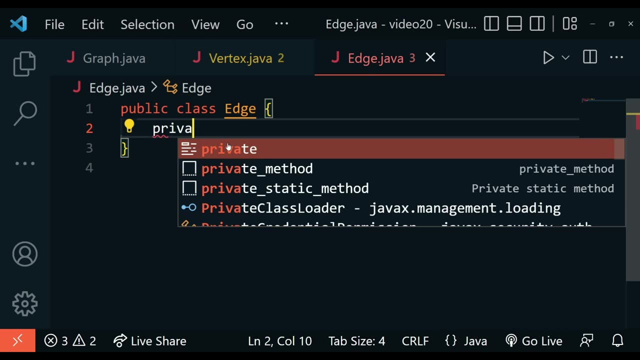 the other stop. right, it's a bus stop, so i don't want to go backwards. so in this case it's just a directed graph. um, what we're going to do here is for the edge. like i said, it's just a line where you see in the graphical representation, but here i'm going to have to try to map it out in code. 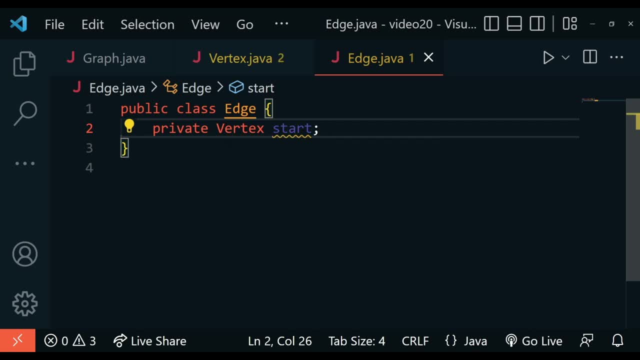 so i'm going to have the start vertex, where it's coming from and where it's going to, so pry vit private vortex, and then we have the end, and over here we want to wait. we're also going to create this as a weighted graph. that will have a cost. for how much uh expense? 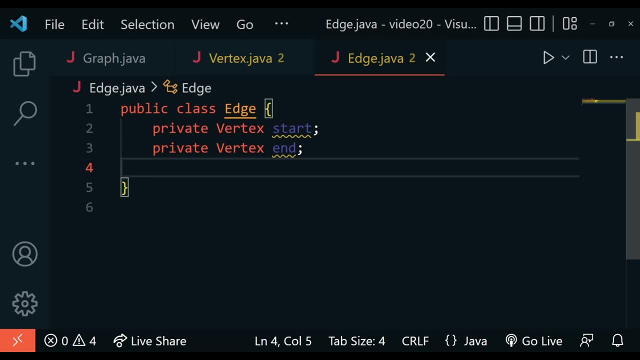 will it take to move from one place to another? remember those numbers which were on top of those lines. so that's the weight here. so it's going to be a weighted graph as well. so i'm going to put a weight in here as well, and it's going to be called integer and i'm going to say wh. I'm going to put a. 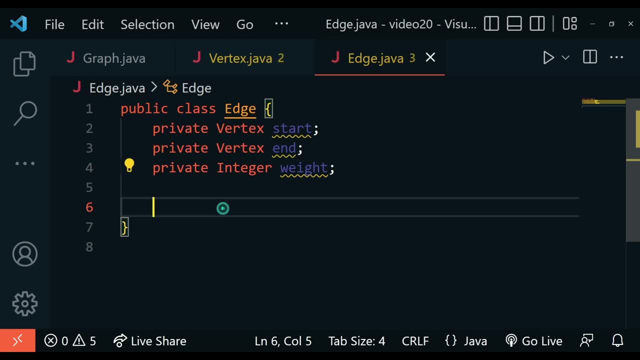 integer on this graph as well. i'm going to put a weight in here as well and it's going like a bit representations at that. i'm going to put a integer option and i'm going P and i'm going to put a weight. And notice, I'm using integer and not int. It's the reason. the reason is that if I don't want 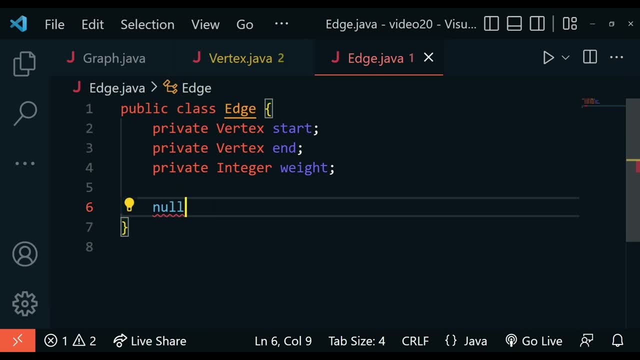 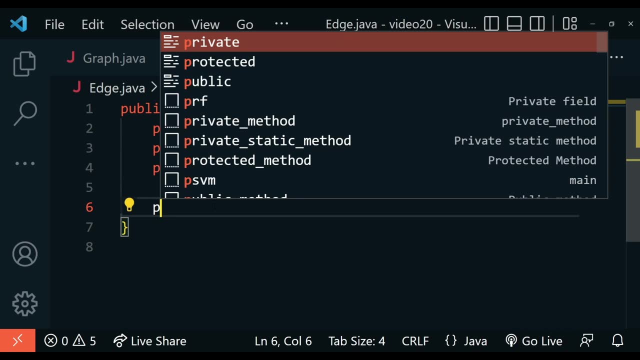 to put anything, I could just type in null And it would allow me to just like pass it with no reason. And if I had an integer, I'd pass in something like minus one, Alright. so now over here we have a constructor, and I would say public edge, And let's create the constructor here. So 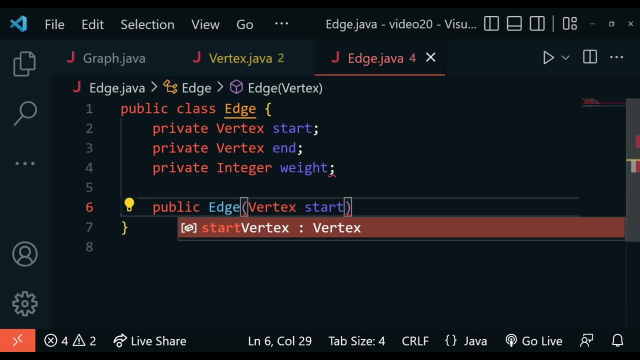 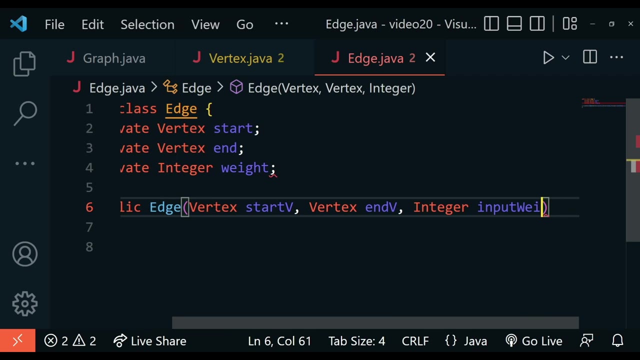 the vertex and I'll say the start vertex. So I'll call it as the start B, the vertex, And we have n vertex, we have n V, we have the integer And we call it as the input weight W. So there you go. 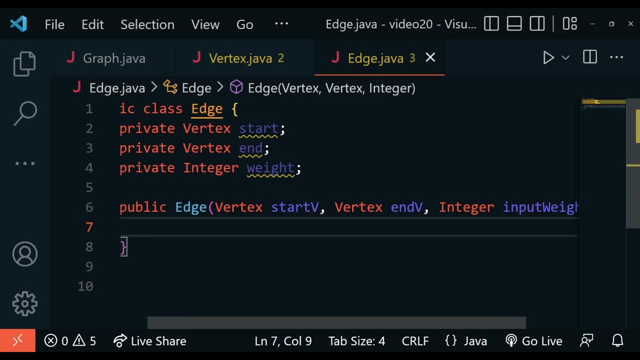 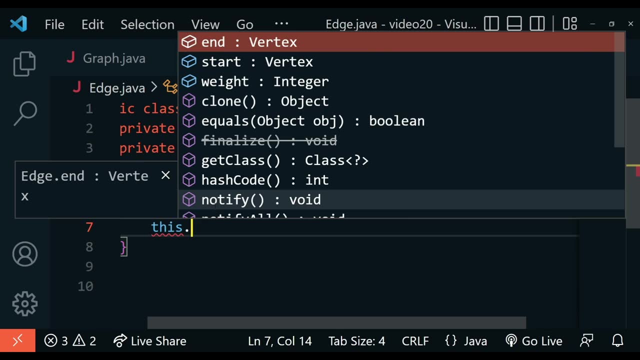 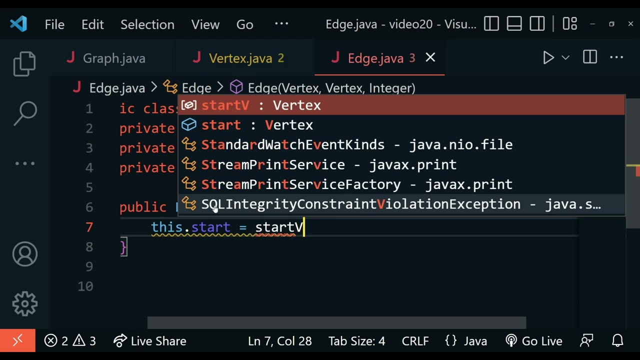 So we got the start vertex, the n vertex and the input weight that we're going to ask the user for. So remember, this is just an edge that we are creating as users. So the class variable, this dot star, will equal to the start vertex, which will be passed in as an input parameter. 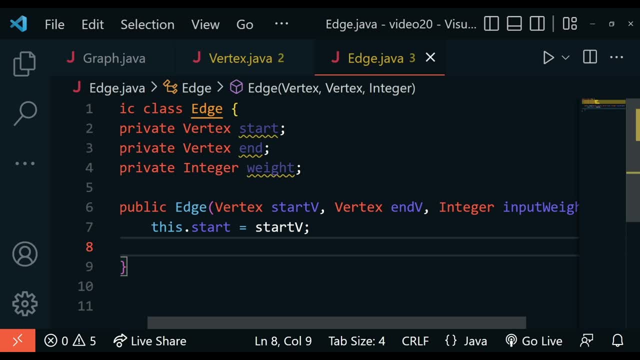 So remember, this is just an edge that we are creating as users. So the class variable, this dot star, will equal to the start vertex which will be passed in as an input parameter. The same thing goes for the disk dot end And it will equal to the end vertex. so we say end vertex And we 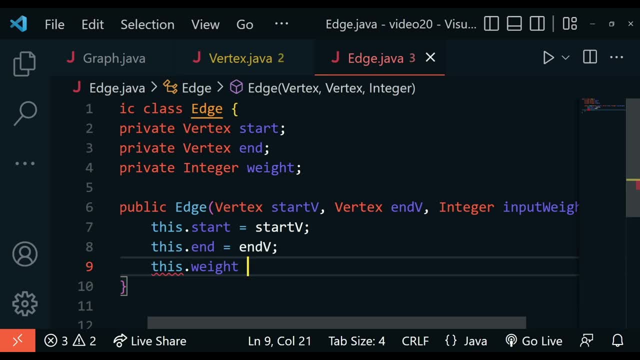 have the weight. So we say this: dot w e, i, g h t and we equal it to the input: w e, i, g, h t. There you go. So now we're done with this, And let's just add in some other helper methods. So let's. 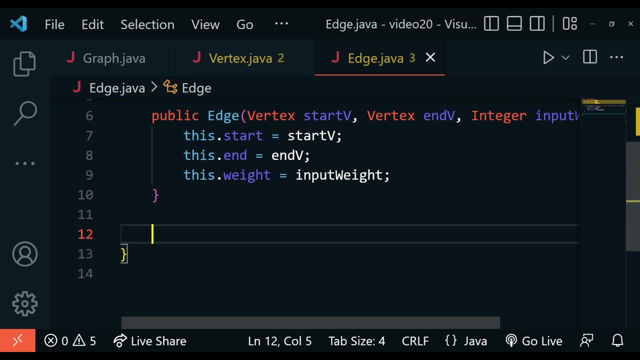 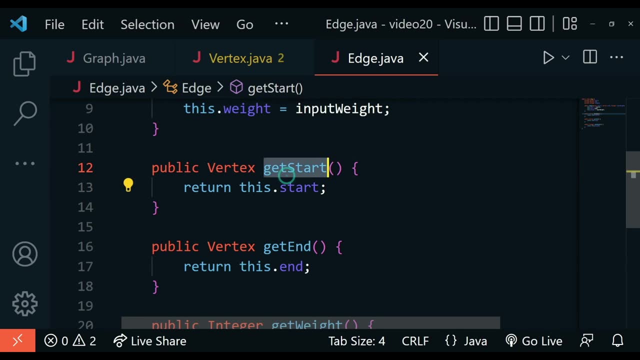 just add in some other helper methods. So let's just add in some other helper methods. So I'm going to be adding some helper methods along with this And I'm just going to be copy pasting this. So here these are the public vertex get start and it's just going to return the start vertex. 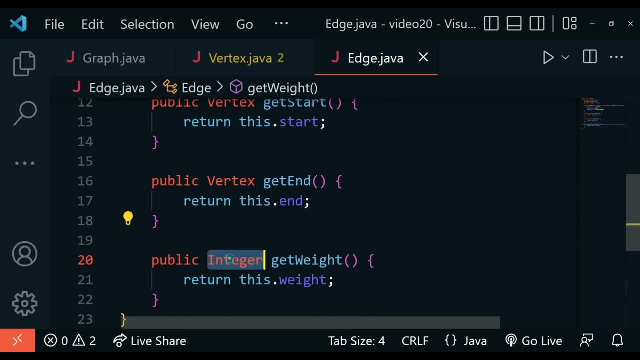 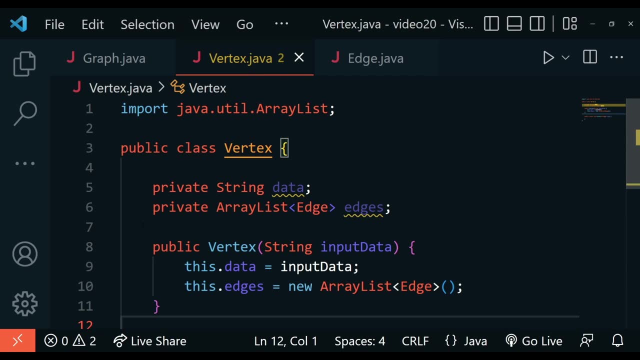 the public start. vertex get end will return the end vertex of the, you know the edge within the edge, and the integer get weight will just return the weight. Okay, so that was cool. Let's go back to the vertex dot Java file and just make some methods here as well. So for the vertex dot Java, 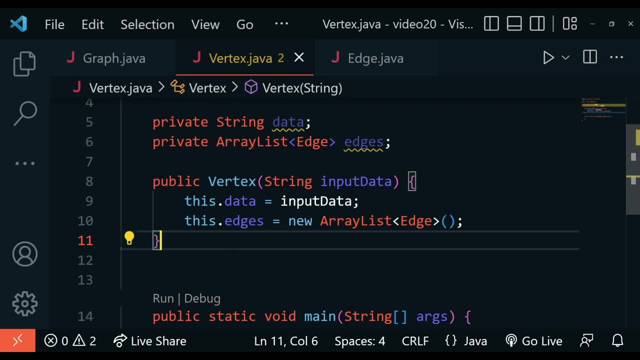 remember, like I said, I'm going to be adding some helper methods along with this, and I'm just going to be adding some helper methods along with this and I'm just going to create a big extension and go run one of the others and I'm going to check out a second option here. so let's call this get. 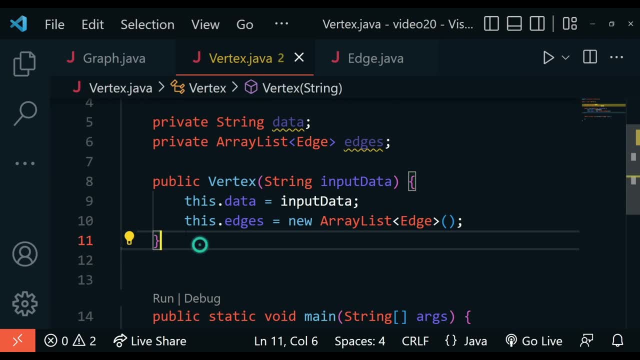 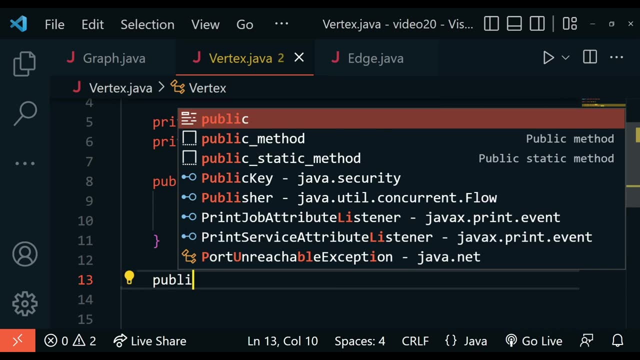 the product. you can pass this excuse and set the public like the public string. but instead we wanted to create a function that will allow us to add some edges. right, we're not giving the, we're adding, adding a layer of abstraction here and we're allowing the method over here will just add. 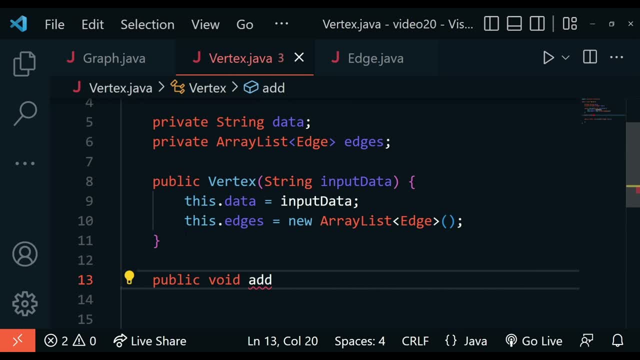 edges for us. So what I can do here is I could say a public And I'd say void, add e d, so e, add e d, so add edge. and if we want to add an edge to a vertex, So remember the current vertex is: 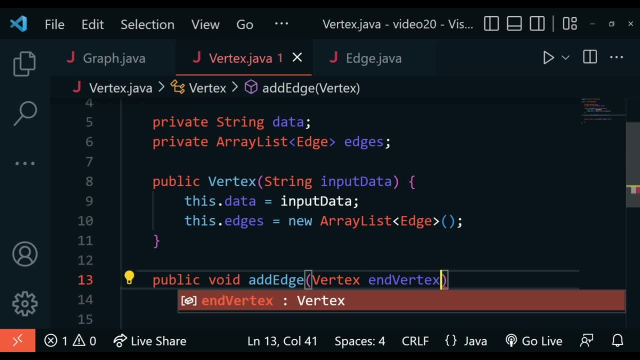 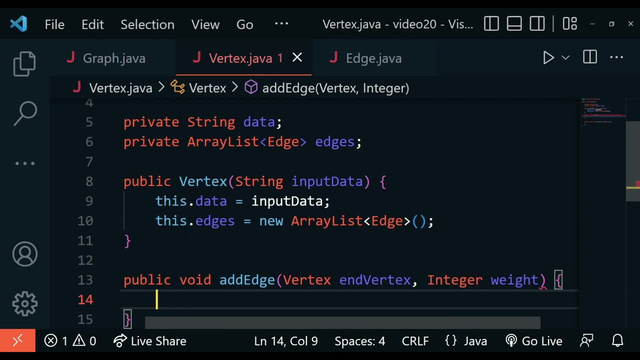 already in the context. So this will back add the vertex, which you can actually just do right here. mucha be the end vertex, So I'll just pass in the end vertex here And also the weight if you want to give it some kind of weight. Remember I said weight is optional If you don't want to give it. 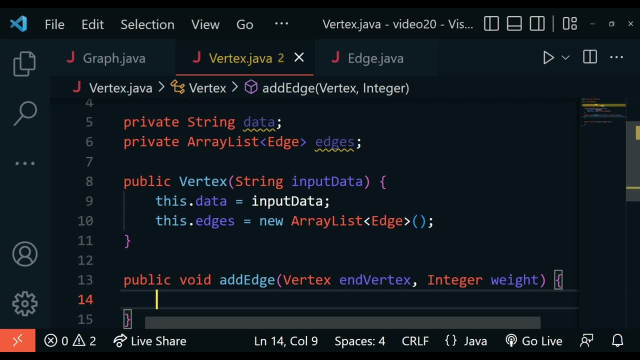 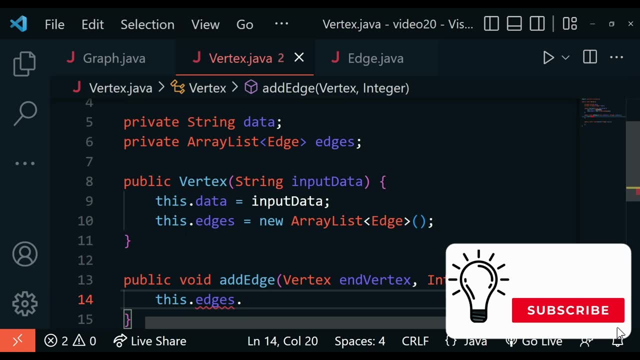 will be assigned as null To do something like that. First of all, I'm going to have the call to this. I'm going to say this: dot edges, edg es, because it exists an edges over here, And then there is a function that was called add for the array list, because edges is an array list, And 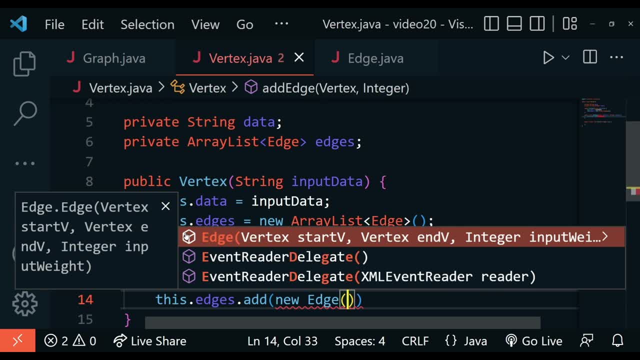 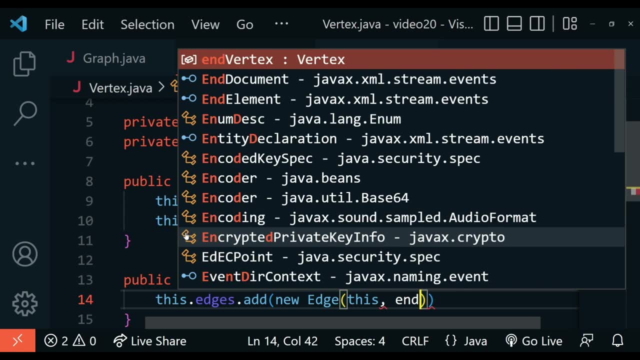 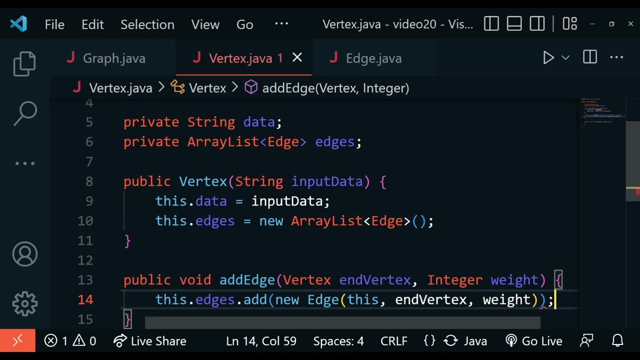 we just add in a new edg And we call in the constructor. So this constructor will pass in the this, it will get the edges and vertex. So it's going to be n, vertex And also be the weight of the edge. So all of this will be mapped in here. So this is our add edge And it's going to just 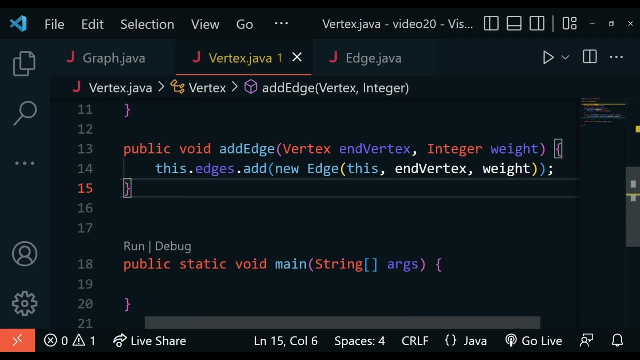 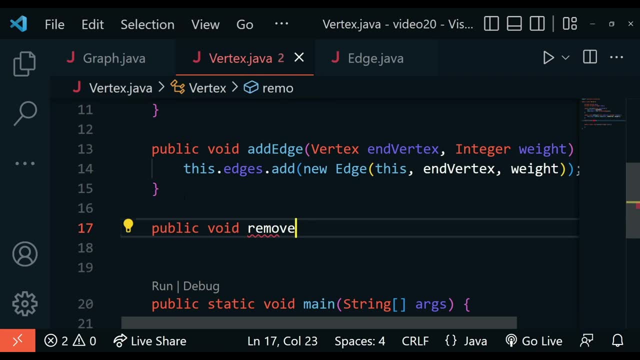 going to add some edges here, Alright, so now we're going to have to create the remove edge here. So we're going to say public And I'm going to say void, remove edg. And we have vertex And we have n vertex And over here we have the this dot edg edges. 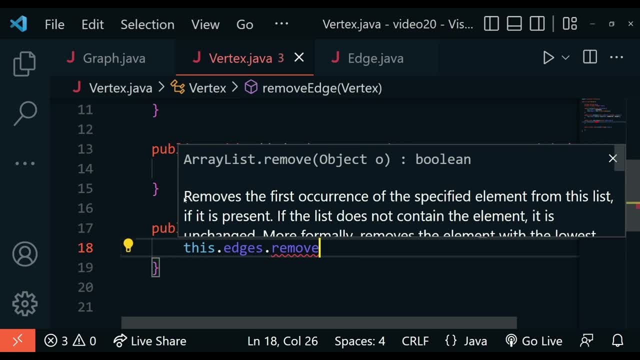 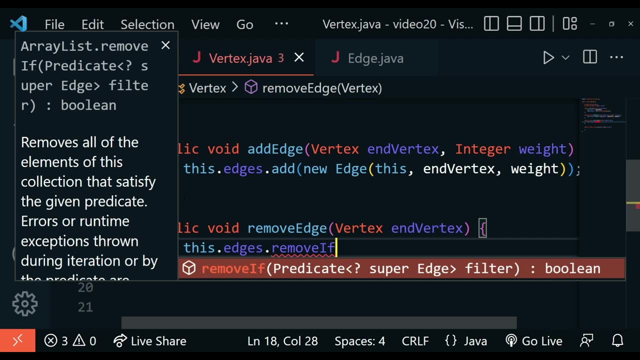 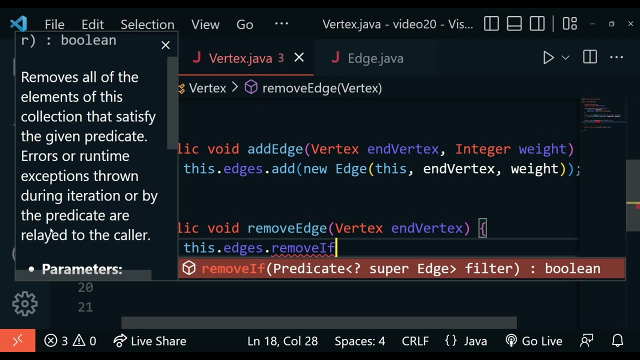 dot remove And the method for this is- since it's edges is an array list remove. if will allow us to add a predicate and remove All of the elements of this collection that satisfy the given predicate. errors at runtime, exceptions thrown during iteration or by the predicate are relayed to the color parameter here. 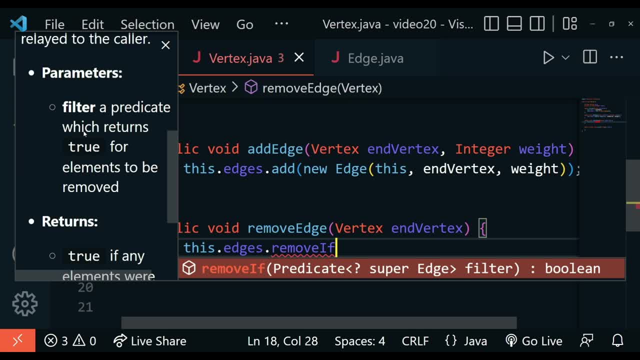 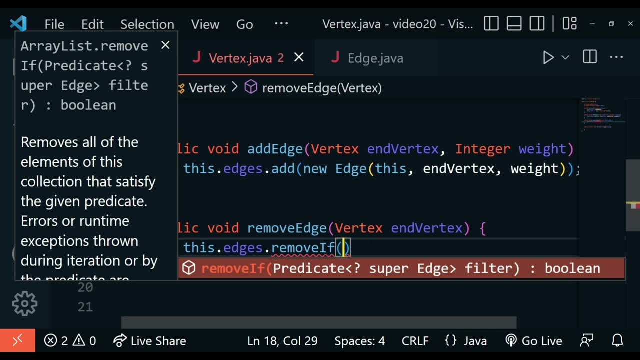 is a predicate, And here you can read it. it says: filter, a predicate which returns true for elements to be removed, And I'm going to add that predicate here. So over here I'm going to add in, So I want to remove that vertex. So here I'm saying: remove edge, right, And I'm in that vertex, So I'm in. 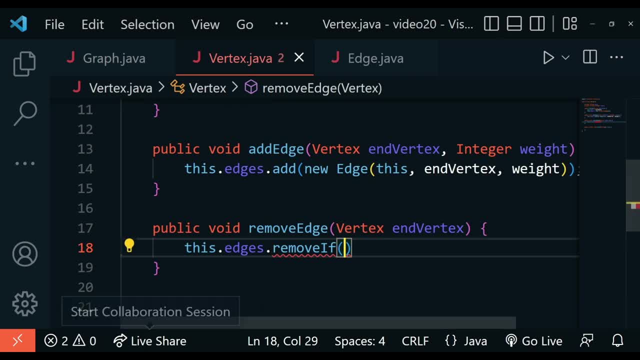 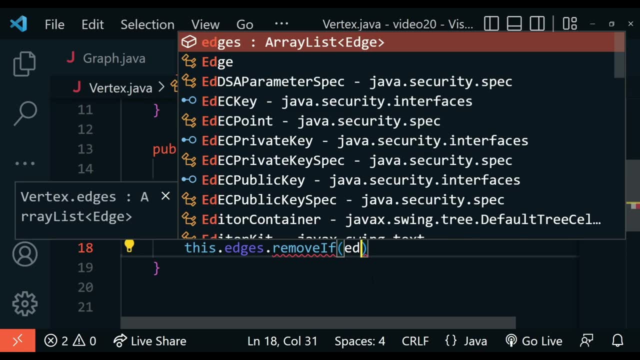 the vertex dot Java And I want to remove that edge that was passed in As this one. so n vertex right, I want to remove that edge from here. So I would say edges dot remove. if now say I'll remove that kind of edge right, and then we put this arrow bracket, So this: 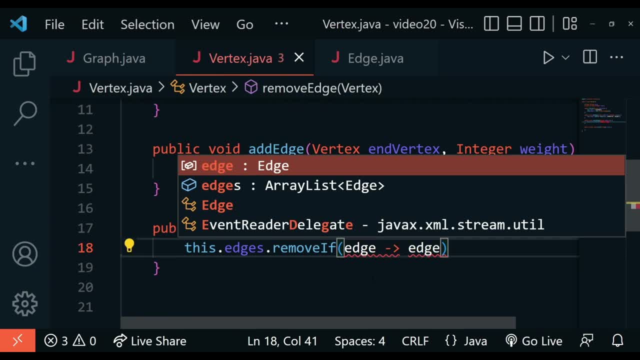 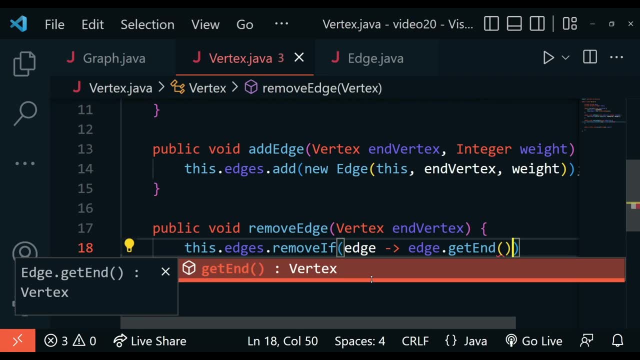 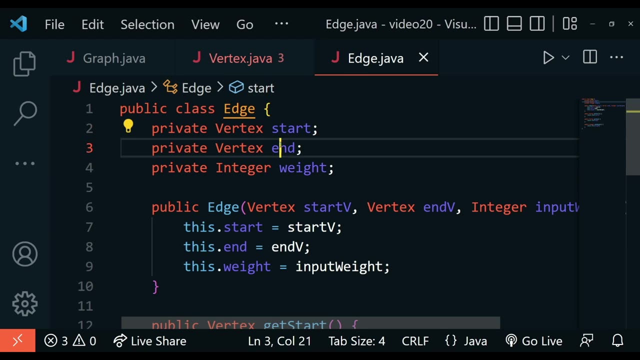 is the arrow sign, I would say edges, And then we say get. and because we're getting actually two things here, The edges are having two places. One is the first and the second is the end. So you can see in the code over here we have the start and the end, So the edge has two. 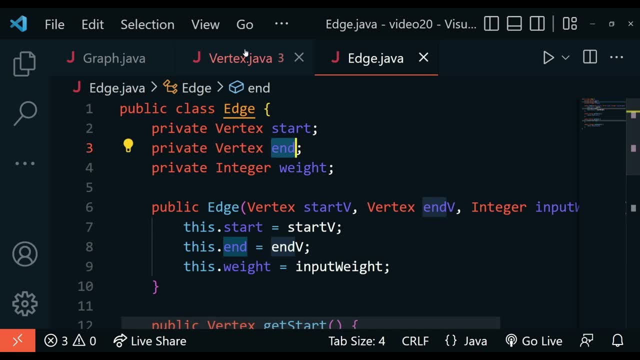 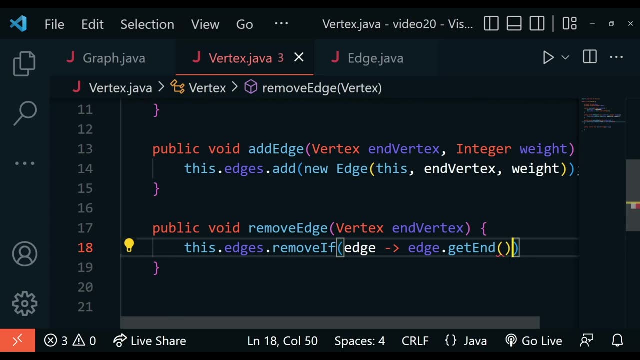 things And what we want is the end. So that's why we are getting the second one And that's going to be over there. So dot get end. And then we say dot equals. So we say, if that equals to the vertex. 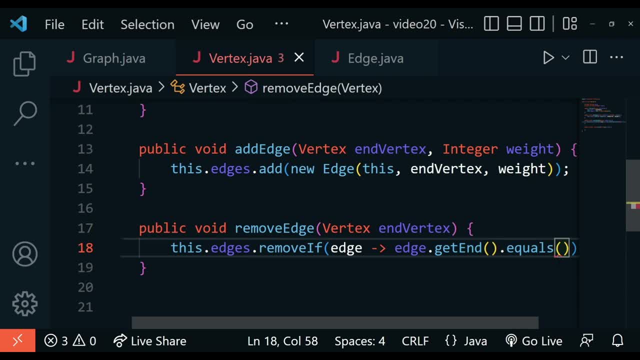 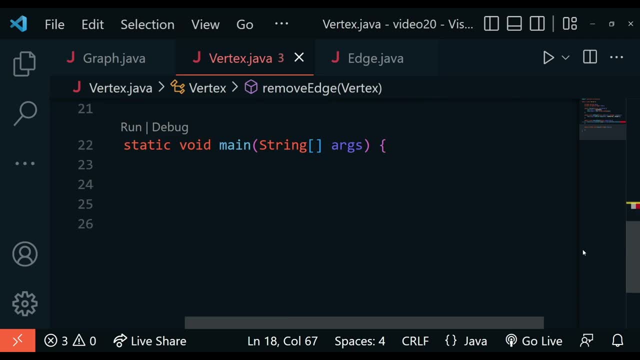 that we passed in here. I'm just gonna copy that and paste it here. If that equals, then just remove that from there. So we just need a semicolon here. If I could get a semicolon, All right, And that should solve. 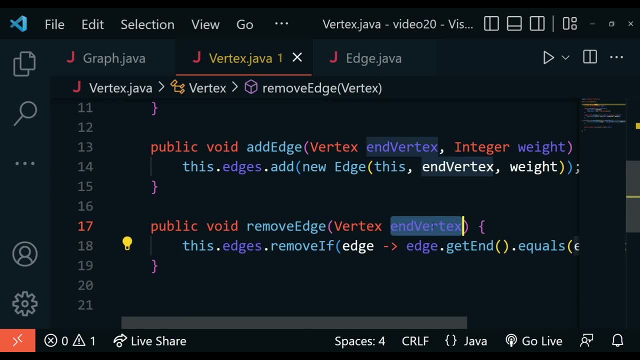 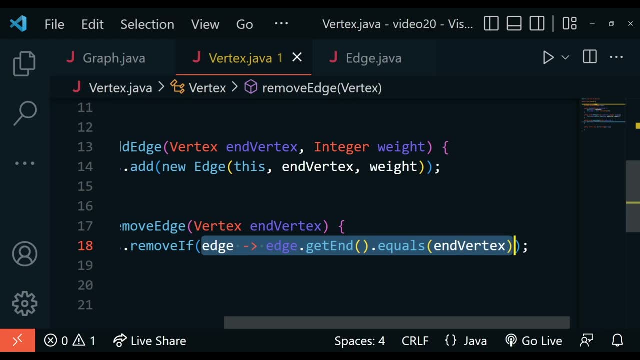 our problem here. So it's just going to remove that end vertex that we passed in as an input parameter And it's going to look at this: edges dot remove, if. and it's going to pass in this predicate logic that says: find that edge which has the end vertex equal to the end vertex that. 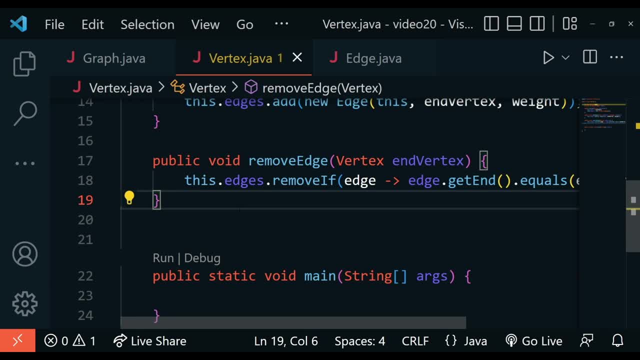 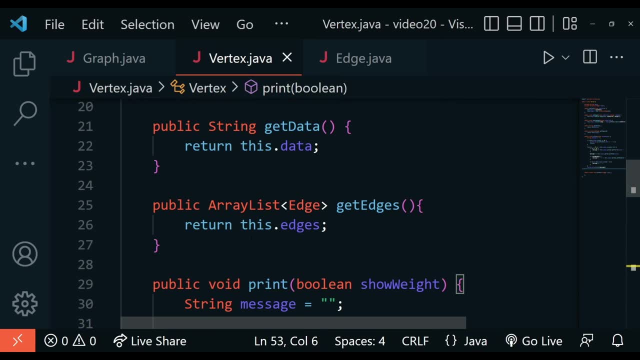 was passed in pretty easy, Okay. so now we're going to add in some other helper methods. I'm going to copy paste this as well, So just paste it here. So the first thing. let me just first zoom out And 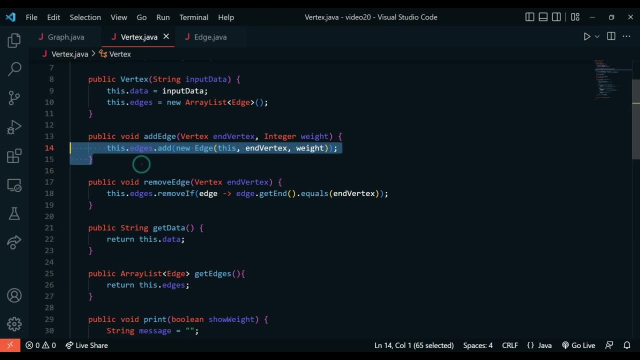 show you what I've done. Here we have this remove edge And we have the add edge, Perfect. Over here we have this get data method. it's a string return type And it's just going to get the data for the 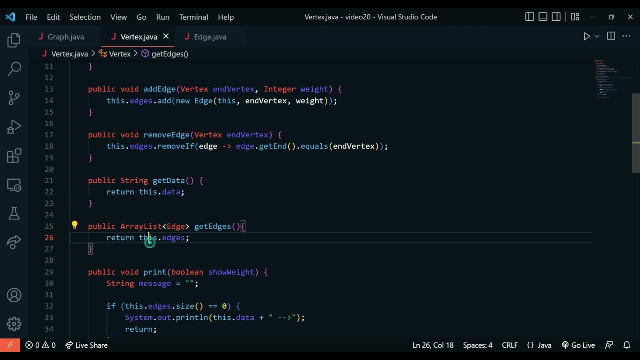 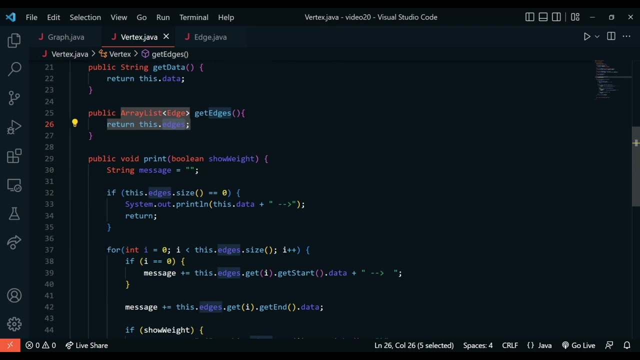 vertex- pretty easy, straightforward- And the array list edge. So this is the return type And it's saying get edges. So it's just going to return the the edges that the certain vertex has. So it's just going to return the list of it, this dot edges. All right, Now over here we have a public. 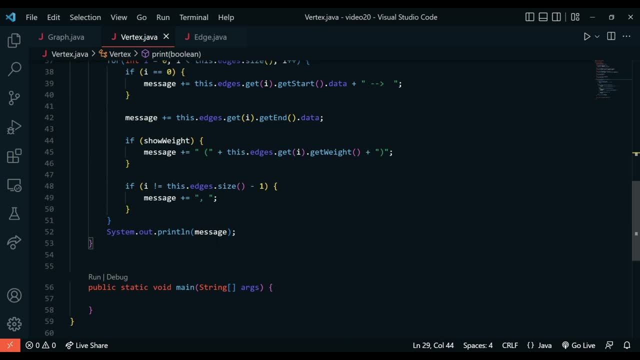 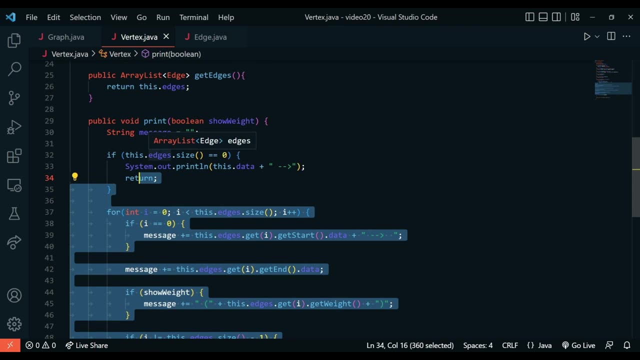 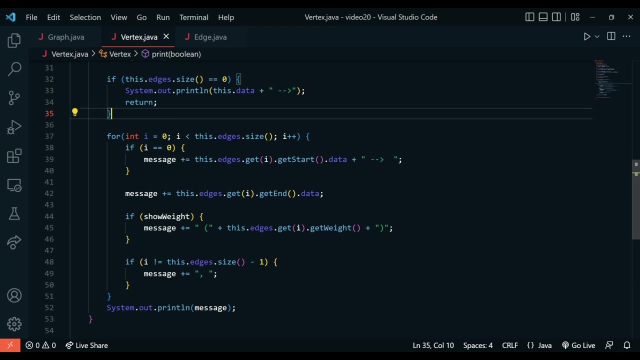 void print Boolean: show weight. So over here we have this print method that's just gonna allow us to visualize our implementation And it's just going to show us how the graph is looking like inside of our structure. So it's pretty easy. you don't need to go into detail for this, And if you want to, 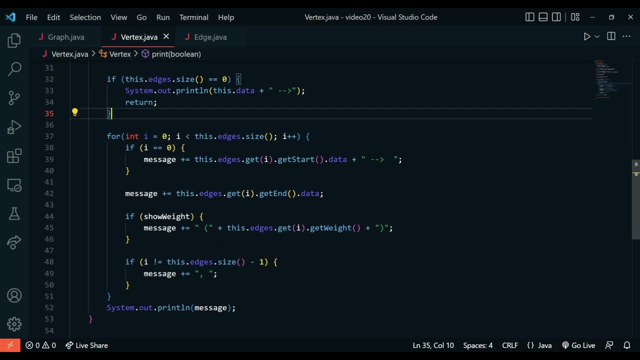 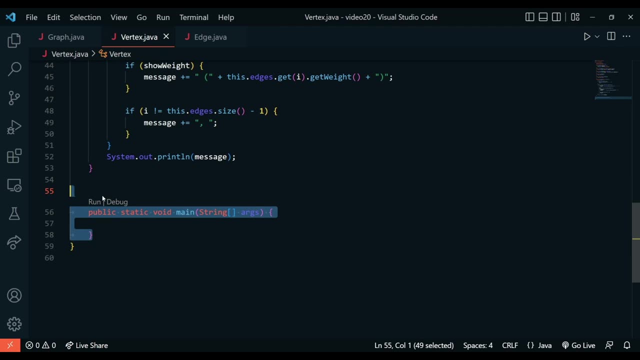 write this down. you can pause the video and start typing this in: We're done with the edgejava, And we're also done now with the vertexjava. In fact, I don't even need this main method here, So I'm just going to remove that here. 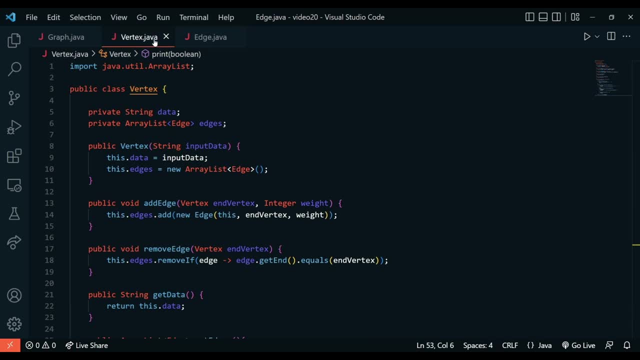 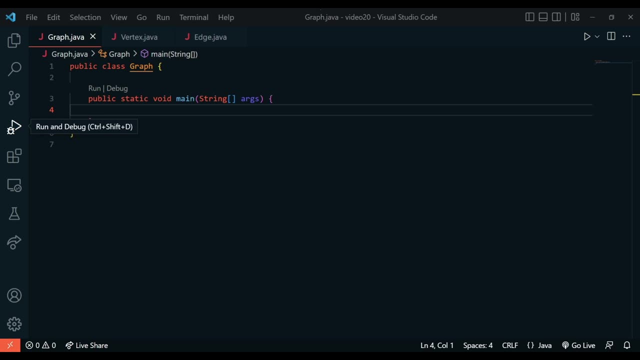 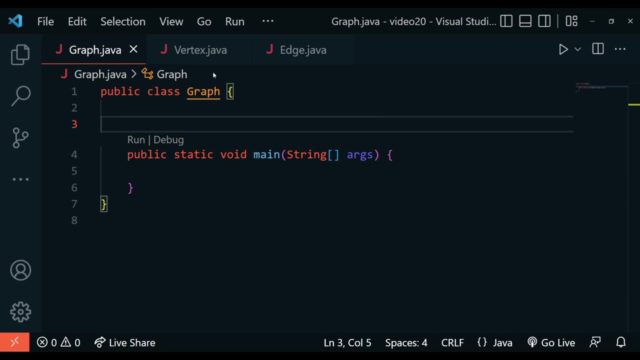 Now we just have this. So the vertical edgejava and the vertexjava are done. Let's go to the graphjava, the main thing, the main boss. So over here, we're just going to add in the following things: Remember, like I said, a graph is a list of vertices. That's exactly what we want to do. 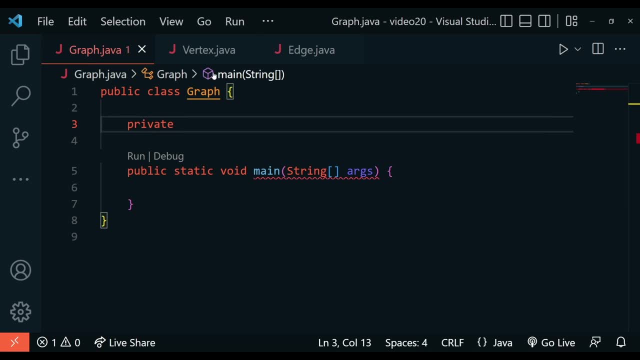 here. So I'm going to say private And I'm going to say array list And I'm going to put in the type here. the type for this is vertex, because we're putting in vertices and we're going to to pass in vertices, like this is the name. Now we also have a type which I specified, that there. 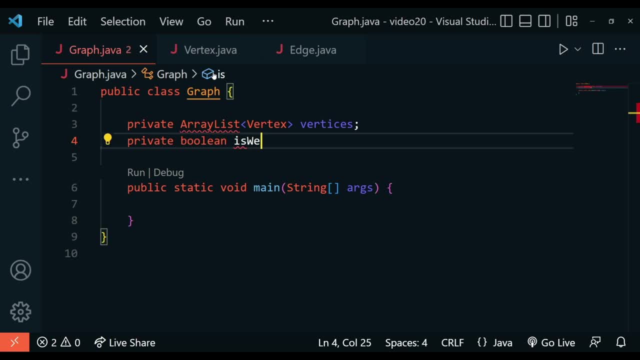 could be different kinds And my graph will be a weighted graph. So I'm just going to put in: is weighted Boolean variable. I'm also going to put is directed Boolean variable And this is just going to tell me if the graph is directed with arrows or if it's unidirectional or bidirectional. 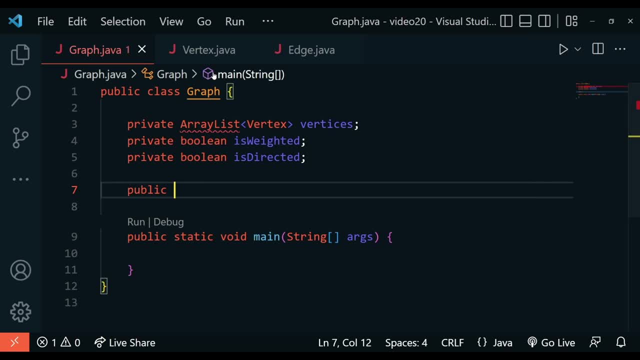 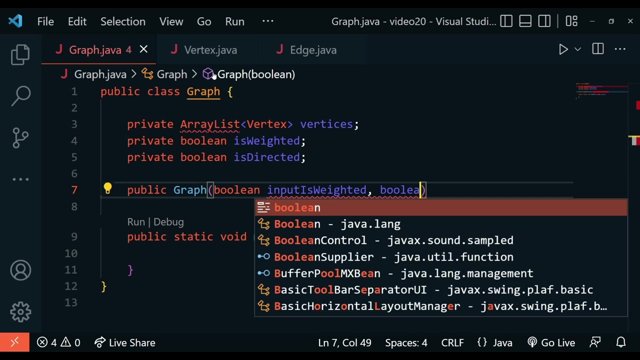 So that's, that's the thing. Let's create a constructor for the graph And we'll just say public graph, Graph, and then we'll just pass in Boolean And we'll say: input is weighted. So the the things that are passed in will be determined by the user And Boolean input is directed. 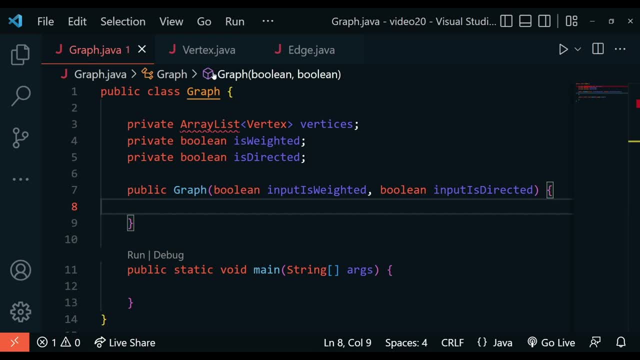 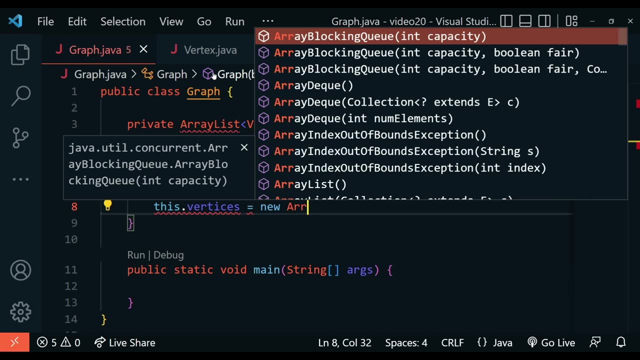 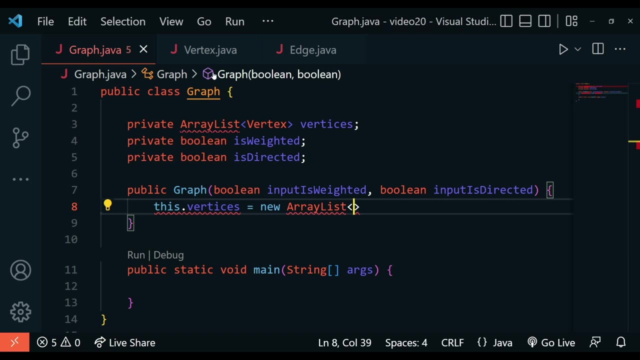 So we're done with this, And here we're going to have the this dot vertices And we're going to say new array list And we're just going to pass in. So over here we have graph and then we have Boolean input is weighted And then we have input is directed. So 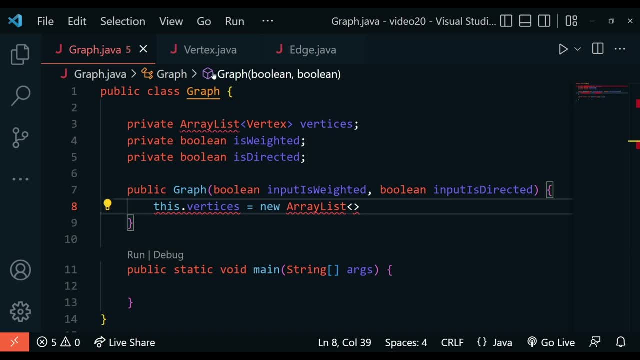 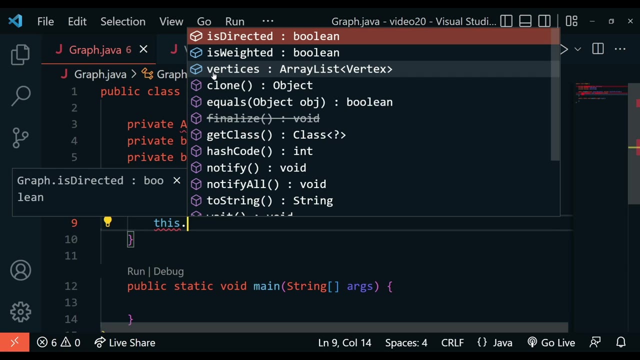 like I said, we have to first initialize the vertices array list. So I'll just say: new array list, put the round brackets and then the semi colon. this will initialize our vertex, This will initialize our vertices list. And for the weighted thing, so we can say: is w e, weighted is. 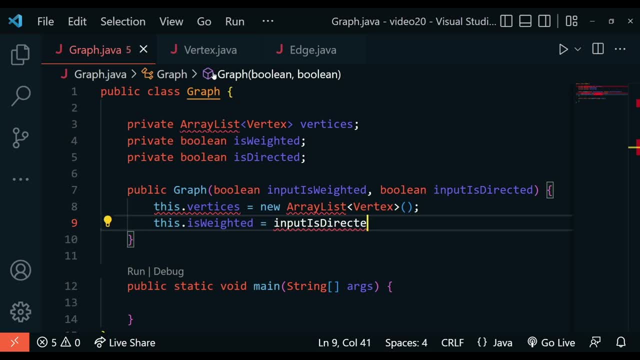 equal to, and we say input is weighted. So w, e, i, g, h, t. For the other one, which is directed, so is directed is equal to, input is directed. There you go, Cool. So now this is created And, yeah, I have to import the array list as well. So just import that. 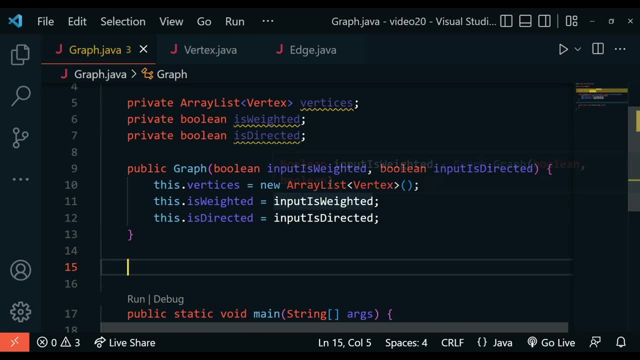 as well. Now let's create some methods, And the important methods that we want to do here is that we want to create a method that will allow us to add vertex, add some vertices to our array list, And the name for that will be self self explanatory: It's called vertex And that's a. 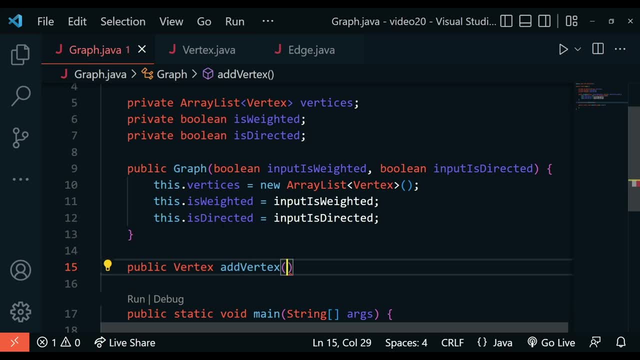 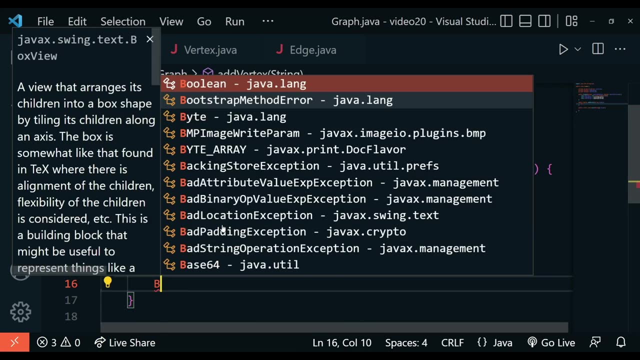 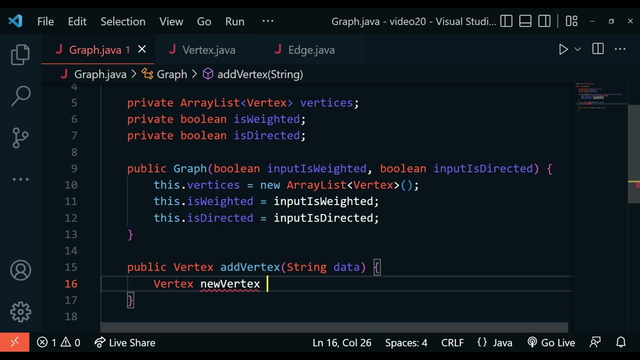 return type, So it's going to be called add vertex. The data that will be passed in was a string, And over here we'll say vertex And we'll say new vertex. And over here, we're just gonna create a new vertex here. So we'll say new vertex And. 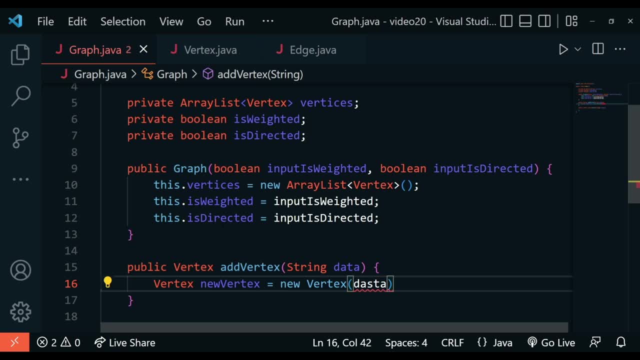 we'll pass in the data that was passed in And over here we're gonna put that inside of our list. So we'll say vertices dot add and we put the new vertex semi colon And then we have the return new. 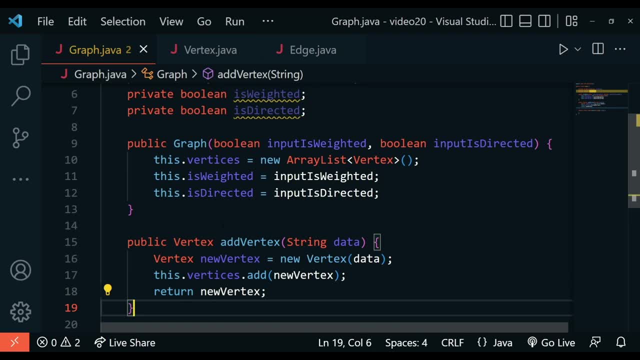 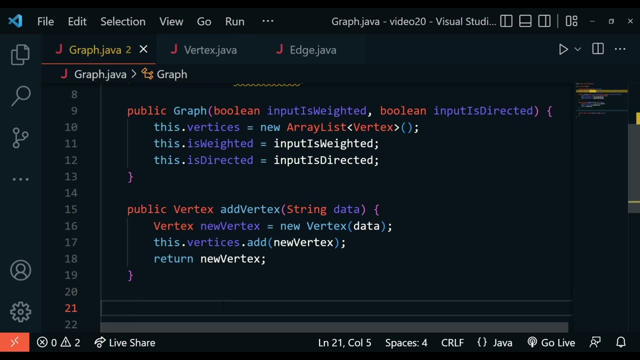 vertex. Cool, So we're done with this. That's the add vertex method And it just returns us the vertex, So we'll have to assign it to a variable in the main methods. Now we're going to create the public void. 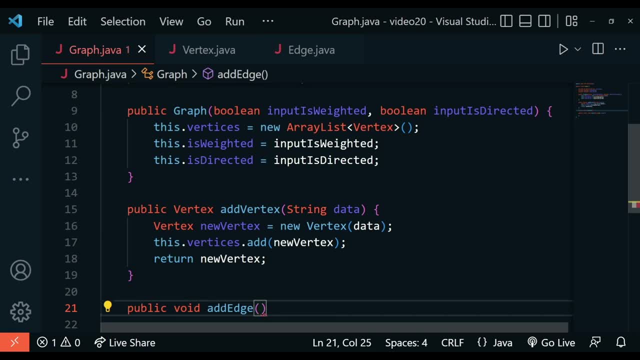 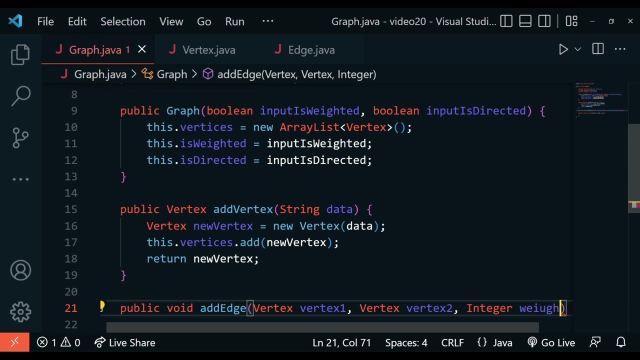 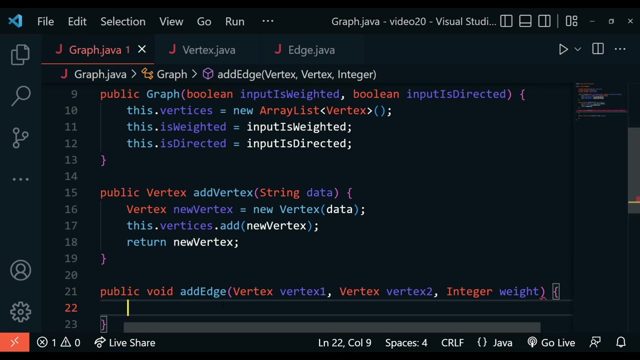 Add edge method And this will allow us to pass in the vertex vertex one, the vertex vertex two. So this is the start and the end vertex and the integer weight. Like I said, I wanted to create a level of abstraction here, So I'm allowing our graph to have the add edge functionality as well. So over. 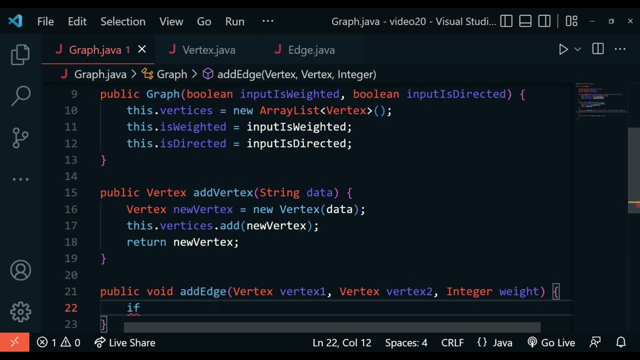 here it's pretty straightforward If I said if the thing is weighted then there's going to be no weight for this, because I passed an integer weight And I have to first check the Boolean variable here. So if I say is weighted, not directed, but is w, e, I, g, h, t, Now if the weighted 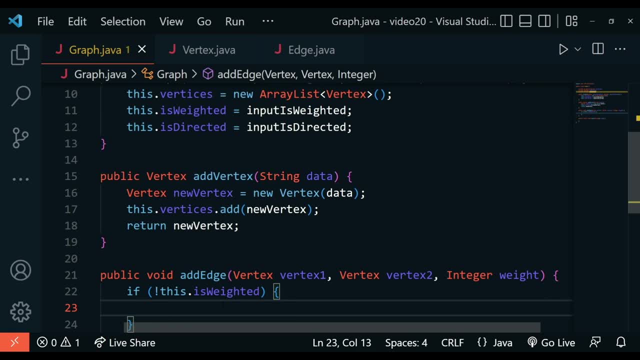 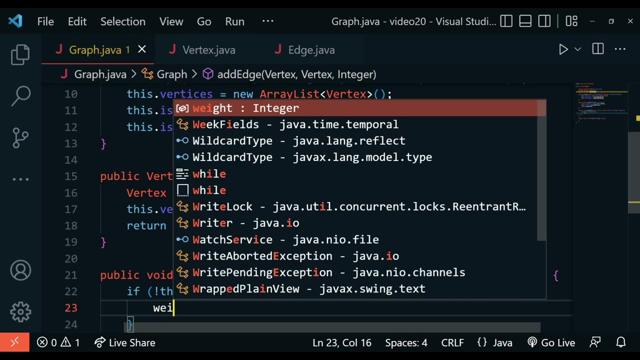 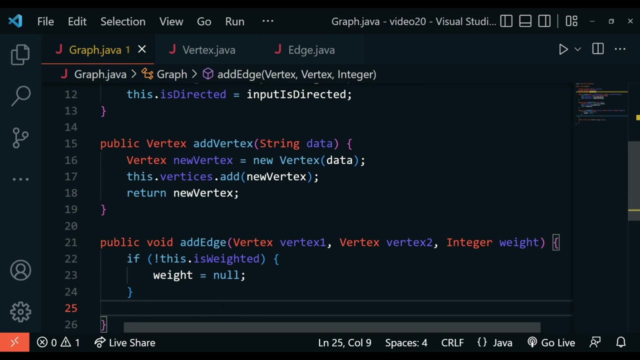 was false then. so it says: if weighted is false, right. So we'll just say: the weight that was passed in will be assigned as null, All right. And that falls meaning if the thing is weighted thing, so we'll say: vertex one, dot, add edge And over. 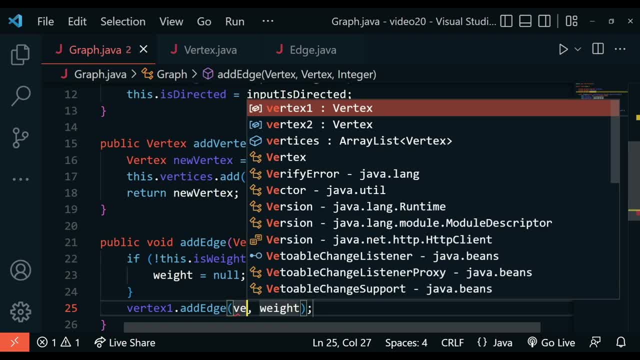 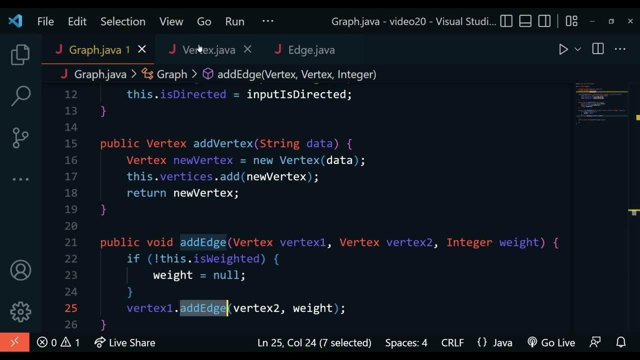 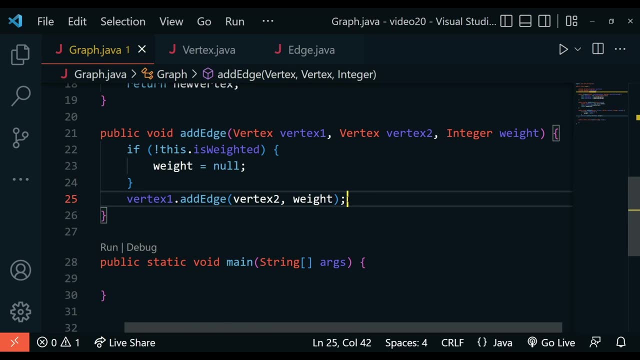 here we're actually adding the vertex two, And here the weight will be passed in as well, And this is the add edge method. that's from the vertex class here. So the vertex add edge, this one. Now over here we want to actually add in the other thing around as well, because we don't need 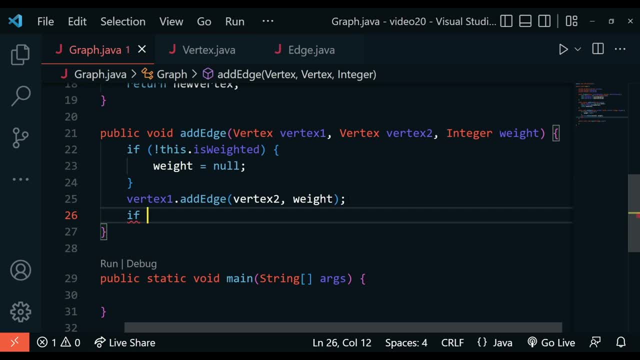 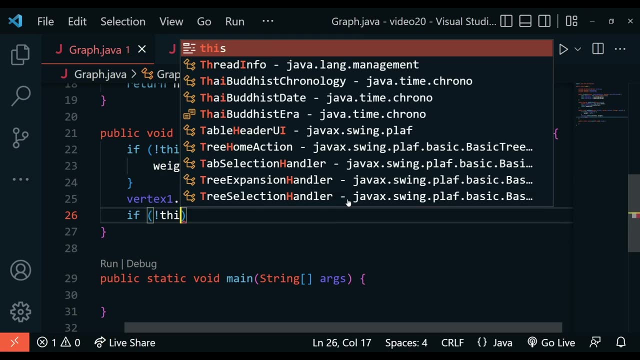 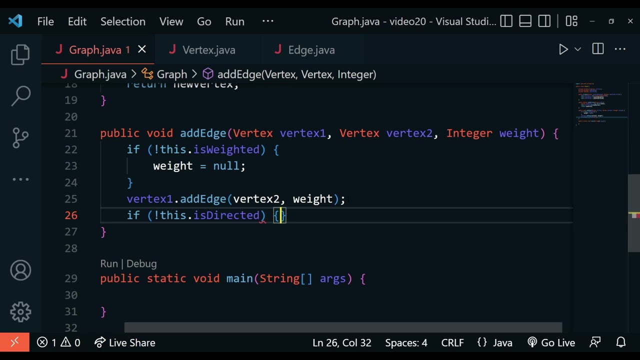 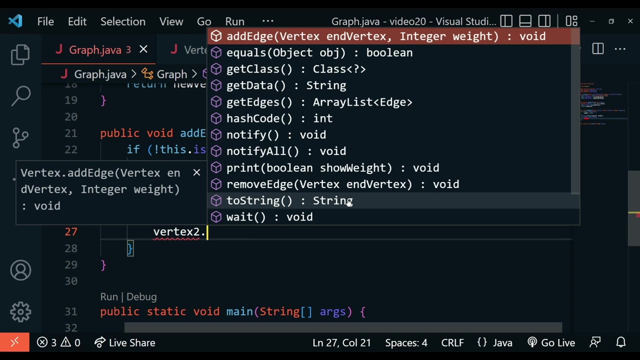 the add next, such as if it's unidirectional. so if it's undirected, than both right, And if it's directed, than this one. So I'll say: if it's not directed, than both. so this dot is directed, if it's not directed, Then we'll have the vertex. Vertex, two dot, add vertex, Or yeah, so vertex. 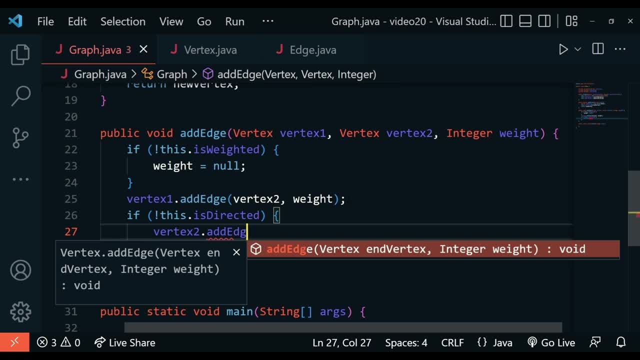 two dot. add edge here. oh, just once I tell you, here I'm going to sit down and I'm going toethier. we're gonna add the edge And we're gonna say vertex one, And we're also going to put in the weight over here as well. And 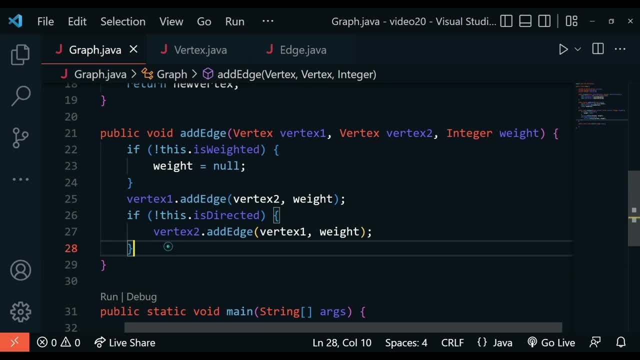 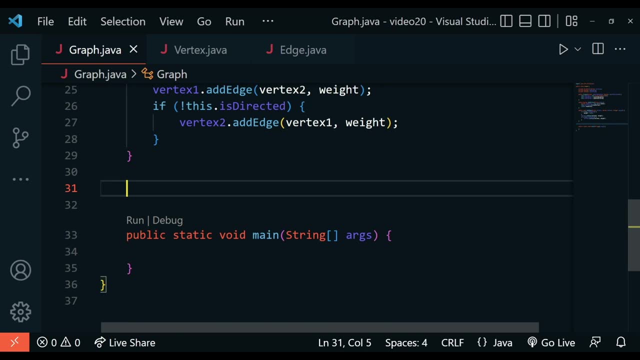 there you go. Similar to how we created the add edge method, we now need to create the remove edge method. So let's go here a little down And let's add the remove edge method. So we're just like I said. I'm giving that the power to the user to do. 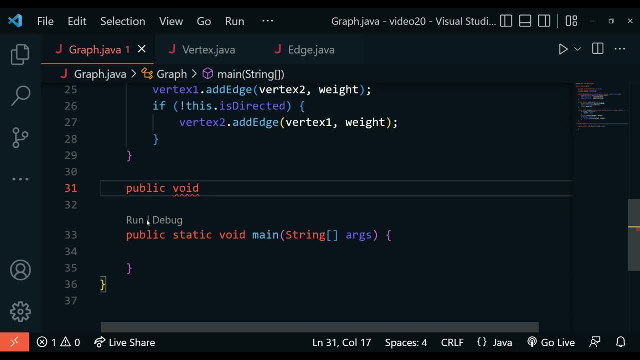 all of this So, and the user doesn't even have to know how the vertex Java or edge Java works. So that's the layer of abstraction that we're creating here. remove edge EDG And over here we're gonna pass in the vertex And we'll say: 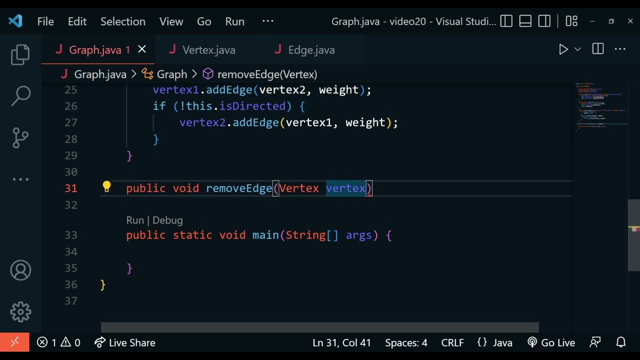 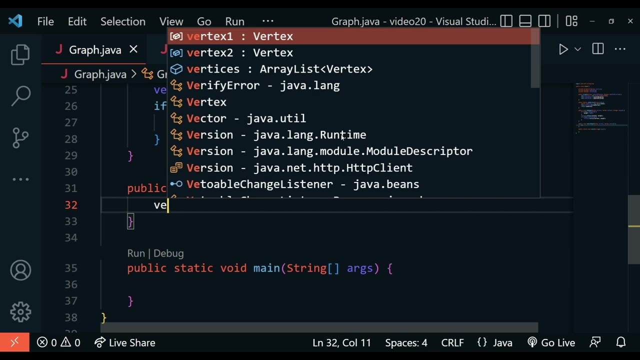 vertex. So to remove the edge, you'll have to need- you'll need the vertex one. you'll also need the vertex to remove it. Now, to remove it, it's pretty simple. We say vertex one, dot remove. this is the method that was there. So 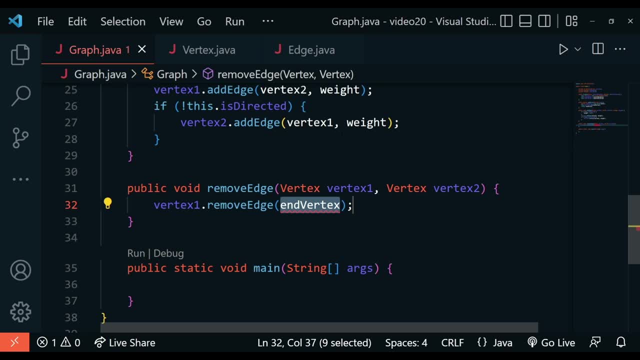 remove edge and it takes another vertex And we have the N vertex here. we're just gonna pass in the vertex two And there you go, And then, like I said, we have to check if it's not directed, if it's bi directional, then we have to remove. 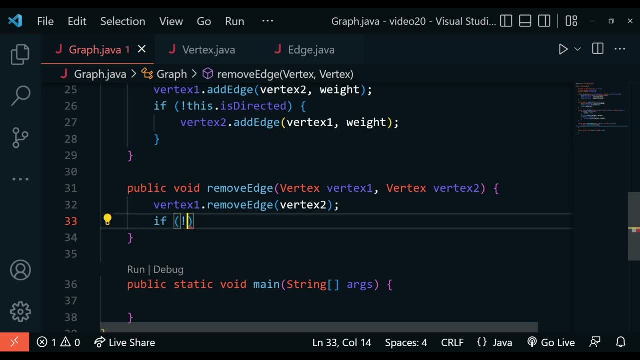 the other way around as well. So I'll say: if this dot is directed, so if it's undirected, right, so if it's bi directional, then we'll have to move the other way around as well. using vertex two, dot remove edge and we put in the vertex one, Okay, so that. 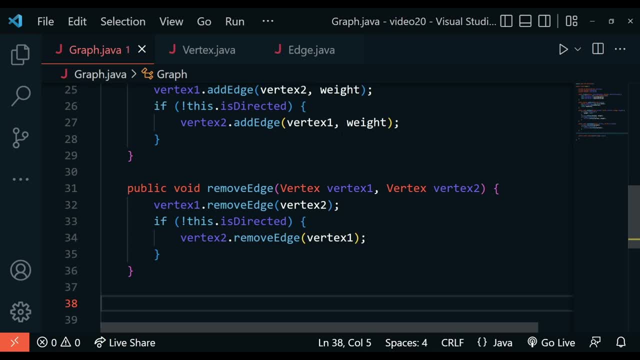 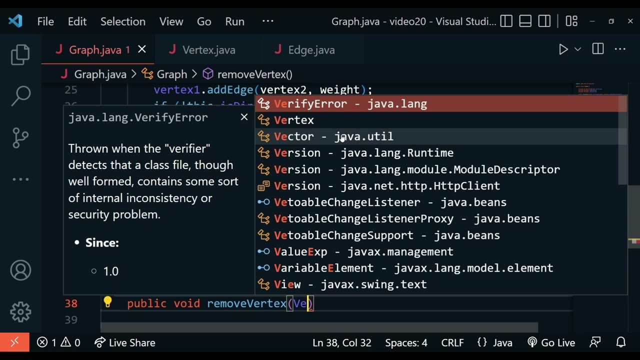 was pretty much it with the remove edge. Now we have some other methods like remove vertex, So I'll just add in them to move vertex quickly over here: void remove vertex And for the remove vertex we have the vertex that's passed in. 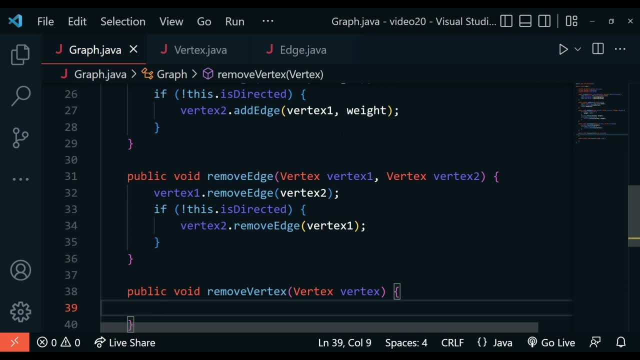 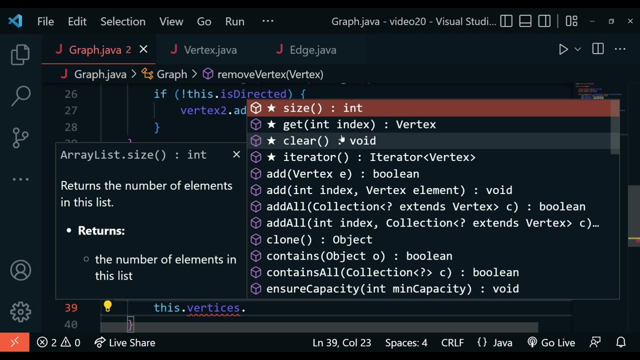 here. So we're going to use the remove method. So I'm going to just paste that in And let's see, I'm going to say this: dot vertices, which is the list that is existing here in this class, this instance variable, And we're going to use the remove. 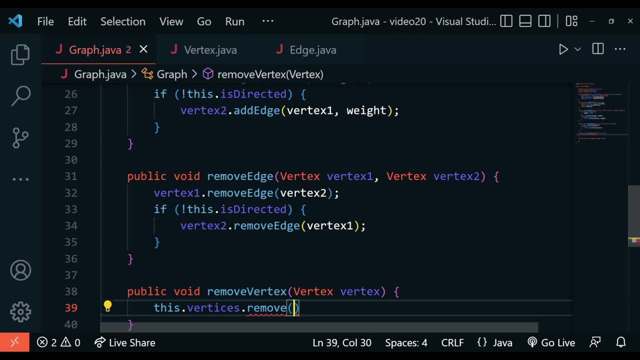 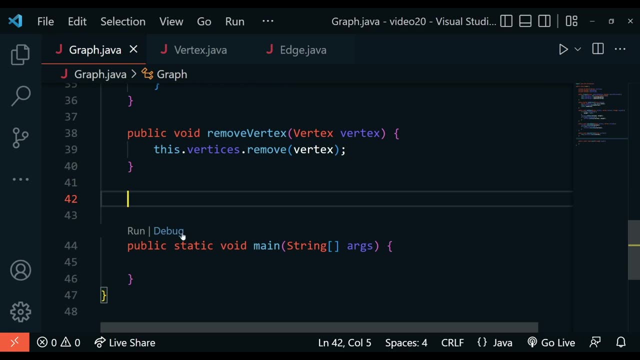 method. that's provided by the array list, And we're just going to remove the vertex that you just asked for, right? so that's just going to be removed here Now. to save some time, I'm just pasting some helper methods that we also need here, So I'll just 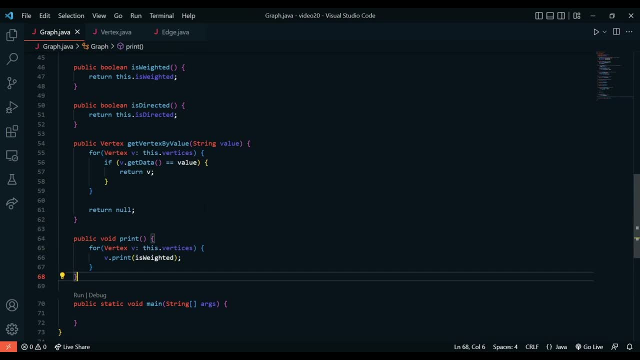 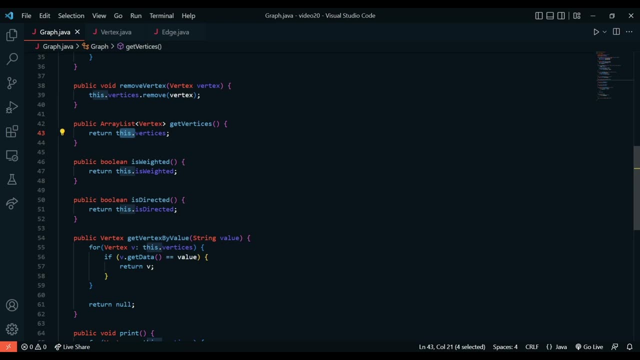 paste that in And let's see how it looks like. So here we have the get vertices, the remove vertex, the get vertices method. it just returns, the relist is weighted, is directed, So that the last thing, what we did, was this one, which was remove the vertex, And then 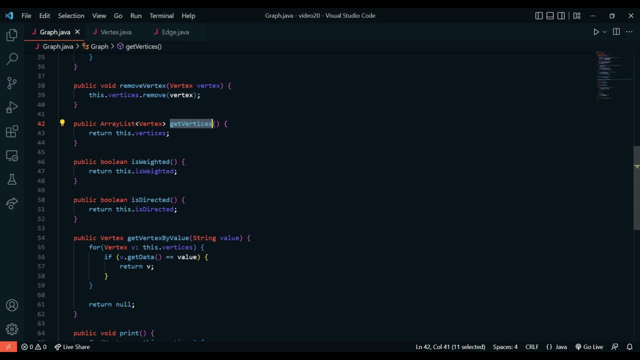 after that: this one is just a get vertices. it's just going to return the array list vertex. So the whatever the array list is, it's going to return all the vertices here inside of that current graph. public Boolean is weighted will return if the graph is weighted or not. And 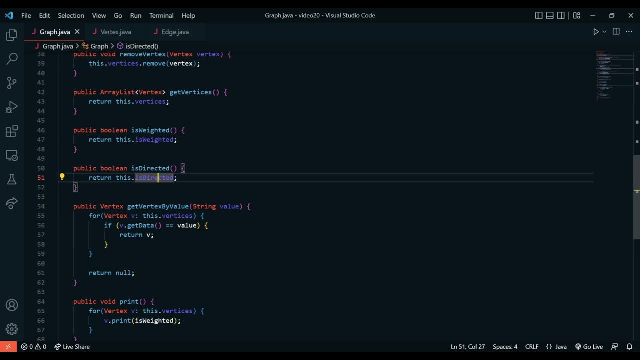 Boolean is directed will turn, if it's directed or not. Public vertex. get vertex by value, passing a value, And it will loop through this for condition it's going to go vertex. So you pass in a string value and you're trying to look for that. 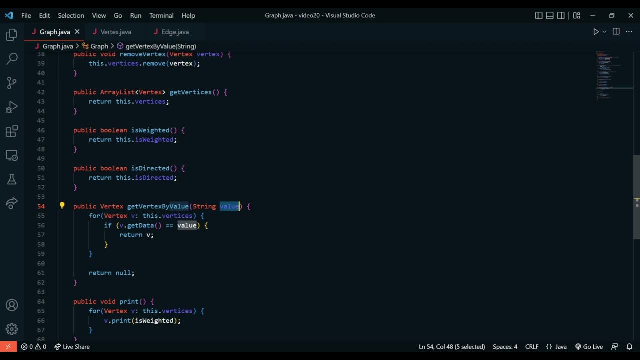 vertex for that kind of value. So let's say I have a stop in New Jersey, let's say Jersey City. I'm looking for Jersey City stop for my bus. you know bus route. So in the bus service that I'm trying to map out here, let's say I have Jersey City. 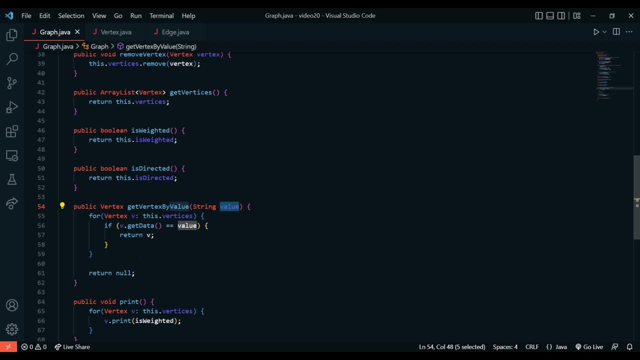 pass in here now. I'm gonna have to look for that stop if it exists in this entire bus ecosystem, So if it exists in the bus routes, if, if there is any kind of bus stop that has the name Jersey City, and then it will be returned here. So 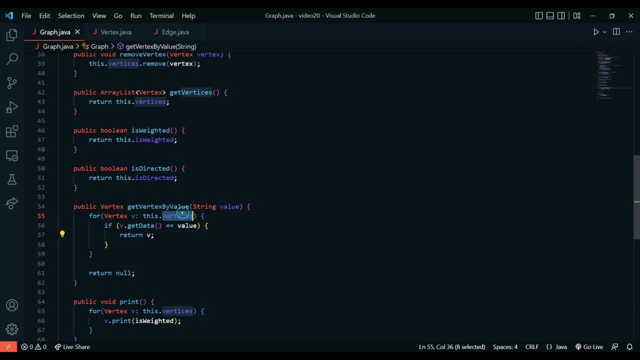 over here. I go for each loop And it says: over here the vertices are list. So I'll say for every vertex v if the value. so I'll use the get the data value and this vertex. remember that I created get. 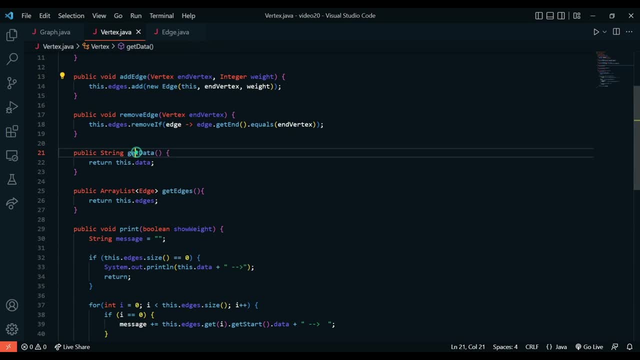 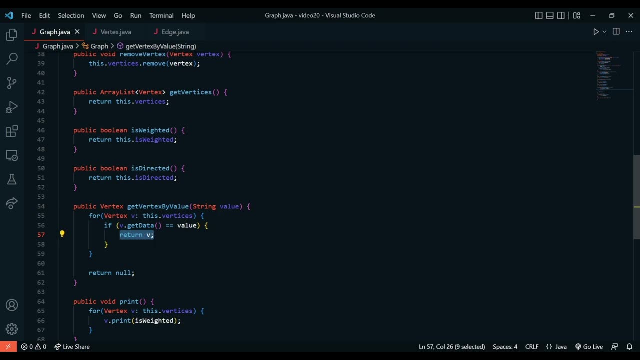 data over here somewhere, So it's supposed to be somewhere over here. there you go. it returns a data string And if it equals to the value that was passed it as an input over here, then we'll return the V vertex and then you'll have it as a. 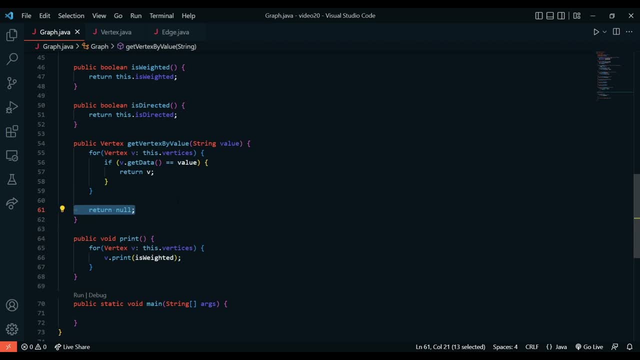 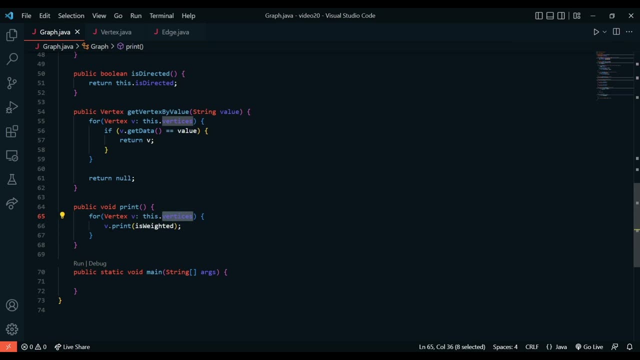 vertex here, So perfect. And if it didn't exist, it will just return null. So that will help us know if the vertex exists here or not. And now over here, if you want to print it. so for vertex v in this dot vertices, V dot print and we have is. 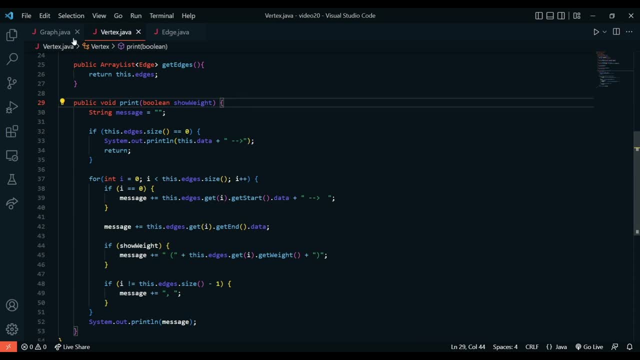 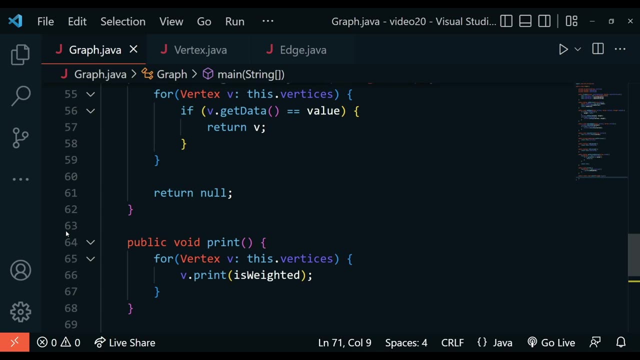 weighted. So you know the print method that we created here. this will allow us to see all of these vertices, And here's what it's going to look like in action. Awesome. Now let's create the main deal here. Let's create some graph. 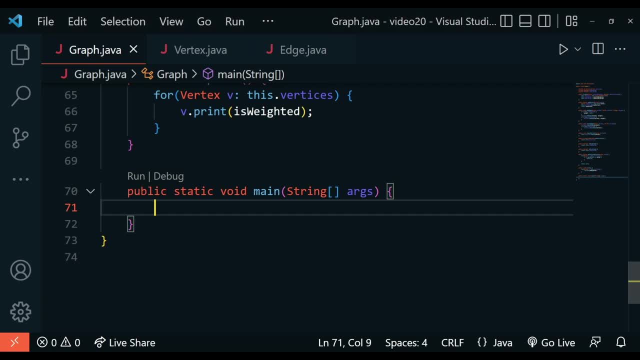 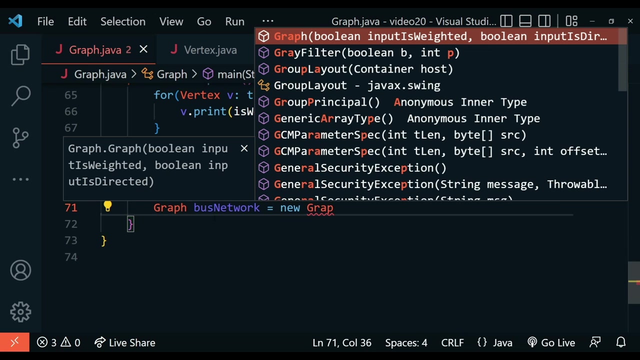 Let's create the graph data structure And let's try to map it out. And I'm going to remember I said I'm going to create a bus station, So I'm going to say gr a, ph and I'm going to say bus network And I'm going to say new graph And 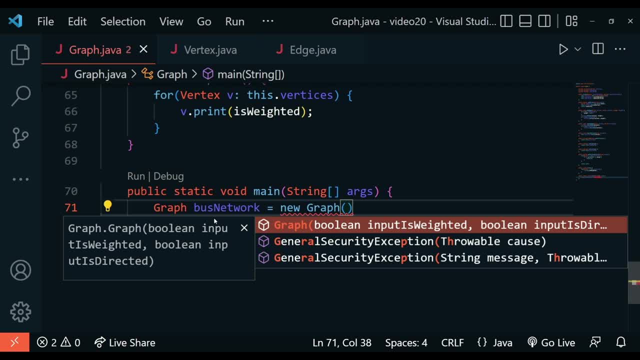 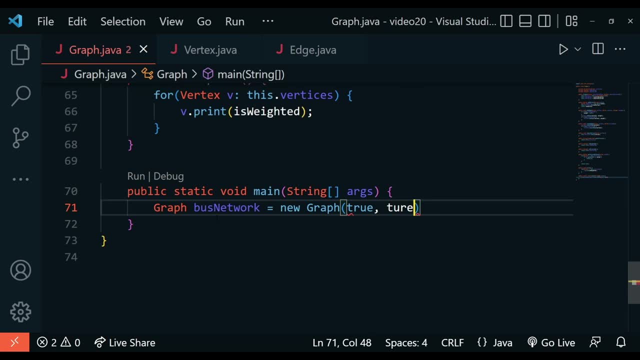 over here we're going to pass in is weighted. And for the director thing, we're going to pass in both, true, true. So t r u e and t? r? u e. Now let me tell you why I did this. The first one was input is weighted. 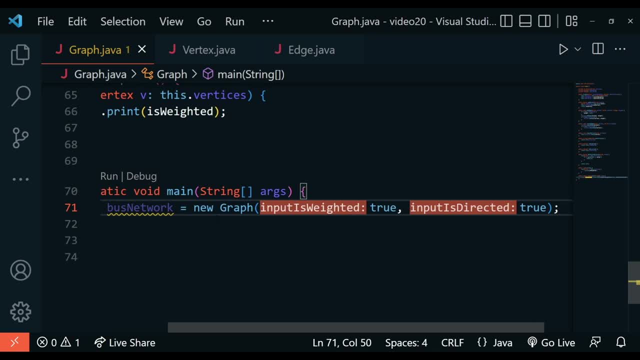 So it is weighted, there's going to be values associated to it. So for every edge there's going to be some kind of distance and input is directed, meaning that there's going to be some kind of arrow and it's so it's a, it's not bi directional, It's not two ways, It's. 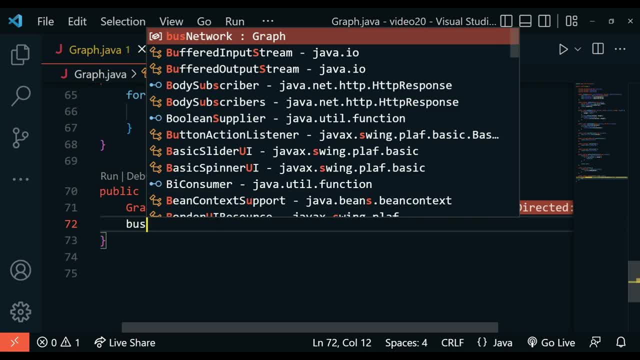 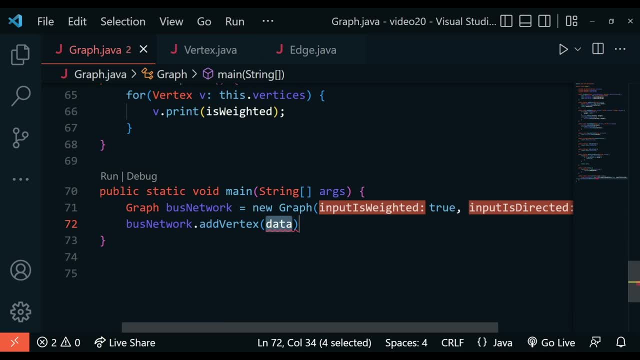 just one way going forward. So bus network, And I'm going to use the add vertex method that we created here in this method. So it asks us for a string data And we'll just say: let's say Clifton, And here we have it, semicolon. But remember that this add vertex 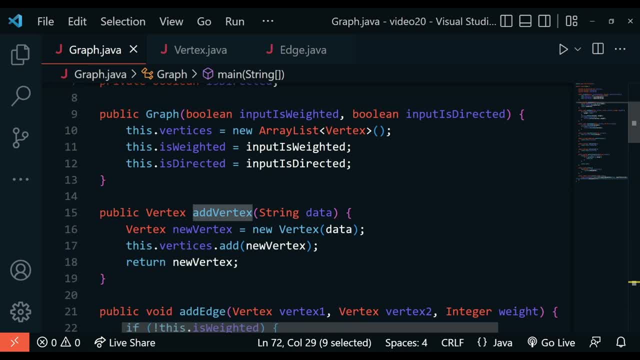 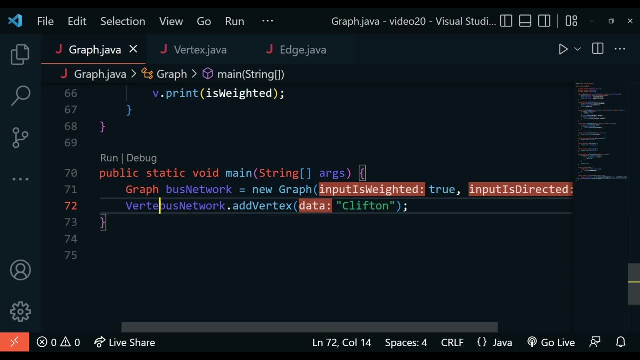 method. if you go, if you go and see the method here, it's actually returning a vertex. So we're gonna have to store in some kind of variable. So let's store it in a vertex And I'm going to call it a vertex. And I'm going to call it a vertex And I'm going to call. 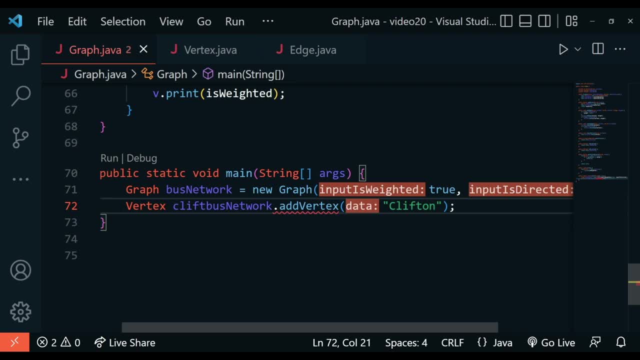 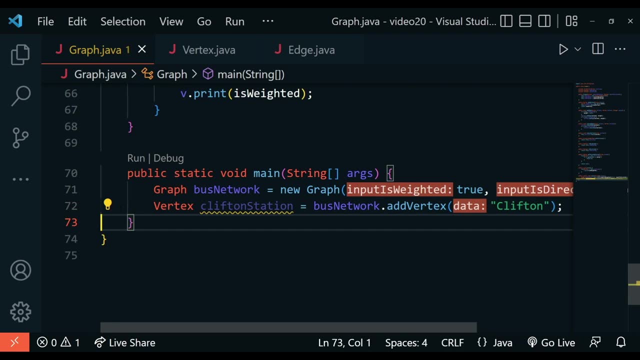 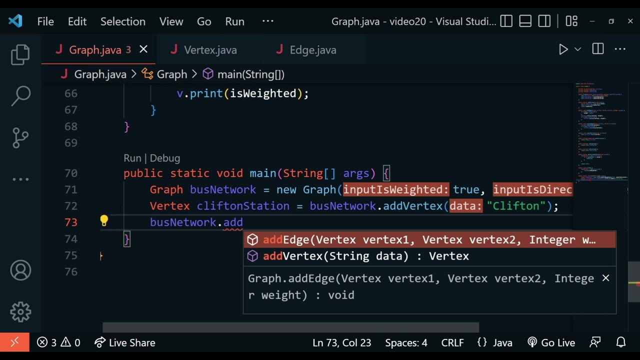 this as cliff Clifton station And equals to that. So there you go, And the same goes for the next one. So I'll say bus network dot, add vertex, And we'll take vertex And over here we'll have the next station. I'll just add a Cape May station And let's have 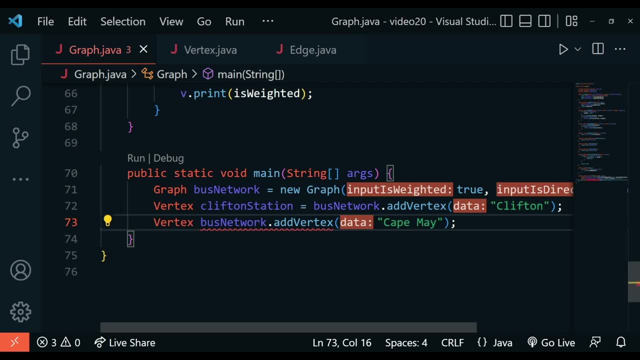 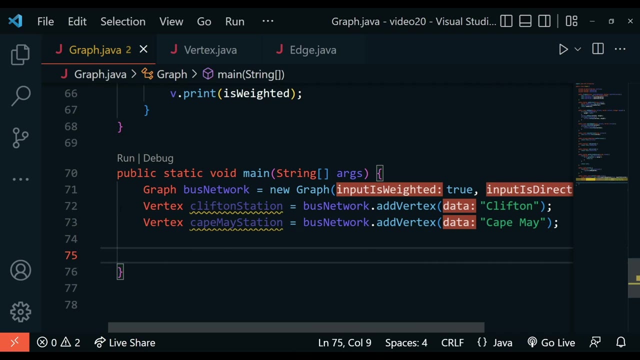 the vertex here as well. So vertex, and I'll say Cape, Cape May station, And just there you go. So we created two stops And I think that's enough for now. So now what we have to do is add the edges and the connections between them. So we use the, you know the. 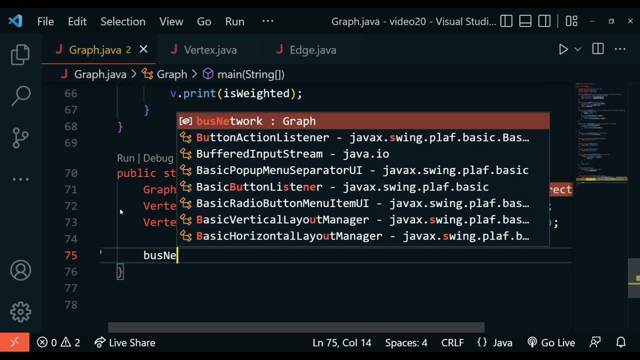 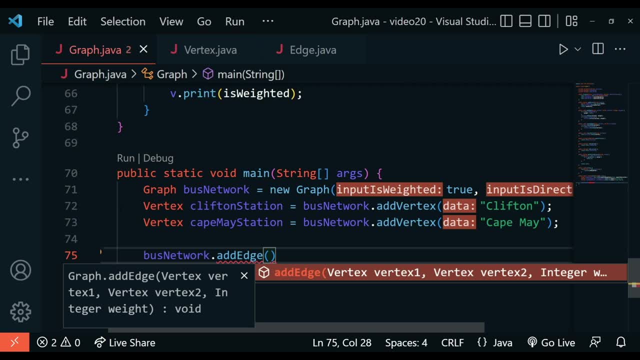 add edge method. So we'll use bus network And we'll say add edge. And we'll say add edge. And to add edge we have to put one station to the next. So we'll say Clifton station And we'll say the Cape May station. So that's the connection. And we'll also have 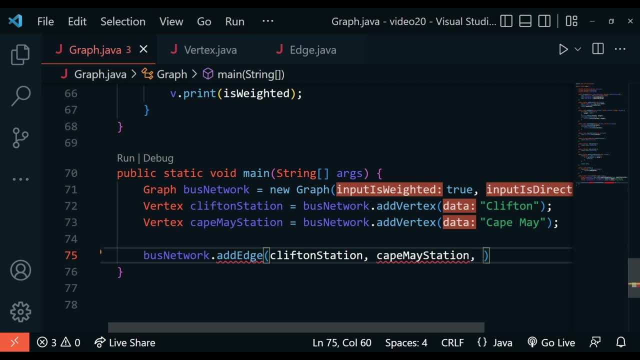 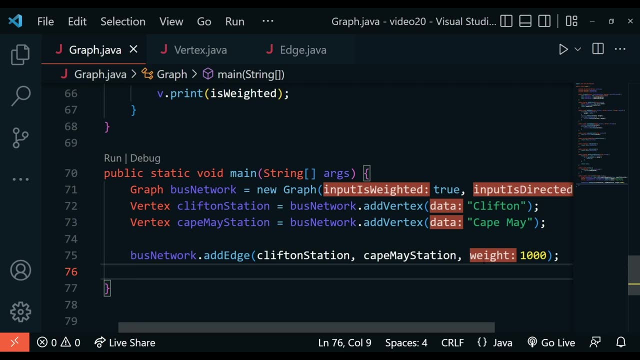 to put a weight left, to put a weight as well. So I'm going to say it takes 1000 miles to reach there And that's our weight. Cool, Now it's connected, And remember that I'm not putting it. So I'm just putting it one way and it's just going to connect it. And 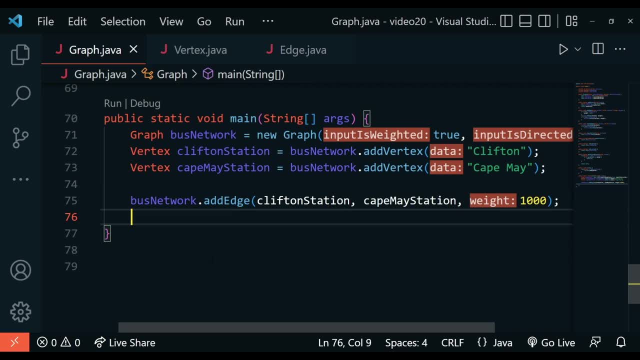 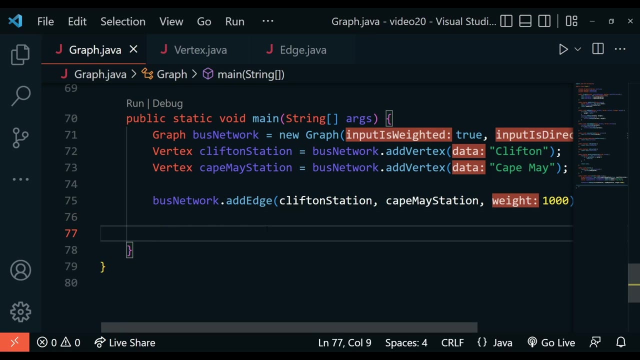 that you know, directed way. Here we have that. If I wanted to remove an edge, it would remove it using the same. but I'm just gonna say bus network dot remove, edge and just pass in the same two things, not the weight that time. In this case, I just want to print it. 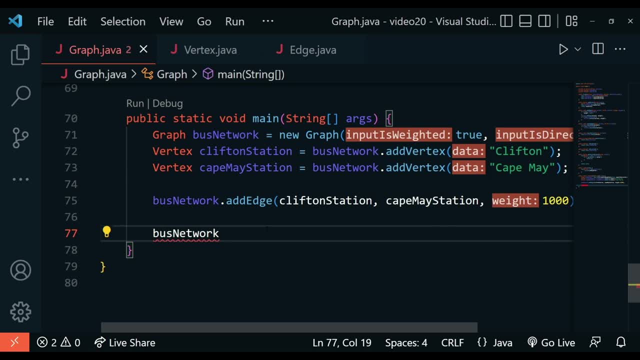 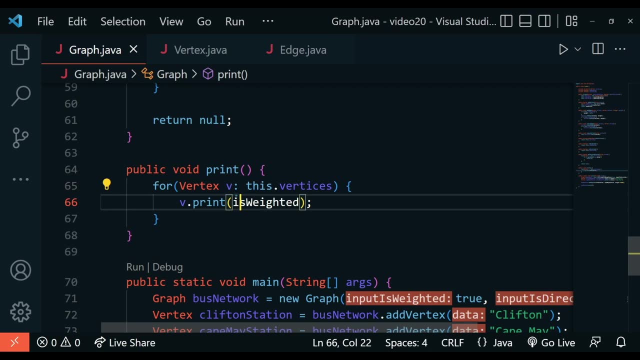 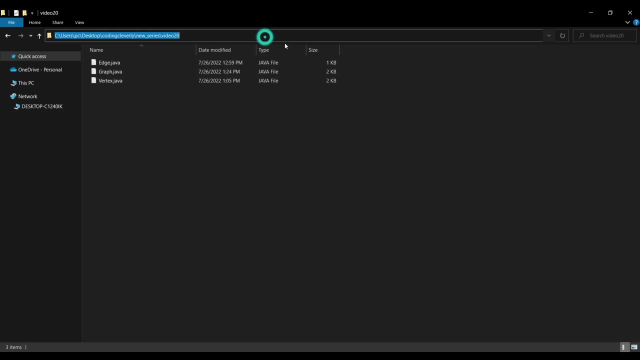 out and see how it looks like. So bus network dot print And this is our method. that was that is created here and actually calling all the vertices. So it's going to be printing it through here- Awesome. So let's run this baby up and see how it looks like. So I'm going to command. 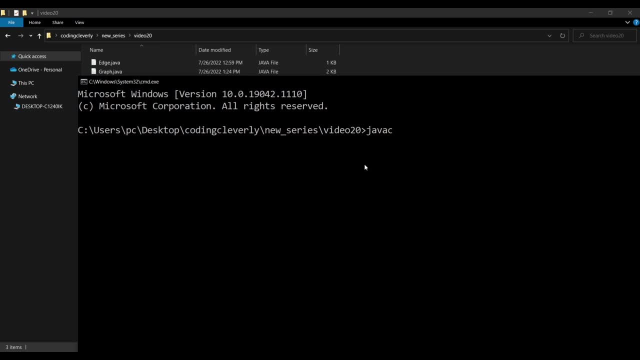 prompt here And I'm going to say Java C. the name of it is called graph Java. it compiled And now after that I'm just gonna paste here. So over here we have the direction from Clifton to Cape May and it takes 1000 miles. So that's exactly what we did here. Let me just minimize. 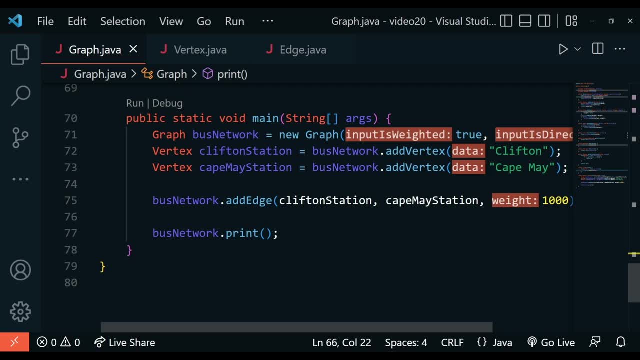 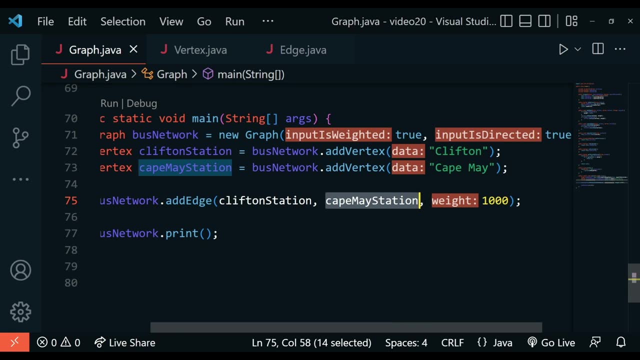 it quickly And go back here. And if I look over here, I actually created a direction from Clifton to Cape May and it takes 1000 miles And I didn't do the other way around. Like I said, this was not undirected. it was directed because it was set to true And here, 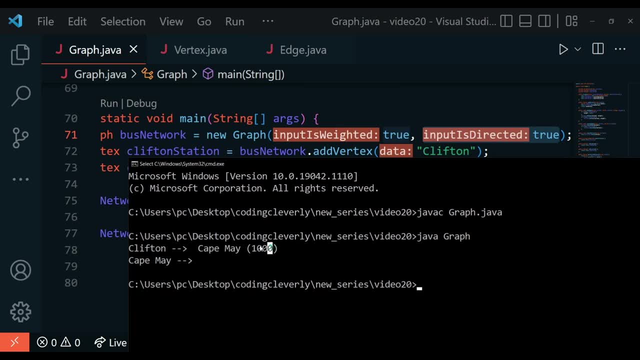 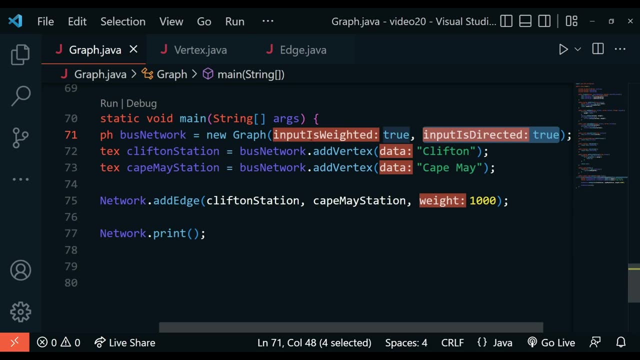 you can see that there's just one way, from Clifton to Cape May to 1000.. And I can't go from Cape May back to Clifton. And if I want to do that, I could easily do that. I could just modify this. So input is weighted. that's set to true If I just leave this as nothing. 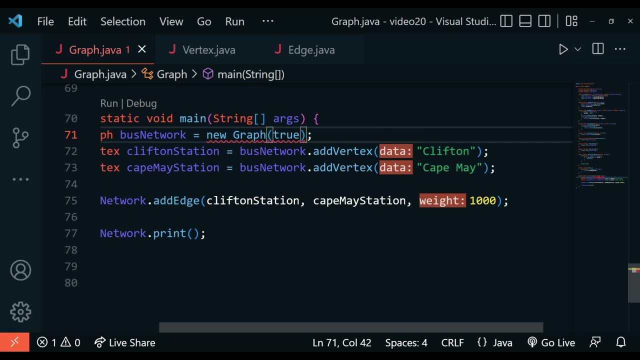 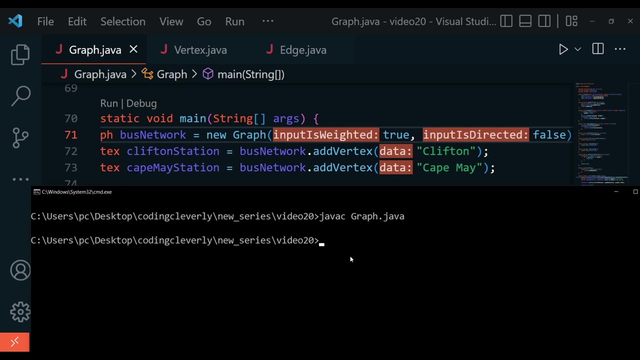 So by default it will consider that as false. So alright, so I'm just gonna have to if I add in false here, and that's just going to make it undirected. So it's going to go both ways around. And if I do this now it's going to go bidirectionally. So I'll say this: 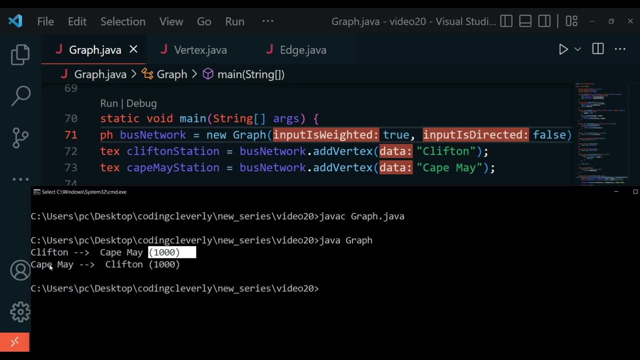 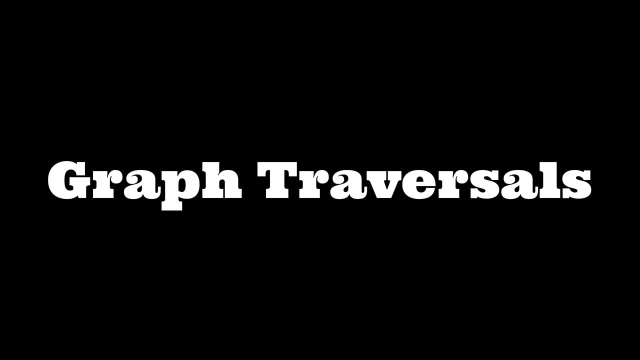 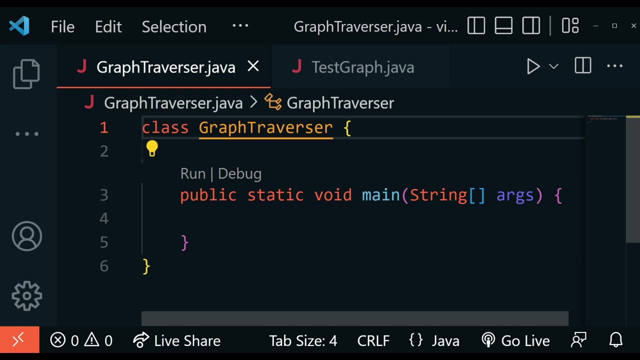 and then after that. so over here we have Clifton to Cape May 1000 and Cape May back to Clifton 1000. using graphs to model complex networks is great, But graph search algorithms are another way graphs can be useful. A graph search algorithm can be used to traverse the entire graph data. 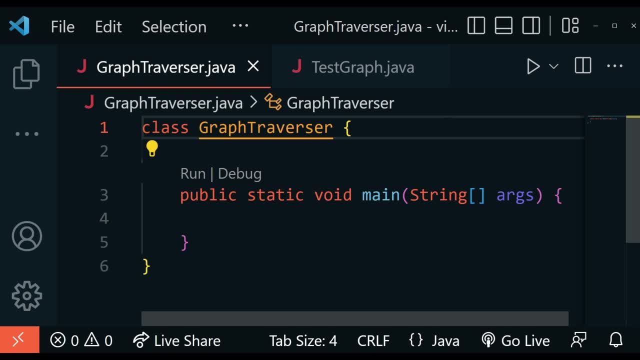 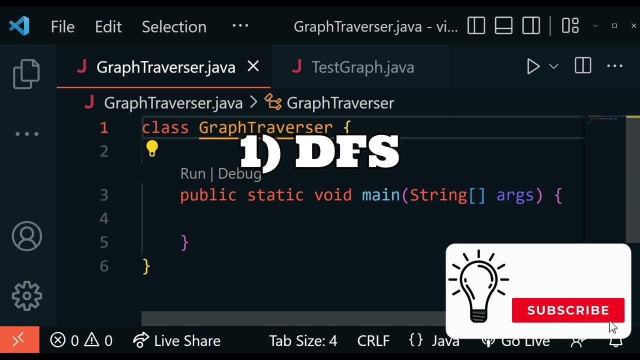 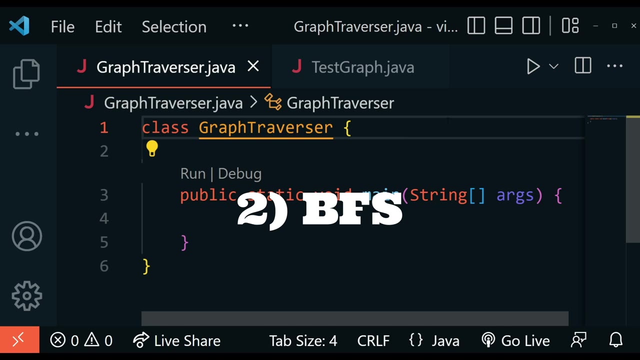 structure in search of a specific vertex value. There are two approaches to using a graph search to navigate a graph: DFS and BFS. DFS, or depth first search, follows every possible path to its conclusion. BFS, on the other hand, or breadth first search, expands the 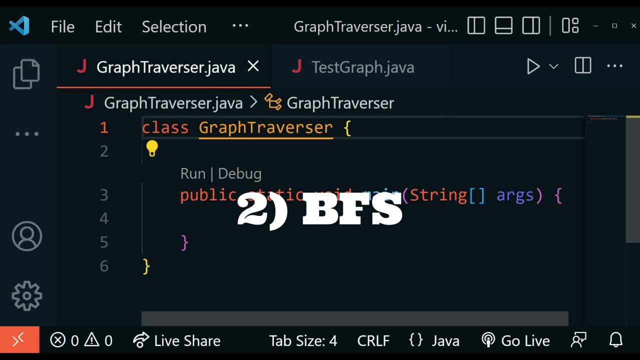 search from the point of view of the graph to the point of view of the graph, So we can search from the point of origin to an ever expanding circle of neighboring vertices. to track down what we visited, we add a list. this list will be very crucial because it 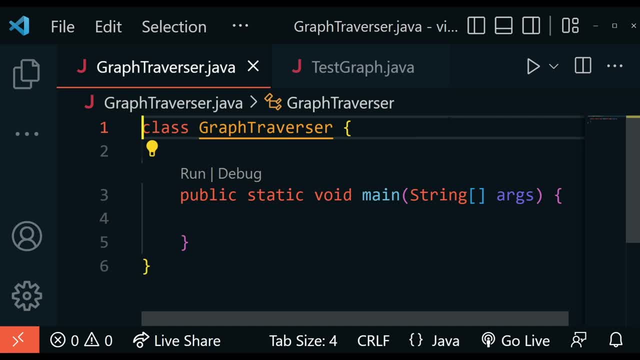 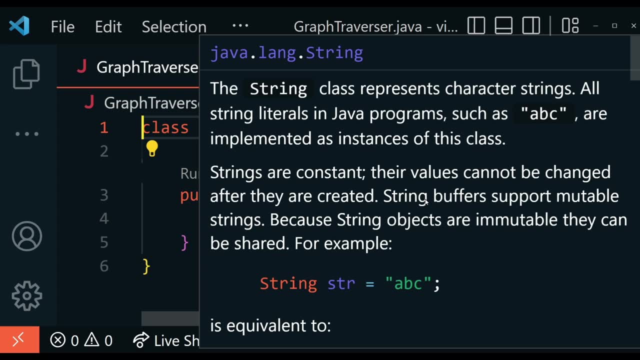 prevents the search from returning to the same vertex multiple times. This is especially important for cyclical graphs, where you could otherwise end up in an infinite loop, And we've seen this in our previous videos. So you might be wondering: how does one compute? 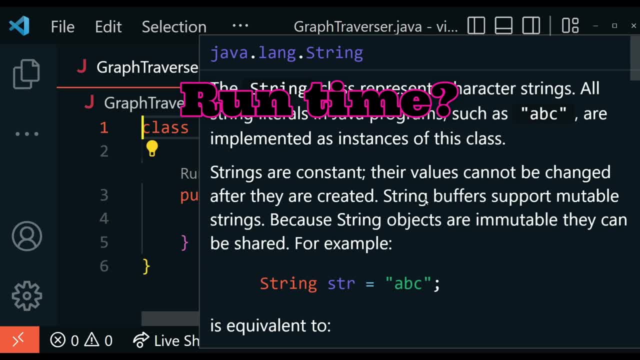 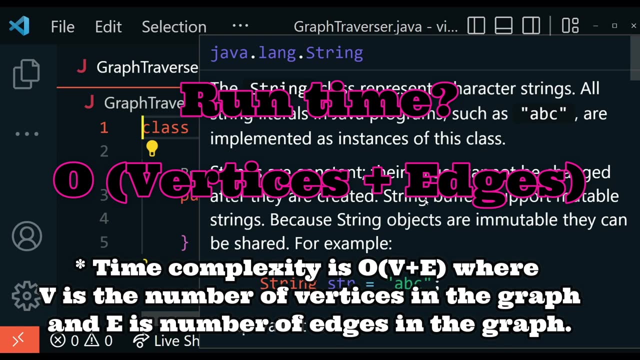 the runtime of graph search algorithms. in an upper bound scenario you would examine every vertex and edge. As a result, the big O runtime for depth first and breadth first search is O of vertices plus edges. So you have the O and you have bracket vertices plus edges. Now here's a question: what if you don't need to find a? 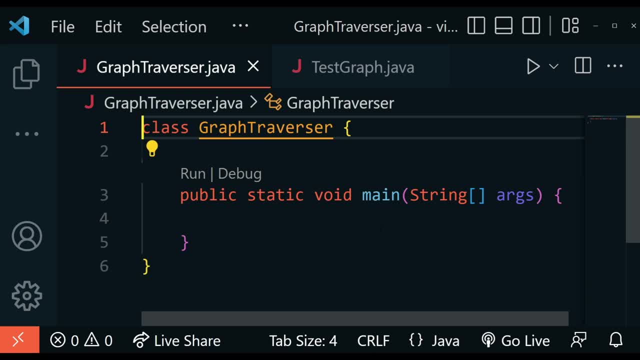 path, but you do need to find a list of all the values in a graph. What should be the solution there? Well, it turns out that, in addition to path finding, depth first search is pretty adept at organizing vertices Or vertex values with a clear order of visitation from beginning to end. So you could use depth. 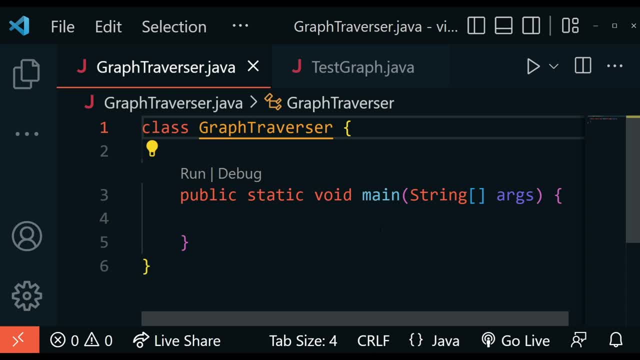 first search to find a path you know like, instead of pathfinding. but you could organize and show the layout of the complete graph structure using depth first search. there are three main traversal orders that you'll come across for graph traversal: pre order. 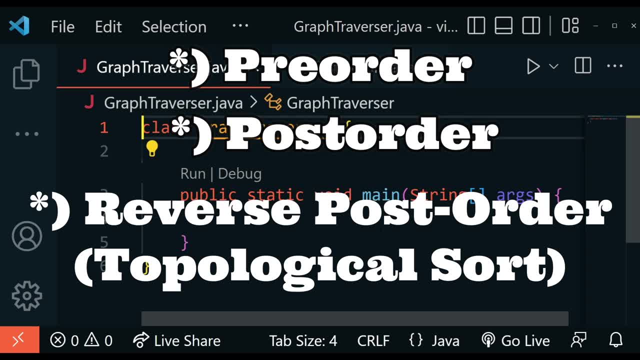 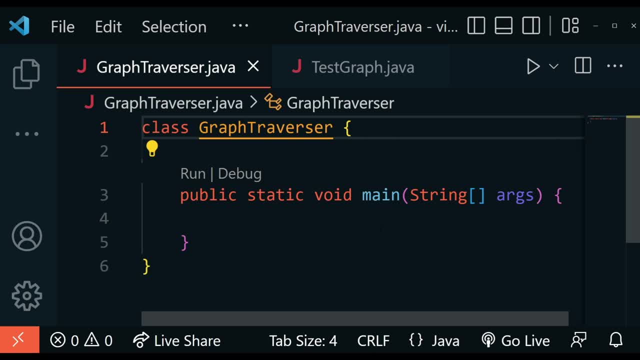 post order and reverse post order, also known as topological sort, pre order, in which each vertex is added To the visited list and added to the output list before getting added to the stack. So that's just one thing to remember here. in post order in which each vertex is added, 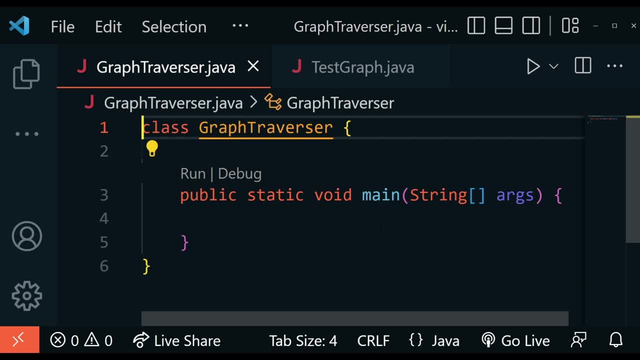 to the visited list and added to the output list after it is popped off of the stack, And then reverse post order, which is also known as topological sort, which returns an output list that is exactly the reverse of the post order list. So post order and. 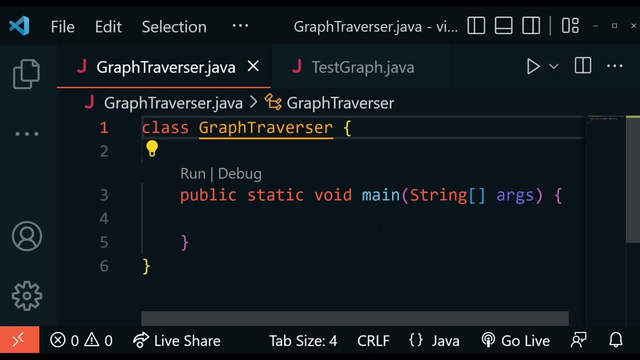 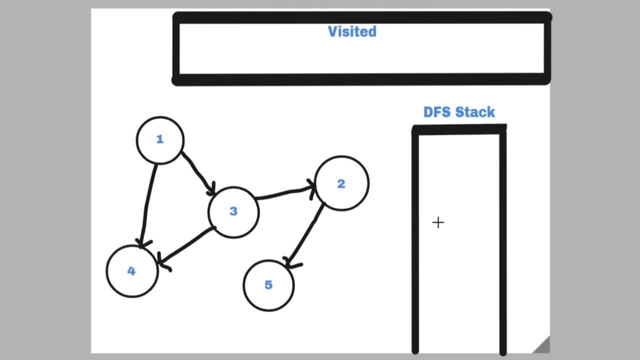 reverse post order are just like the opposites of each other. Here I have a cool graphical representation of a graph. take a look at this directed graph structure that I've depicted here. let's say that we want a list of all vertex values, starting with one in the order. 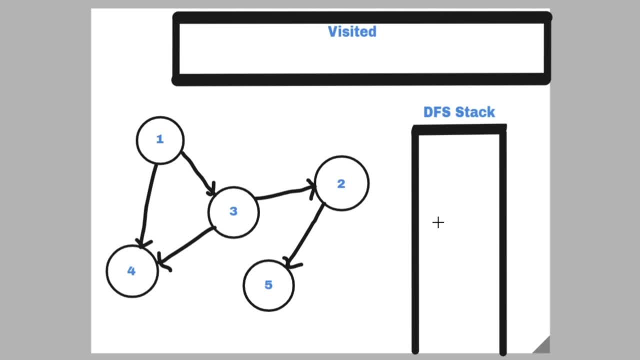 that they are added to the stack. Now a pre order DFS traversal would come in handy. Now, over here we would assume that the algorithm prefers visiting things in numerical order, if there is a choice. So our target value is one, And normally you would want to have a list of all vertex values. 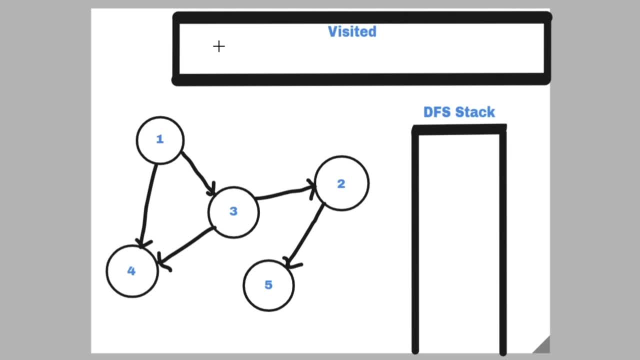 starting with one. So let's say that we want to have a list of all vertex values starting with one. So our target value is one and normally you would want to have a list of all vertices starting with one And normally you would get a target value from the program. So our 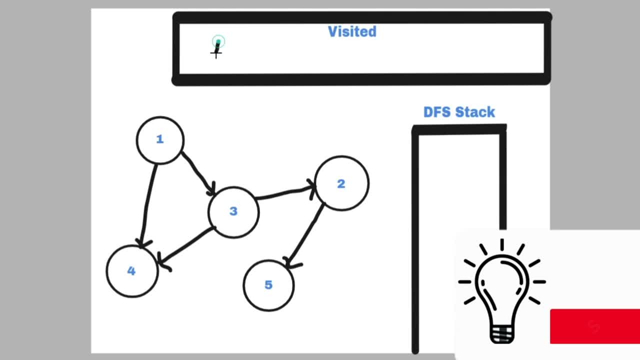 target value is one here, So we're starting with one, we'll go with one. So this is the first thing that's visited. this is also going to be on top of the stack. So over here, if we have a choice, we're going to prefer visiting the minimum number. So over here we have. 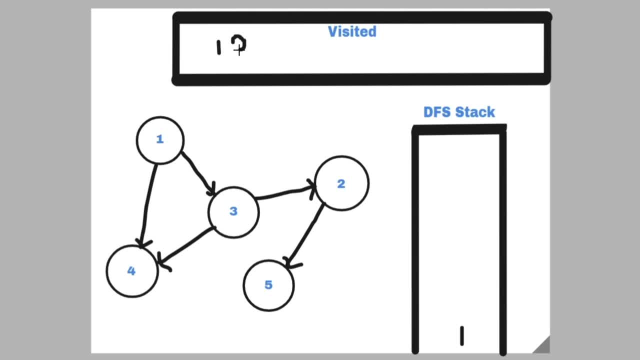 three and four. we're going to check three, So we're going to go and visit three And we're also going to put it on top of the stack over here. After that, we see that there's four and two, So we're going to look at the smaller number. 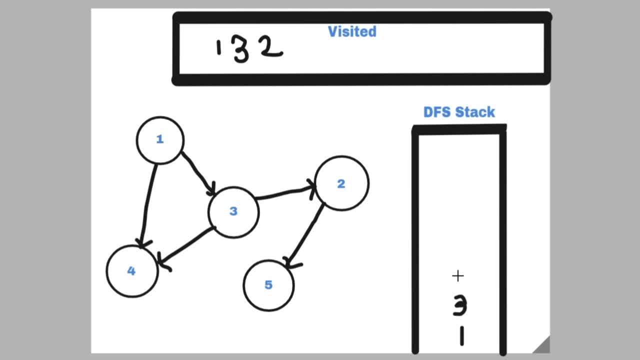 And we're going to, we're going to visit it. So two is going to be over here, Two is also going to be over here, And then we're also going to check for five. So, because it's five and there's no other option, so we're gonna have to check five, we'll put on the stack. 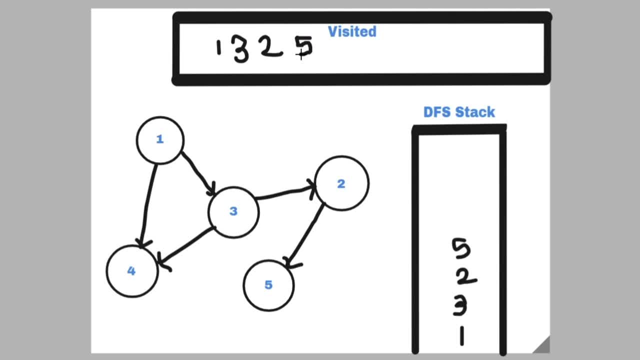 as five over here and the visited will go over here as well. Now the important part came, and you could see that there's nothing after this. So we'll have to pop this thing out of the stack. So we're going to have to just pop it out like this: And now we'll check. 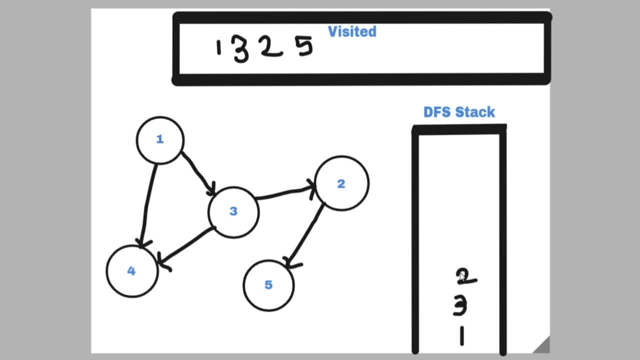 two, So two still has nothing. So we'll pop that out as well, And then we'll check three, So three has something. so it has thing that was not visited, and it was four and it's not in the visited set, So we're. 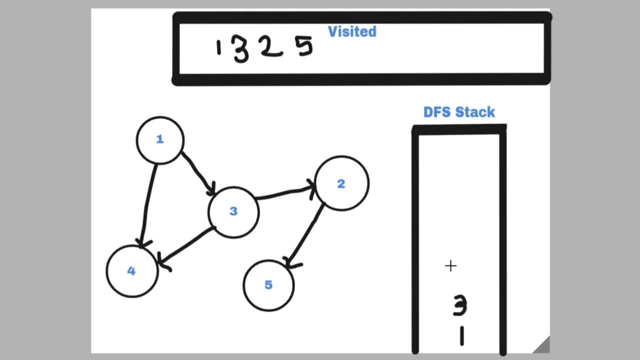 going to add that four over there. So just add four to the top of the stack here And we're going to add four here as well. Now we're going to check for the four And we're going to see: well, the four doesn't have anything, So we're going to pop that out of. 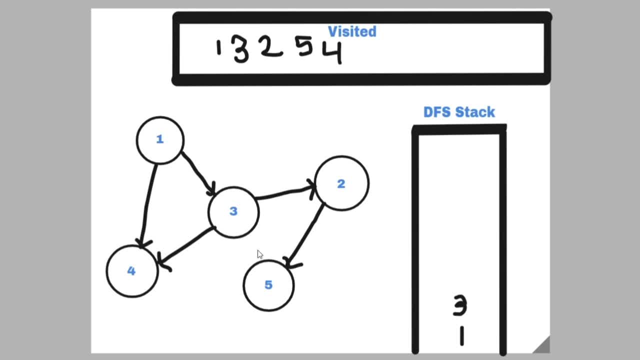 the stack as well, And then after that we have three. So we're looking at for three something, any number that is already, that is not visited. So everything is visited. four and two are visited, So we're going to remove three. we're going to look at one if there's. 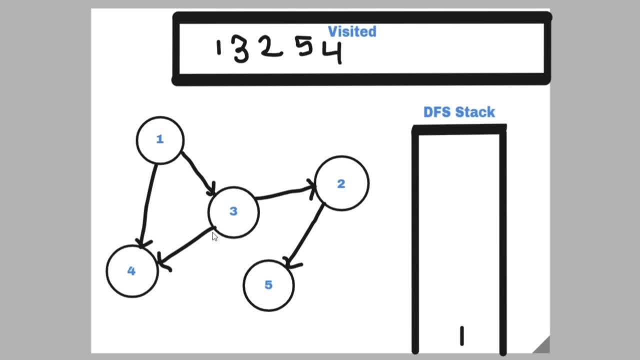 anything that is not visited, we'll have to check. But there's nothing, everything is visited. three and four are there, So we'll remove that. So this is how our list will appear: 13254.. So this is the pre order. DFS traversal- Alright, so, like I said, that pre order is: 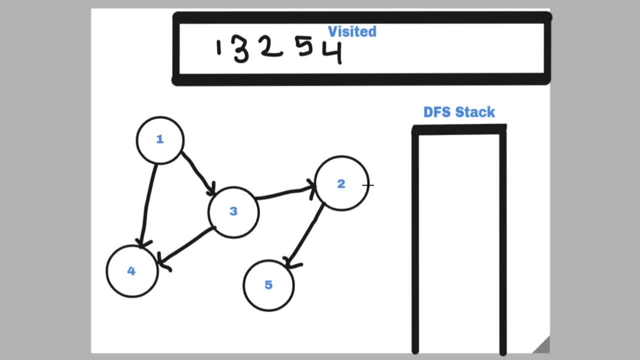 is that kind of order in which each vertex is added to the visited list and added to the output list before getting added to the stack. So this was our pre order traversal. Now we want to look at post order traversal in which each vertex is added to the visited. 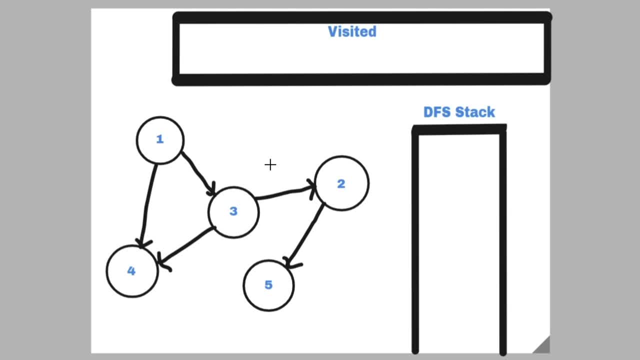 list and added to the output list after it is popped off of the stack. So if we look at- take a look at the post order traversal, we'll go like this. So for the first thing it's one. So we're just going to look at one. 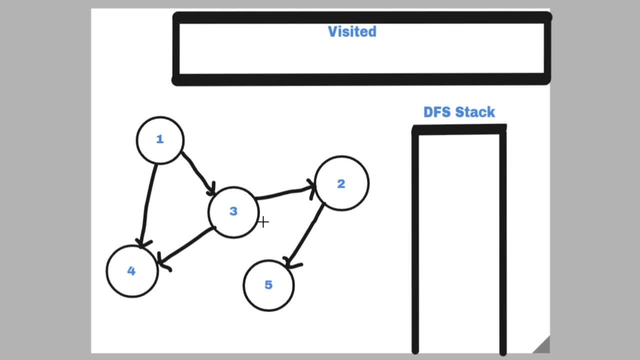 We're not going to add it to the list or anything yet. Then we're going to look at the smaller number, which is three. Then we're going to look at something even smaller than that, which is two, then we're going to look at something, and then we have five. So there, 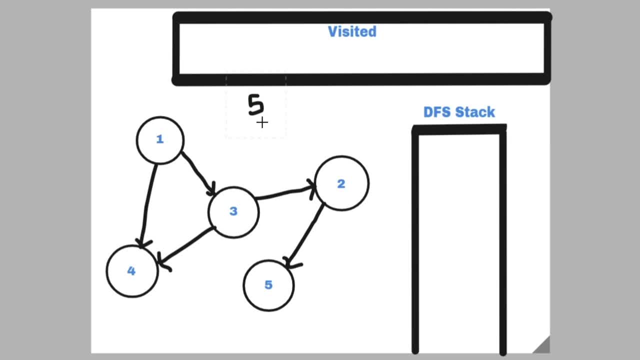 you go, the last number came, So it's going to go like this: five, And then after that it's going to go and see the two, because it's going to be popped off as well. So five, two, and then we're going to look at three. So three actually has something for this. So 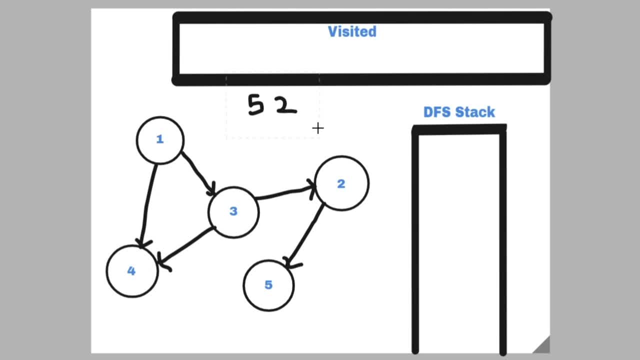 we're going to have to add four, And then we have nothing over here. So four And then we have back to three. So back to three, and then we have, we have the last one, which is one. So this is our post. 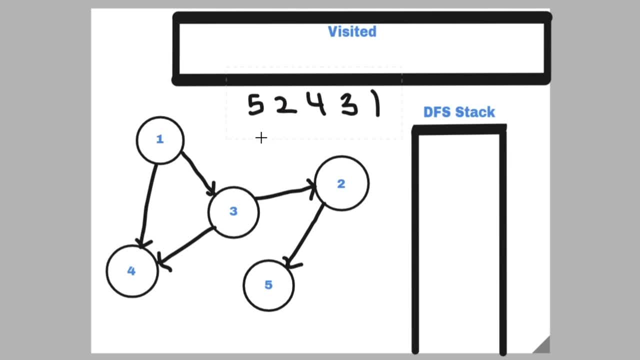 order traversal. This is how it's going to appear, And the reverse post order, which is also known as the topological sword, will return an output list that is exactly the reverse of the post order list. So this is the post order traversal, and the exact opposite. 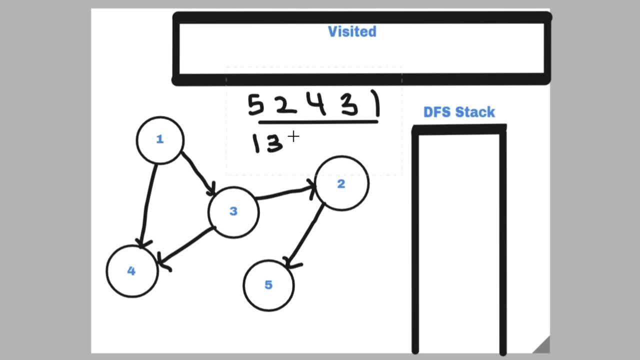 of this is 1342.. And then five. So this here is the reverse post order, also known as the topological sword, And these are just different ways to traverse the graph. The most common was the first one, which was pre order, And that's the default thing And it's easy for. 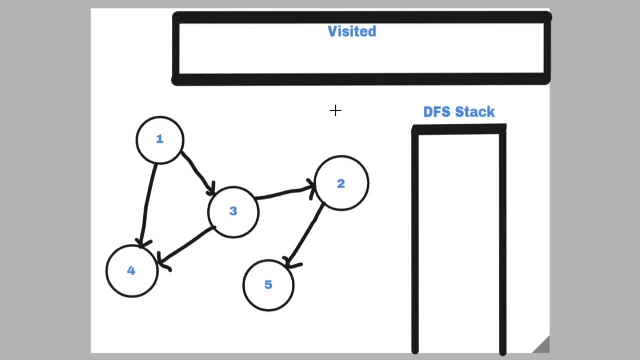 us to just get a full overview of the graph Like that. Alright, so let's have a conceptual overview of how the depth first search, DFS, is going to work. So let's suppose we have our target value as one, So we're going to. 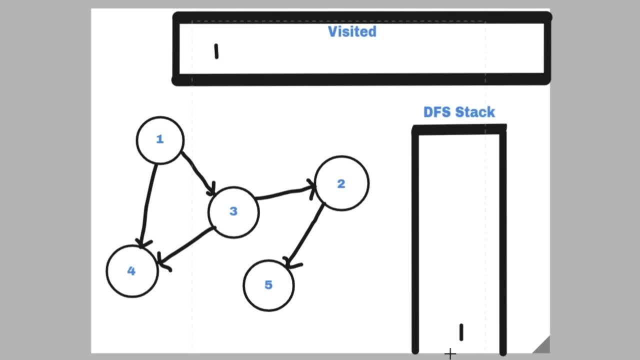 go and visit one here And we're also going to put it on the stack. So this is the top of the stack. then we'll have to look at the number that is smaller from the choice over here we got three and four. we're looking at a smaller number And we'll put three on. 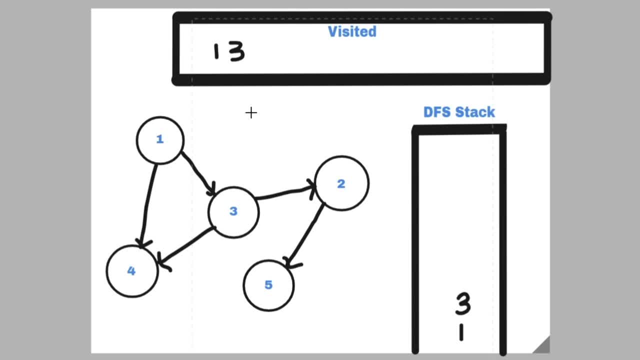 top of the stack here And we'll put it as our visited set as well. So we have three, And then after that we look at the smaller number from these two, And the two is the smaller number. So we'll put it in the visited set And we'll also put in the DFS stack. 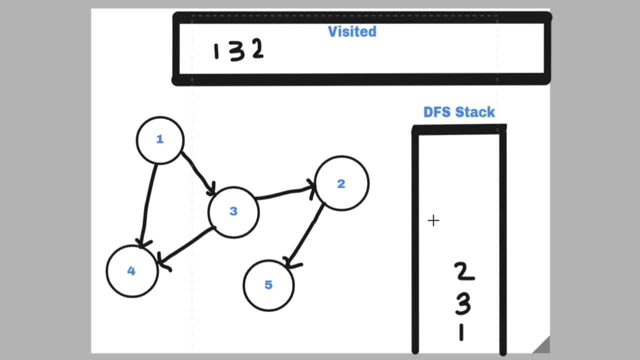 So we'll put it up on the top over here. And now we can see that five is the only option. So we'll have to use five here as the visited, And then we'll have to put five here on the top of the stack as well, Since there's nothing over here on the, there's nothing after the. 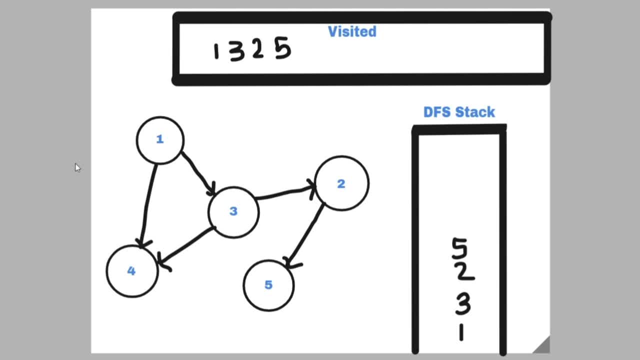 five. So we're gonna have to pop this out. So to do this, we're gonna have to just select this number and just pop it out. And now we're going to look at two. So there's nothing with two as well. 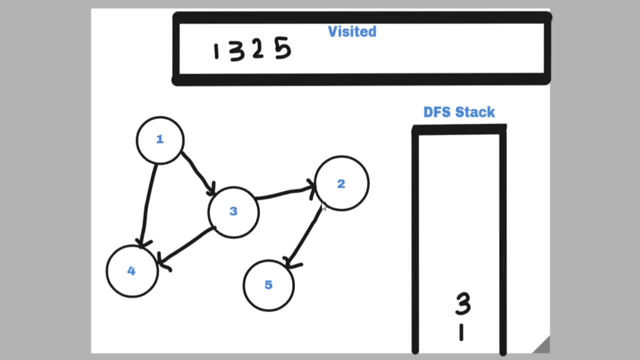 So we're gonna have to pop this out. Three has some unvisited vertex, which is this for one, because it's not in the set over there, So we're just gonna have to use this now. So we're gonna use four and we're gonna 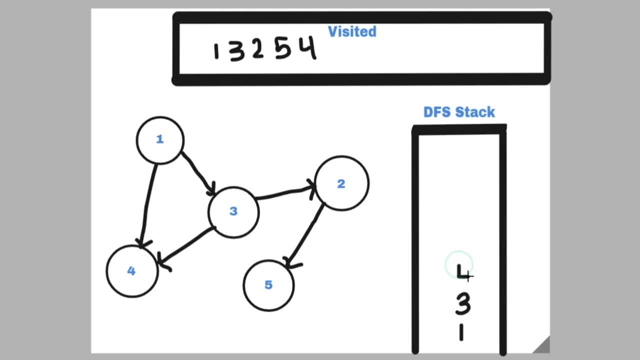 put it over here. So four is going to be over here and and four will be on top of the stack as well. Now we look at four, because this is our current, current vertex And there's nothing over here that's unvisited, So we're gonna have to pop this out again. So let's. 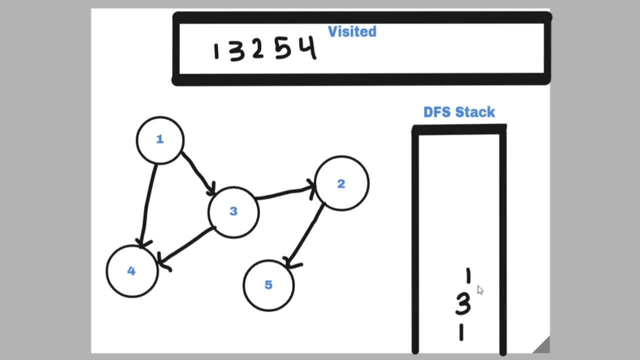 just pop it out. So there you go. So this is popped out. And now we look at three: there's nothing unvisited, So we'll just pop this out. look at one, and there's nothing unvisited, So we'll just pop that out Once the stack is. 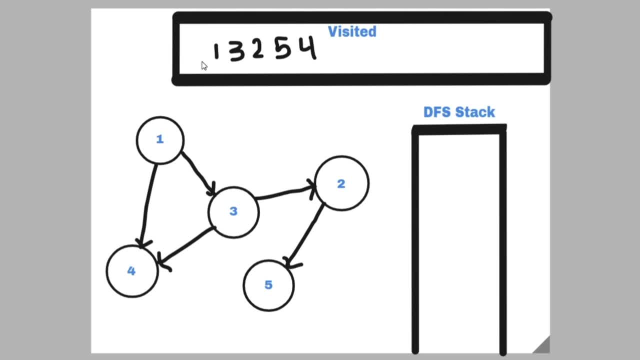 complete from here. so it's empty. we'll have a list over here: 13254.. And this is a list of all of the vertices inside of this entire graph. So we have 1325 and four. this was our DFS depth first search. Now let's write the code for this. So here I have a class. 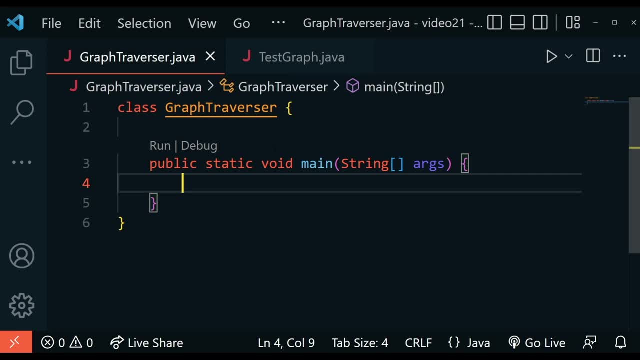 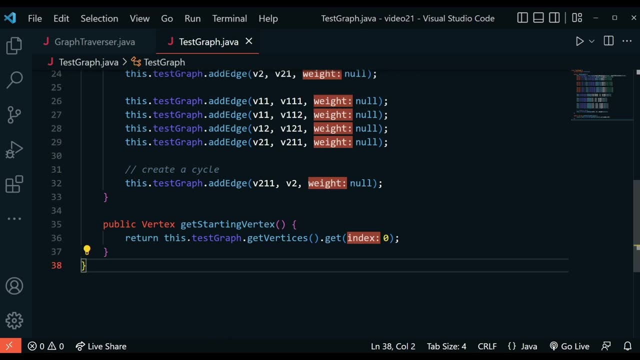 graph traverser And it has a main method And also I have a sample graph that I've created earlier And it just contains some vertices And yeah, it just has a method here that says get starting vertex And we'll get the first vertex here from the graph. Now our job here is to write. 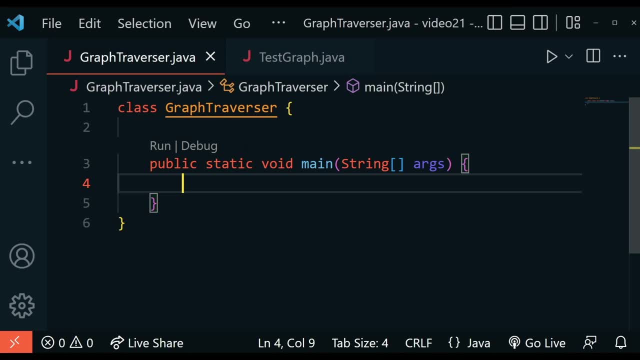 the code for depth first traversal. Versals are extremely useful when trying to find a specific value or path in a graph. We'll start with the depth first traversal method for recursively traversal, So we'll start by crossing a directed graph. To summarize: depth first reversals- iterate. 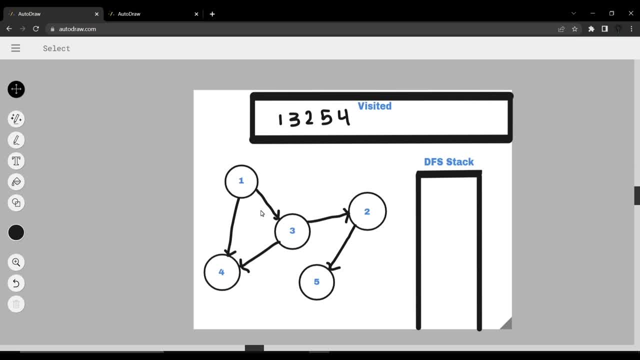 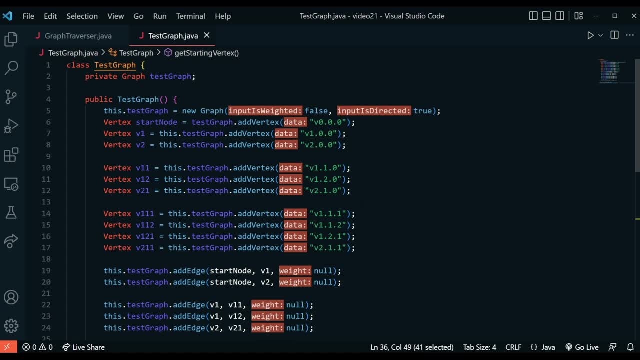 down each vertex, one neighbor at a time. In this video, I'll focus on traversing the entire length of a single path and printing the data value of each vertex. Now, in test graph dot Java, I've created a sample graph for us to test the traversals against. this is all linked. 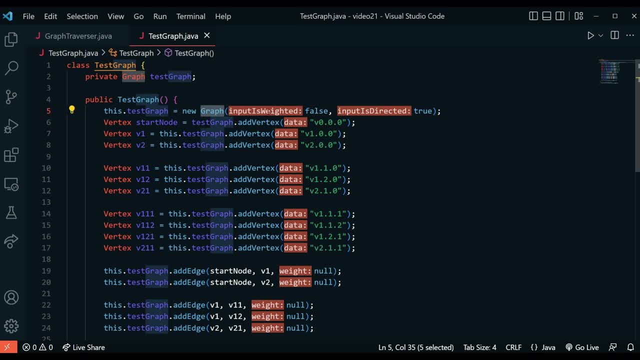 to my last video about graphs. So we created a graph here and we have this: input is weighted as false and is directed as true. So there's no weight, but it's directed, meaning it's it's, it has directions right And we have a vertex start node and we have test graphed out. 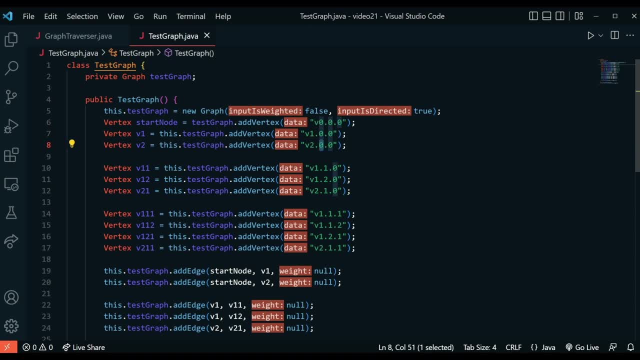 add vertex and we have the name. So these are the names of our vertices And yeah, so they're all these vertices here. Now I have all of these vertices that I added and then I created these variables to associate to them, And then after that, what we did is add edges, So connections. 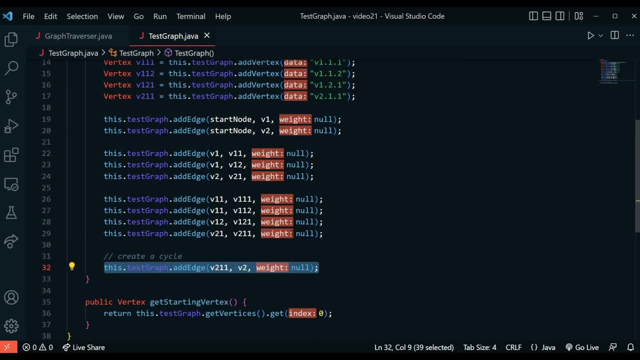 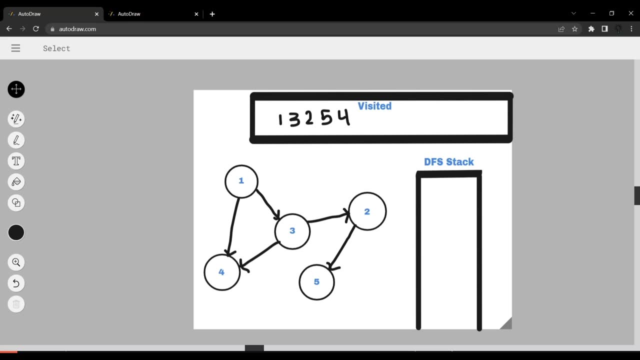 were done. After that, we created a cycle here as well, And this is not exactly the same graph that I've made on in the diagram, So which I have. what I have here in the diagram was just simple so that you could easily understand how DFS works, But here I just created a complex one. 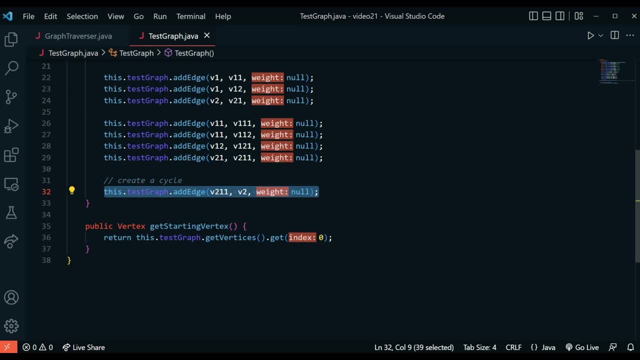 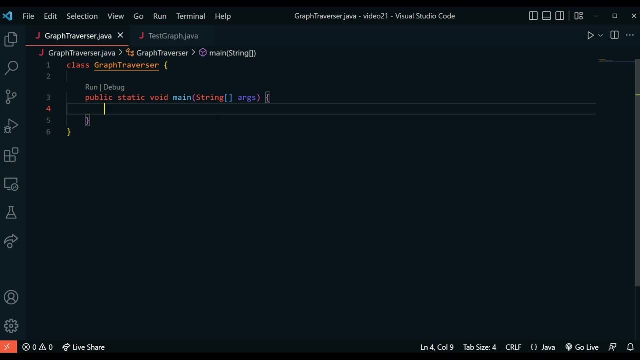 so that we could test out cycles as well And other things. After that, we have this graph traverserjava. To keep things simple, I created a separate graph traverser utility class in graph traverserjava And I'll implement the traversal iterator as a static method here. 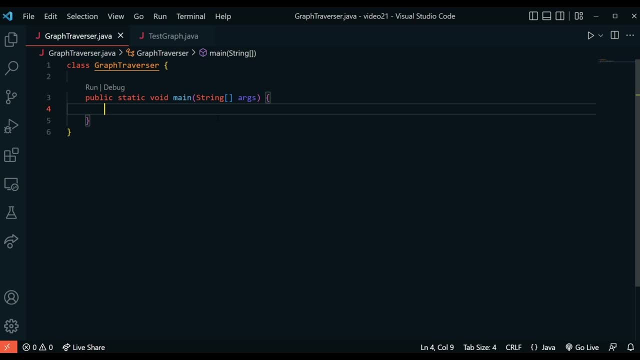 Now I've seen implementations in which they created the iterator interchangeably, And I've also created a static method here. Now I've seen implementations in inside of the graph class, So now let's start writing the code here in the graph traverserjava. 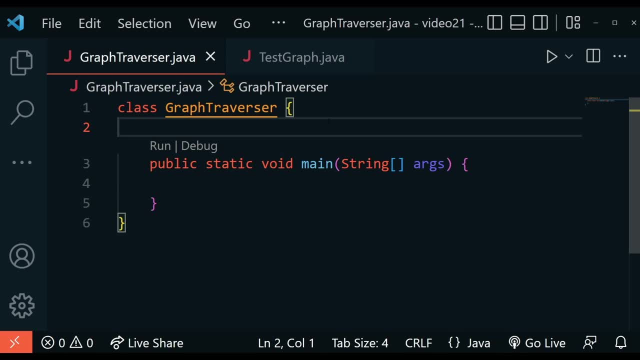 utility class. We're gonna first of all, let's just add a method that is for the depth first traversal. So we say public and we say static because it's a static method, and void. And we're going to say depth first Because we're using a static method here, because this is a utility. 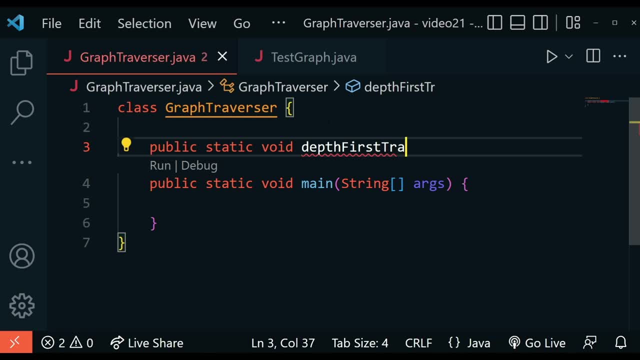 class. So depth, first traversal, And here I'm just going to pass in the vertex to start with. So when I need the start vertex and also I need a list of all the visited vertices for this, start one, So that will be called as an. 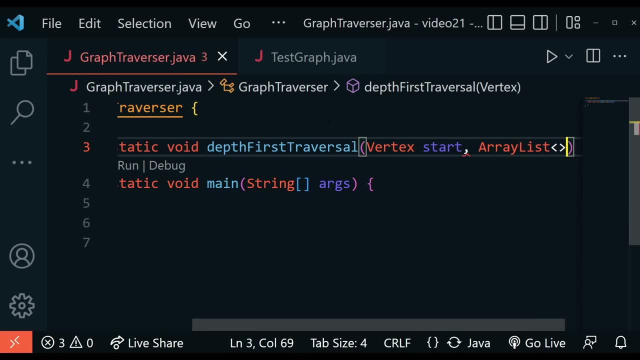 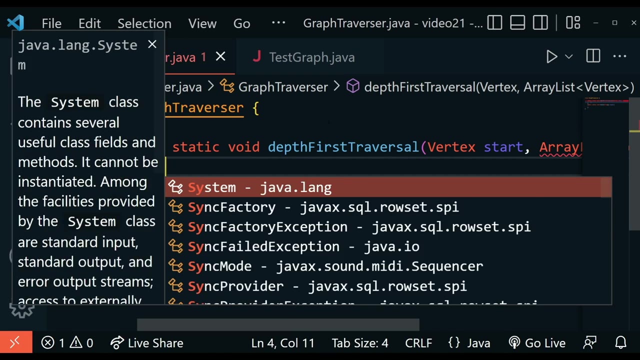 array list And I'm going to put in the vertex type here And we're also going to put in the name as visited, And then we have vertices- Cool, So now we're done with this. Let's add in the things here. First let's just print out the 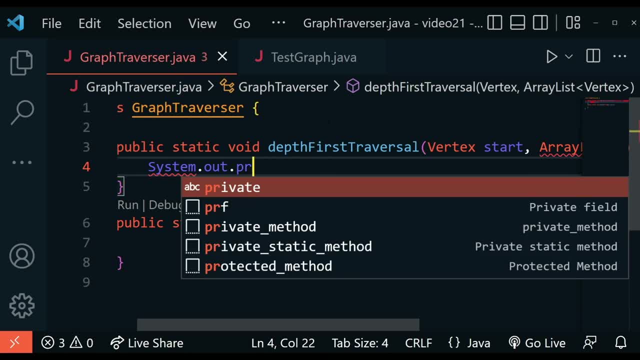 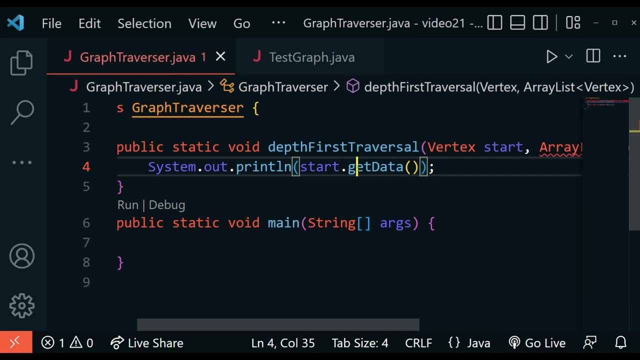 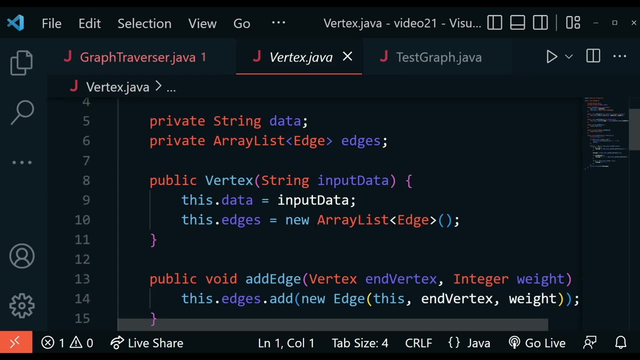 value of our start data. So we have a system dot out of println And we say start dot, get data. So you might be asking: where do I get this get data from? So I already have a vertex dot Java included here And I've created this in my previous video. So we have a get data method. 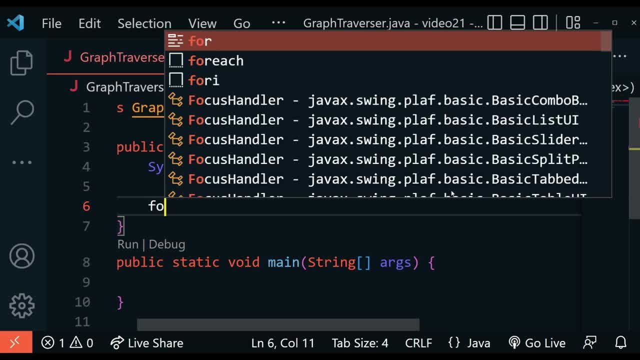 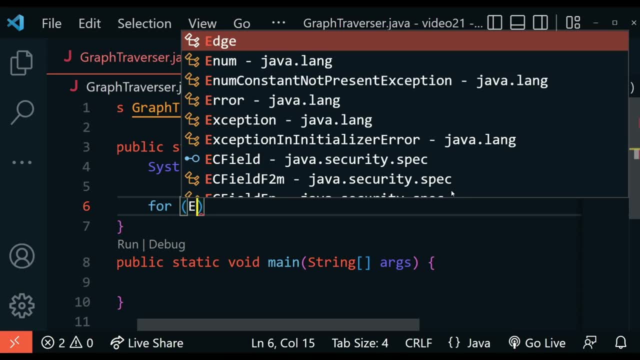 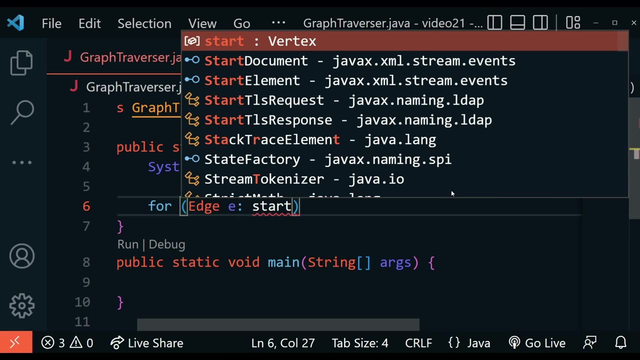 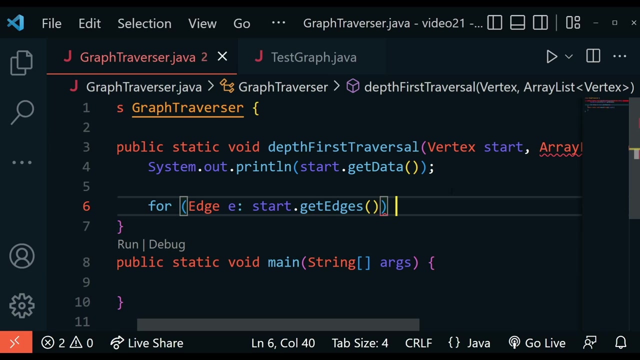 and it's just returns the string data. Now we're going to have to iterate through this vertex And we're going to check its edges. So all of the edges for the start vertex. So we could use an edge EDV of E. So for all the edges, E in the start dot get edges. So this is also a method inside of. 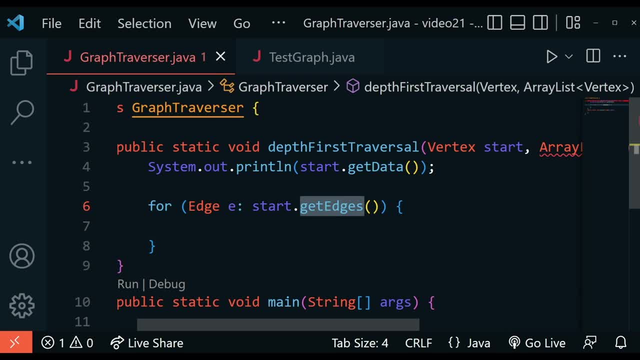 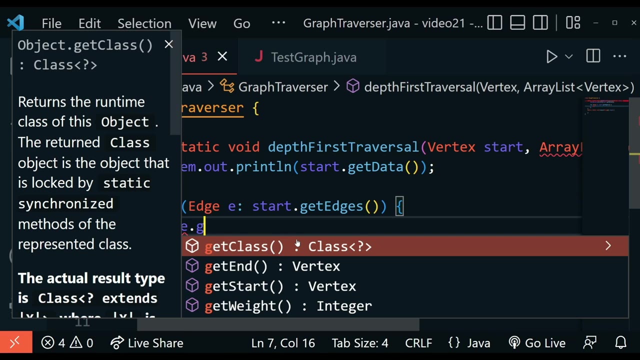 the vertex class. So over here I'm saying for every edge inside of the start edges. So this means all of those neighbors that are connected right, so we have to get the neighbor vertex. To get that we got to use E, dot, get And, and this will give us a vertex. you can see that return gave us a vertex. 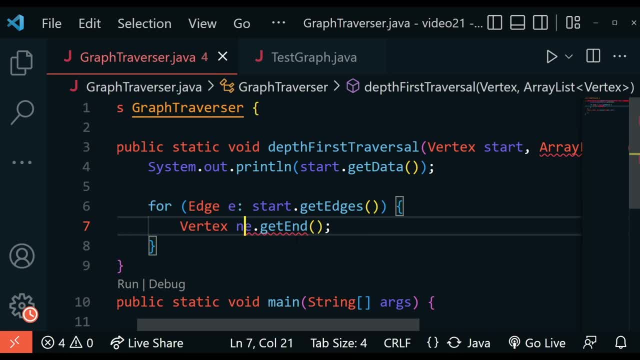 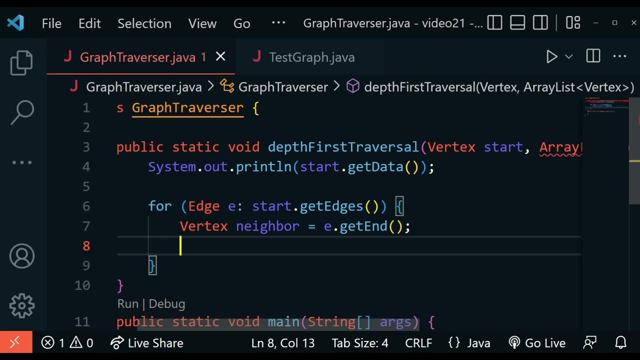 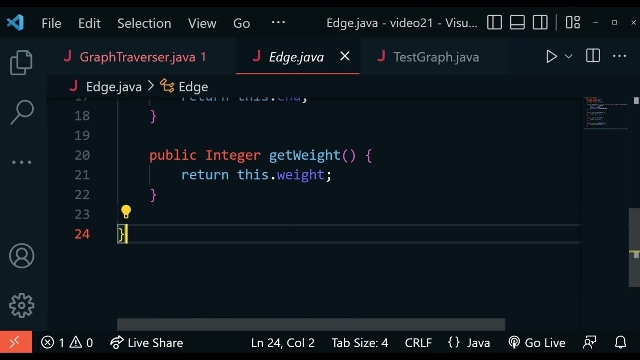 and we can save it as a vertex Neighbor any IDHB or Now. one thing to note here is that this E is an edge and the get end is from the edge class, So this is also here. So get end is going to be somewhere over here. there you go, And it returns the vertex end from there. So it's. 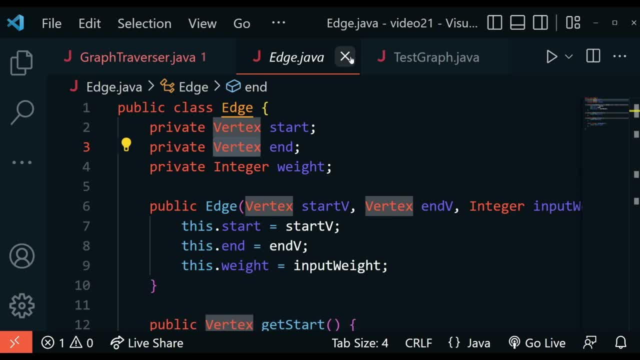 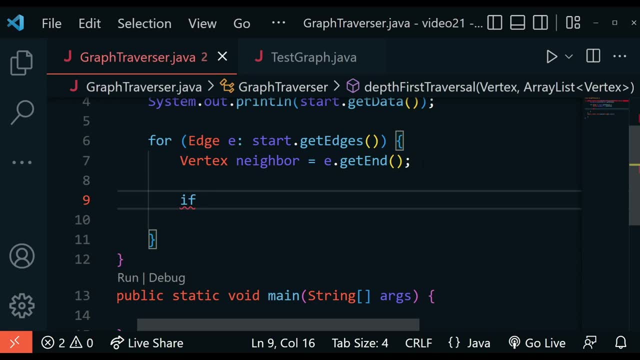 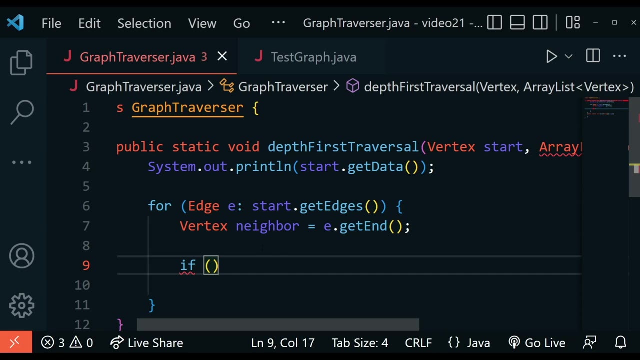 just pretty simple, this one, the end vertex. Now, right after this, I'm gonna have a conditional here And I'm going to check if, if my visited vertices does not contain this thing, so I'm going to add it inside. So now we can know- and we could, we can mark that- that we already visited. 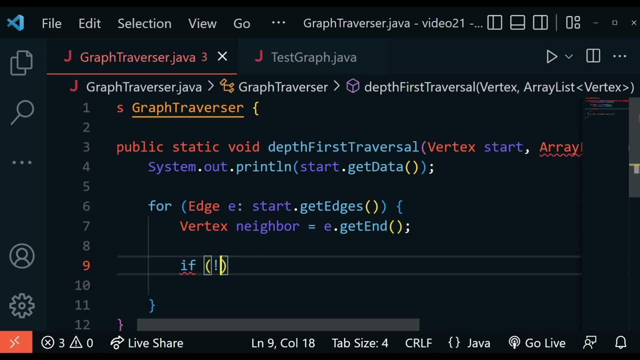 or not, to keep track if we visited vertices or not. we're going to add this conditional. So if we're going to use visited vertices And then we say dot contains, And then we have the, the neighbor, And I say: if that contains inside of the visitor vertices, because you know that. 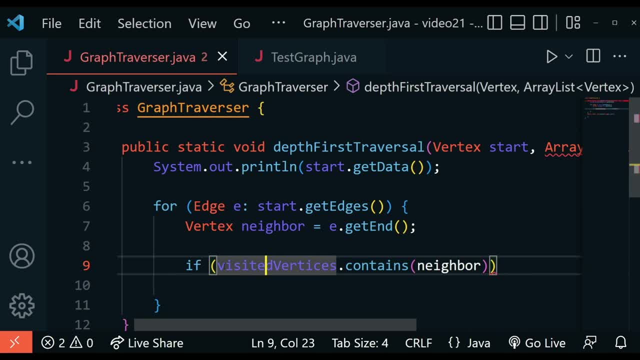 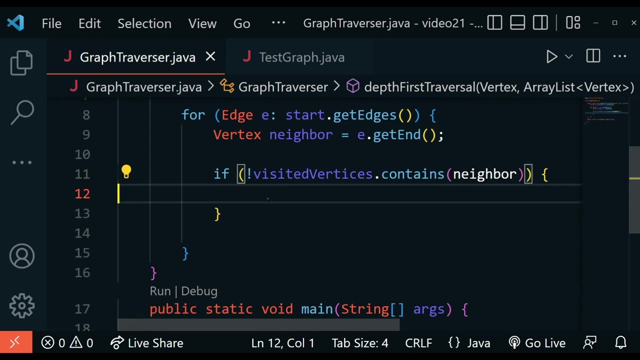 the visitor vertices was passed here And I'm saying if it's not inside of the visitor vertices then we want to add it. So we'll just put a negation here And let's also quickly add this import. So just over here and quick fix: import the array list as well on top. Okay, cool, Now over here. 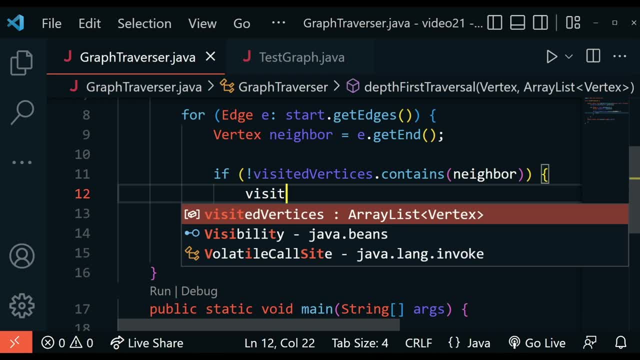 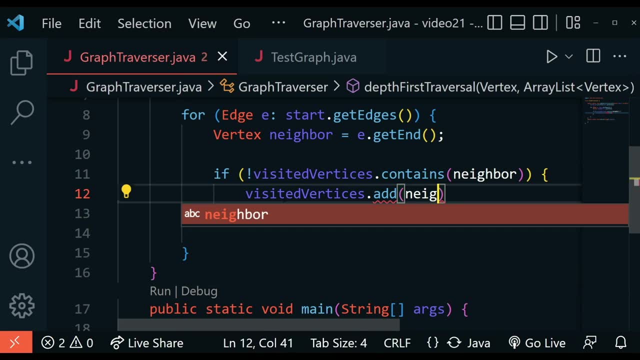 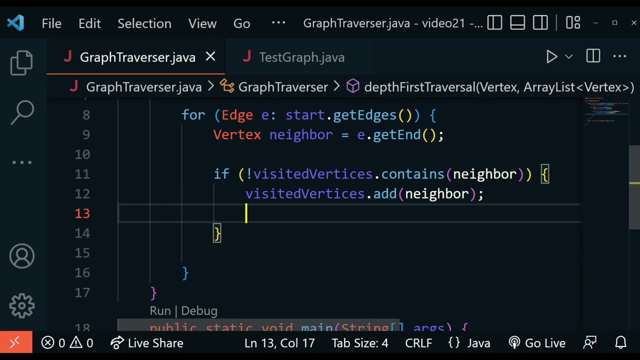 in this, inside the conditional, I'm going to add in the visited vertices and I'm going to say dot add And I'm going to add in the neighbor vertex here. So I'm going to say neighbor, since our visitor vertices holds a vertices vertices and we could easily add a vertex here. 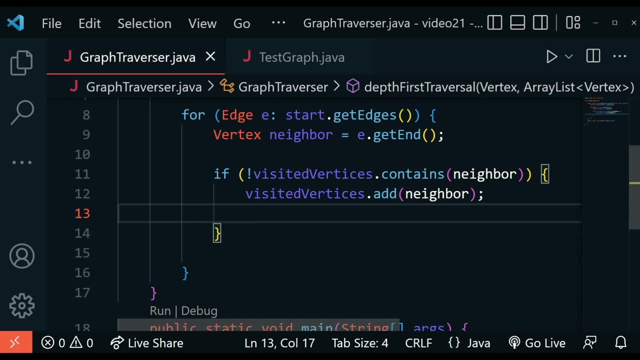 the really important recursive call here is that we're going to do a recursive call that will go to the graph towards her again. So we're going to call the graph traverser, which is this current class, And we're going to call the method, which is death, first reversal. 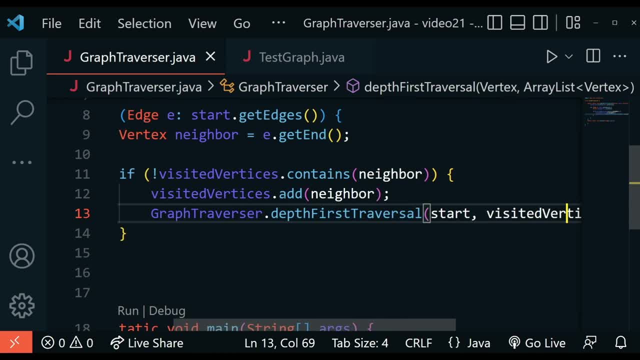 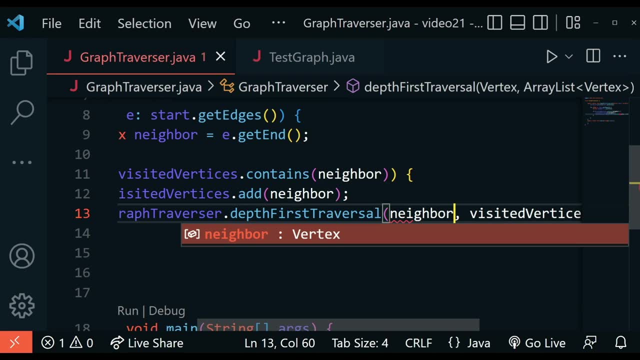 And now it's requiring us a start and visita. So the visitor vertices will be the same thing, But now we're going to go with the neighbor, so m e i d h b o r. Okay, so we're done with that, And 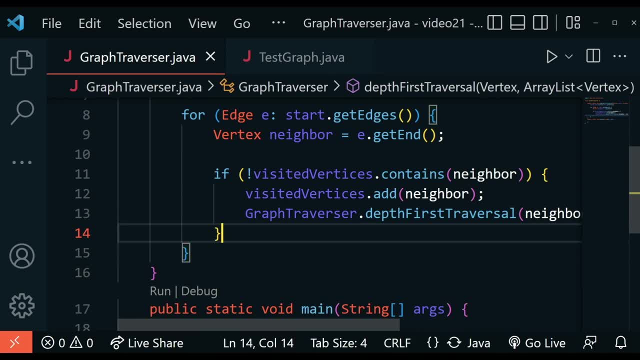 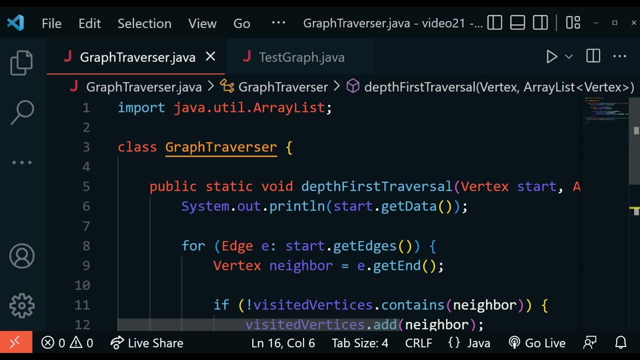 the conditional is done. And here is the for each loop it's going to iterate through all of the edges and it's going to go until it's done. So that's pretty much it with our depth first traversal. we could test it out in our main method. we're going to create a test graph. 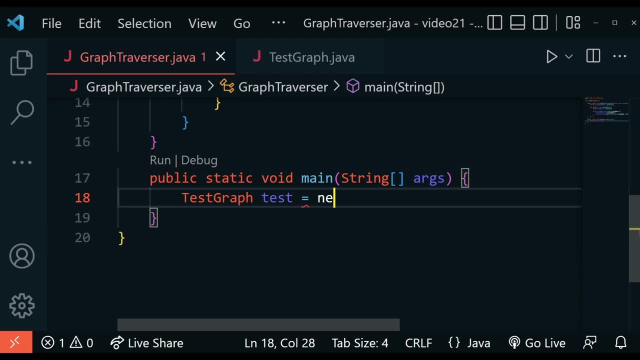 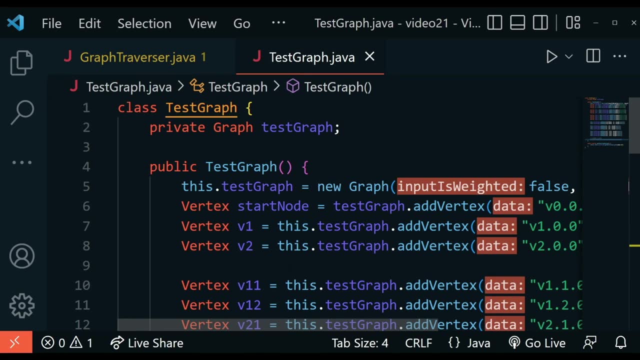 And we're going to say test And what we're going to say is new test graph. Okay, so where am I creating this from? This is actually from this place And this is just creating a test graph. Remember, like I said, it created this whenever this is a public test graph constructor And in 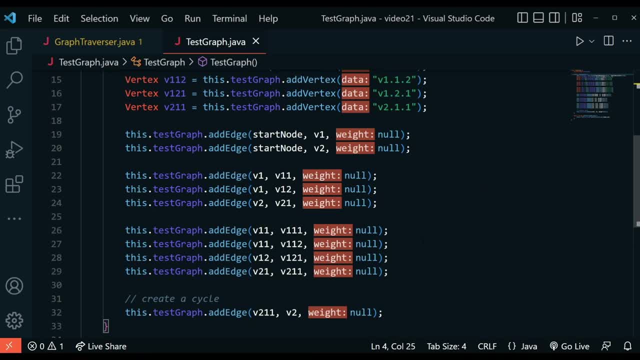 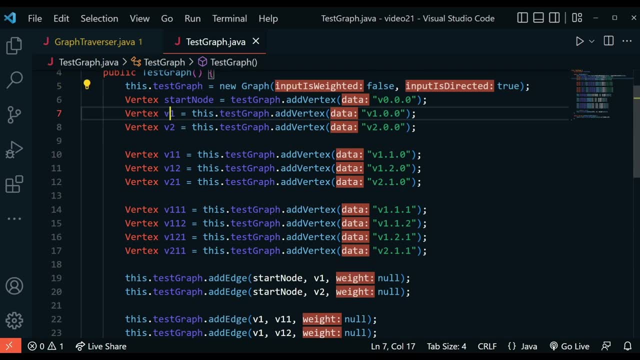 the constructor is just doing all of the work for us, So normally we would put this in a main method, But we're putting this in a constructor, So it's creating a gigantic, ginormous kind of graph with so many vertices, So v1, v2, v1, 1, v1, 2, all of these are 123456789, nine vertices. 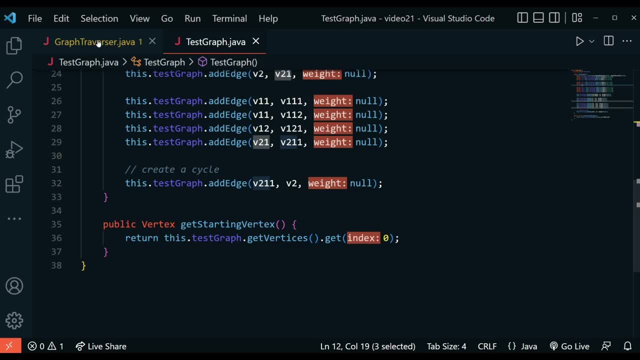 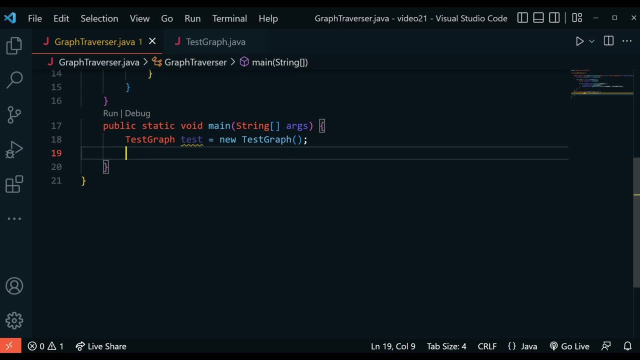 and they're connected edges. And what's it going to do is it's going to show us through this. So we're just going to create it here And we're going to pass it in. So, before that, we actually need the starting vertex of our 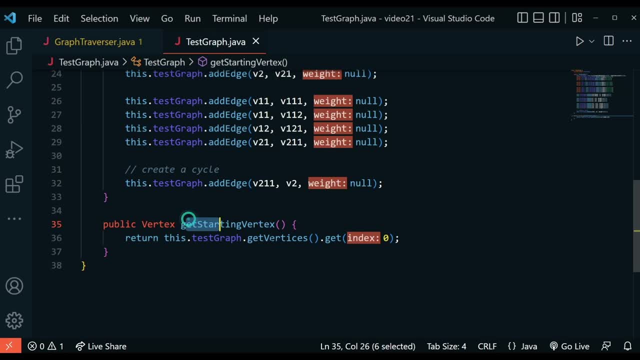 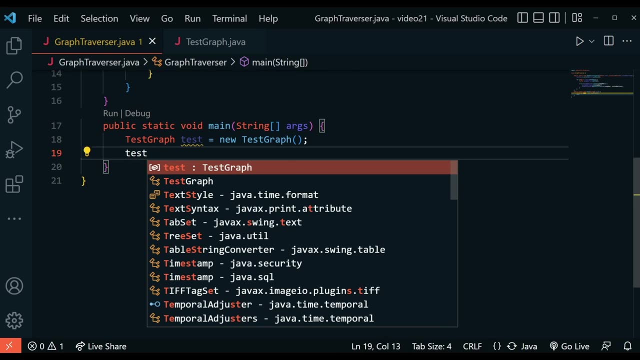 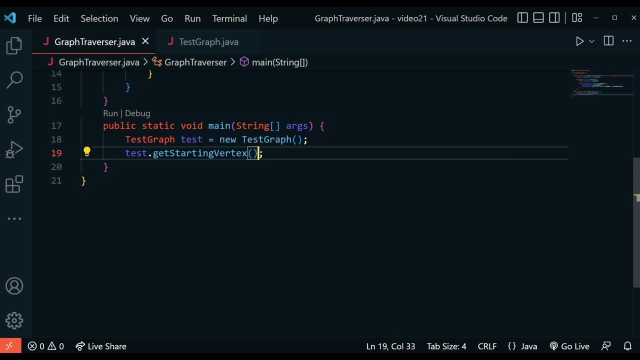 test graph as well, And we have created this handy method here which was get starting vertex, which returns us the first vertex in our graph. So we could use test And then we say get starting vertex, And this would just give us the starting vertex and we go save it somewhere. 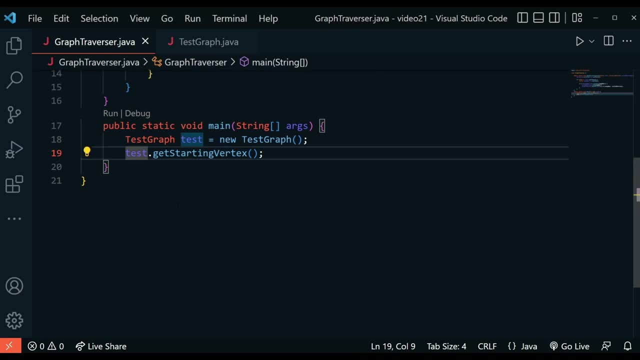 inside because of return. this actually returns a vertex type. So we could say vertex And we say starting vertex. So we'd say starting vertex And we'll just equal it. Okay, cool. So now that it's equal. now we could add in the visited: 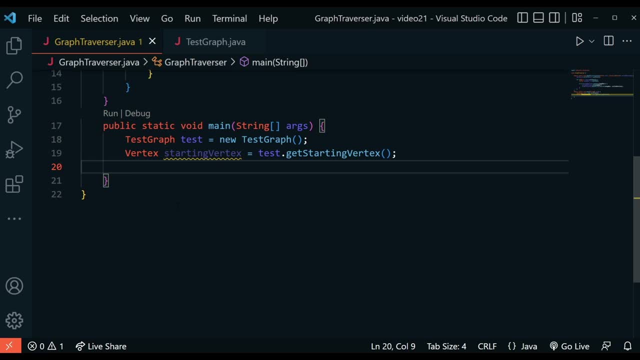 vertices. So now let's add the visited vertices list, So array list, And I'll put the type as a vertex And I'll call this as visited vertices. So visited vertices. And here we're gonna pass in a new array list. 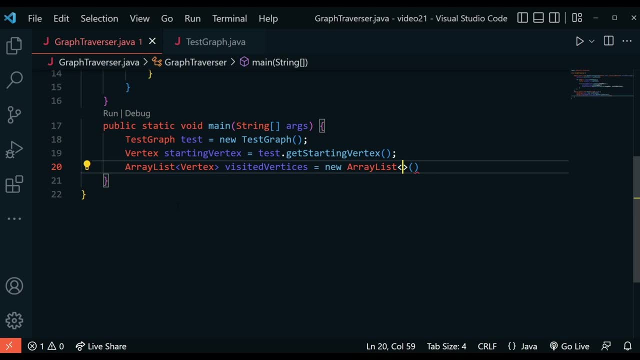 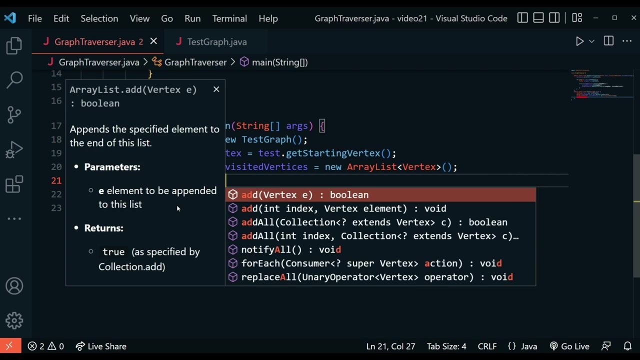 And here we're gonna to just instantiate it So like that I just semicolon at the end. So we created a visited vertices array list as well And we're going to add in the starting vertex because it's already visited. So we're just going to add it before all of the operations And we'll just add in. 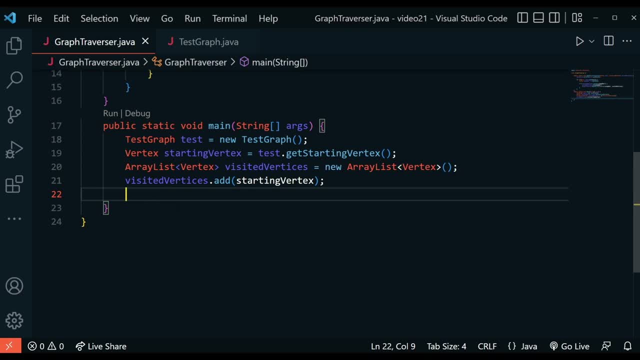 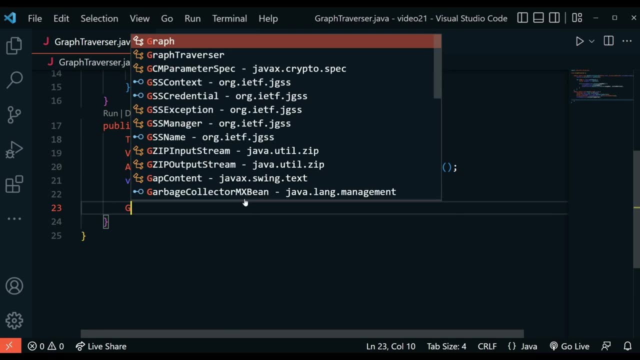 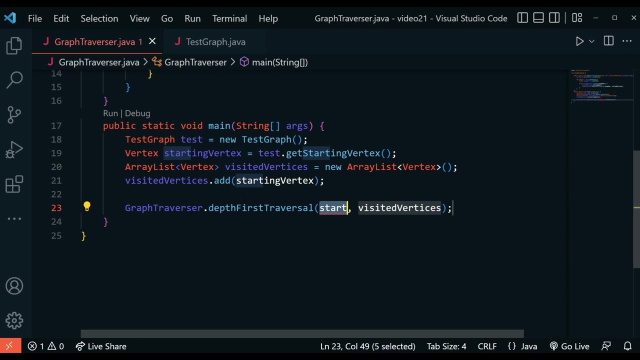 starting vertex here. Cool, Now, once done, we're done with this initial thing. Now we can finally call our depth first traversal. So this thing, and it's really easy, It's the name of the graph traverser, dot- depth first traversal- And it's asking us for the start vertex. So it's a starting. 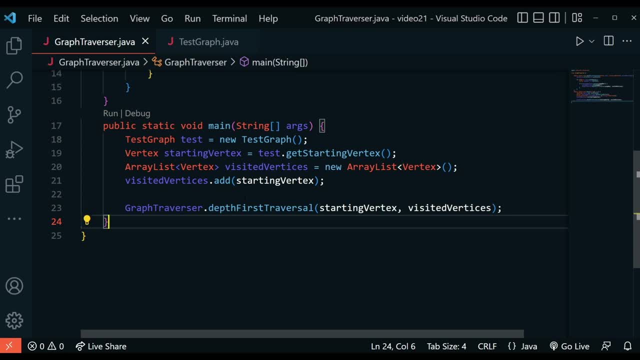 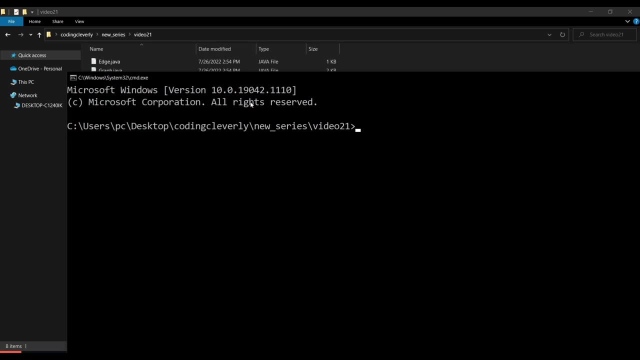 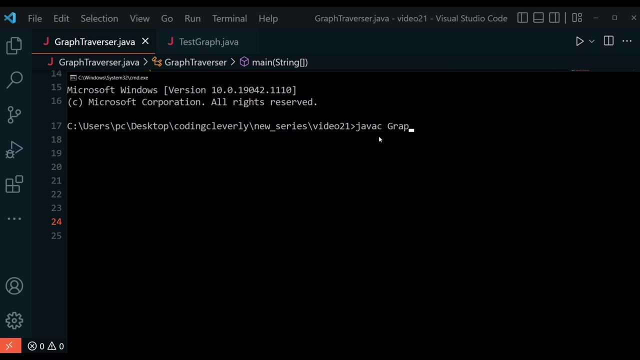 vertex and the visited vertices and this should print it out. So let's go into this place, which is right here, And command prompt it here, And let's go down and let's say Java C And we say graph traverser, dot, Java, And now let's just run it So Java graph. 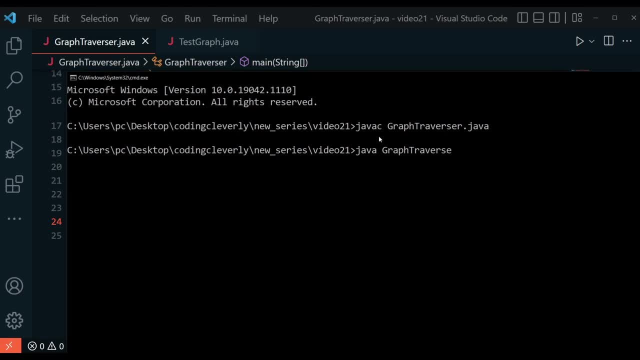 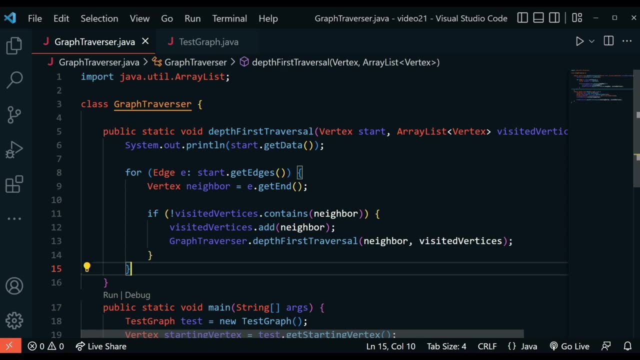 traverser. So here we have the the way how this will work. That's pretty, pretty dope. Now it's time to focus on breadth first traversal. As a reminder, the breadth first traversal iterates through the graph and layers. It goes down one layer which comprises the start vertexes, direct neighbors, then it proceeds. 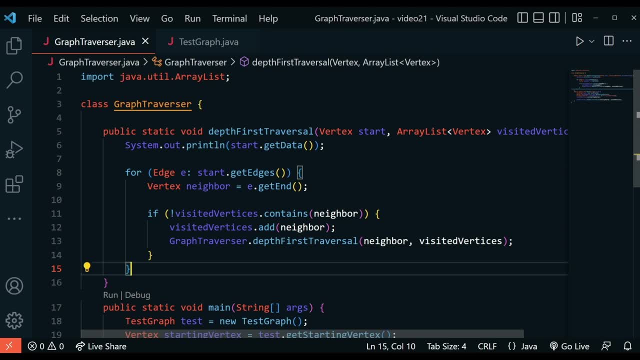 down to the next layer, which consists of all the vertices that are neighbors of the vertices in the previous layer, And for this example, I'll focus on traversing down one layer and then take a similar approach as we did with the depth first traversal, by keeping an array of visited vertices to prevent 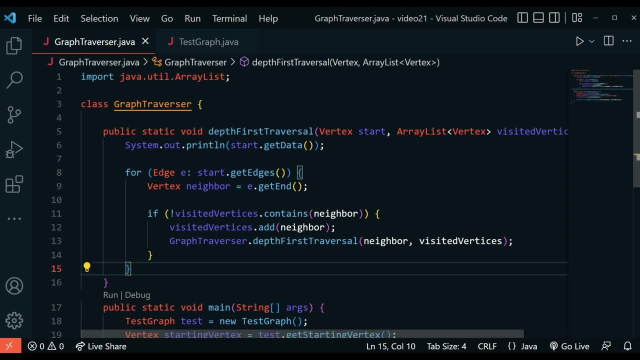 us from iterating through the same vertices over and over. However, we will iterate through all of the direct neighbor vertices instead of iterating down the neighbors first edge. that, like we did in depth, first traversal, we will also use a cue to traverse through the graph instead of recursion. 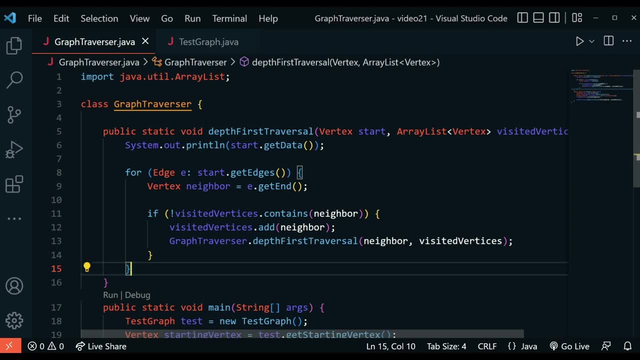 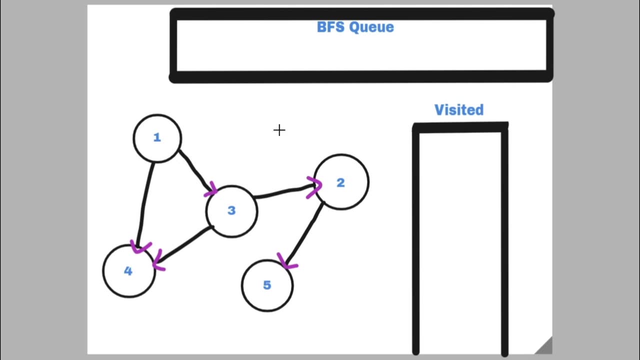 to explore the different ways we can implement the traverse, I'll reuse the same test graph that was used in the depth first traversal implementation. Alright, so what I have is a directed graph and I'm going to have to apply breadth first traversal. So what I'm going to do, 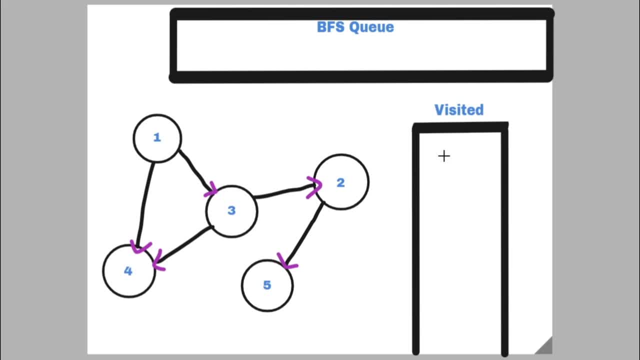 is. I'm going to get my target value- suppose we have it as one starting value- and I'm just going to put it in the visited and I'm also going to put it in our BFS cube. we're going to look at our 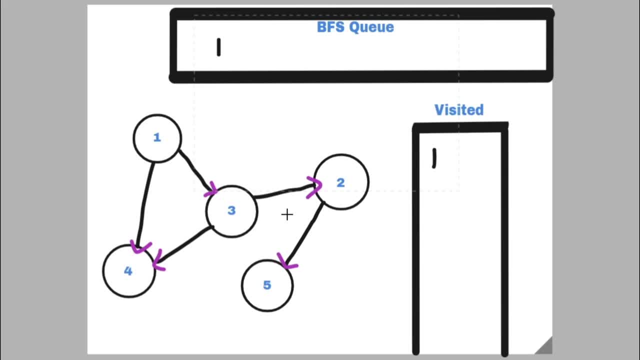 adjacent vertices and see the smaller number. So here we have three and we're going to choose that as the first one. So we're going to say three as our visited And we're also going to put three here as well. Now that we've done that, we look at the other adjacent one, which is four. 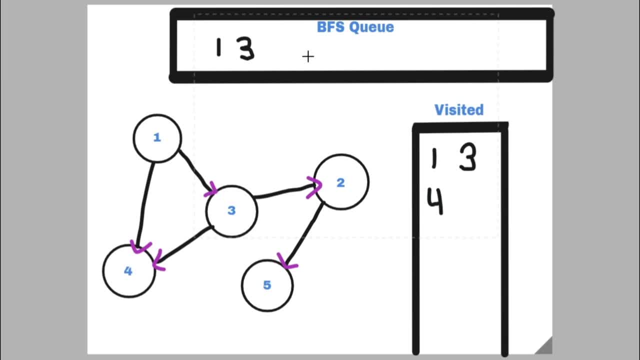 and we're going to add that in our visited set And we're also going to add it here in a queue, Now that we've exhausted our current vertex, since there are no more unvisited vertices, so we're going to have to remove this one from our queue. So we're going to remove this one, And now three will be our. 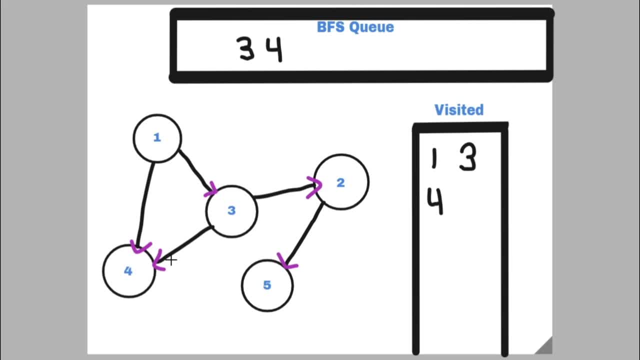 new current vertex. I will look at the adjacent ones here. So we have two and four, but two is smaller So we're going to use choose two first. And here we have two in the visited and two in the queue. Now we also have four, but four is already visited here, So we're not going to look. 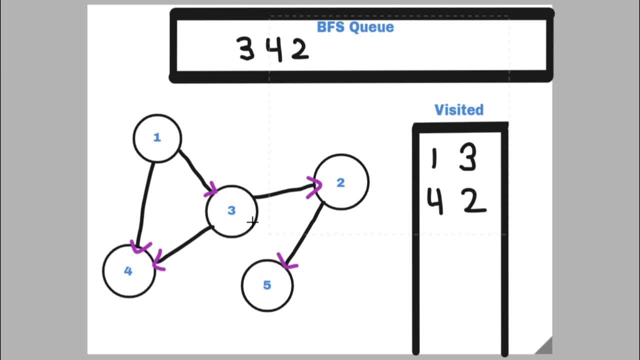 at that. Now that we've done this, we're gonna have to exhaust, since three is exhausted Now we're gonna have to remove that as well. So we're going to dequeue it And we're gonna now look at four. Now four is. 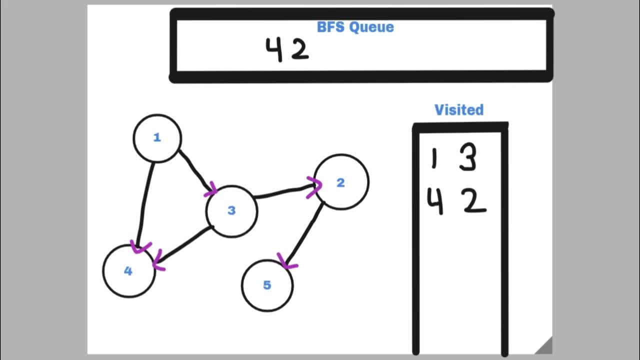 over here and there's nothing that we could visit, So we're gonna have to remove this as well. So we'll remove four, And after that we could see two is now our current vertex and two has a neighboring, a neighboring vertex, which is five. So we'll put five here. 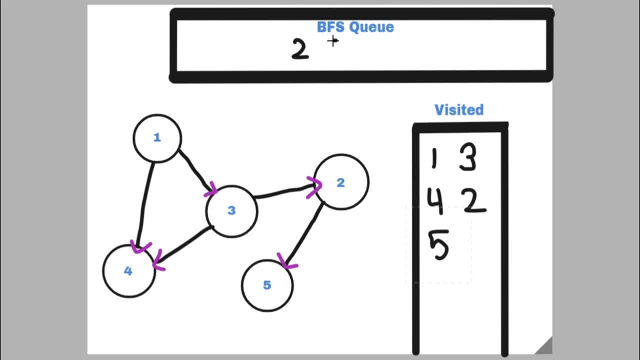 and it's the only neighboring vertex, So we'll just put the BFS queue over here. So now that we've exhausted two, we'll remove it from there as well. And five is also nothing, So there's nothing with five as well. So that's completely exhausted as well. So here we have. 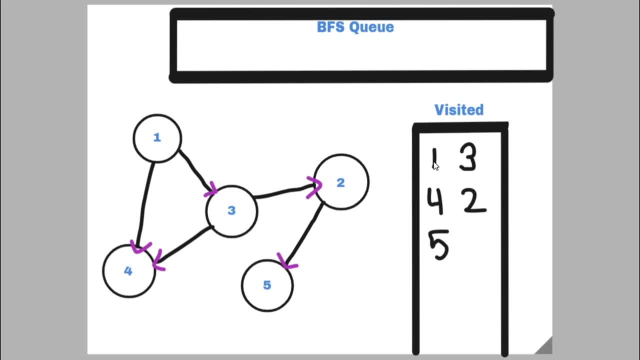 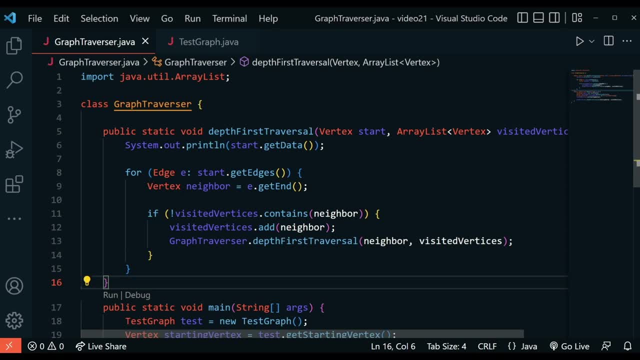 completely visited the entire graph using breadth first search, 1342 and five- Awesome. Now let's write the code for this. So I'm going to the same file where I created my depth first search And I'm going to add my breadth first search right after this. So this is my depth first search. 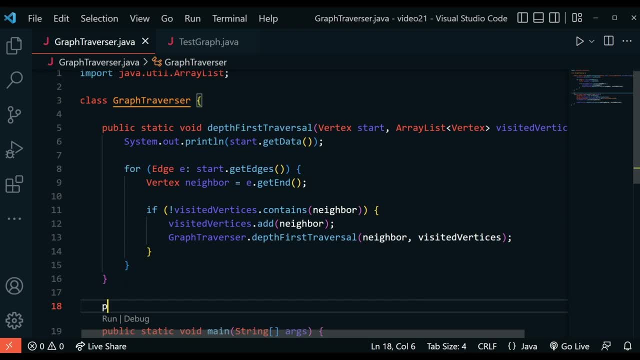 And right after this I'm going to create my breadth: first search. So I'm gonna say public, And we're also going to make this as a static Method, since this is a utility class: br, e, a, d, th, f, i, r, s, t, and then se search, So depth. 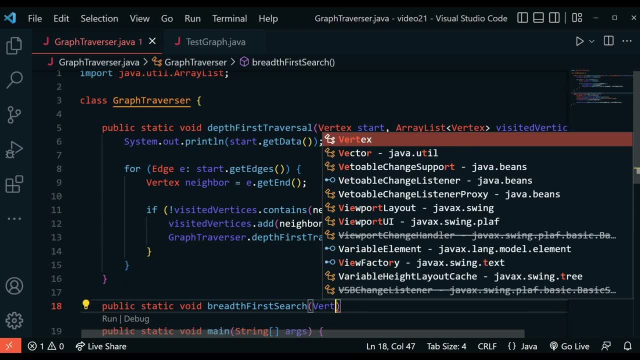 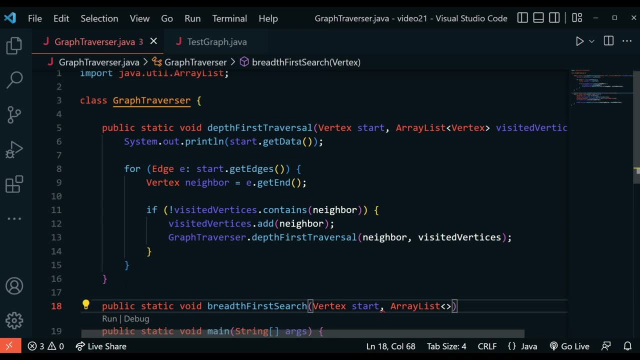 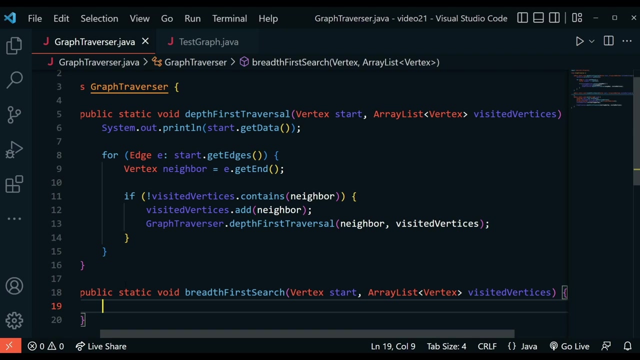 first search. that's for so breadth: first search. add in the vertex start, just like that, And also the array list, which is the vertex, And this is going to be called the visited vertices, just like what we did Up on the top for our depth. first traversal Now, since you saw the graphical implementation there, 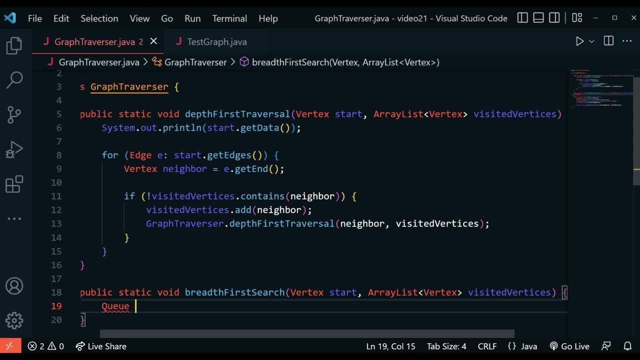 I use the queue, So I'm going to create a queue here as well. So, queue, and I'll call it visit queue, And here we're going to equal it to new queue. So q? u, e, u, e, And we're just going to put. 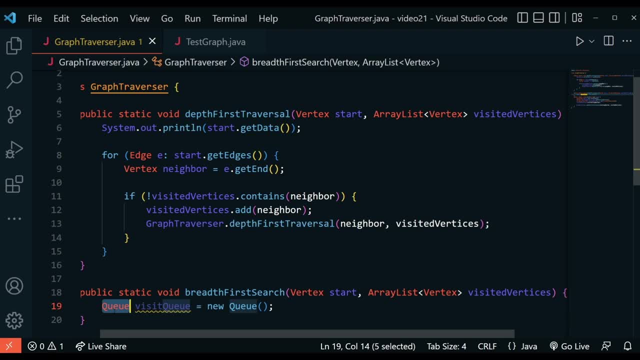 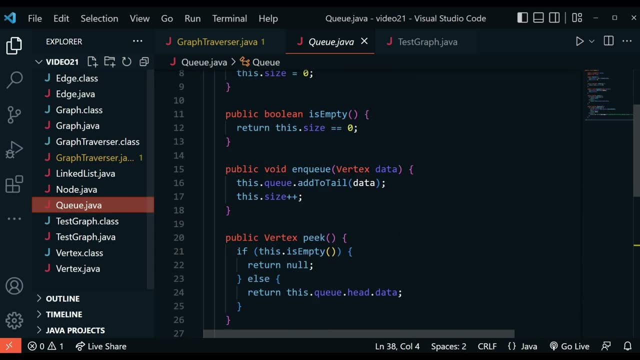 that as well. Now you might be asking: where is the queue coming from? Well, I actually have the queue file here as well. So this is the q dot Java file, and we've created queues before, but I actually modified it here a little bit. 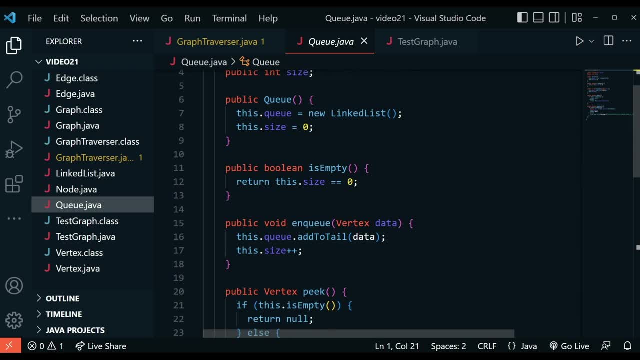 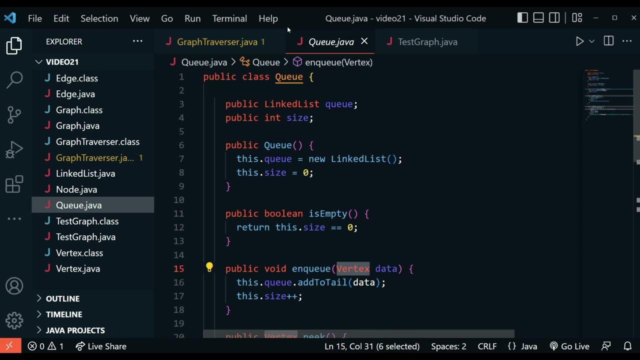 So the same exact queue that we've created in our video series, but I just modified it a little bit just to add vertex as the data now, instead of a string or some kind of integer. So removing that, and now let's just go here And over here. now we created our queue. 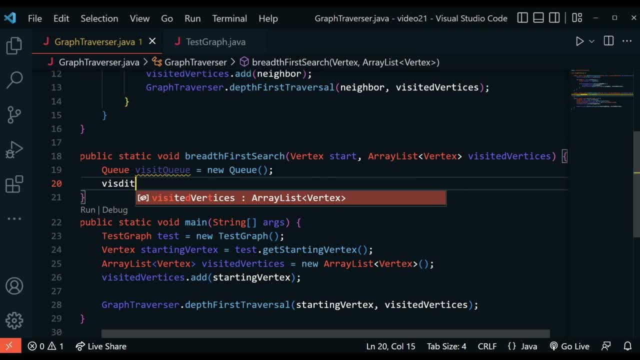 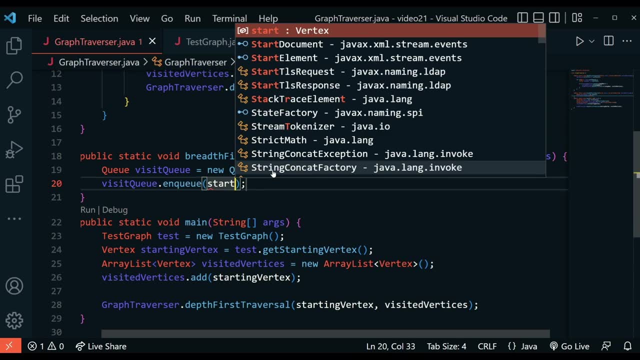 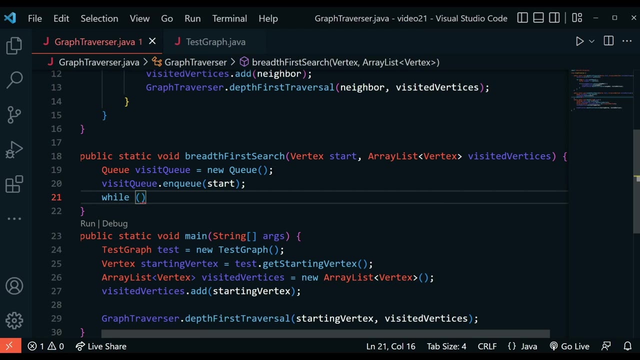 it's called our visit queue And we're going to have the visit q dot nq first thing, which is the start, which was passed in as the input parameter And that's the vertex there. Now we're adding a while loop And this is going to go until the visit queue is not empty. 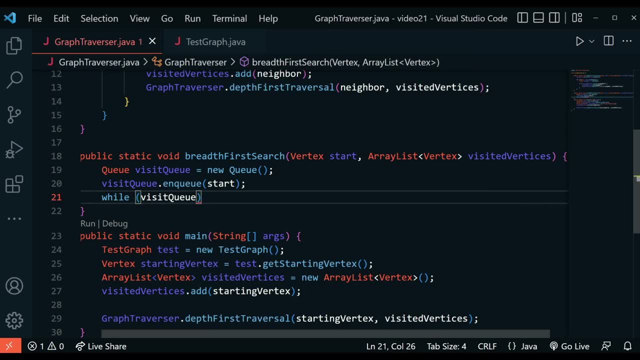 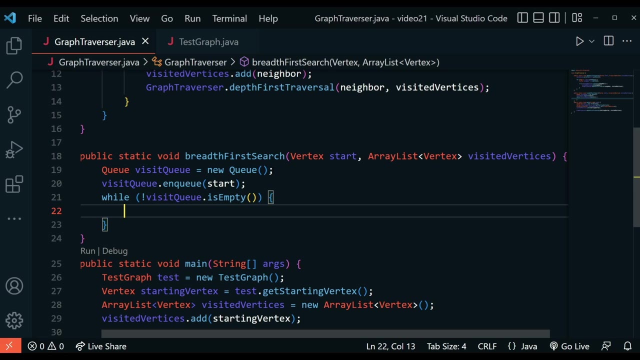 So I'll say visit queue, because this is a queue, it has this method, which is is empty And I've created that one. So I'll say, if it's not empty, we're going to go inside of this visit queue and keep doing those removing queue things And you know, traversing and using. 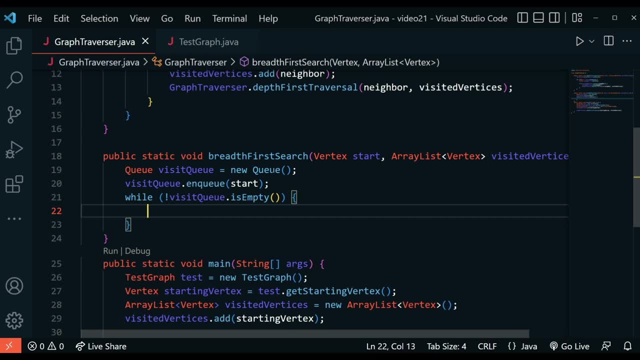 breadth, first search there. So for that I could let's just get something down and actually dequeue the, the element in the queue. So we could say visit. So we could say visit q dot dequeue. And here we have a vertex that we have to dequeue. So we'll put it inside of a current variable. 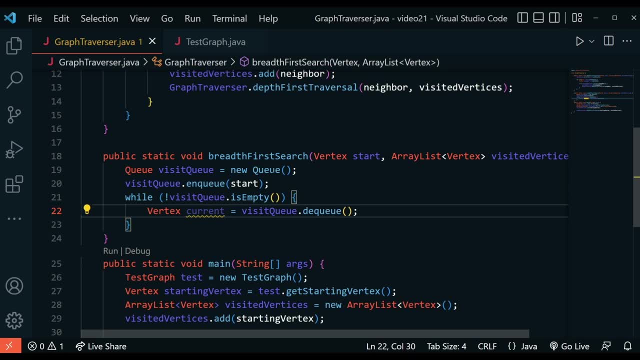 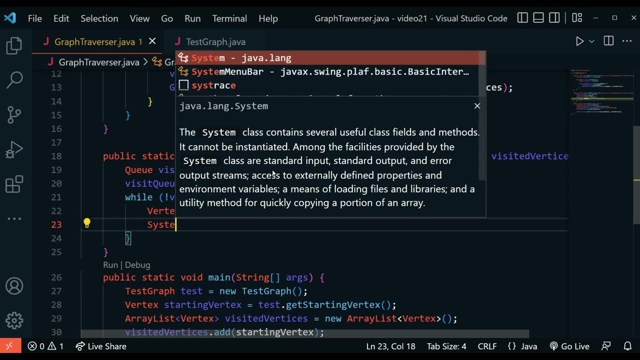 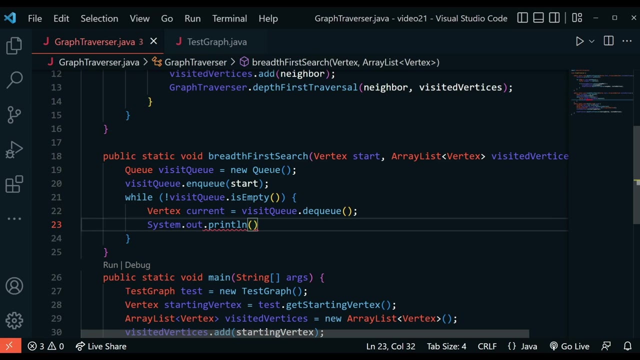 So I'll say current, All right, so now that it's in current we could print out the value here as well. as we'll say: system dot out, dot, print ln. And then we say: you know current dot data And there's a get data method. that was in the 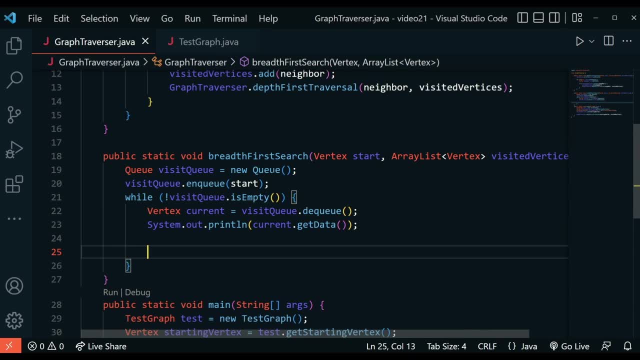 vertex class. So there you go. it's working there, Now that we're using a for each loop to go through each of the edges inside of this current vertex, because that's what I showed you in the graphical implementation. Now I'm just mapping all of the entire explanation down in code. 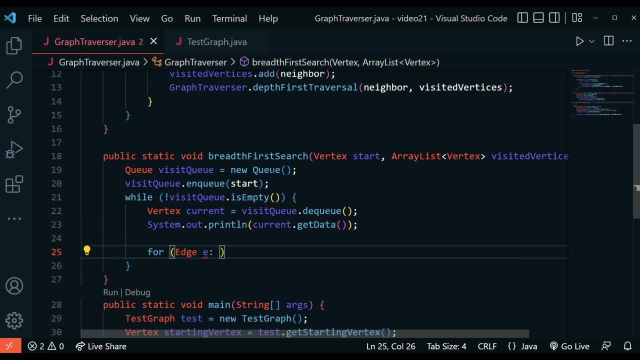 So I'm saying edge for every edge of the current vertex. so it's a current dot get edges, which is returning an array list of edges, And what we could do here is that. so now we're going to get the neighboring vertex of the current vertex To do that we could easily get it from. 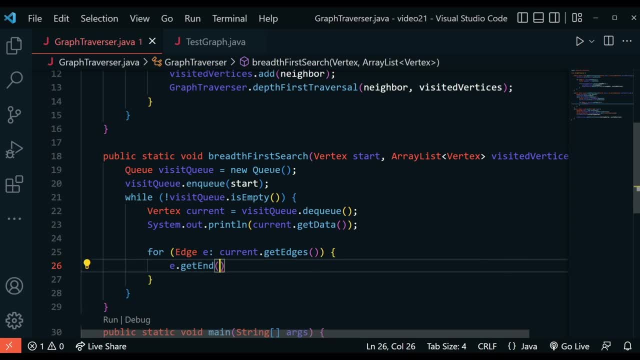 e dot, get end And that returns us a vertex that's our neighboring vertex And we pass it in to this vertex variable and I'll call it as neighbor And over here will apply a conditional And we'll say if the now, since I'm using a visited vertices array list over here in my input parameter that checks if. 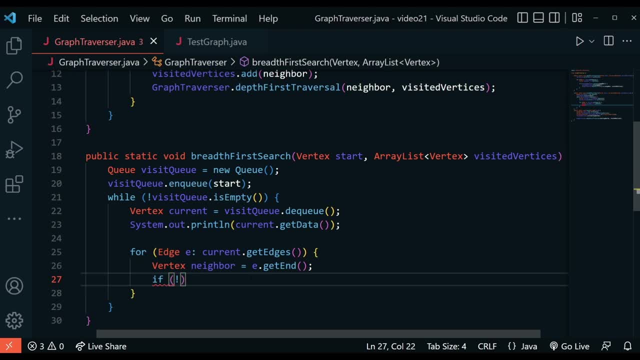 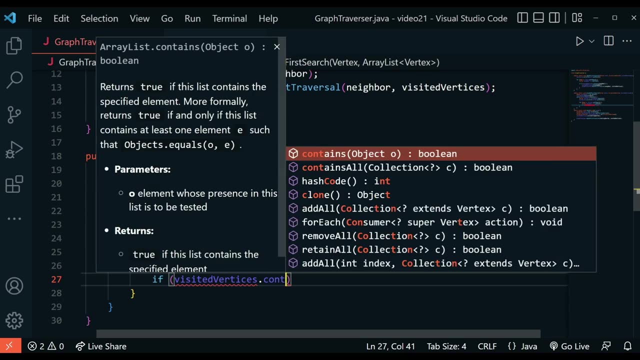 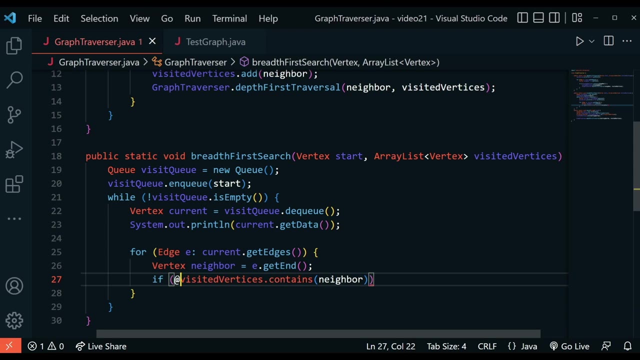 something is not repeated twice. so I'm saying: if it's not existing, so I'll say: if visited vertices dot contains and a neighbor thing, and he I, g, h, b o r. So I'm saying: if it does not contain it, then you should add it. So I'm saying, if it does not contain that neighbor vertex. 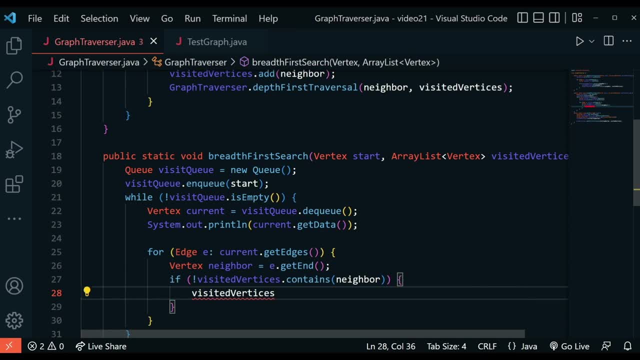 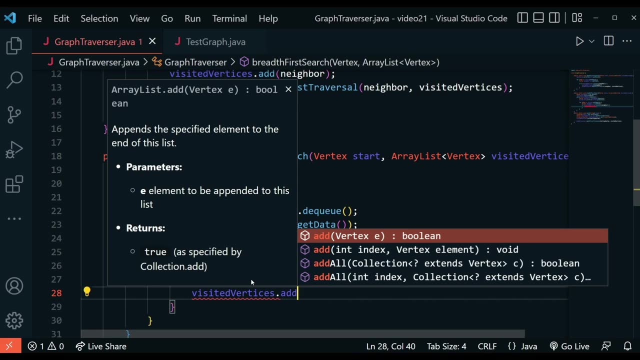 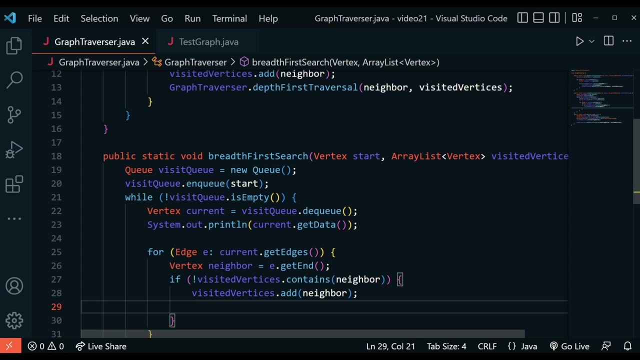 then you should add it. So we'll say: visited vertices, dot add, And so visited vertices, dot add, And then we'll add in the neighbor vertex Perfect. And then the last thing that we could do here, because we created this, visit Q and we'll include: 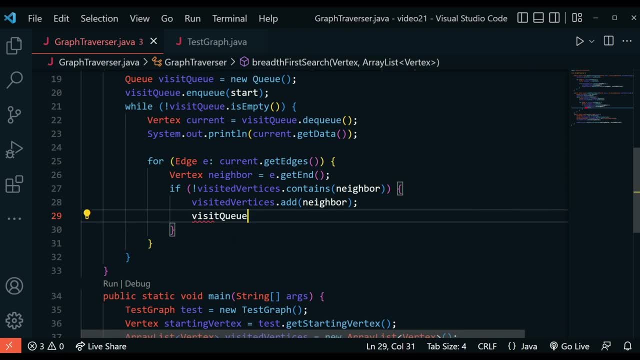 this inside of our visit queue. So we'll just say visit q dot n. q, which is this, and we'll put in a vertex data. So we'll put in that vertex, which is the neighbors, and e, i, g, h, b, or so this will be. 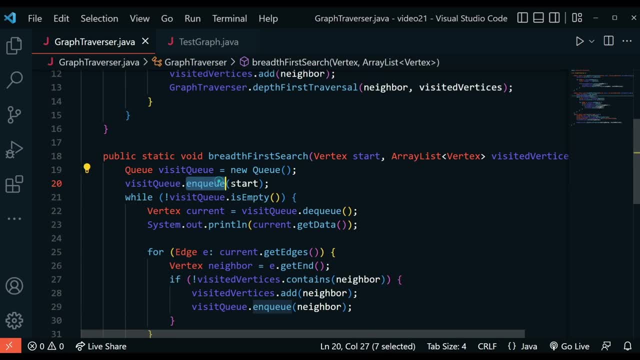 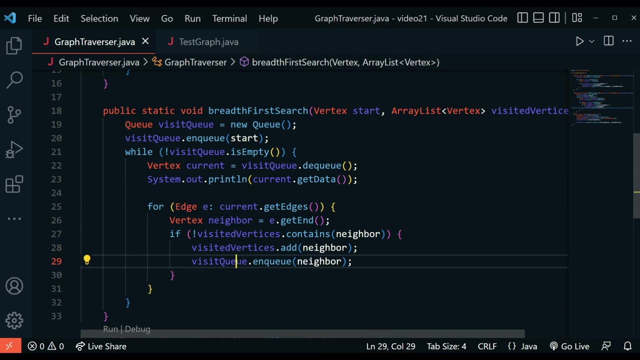 inside of our visit queue. So we'll do that X dot add And we'll put in the neighbor vertex into our, which is um this queue, and it just currently had only the start. but once when you get the edge of the, the neighboring vertex, you also pass that inside of the visit queue. so that will be now. 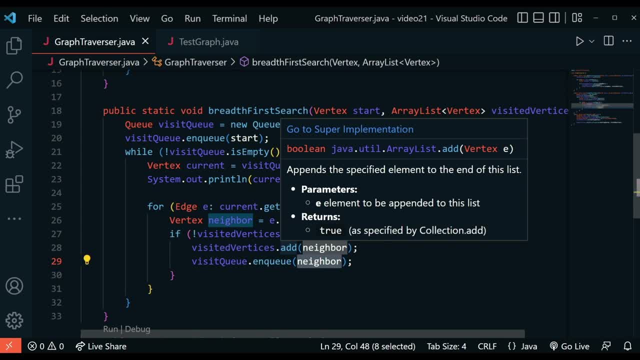 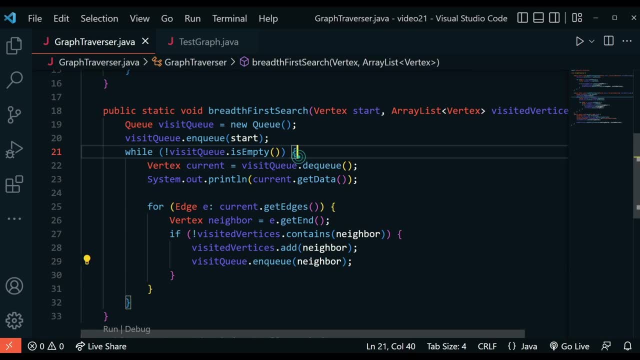 the current vertex and it will go until, um, there's a dead end, and then it will just um, remove from the in queue and then so once it's exhausted, like you see over here in this while loop- so it's just going to say until it's empty, not empty. so it's just going to keep going and once it's exhausted, 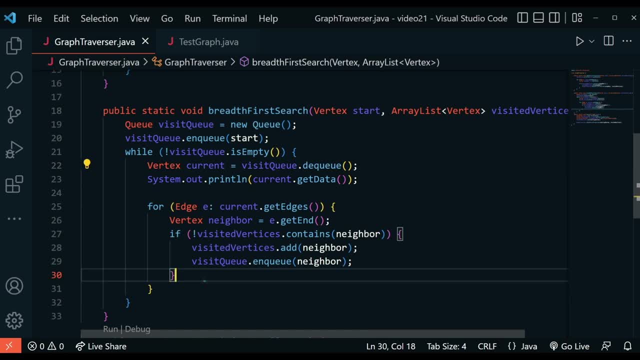 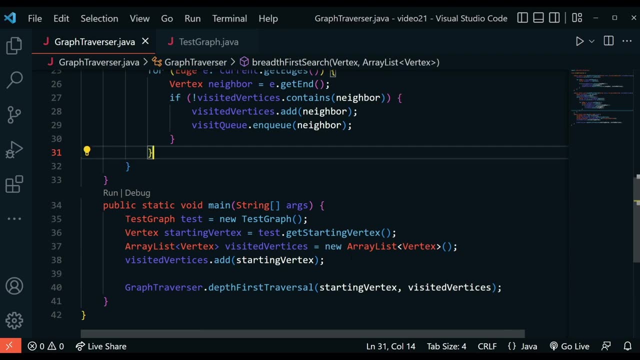 like you can see over here, dq. so just see the other vertices that are there to traverse. now let's go down in the main method and just have everything over here set like this: so just pause the video and type along and over here for the starting vertex: test dot. starting vertex. here we 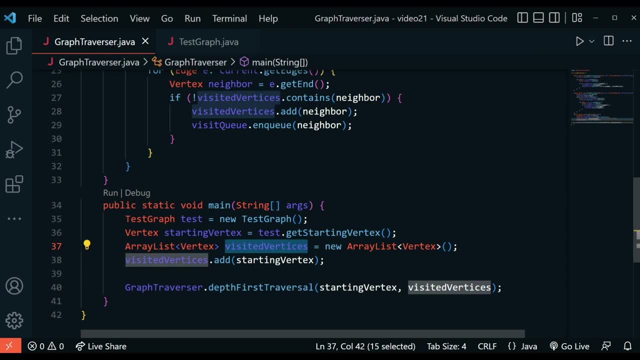 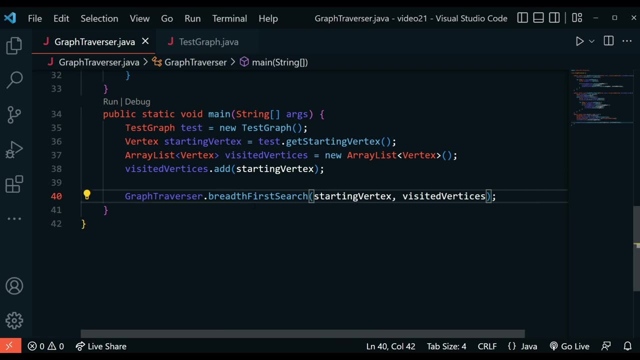 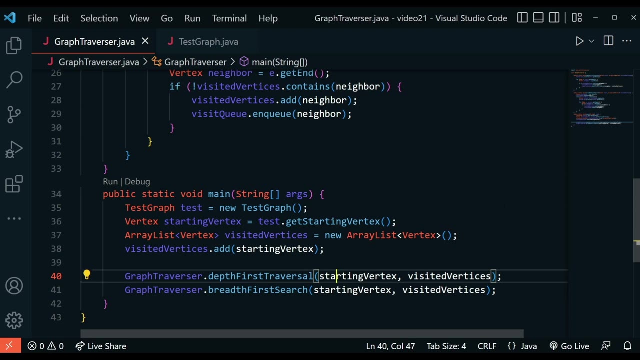 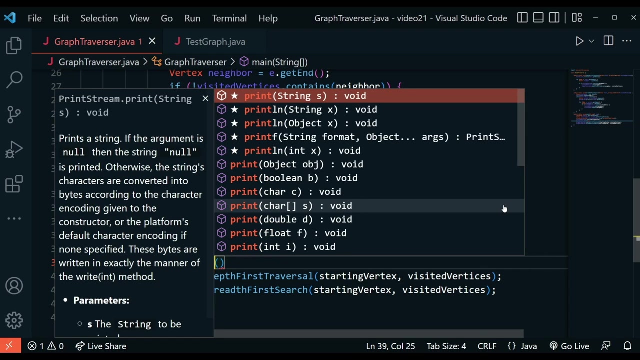 have a array list, vertex, visited, vertices: the same thing, and this is the same exact thing. so instead of depth, first traversal, we're going to say v, breath, first traversal, and the rest is history and compiling it and running it. let me just label them as well. so jump that out: dot, print, ln, or we just have a line here, so print, and then we say: 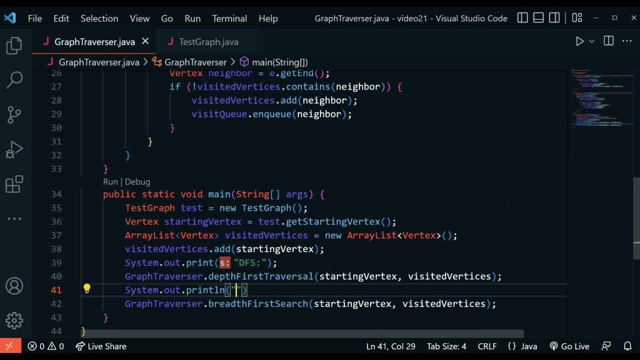 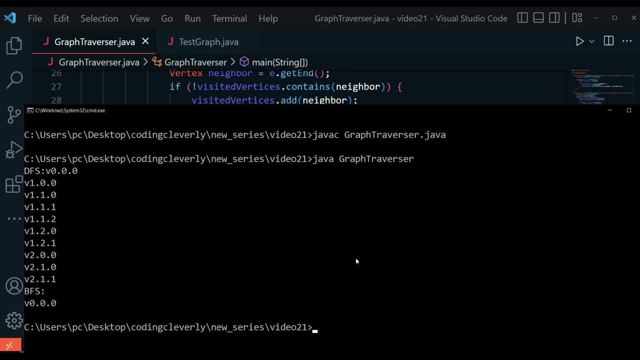 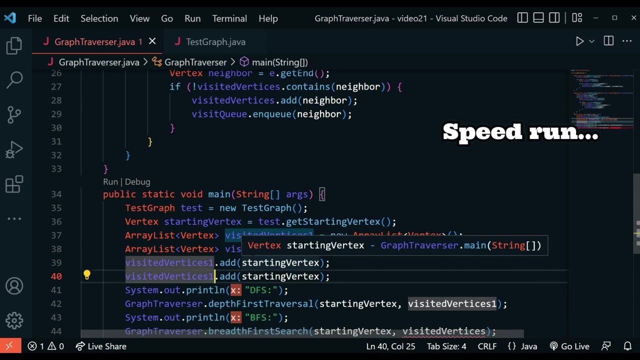 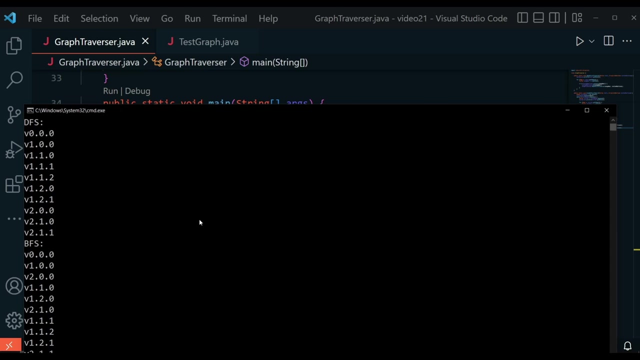 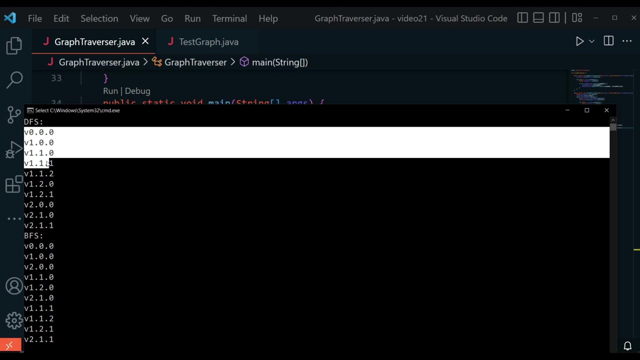 d f s, i'll say b f s, run this. so here you go, the difference between the two of the traversal techniques. here we have dfs, at the other side we have bfs. so we have over here zero, one one and something like that, and then we have. 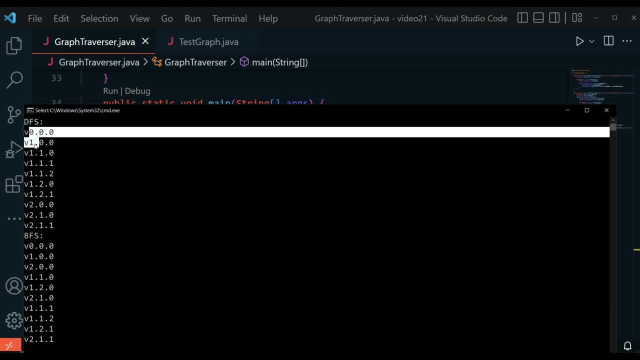 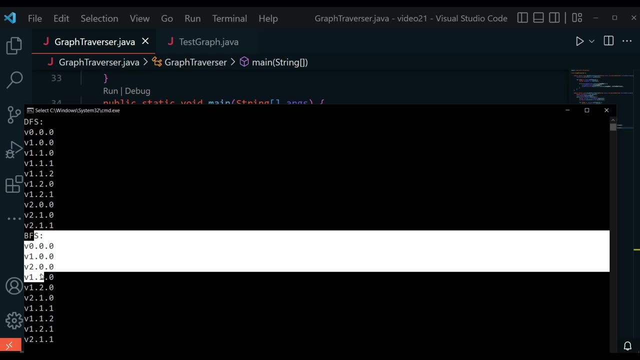 two over here, so something's going on differently. but if you look at the total numbers- one, two, three, four, five, six, seven, eight, nine, ten- one, two, three, four, five, six, seven, eight, nine, ten. one, two, three, four, five, six, seven, eight, nine and ten, so the total number should be ten and there's ten over here. 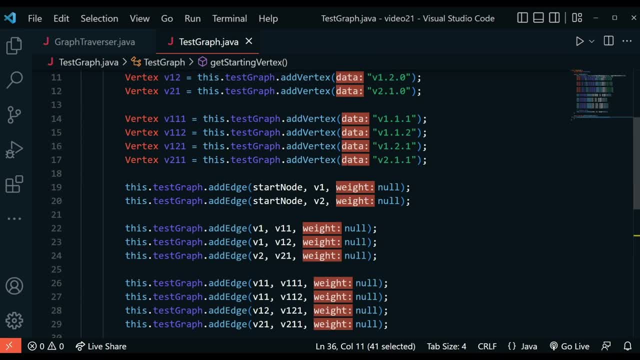 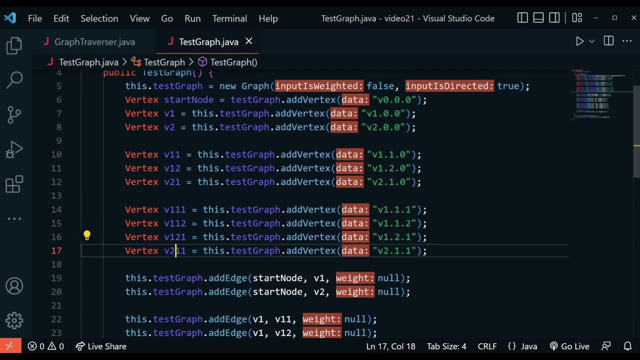 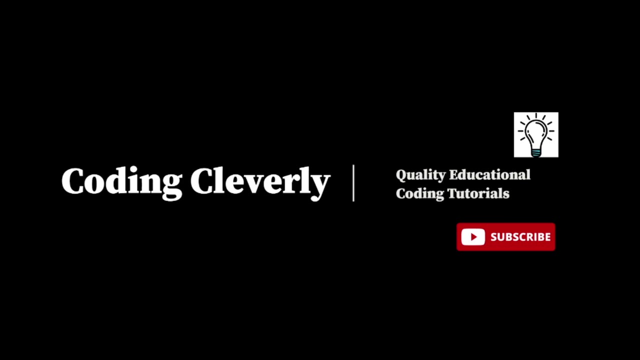 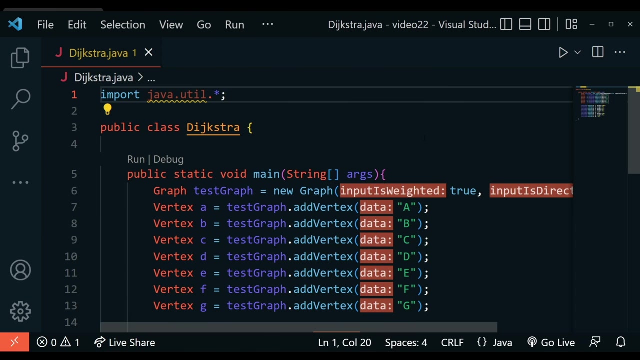 and there's ten over here, and if we look at the test graph, dot java here. so the start, node one, two, three, four, five, six, seven, eight, nine and ten. awesome, so that was it. that was my code for depth, first traversal. welcome to another video. today we're going to be talking about dykstra's algorithm, a very important. 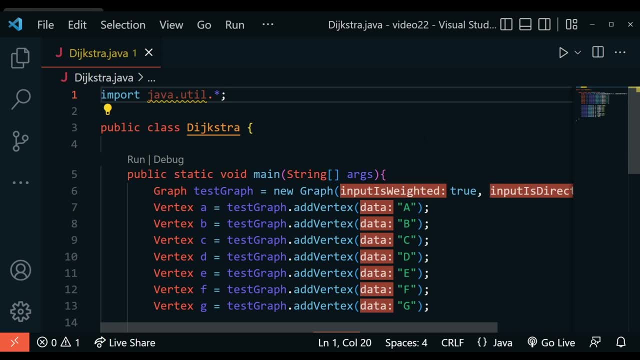 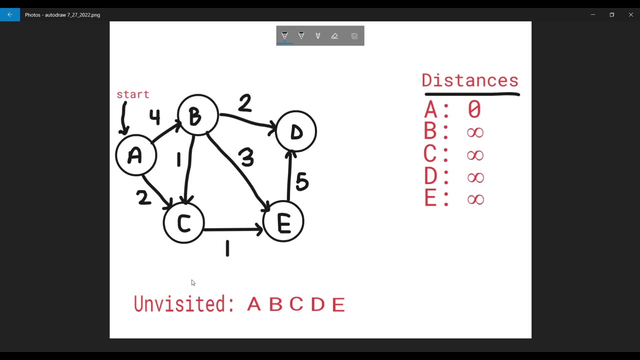 algorithm. in the computer science world, finding the shortest distance between vertices is one of the most common applications of graph searches. finding this distance has a number of applications, including determining the best route to a destination and transferring data over a computer network. consider the graph finding the shortest path between vertex a to vertex e. 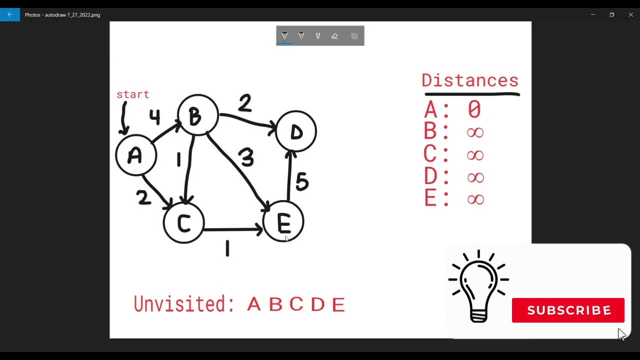 may appear simple in your mind, but telling a computer how to do so is a bit more difficult. Fortunately, there is an algorithm that computes the shortest distance between any two vertices in a graph. This is known as Dijkstra's algorithm. Now let's look at the conceptual overview. 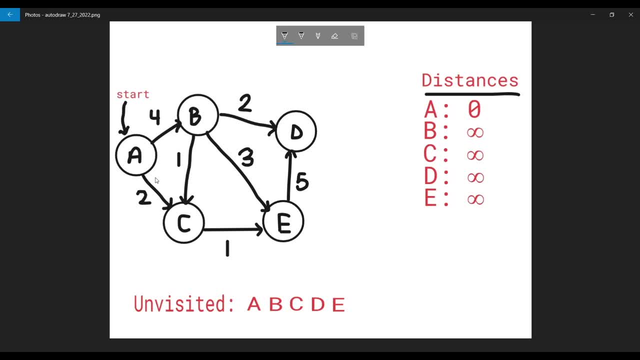 of how the Dijkstra's algorithm is going to work. We're gonna start with the starting vertex and you can see that the start is pointing to A, So this is my target vertex. Here I have a distances cube and I also have this unvisited, which is in the bottom. 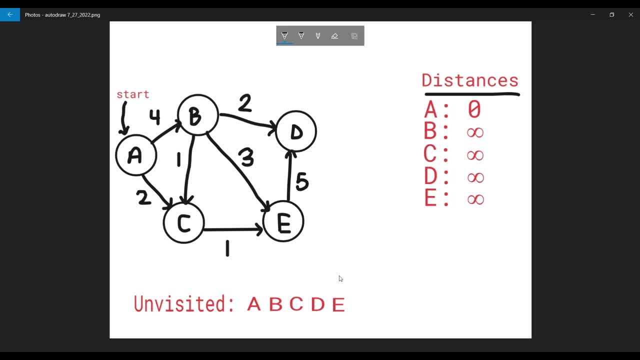 Now I'm gonna look at the first step here in this algorithm, and the first step is to pop off the minimum distance of the unvisited vertices. Now you can see over here, the minimum distance here is zero and these rest are all set to infinity. 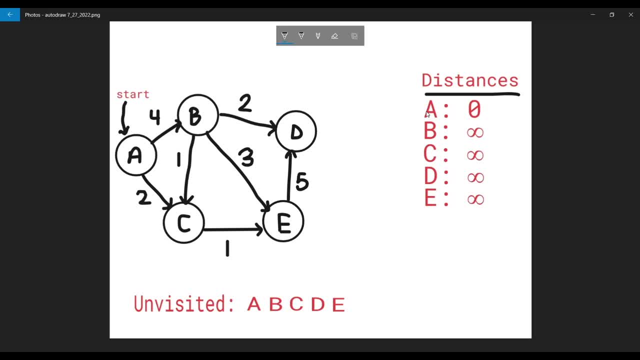 meaning that the distance from A to itself is zero and the distance from A to any one of these vertices is infinity for now. And if we look at the minimum distance right now, it's zero. So we're gonna pop this off. So we're gonna pop it off from here. 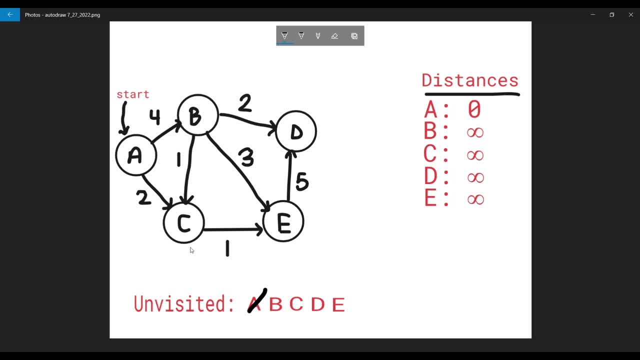 and then we're gonna look at the adjacent vertices corresponding to this first vertex. So you can see over here. so from A to B, the distance is four. Now, if you compare this with the original distance, which is infinity, now four is less than infinity. 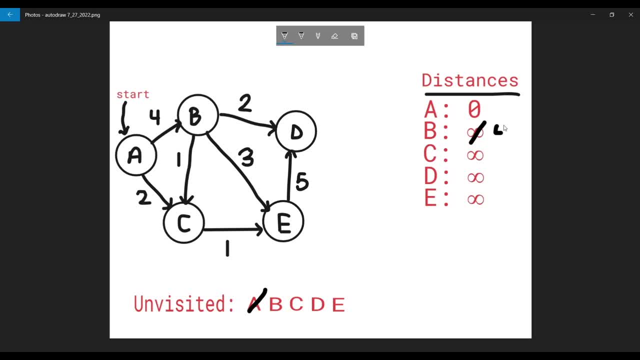 so we could replace this infinity with four. Since we replaced that, now we could also go and check the next corresponding distance. Now A to C has a weight of two. Now you could see that two is less than two, and then you could also go and check the next corresponding distance. Now A to C has a weight of two. 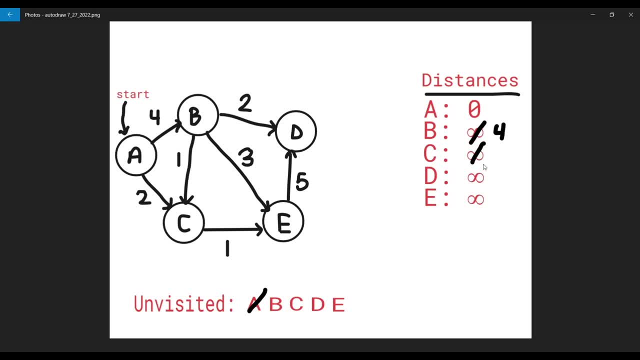 Since we replaced that, now we could also go and check the next corresponding distance. Now we could also replace this infinity with two. Now we're done with that, and this is our first iteration of the algorithm. Now we're gonna go to the next iteration. 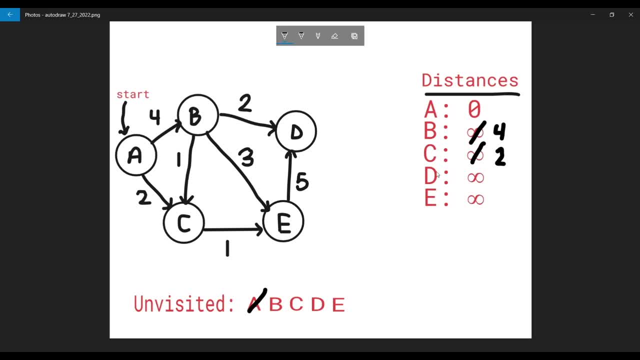 Now we're gonna pop off the minimum distance of the unvisited vertices and for now we could see that two, which is for C, is the minimum vertices. We're gonna pop that off from here and we're gonna start with C. 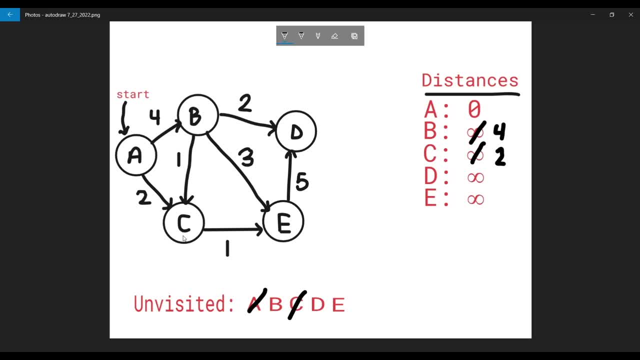 So you could see C has. So C only has one neighbor, and that is E, And the distance from C to E is 1.. And you have to look at the distance from A to C too. So the A to C was 2, and from C to E was 1.. 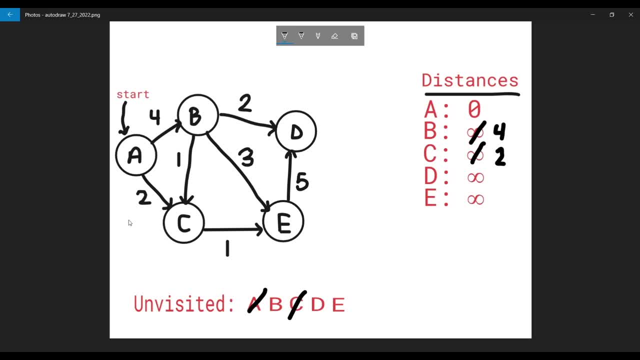 The total distance from A to E is 3.. So 2 plus 1 is 3.. So what we're going to do here is we're going to make from A to E as 3.. And then we're going to look at the E portion. 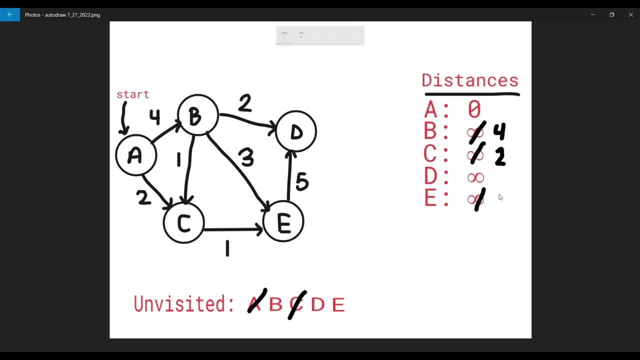 and we're going to see that 3 is less than infinity, so we're going to replace this infinity with 3.. Now, since there's no more neighbors left, we're going to do the next iteration, for this algorithm C has no more neighbors. 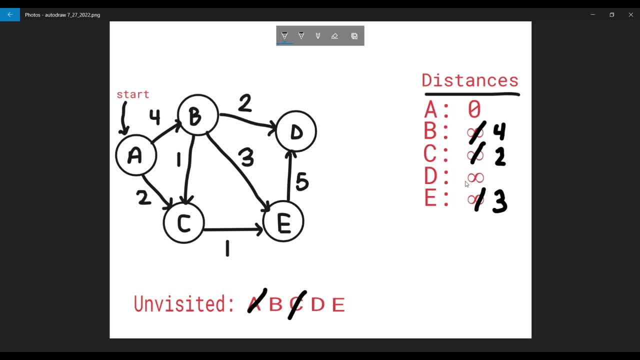 So now we're going to pop off the minimum distance of the unvisited vertices. You can see now that the minimum distance is 3.. So it's in E. So we're going to pop this off and we're going to go to E. 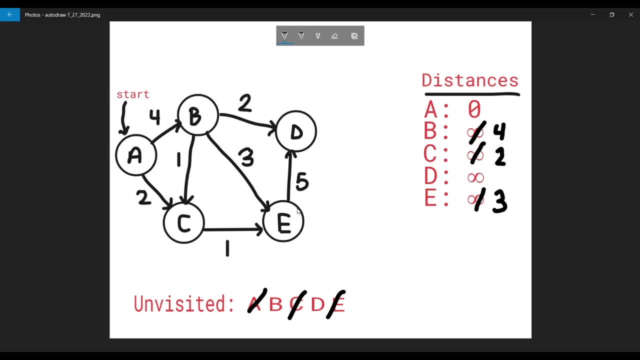 And look at the neighbors for E. So E has only one neighbor, and that is D. The weight for that is 5.. The distance will be 3 plus 5. Which is 8.. And 8 is less than infinity. so we can replace this infinity with 8.. 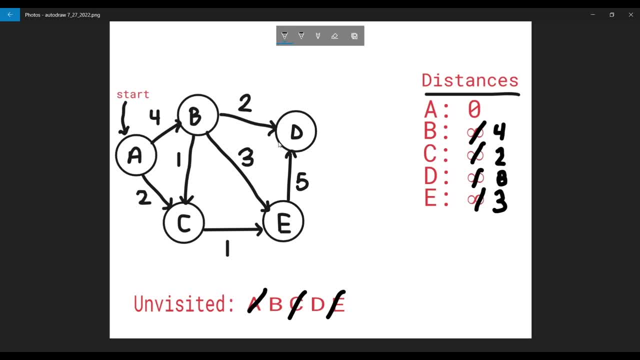 Now that we have replaced that, we can also see that there's no more corresponding vertices, So we can stop here and do the next iteration for the algorithm. Now we're going to pop off the minimum distance of the unvisited vertices, So you can see that the minimum distance is B. 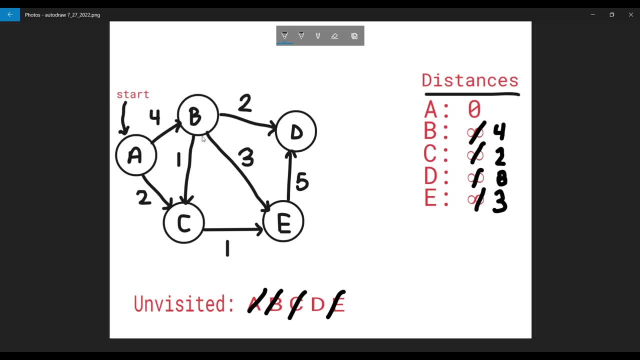 So we're going to pop this off And over here we're going to look at the corresponding neighbors. Now B has 1,, 2, and 3 corresponding neighbors. We're going to start with the first one, which is C. 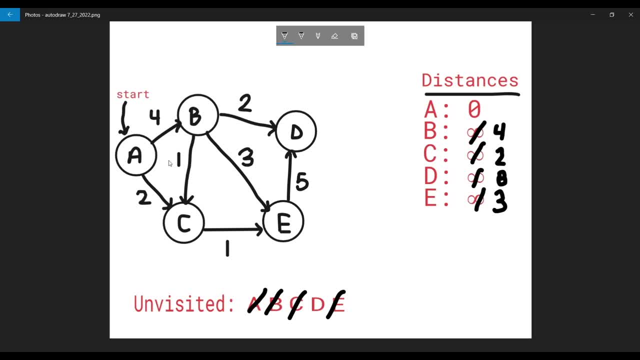 So B to C is 1.. And now you can see that from A to B, which was already existing, was 4.. And from there to C it's 1., So 5.. So from A to C will be 5.. 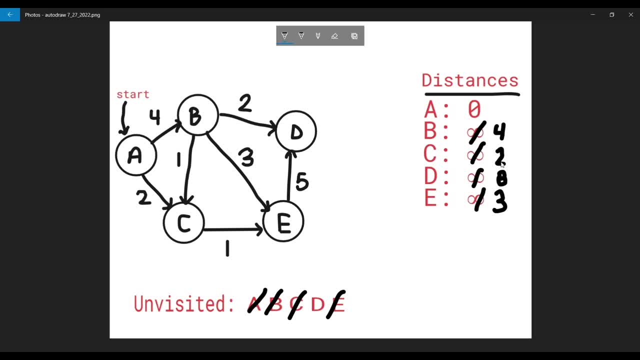 And if we look at the C, it already exists here And you can see 5 is greater than 2.. So we're not going to change this value. Then we're going to look at the distance: Distance from B to E. 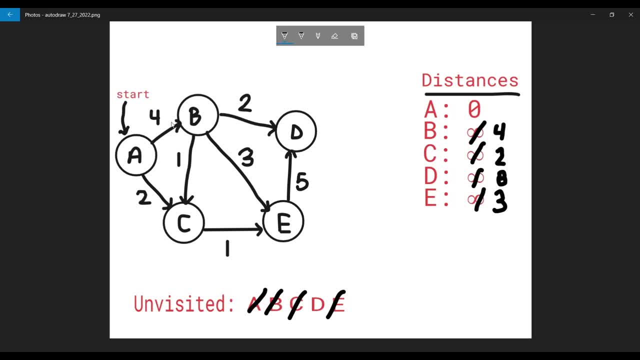 And that's 3.. So from A to B it's 4. And from there to E it's 7.. So if we look at the distance from A to E, that should be 7. And that is greater than the value that we already have here. 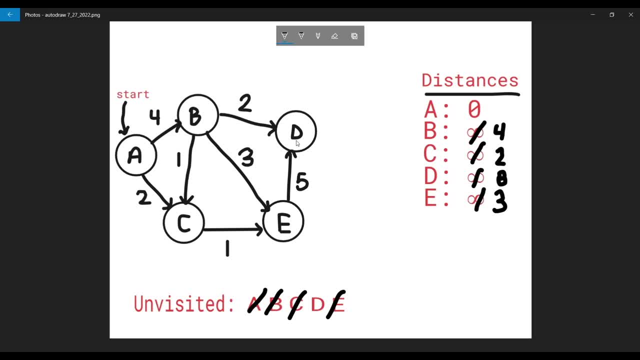 So we're not going to change that at all either. Now we're going to look at the last and final neighbor of B, And that is D. Now, if we look at the weight, this is 2.. And the distance from here was 4, 2.. 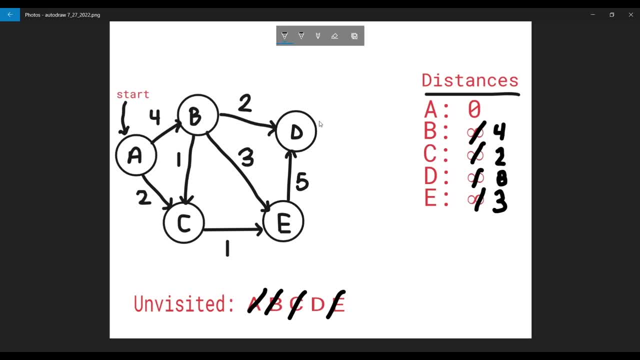 So it's going to be from A to B, it's 4.. And from B to D it's going to be 2.. So the total distance here from A to D will be 6.. And if we look at the distance over here, 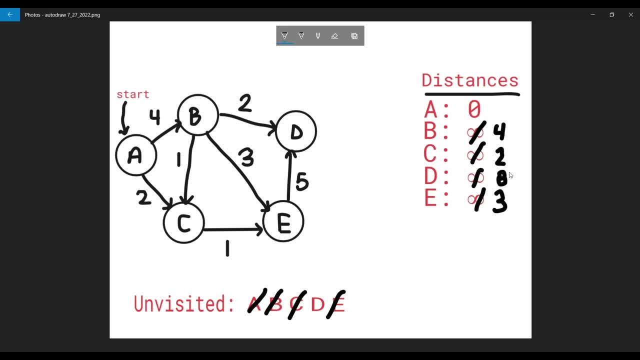 that is actually lesser than what we have existing, So we could replace this 8 with 6.. And that now will be the end of our iteration. And now we'll go to the next iteration of our algorithm. Now we're going to try to pop off the minimum distance. 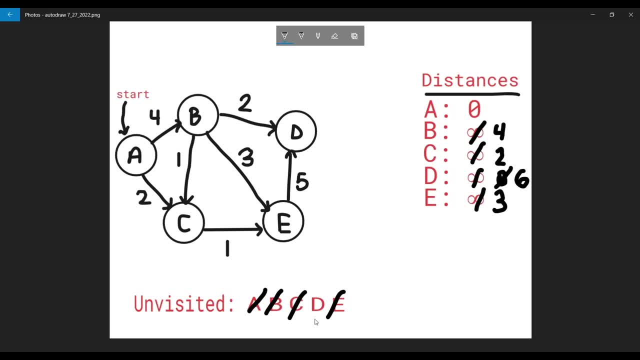 of the unvisited vertices, since we only have one vertices left, which is D, And we look at the minimum distance here, And that is the minimum distance. Everything has been visited, So that's D, So we're going to pop it off. 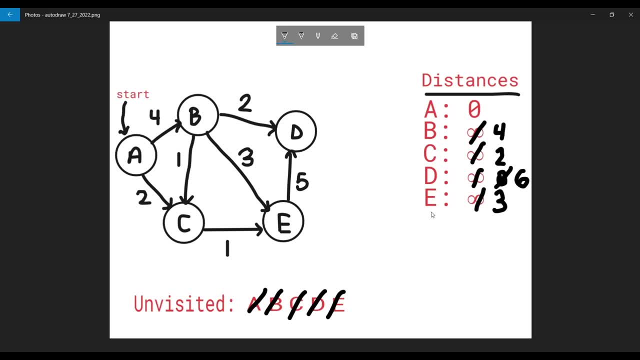 And we try to look at any neighbors for D, but there's nothing. So that's the end of our algorithm there And that's how Dijkstra's algorithm is implemented. So you went over there and saw all of the possible distances. So, from A to itself, the minimum distance is 0. 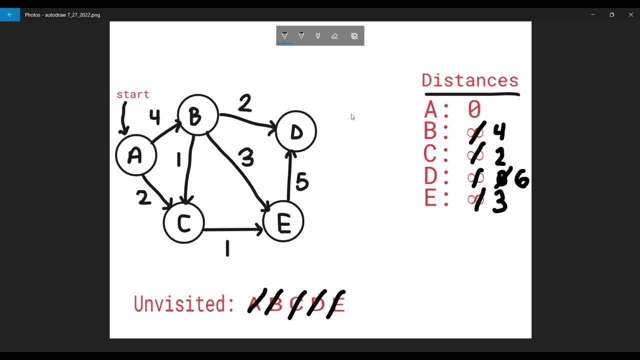 From A to B, the minimum distance is 4 till here. From A to C, the minimum distance is 2, right here. From A to D, the minimum distance is 6, so 4 till here, And from A to E, the minimum distance is 3.. 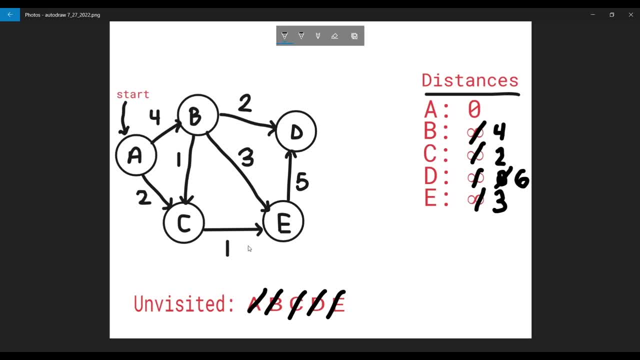 So A to E is the minimum, distance is 3.. So that sums up our Dijkstra's algorithm conceptual overview. Now we're going to start writing the code for this. But before getting on to the code, let's think of what we should add in. 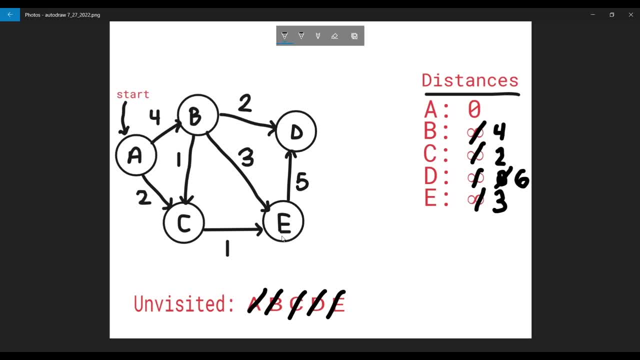 or what objects and what structures should we create? Looking into this algorithm, we're going to instantiate a dictionary that will eventually map vertices to their distance From the start vertex. So, like you can see over here, we're going to put that in a dictionary. 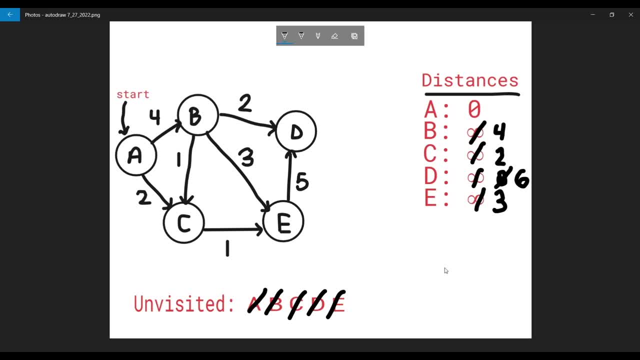 A quick recap before we start the code for this. Dijkstra's algorithm finds all of the shortest distances between a starting vertex and the remaining vertices in a graph. The algorithm operates by keeping track of all distances and updating them as it performs a breadth-first search. 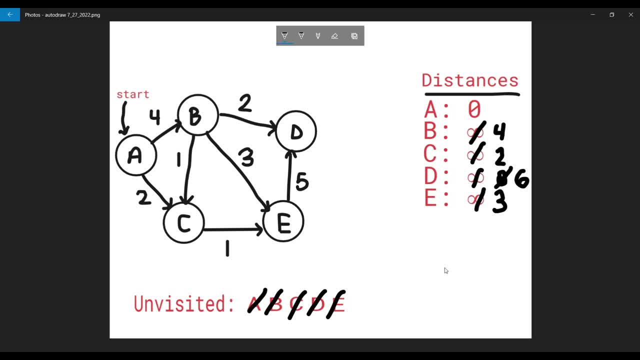 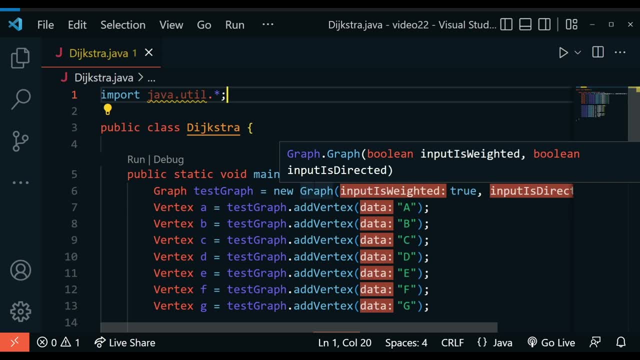 Dijkstra's algorithm is implemented in O of E plus V of log of V, And E means edges and V means vertices. We will first implement the algorithm to find the shortest distance to every vertex. So let's go for the code And all of the conceptual overview that I gave. 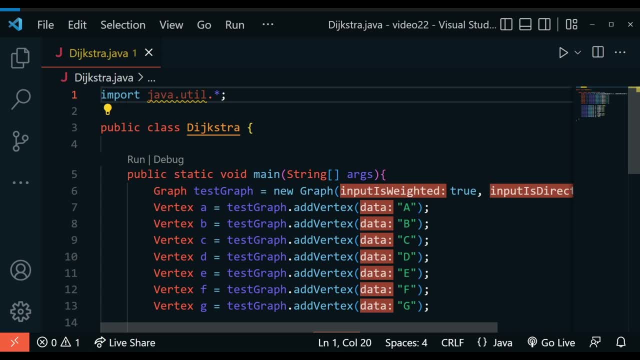 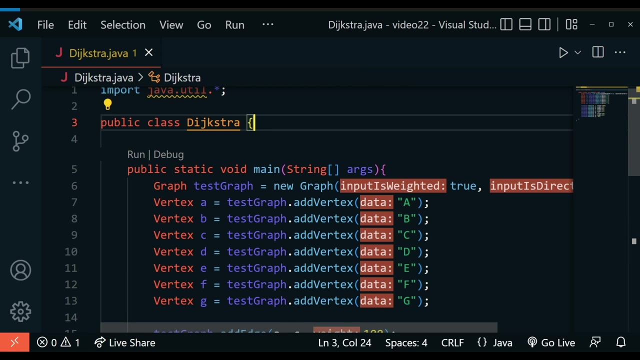 now I'm going to try to map this out in code. So here I have imported javautilasterisk, meaning I'm importing everything that's available in the utility package And over here that you can see is public class, Dijkstra, And there I have a main method. 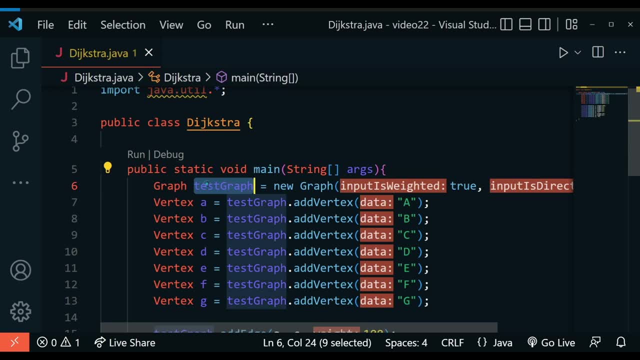 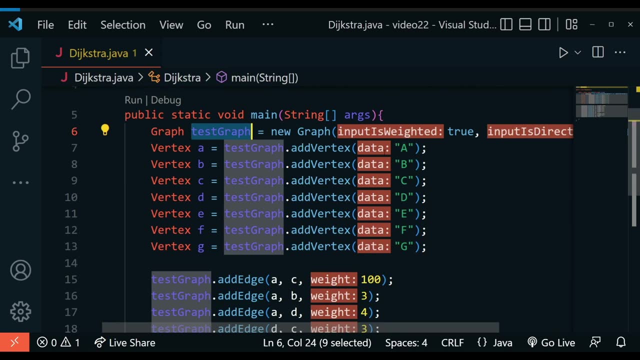 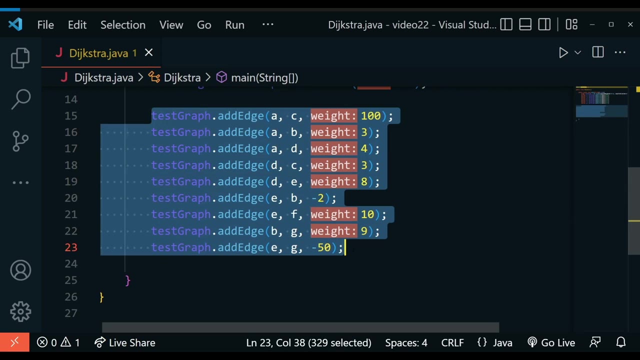 Here I have a main method which is actually creating a test graph, And the weighted and directed properties are set to true And we also add these vertices here. So A, B, C, D, E, F, G, And we also add their connections to each other. 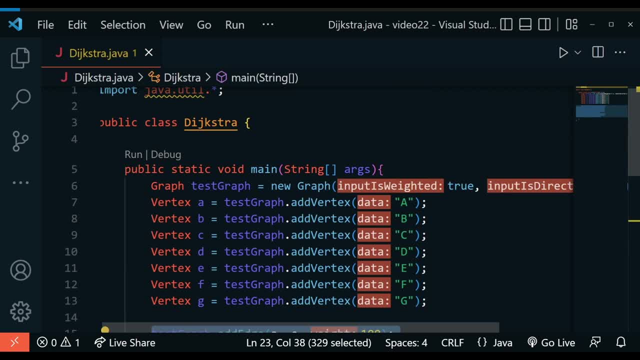 So those are done. So what we mainly have here is a test graph in our main method to test the output of the method, of what we're going to create in this video. So we're going to try to create that method, which is called Dijkstra. 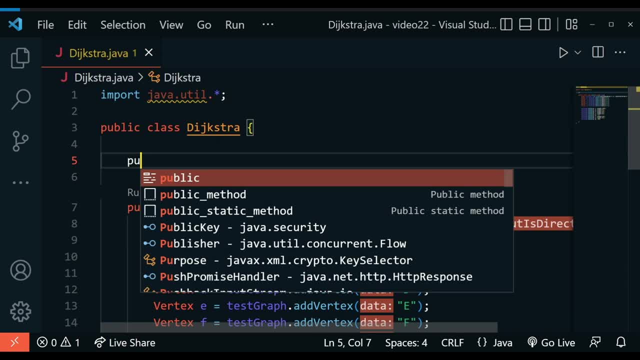 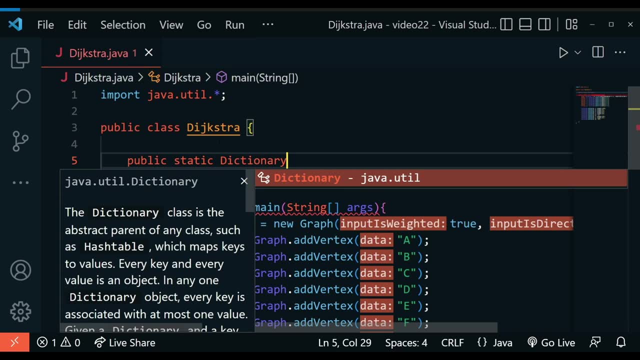 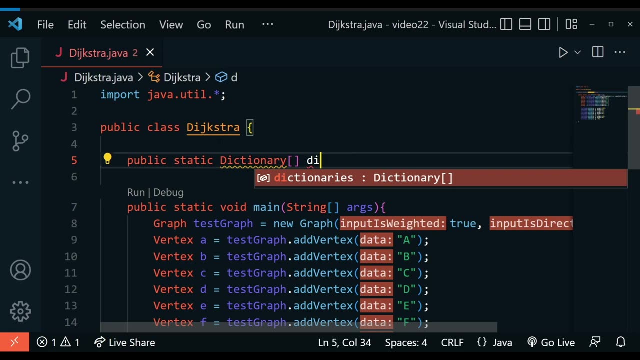 So for that we're going to have the public And we're going to say static dictionary And we put in this. So we're going to return an array of dictionaries And I'll tell you why we're doing this in just a sec. 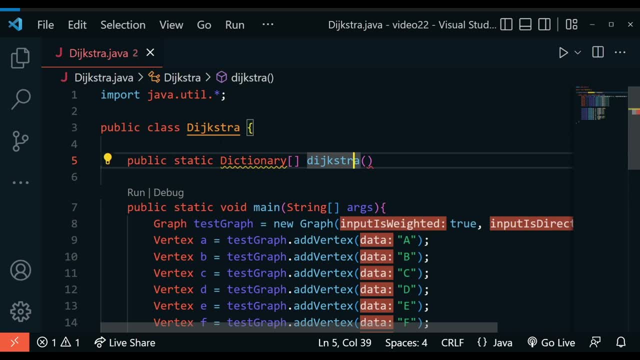 So here we have the name of the algorithm, Dijkstra, And we're going to tell the parameter to add in these two, And then we're going to add in the values. First thing is to have the graph, So D-R-A-P-H. 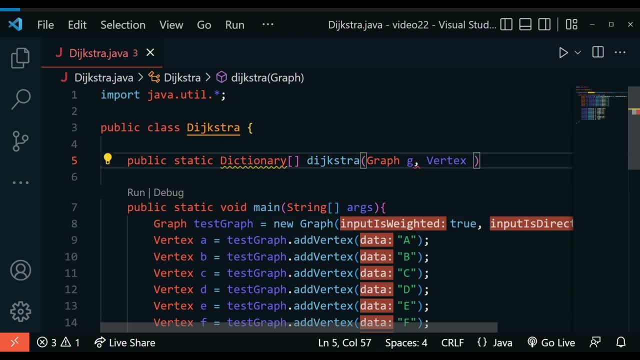 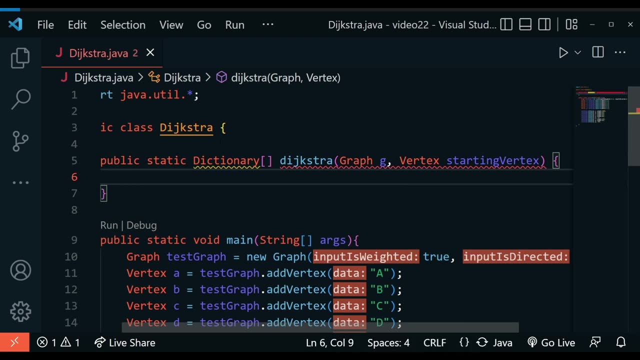 And we call that as G. We also need to pass in a vertex, And that one will be called as starting vertex. So we're done with these two input parameters. Now we're going to create two dictionary objects here, And one will be used for the distances Q. 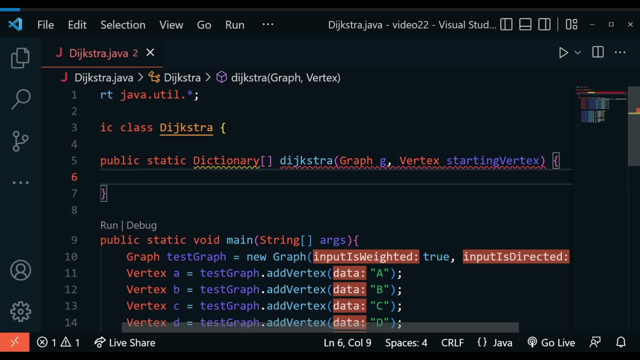 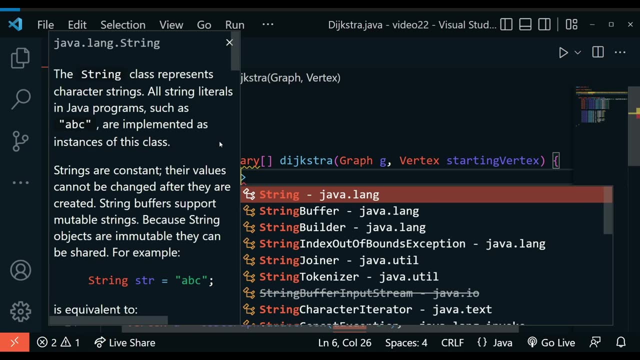 And the other one will be used to keep this vertex And this is very crucial in this algorithm. So we're going to make a dictionary, And a dictionary is just a base of key value pairs. We have a string, which is the key. 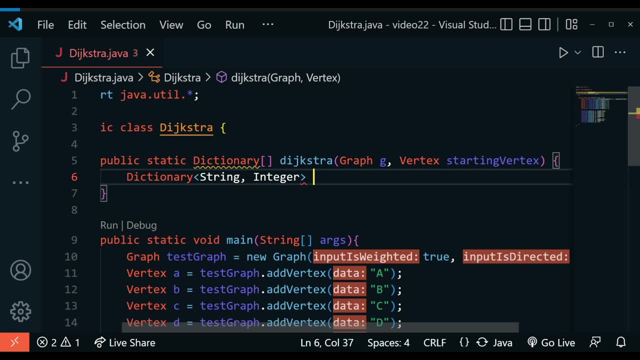 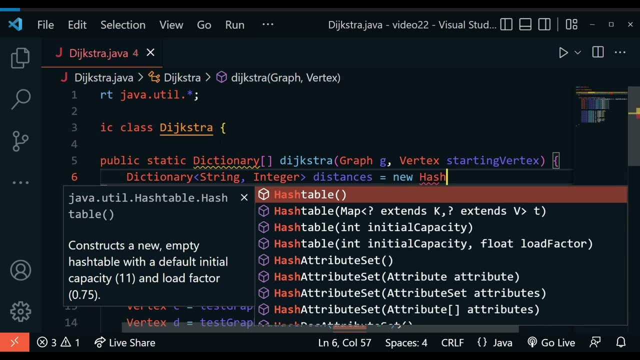 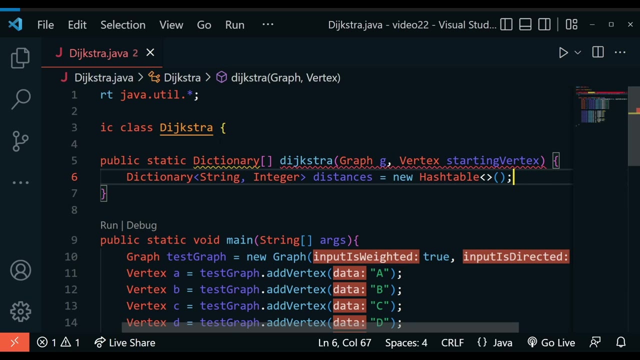 And integer as the value And we call this as distances And we create a new hash table And we put in these angle brackets and the round bracket And then we semicolon at the end. So that's the distances Q. Now we also need another hash table. 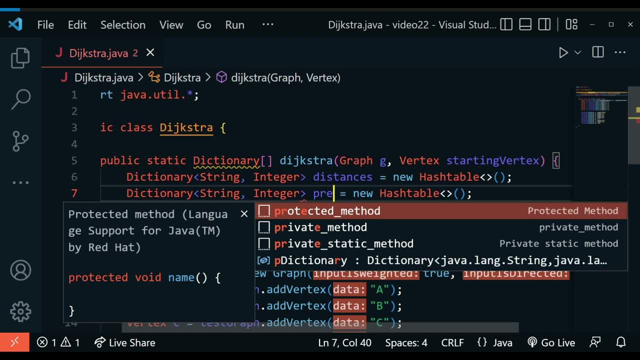 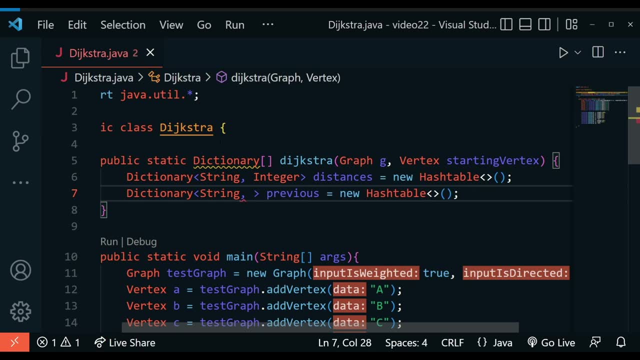 And this one will be for the previous. So we add this as well, And for this we're not going to have the integer as the value, but the vertex. This is going to store the data and the also value that exists. So, like I was doing it over there, 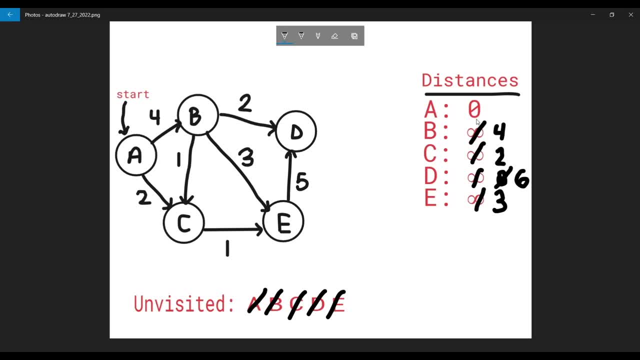 in the diagram, this A, and it maps out to 0.. And this B, that maps out to 4.. So the string is the letter And the value is going to be the integer. And for the second dictionary, which is previous: 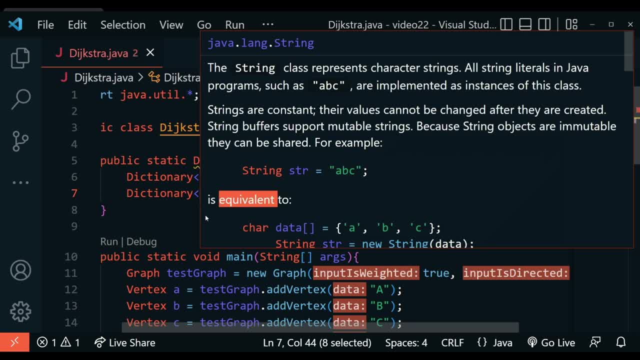 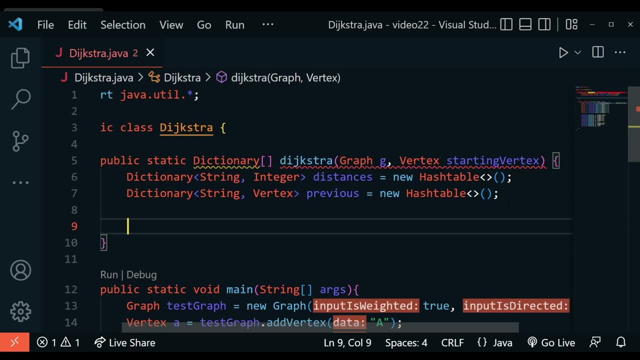 it's going to keep track of the previous vertex, So that will have a string which is the current vertex And vertex will be the previous vertex. Now we also need to add in a priority cube, So I have added some files here. 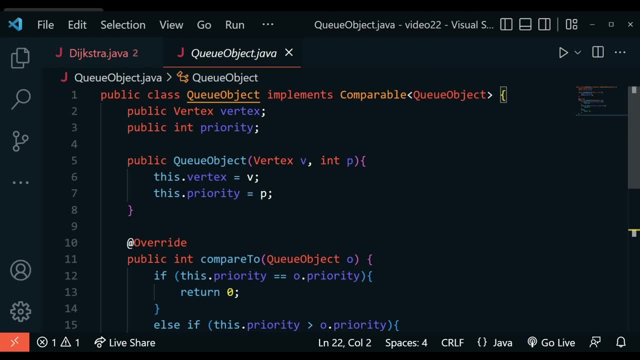 And this is one that's called QObjectjava. This is actually a class that implements the comparable QObject And you can see that it has the vertex and the priority as class variables And you can see the constructor is actually creating this object And it's overriding the compareTo method. 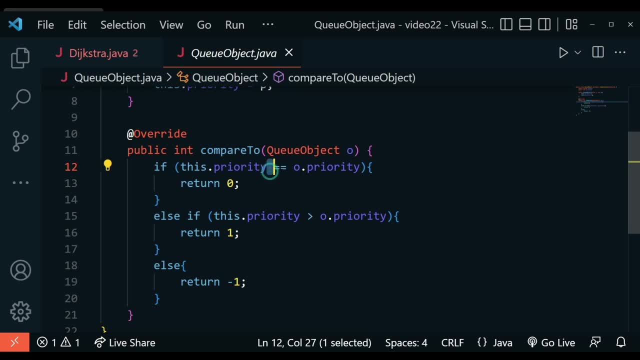 with some priority base. So if it's equal in priority to the input parameter, we just return 0.. If the class variable priority is greater than the priority that was passed in, then we will return 1.. Else we will return minus 1.. 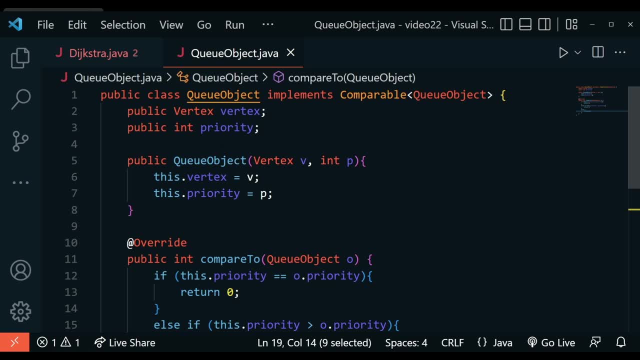 So this is just a file And it's just a fancy queue. It's just known as a priority queue. The main difference between this queue and the priority queue is that this will look at the smallest value, smallest possible value, And it will allow us to pop that one off. 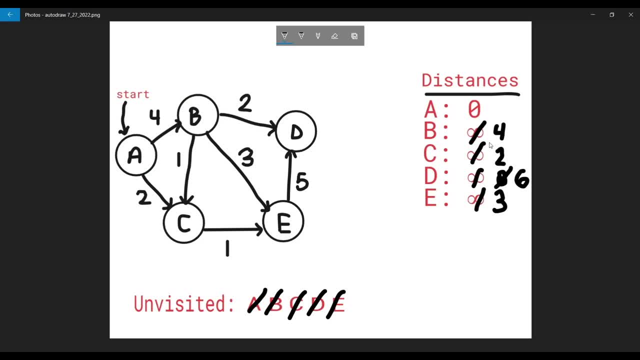 So, like what we're trying to do here, we were trying to look at the minimum value And we were trying to pop that off. That exact implementation, this priority queue, will do it for us without writing extra code, So that's one of the biggest benefits for using that. 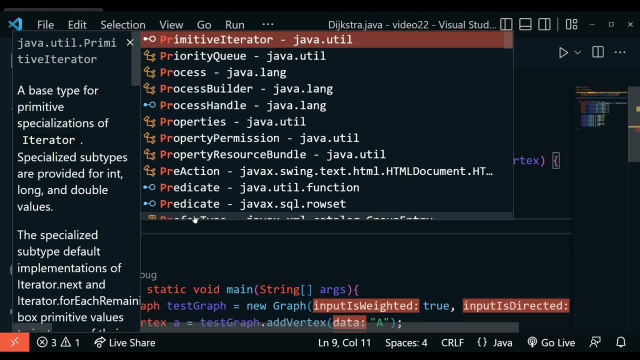 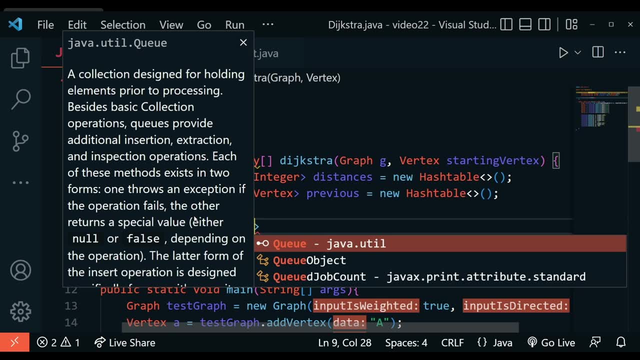 So let's add the priority queue And this is the priority queue, So priority queue, And we're going to add in the QObject here, So Q-U-E-U-E And we're going to say object that we created, And then we could add: 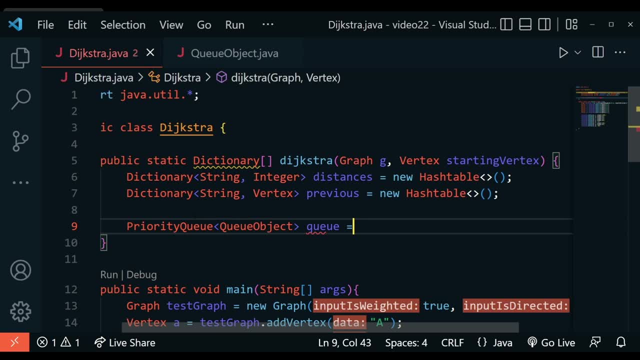 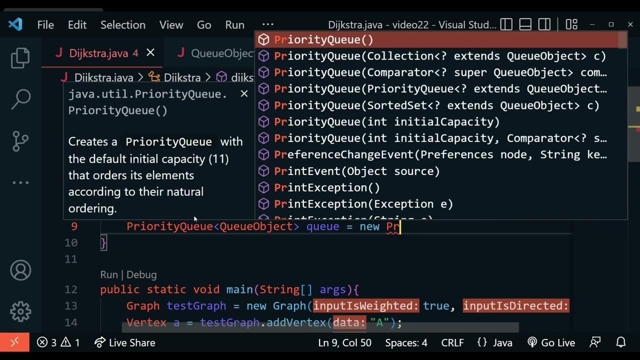 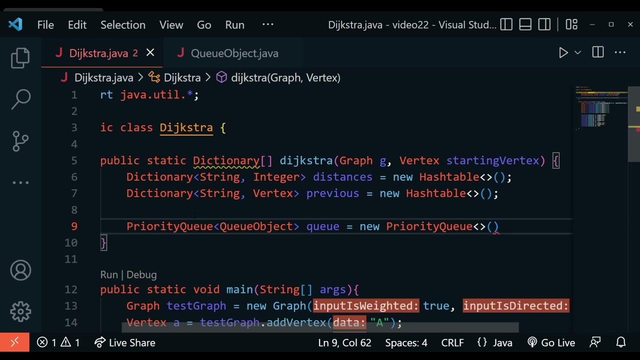 And name for that as Q. Q-U-E-U-E is equal to. Now we're going to add in the new And we'll say priority queue, And here we're just going to add in the QObject once more: Q-U-E-U-E-O-B-J-E-C-T. 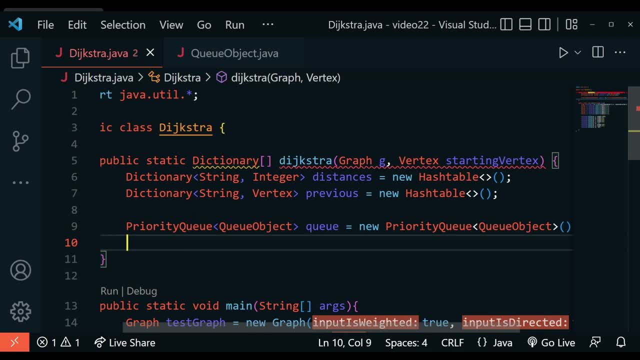 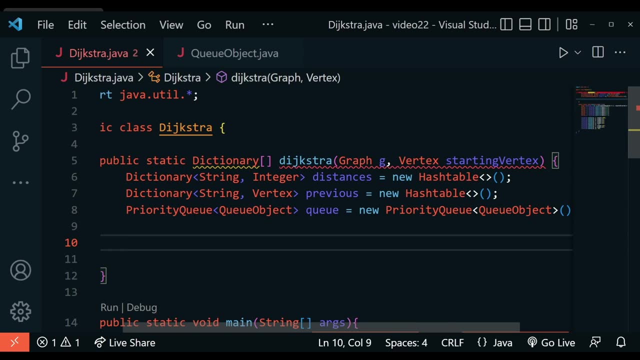 And then a semicolon at the end: Perfect. So this is our priority queue created, And let me just add in this Same exact line, So just after that. Now you might be asking: well, the priority queue is actually empty right now. 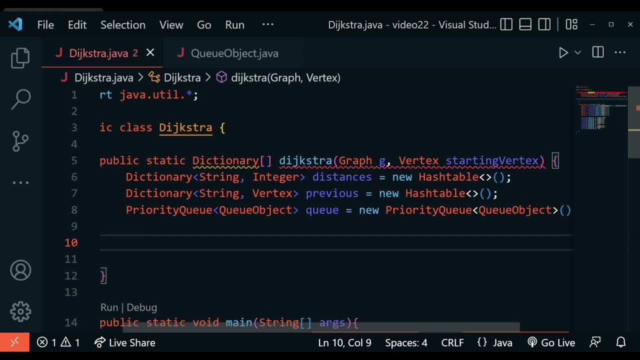 We've got to queue something inside Now. the thing that we're going to queue inside for the first thing is the starting vertex, since we know the distance for that is 0 to itself, So we're just going to queue that up in here. 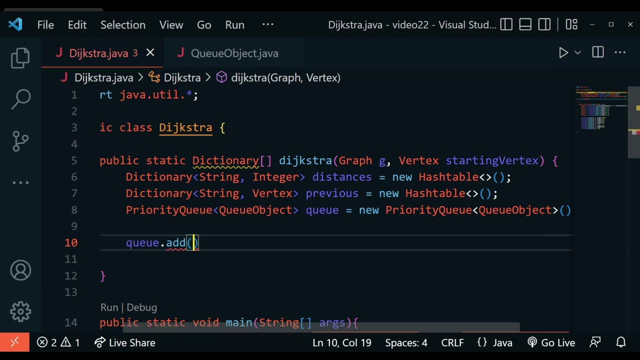 So we'll say Q-U-E-U-E dot add. And here we're just going to say new QObject And we're going to pass in The vertex V and the int P, which is the priority. The vertex V is just going to be the starting vertex. 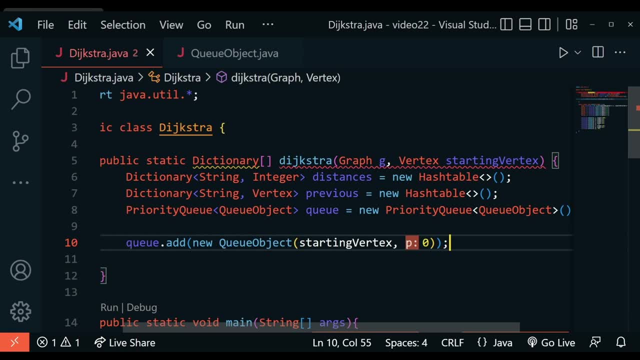 And the priority for this would be 0.. Awesome. Now we're going to try to iterate through this entire graph that was passed in as an input parameter, And we're going to try to iterate through and try to find all the vertices here. 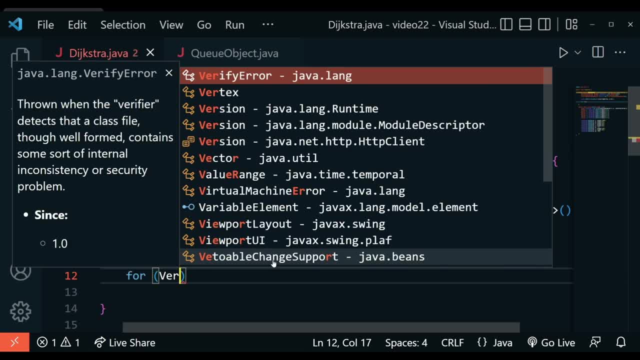 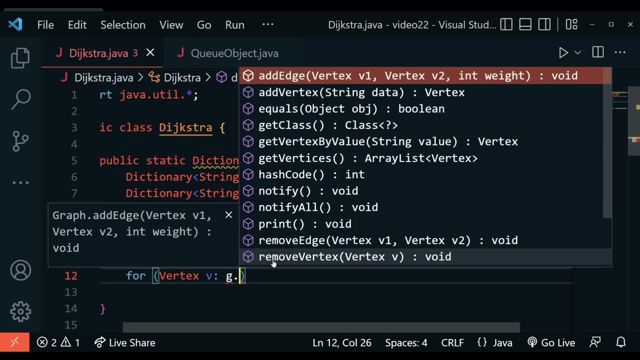 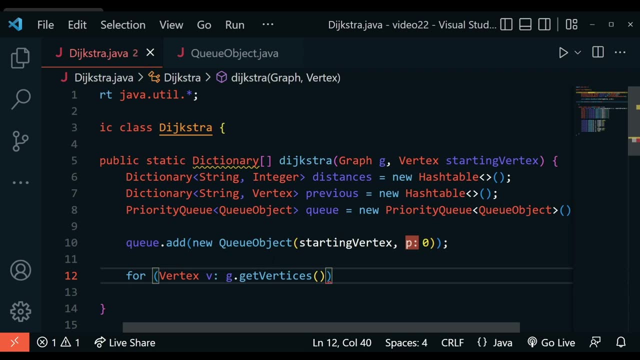 So we can use a for each loop for this purpose And we can say for every vertex V. And we can say for every vertex V in the G dot, get vertices. And this is returning an array list of vertex. And you're just doing this really easily. 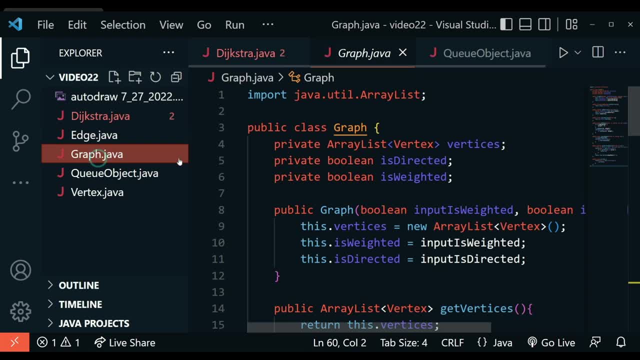 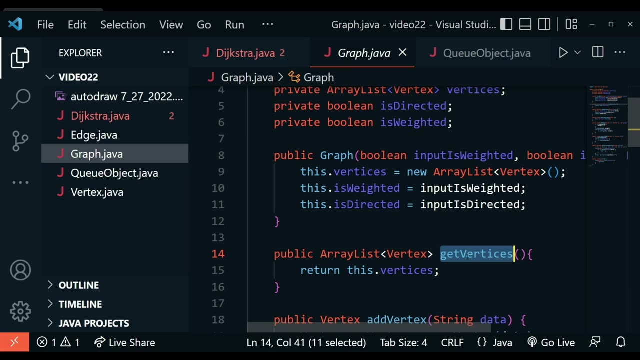 And this is also added here. So I have a graph dot Java file And this is also added. So that's why I'm able to get the method get vertices. So this is get vertices And it should be over here somewhere: Get vertices. 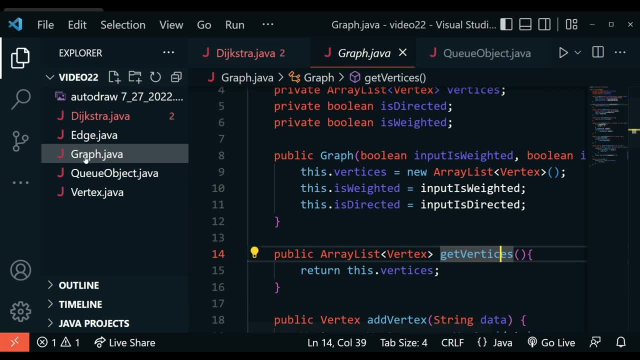 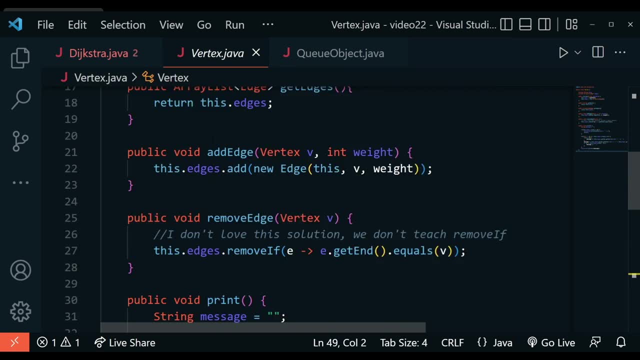 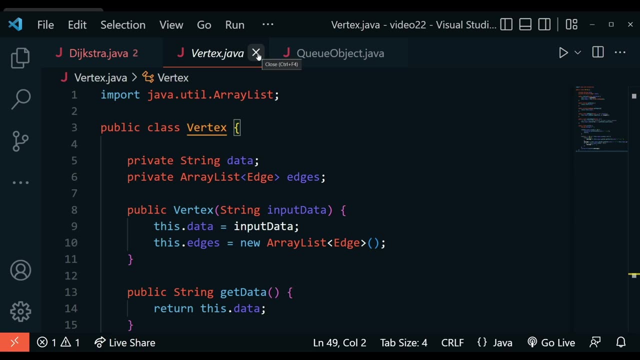 So this is the get vertices method, And I'm also adding this edge dot Java as well as this vertex dot Java. You could look at my older videos, And from there I'm actually using all of those classes that I've created in the graph dot Java, the vertex dot Java. 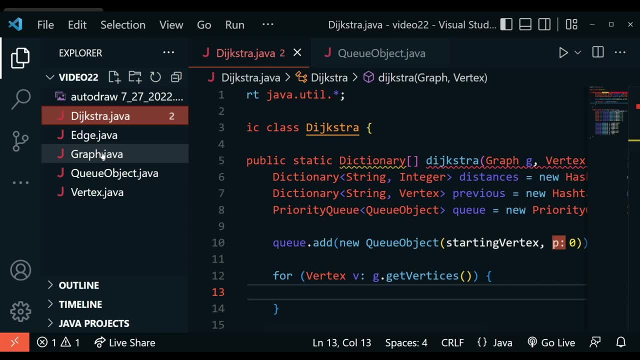 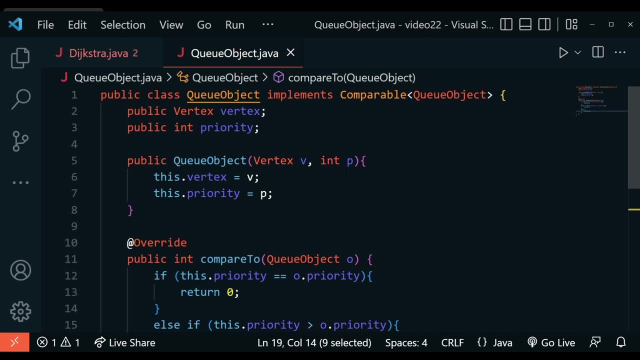 and the edge dot Java were all done in a single video, which was called graphs in Java. So watch that video. And for this Q object, I'm just going to let you see this code, So for now you can just pause the video and copy this. 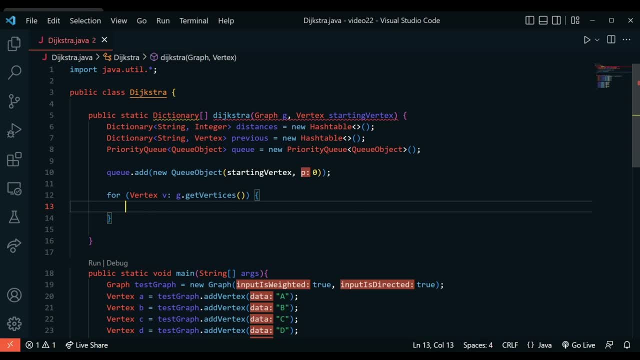 And once you have all of these, we could go back here in the Dexter's at Java And we're just going to iterate through the vertices which are in this graph which was passed in as an input parameter. Now we're going to have to iterate through this. 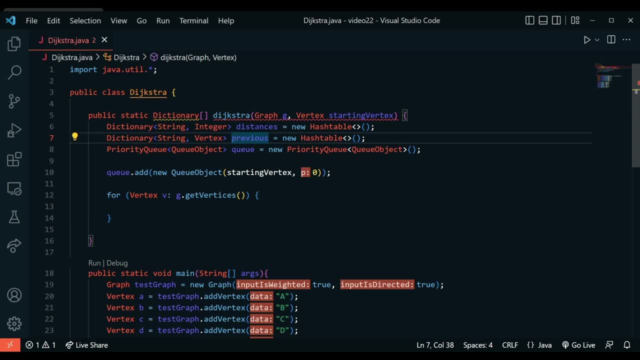 And we're going to actually update our distances, which was over here. So we're going to actually have to update our distances and previous dictionaries. So we're going to try to add all these vertices from this graph To this distances and previous dictionaries. we could do. 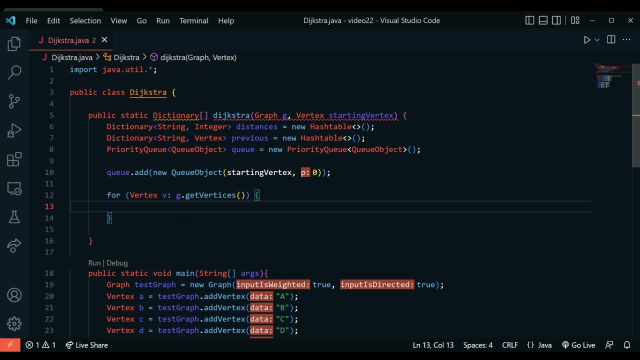 First of all, we don't want the starting vertex to have a maximum integer of max value, because we know that the starting vertex to itself is 0. So we're going to give a condition here and say if the vertex you get is the starting vertex. 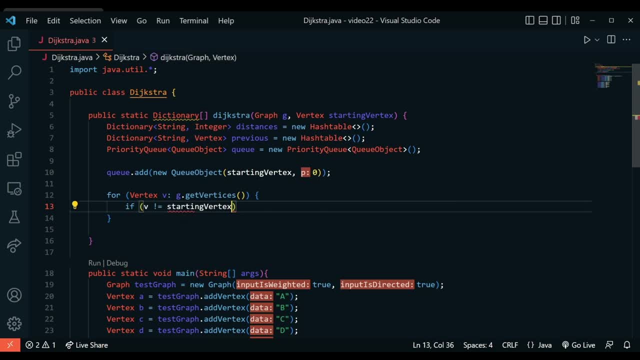 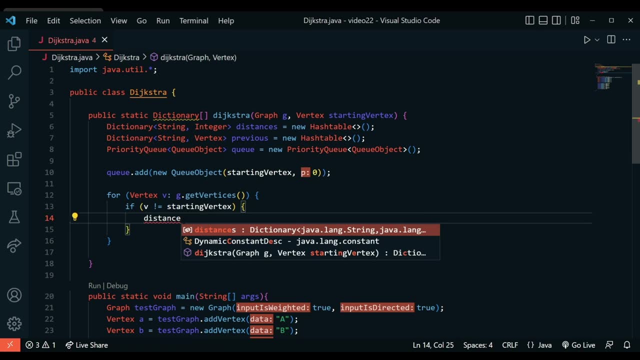 and this is just going to work. So we're going to say, if that one is the starting vertex, we don't want that. So if it's not right, So we want to update the distances and we're going to have to add input. 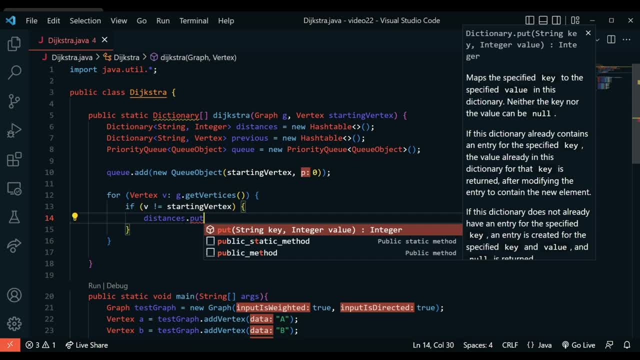 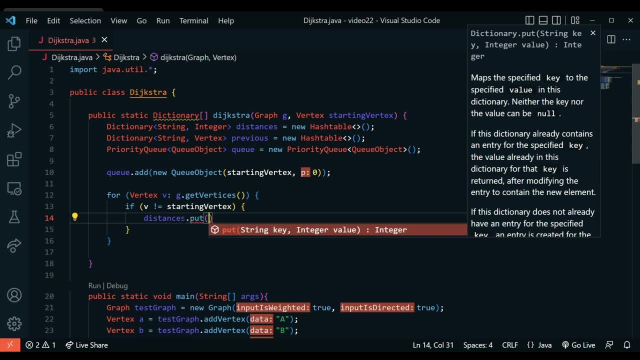 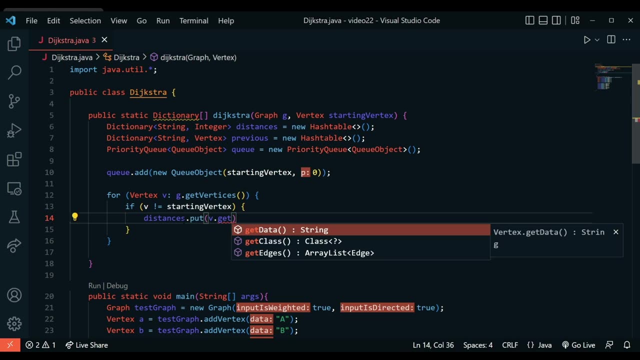 This is a method available in the dictionary And this allows us to add a key and value pair. So the string is the key and the value is the integer. So what we could do here is for the string we could say v, which is the vertex, and we say dot get. 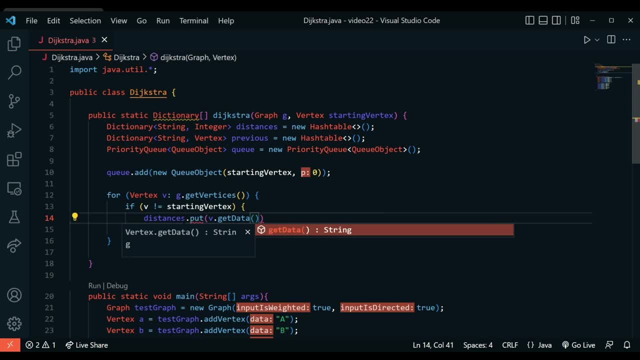 So we could say get data and that would return a string here, And this is also added in the vertexjava, So that's why it's working here. And for the integer we could just add in the maximum, Or we want to use the infinity symbol, right? 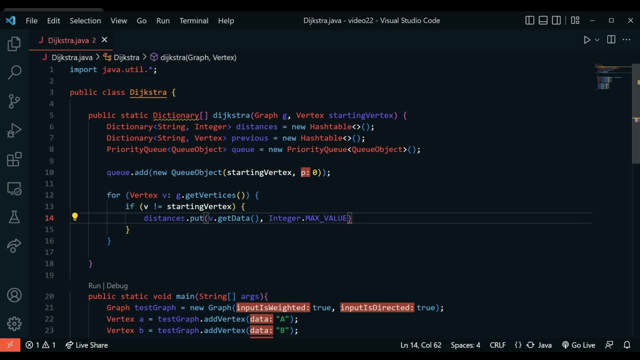 We could use integer dot max value. This would give us the maximum value for the integer in Java And that will be stored inside of the value pair. So key values are done. And for the other case where we have the previous dictionary: 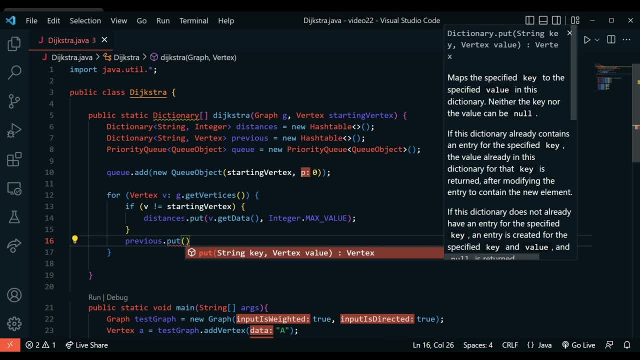 so we'll say previousput. And for this second dictionary we also have a key value pair, but the value is a vertex. So the key is going to be the get data. the same thing, But for the value in this case will be the previous vertex. 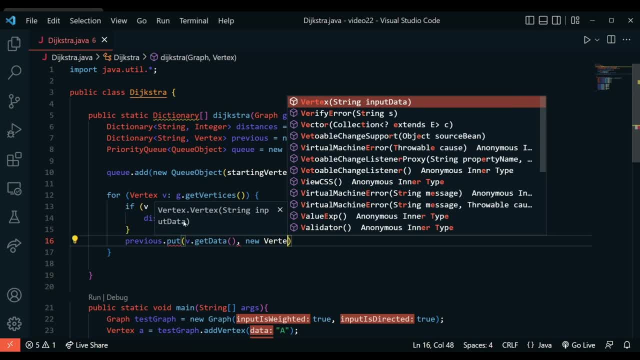 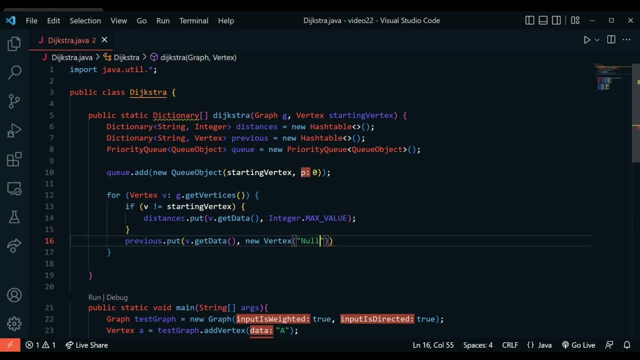 so that we could keep track of this. So we're just going to add in a vertex that will be set to null for now, And then after that we're going to update it inside of our code. So right now, just set everything to null. 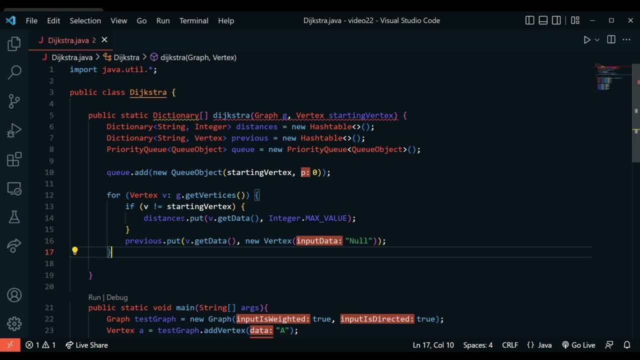 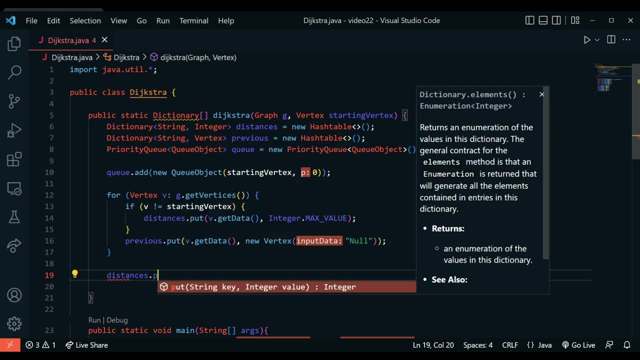 including the starting vertex, All right. so right after this, we needed to add in the starting vertex here in our distances, because we don't have it. So to do that, we'll just add in the distances again And we'll say put. 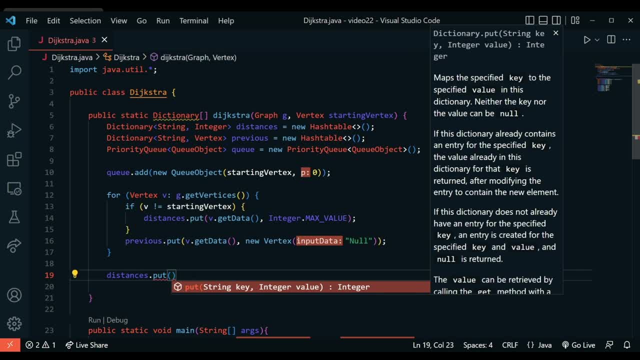 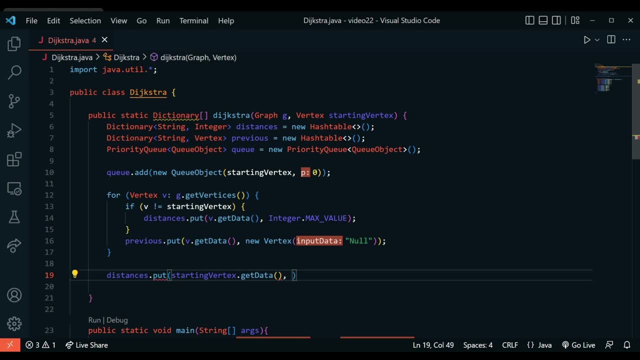 And now we want to add in the key value pair for that And for this, add in the starting vertex And we actually need the value for this And we can say get data And that will give us the string data. And for the value, I'm not going to give the maximum value. 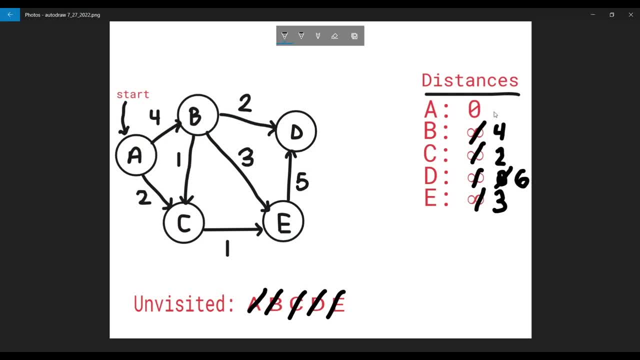 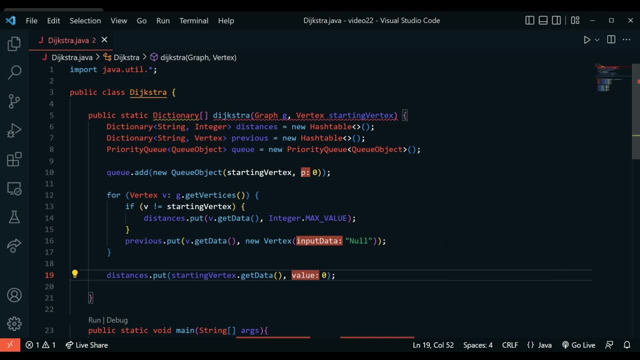 We're not going to give infinity, because if we look at this code over here, initially it was set to zero, So we want to just set it to zero here. I'll put it there And there you go. So we created this entire thing. what you can see over here. 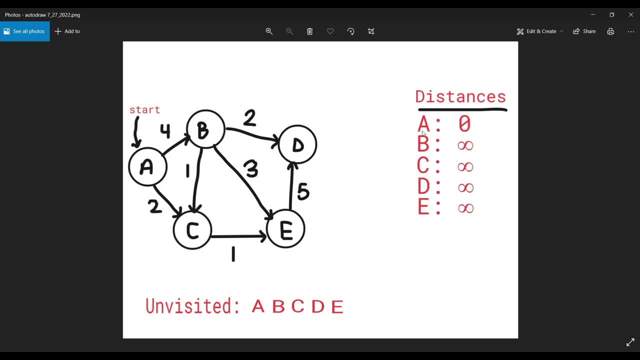 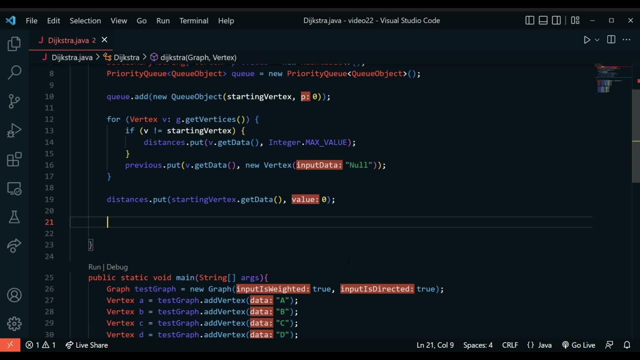 So you can see this entire thing that we've created, which has a set to zero And the rest are all set to the infinity or the max value. Now let's go back And we're going to actually do the second step for this algorithm. 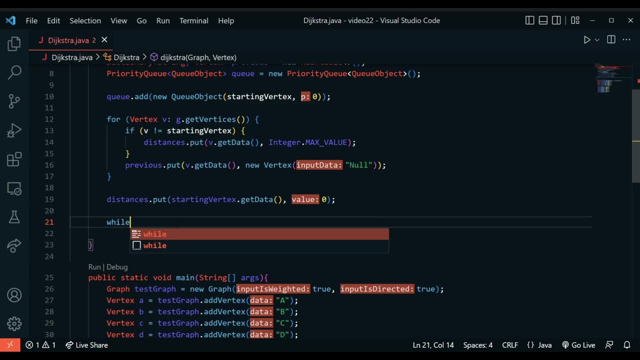 Now it's the fun part. We're going to have to iterate through the while loop And we're going to check if the queue is not empty. So we say queue e, u, e, This is our priority queue. And we say the size method here. 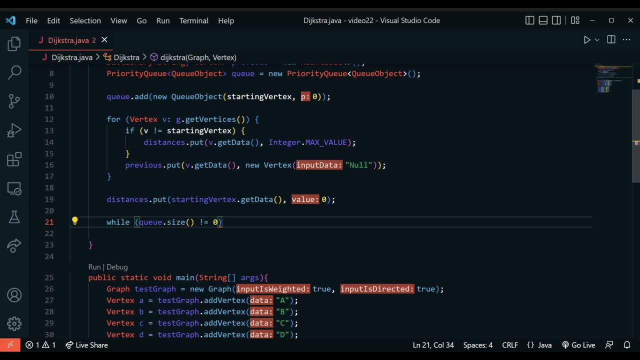 And if we say if that size is not equal to zero, we're going to do some operations inside of this queue. First of all, we're going to get the current vertex here And that is pretty simple. Queuepull retrieves and removes the head of this queue. 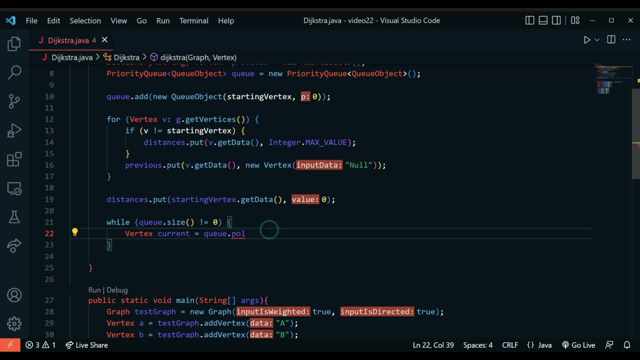 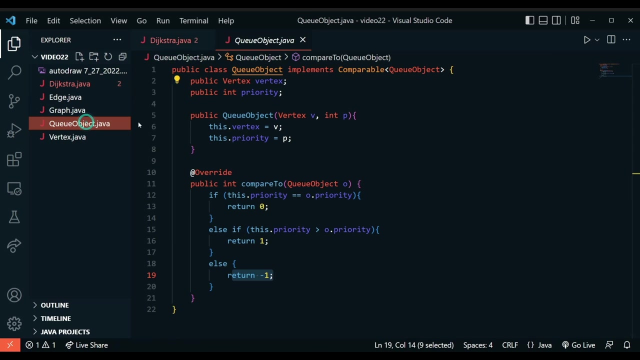 or returns null if this queue is empty. So we're going to actually Remove an item from the queue using this method And we want the vertex here. So we just say the vertex Because we had this over here as this queue object. 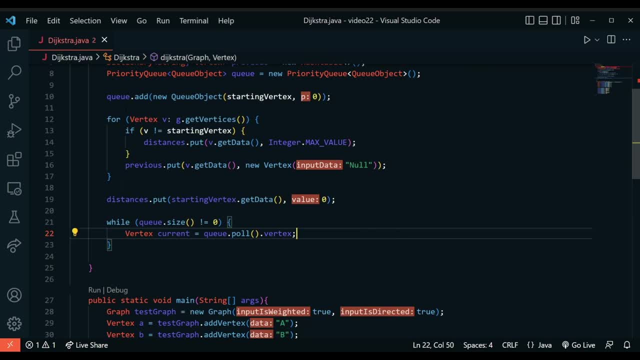 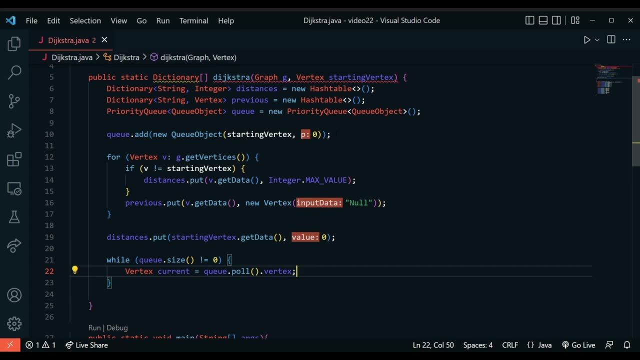 we wanted the vertex here, So we're removing that from the priority queue. So the first thing will just be the starting vertex, And that was added in our queue. So this was added over here. Queueadd new object: starting vertex with the value at zero. 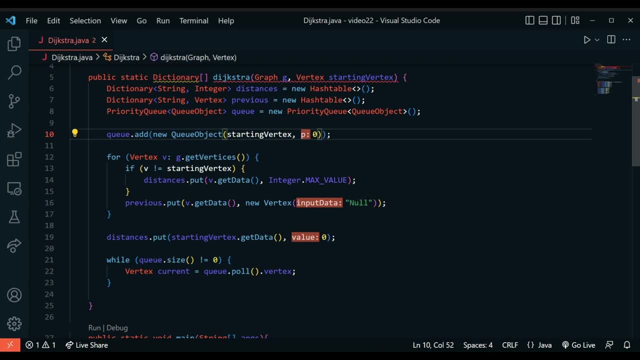 So zero was actually its value to itself. So this is now set to current And we removed it from the queue. Perfect. Now we're going to iterate through this current variable, which is the starting vertex. So we're going to look at all of the edges. 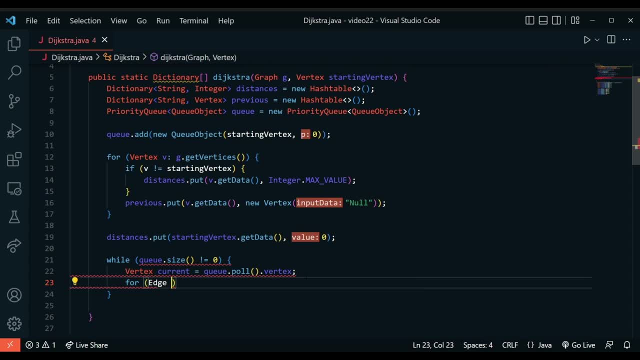 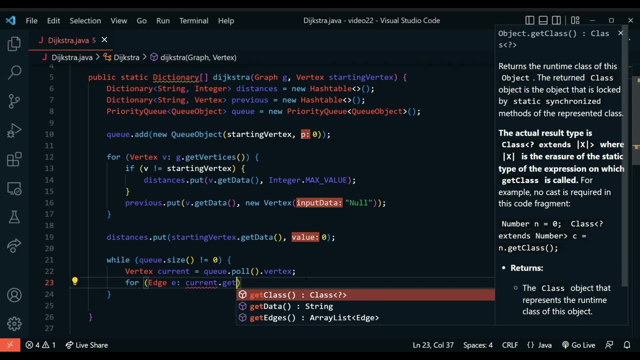 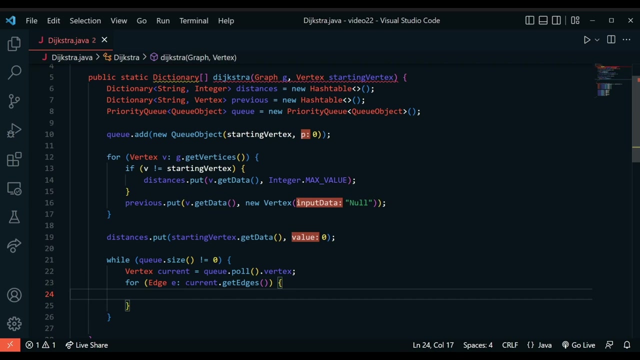 or the neighbors for here. So we say for every edge e and we say mapping out to the currentget edges, which is the array list returning. So for every edges or every neighbors inside of this current. so every edge. An edge contains vertices, remember. 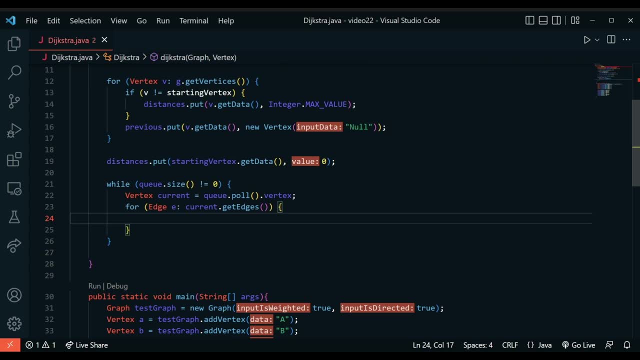 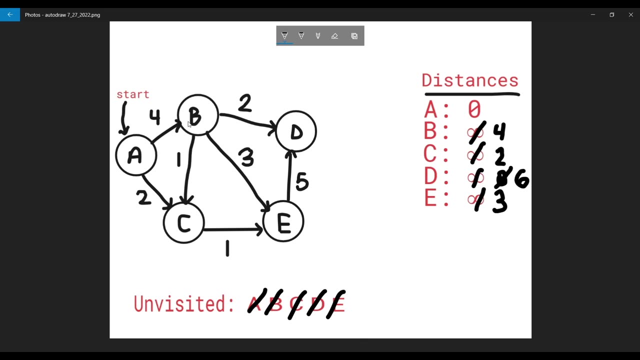 So we're actually going to first look at the value of what the edge is giving us. Remember, like I did in this first one, that we were looking at the values and we also judging inside of our distances. So we looked at, let's say, for the distance to d. 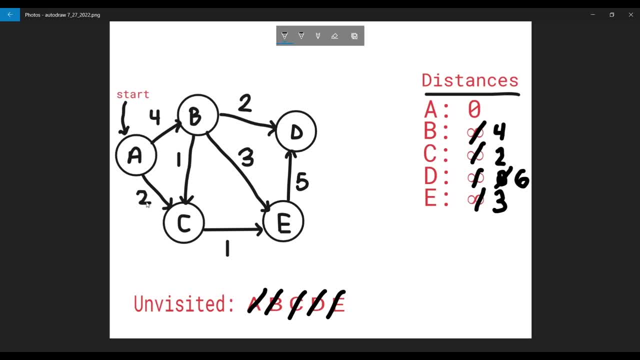 we had some already included. distance was 2, 1, 5,, which was 8.. So that was already passed in. But we also want to keep track of the newer one. So this is like 4, 2,, which is 6.. 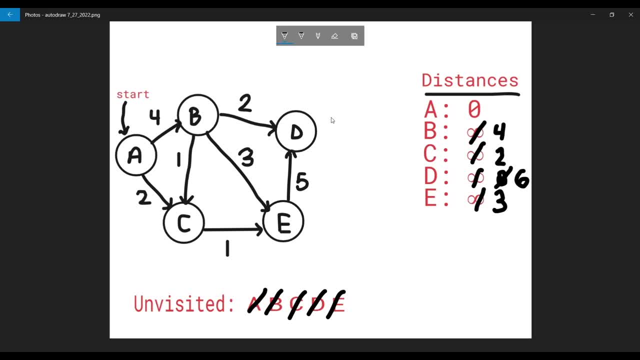 And now this is an alternative one. We have to add that somewhere And then we have to judge, something like if it's less than the original one, then we could replace it. So we want to have an alternative and we want to also have the original. 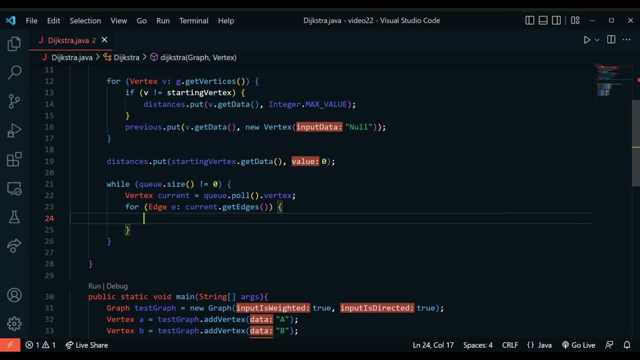 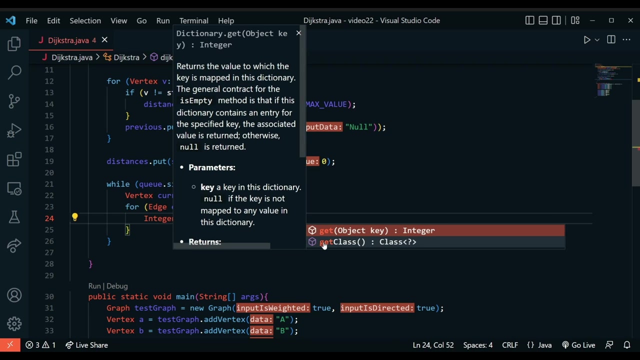 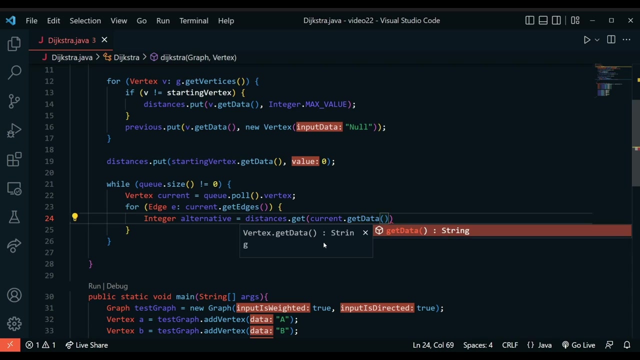 So for the alternative case, we'll add in an integer And I'll say alternative And I could add the distances here. So distances, And this is the distances dictionary And I'll get the currentgetdata And that is the string. 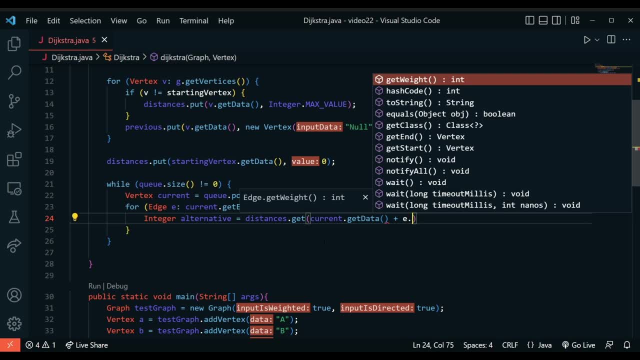 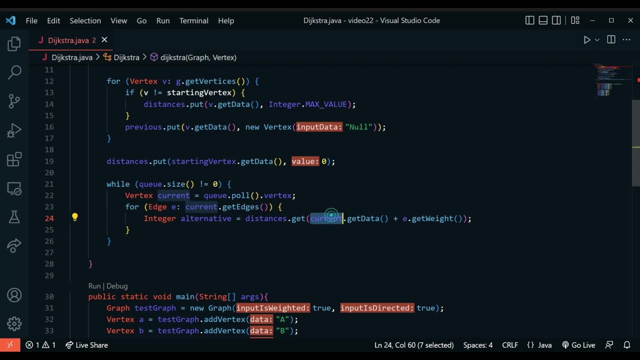 And we also want the plus to the egetweight, So we're going to get the weight as the int. So this is the distance from the current distance of the variable and the edge distance. So what this means is, whatever the distance is existing, 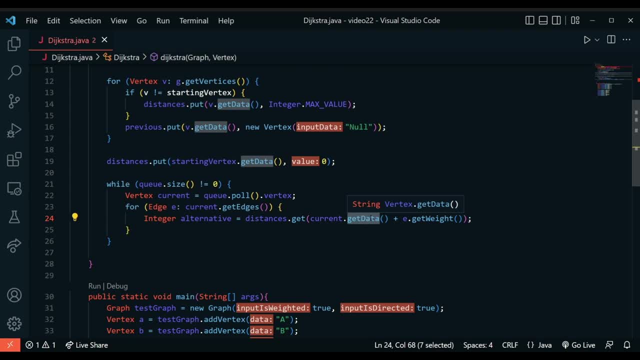 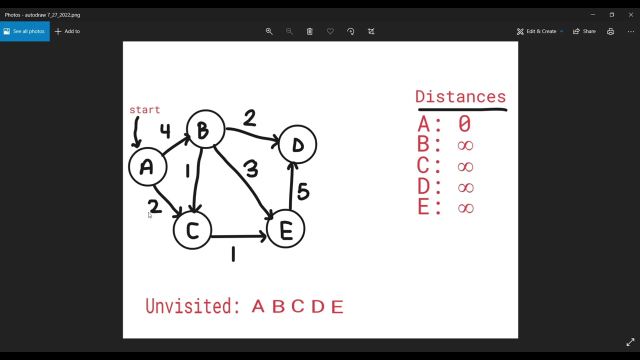 for this currentgetdata, the starting vertex is actually 0 to the distance where it's leading to with its vertex. So the edge where it's leading to with its edge. This makes sense because this is 0 to itself, But if we're moving forward we have an edge with it. 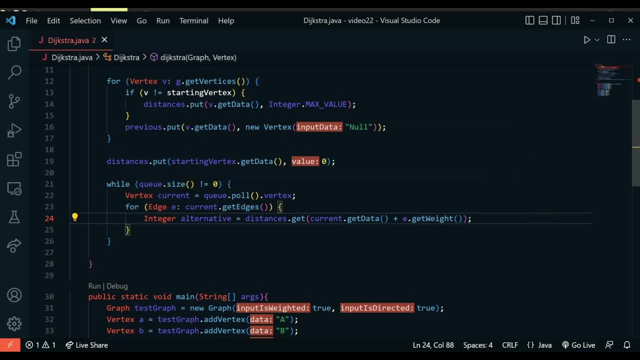 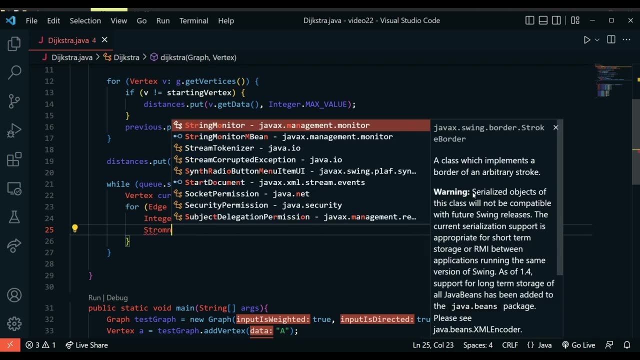 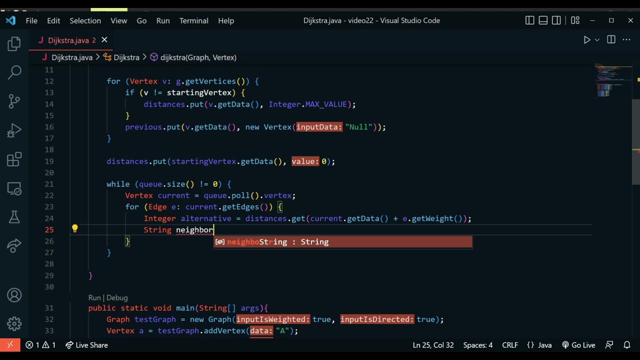 And we have some weight, So we're adding that weight as well. So get weight. So that's the alternative. And we also need a reference to our string neighbor variable So we could add that as neighbor. So this is our neighbor value. 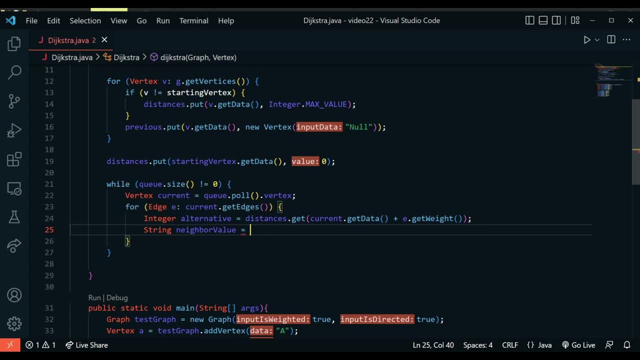 And we just have to keep it inside. So we could say egetend, So this is the end vertex And we want the value for this. So we have eend And we have get data. So over here it's pretty simple. 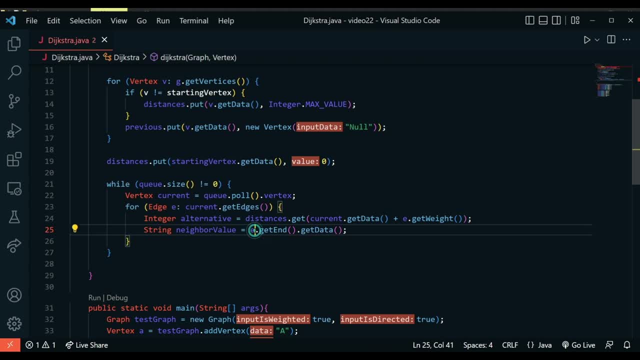 We have a neighbor value And we want to have the edge vertex, So we want to have the edge And we want to get the end, So we're going to get the vertex through this And to get the data. we just say this: 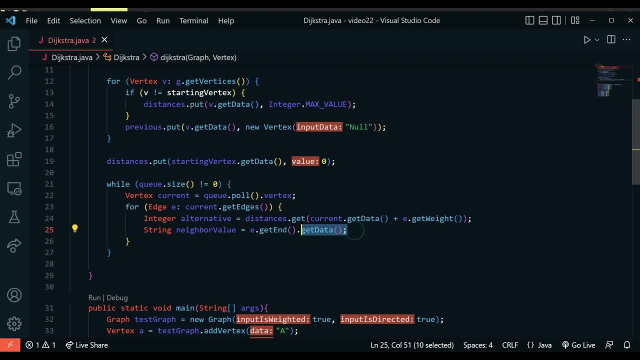 So we're going to get the vertex through this get end And we're going to get the data So that string is actually stored in the neighbor value. Now that the string is stored, we could use a conditional here To check if the alternative value is lesser than the original value. 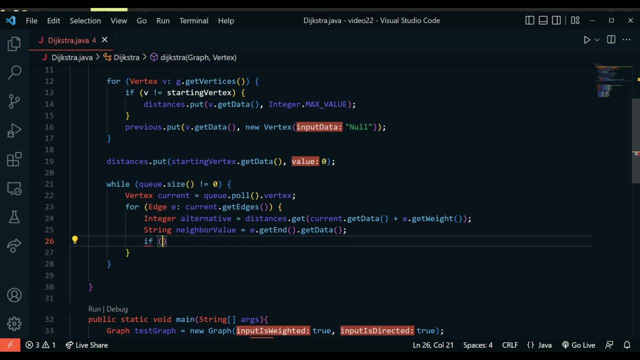 So what we could do here is pretty simple. We'll say: alternative is less than the distances And we want the dictionary. So this is the distancesget, And if we want to get the value for this, we could just use the neighbor value. 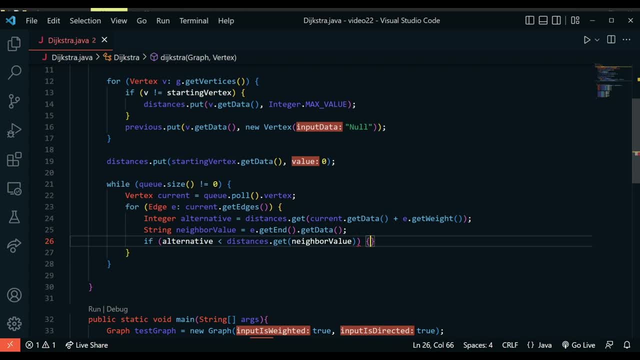 So that's why I stored it over there, So that we could get the value of our neighbor value. Alternative value is less than our neighbor value, So what we're going to do is That neighbor value is actually the original distance That was stored inside of our distances object, which is on top. 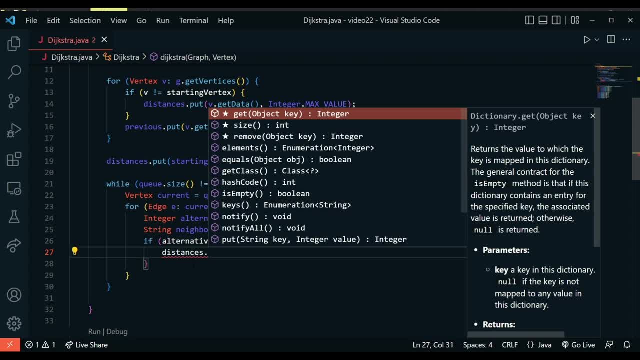 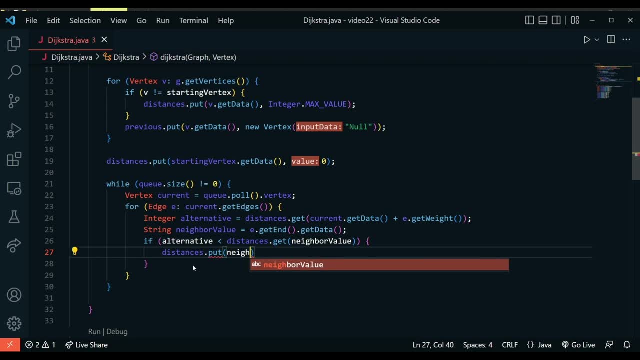 So over here we have distances. If that is possible, we're just trying to override it then. So we're going to say distancesput And we're going to get the neighbor value, So that exact neighbor value, But we're going to change the value to the alternative. 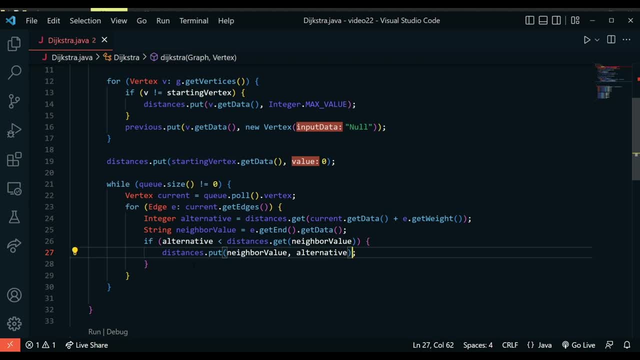 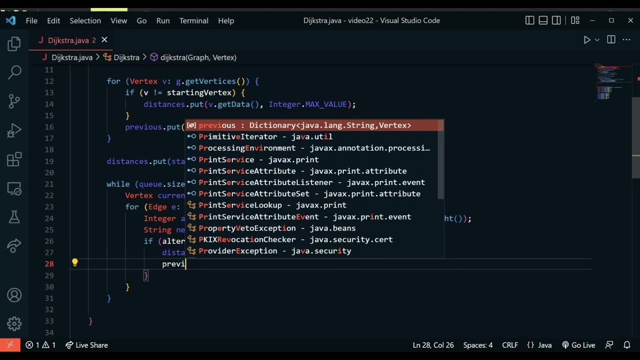 So we're going to get the key and the value. So this is the string neighbor value, And then the integer will be now the alternative Distance. also, we're going to have to modify our previous, So we're going to have to add in the neighbor value as well. 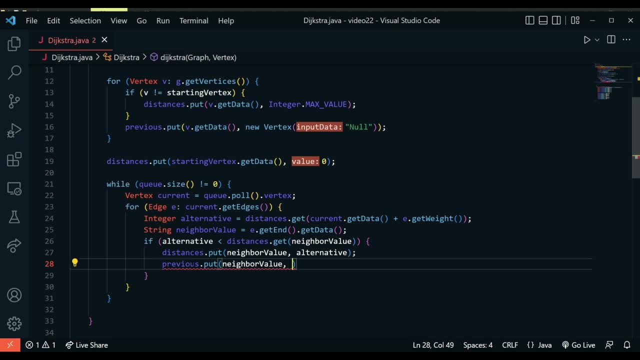 So for the neighbor value we actually need the previous reference, And the previous reference will now be for our current instance, But the current one, which is now which is actually starting vertex, will be the previous vertex for our neighbor value, which is the current one over here. 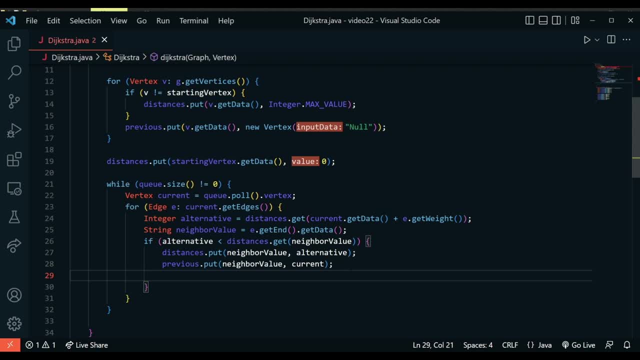 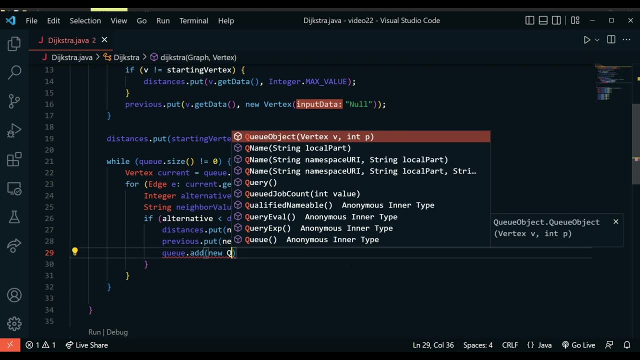 So it's just going to keep iterating this and updating our previous Reference, And the last thing what we want to do is we want to add the neighboring value to our Q U, Q U, E, U E object And we have to add in the vertex here: 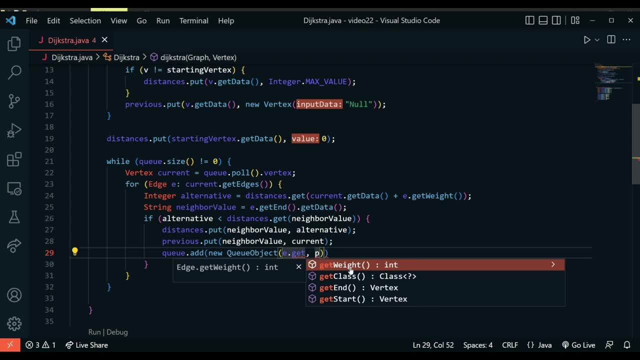 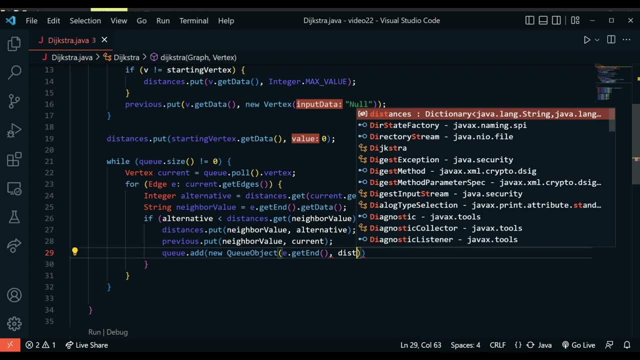 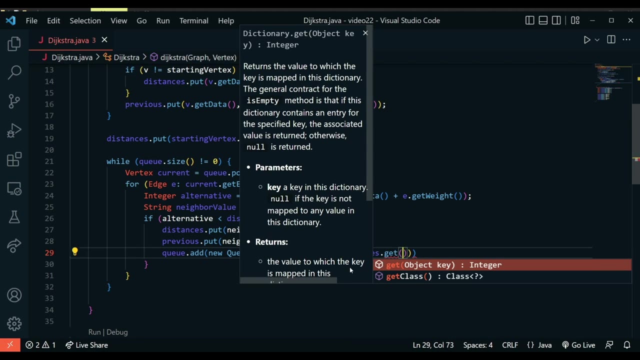 So we're going to say E dot get end. So that's going to give us the vertex here And to get the priority we could say the distances structure dot get, And to get the value I'm just going to add in neighbor value. 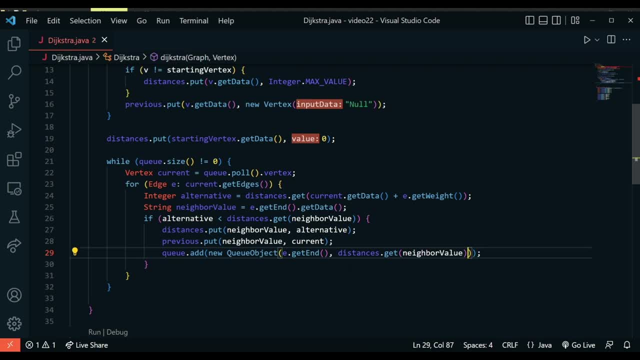 And that will give us the value. So this is neighbor value is the key And it will give us the value which is associated to this key And that will be updated to our Q And that's going to be our priority, So that will be added. 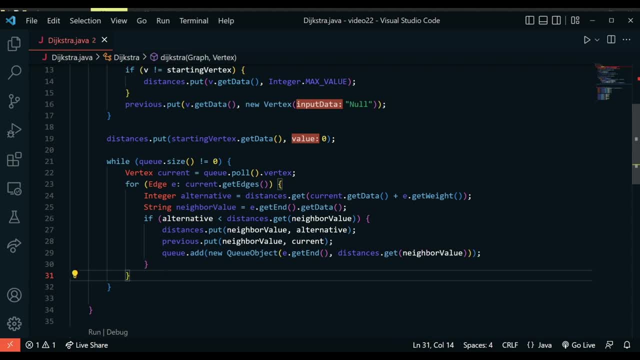 And once it's done, we're actually going to break out from this for loop when all of these edges are done And that will be updated, And after that until the wild size is not less than zero. So this is just the line that we'll. 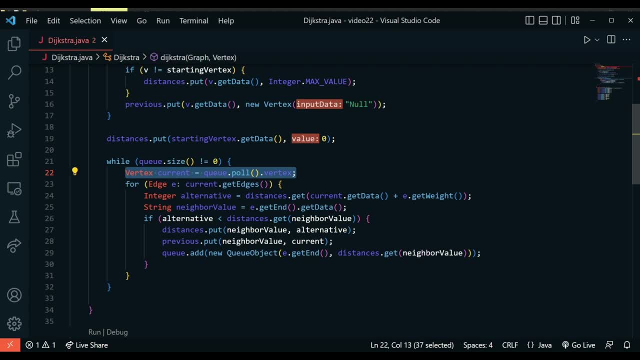 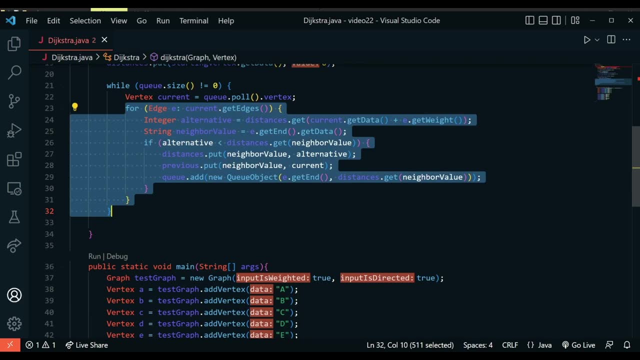 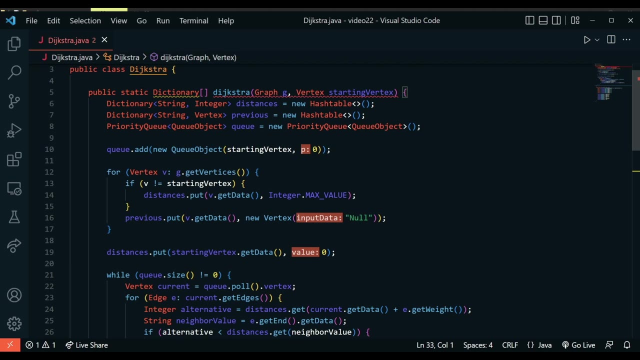 pop off the minimum distance of the unvisited vertex And the rest is history over here. What you saw all in the conceptual overview. everything is happening and adjusting, And right at the end. so when the while loop breaks. so the Dijkstra is requiring us to return a dictionary array right? 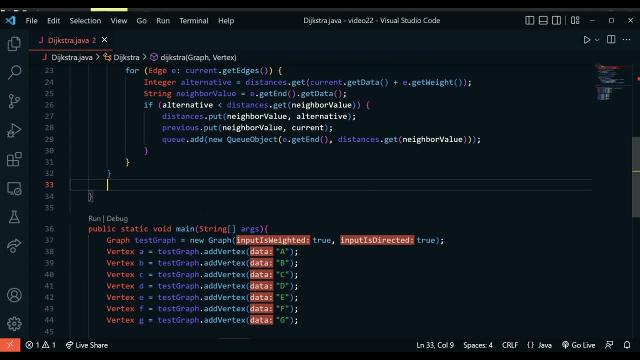 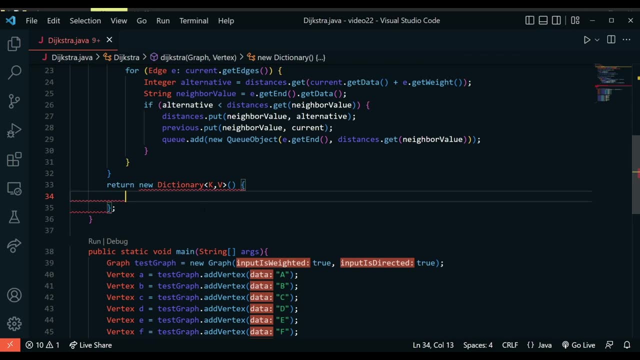 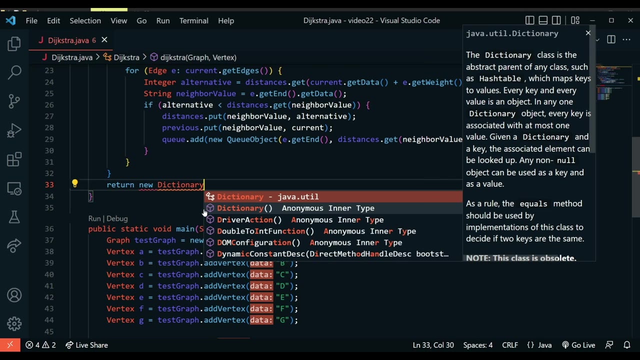 So we want to return that. So over here, right after the while loop, we could return a new dictionary And oh, so over here we're going to return a new D-I-C-T-I-O-N-A-R-Y And we're going to get this bracket over here. 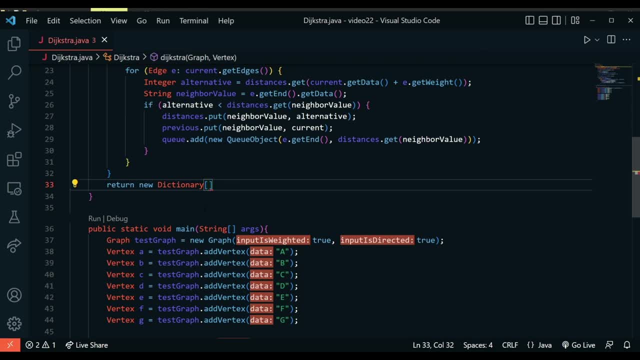 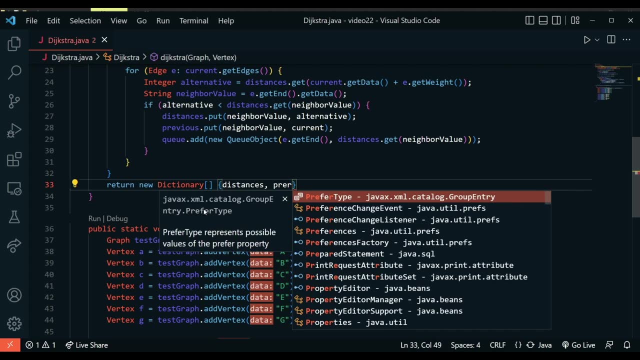 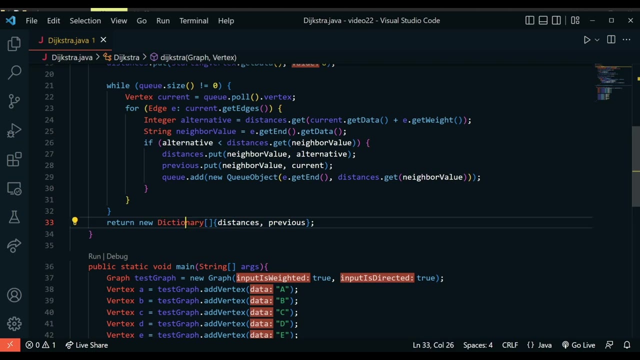 which is the array for this dictionary. And this is the array of the dictionary And we want to pass in the distances- distances with the previous structure here. This is the return statement. We're going to return a new dictionary And it will have the distances and the previous dictionaries. 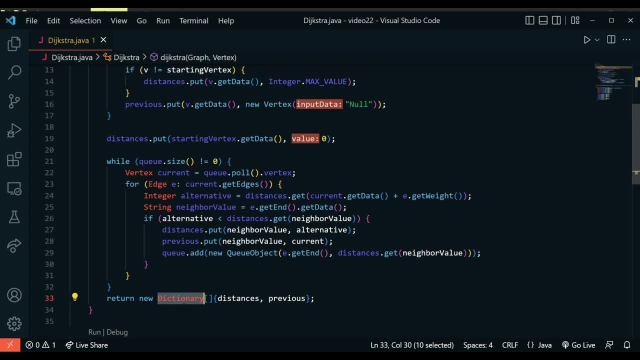 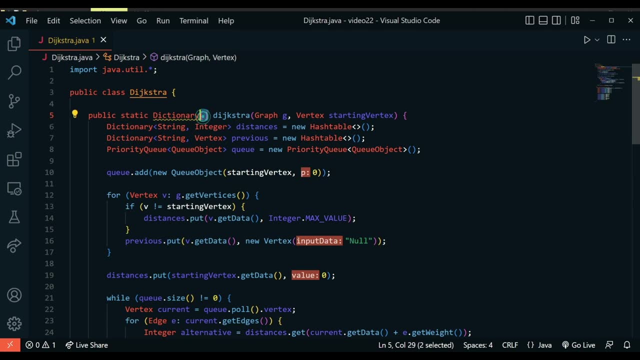 So we'll have both the distances and previous dictionaries inside of this dictionary array which is returning here in our function, So we can hear that dictionary array is returning. So this is the return statement at the end. And yeah, so that was pretty much it with this function. 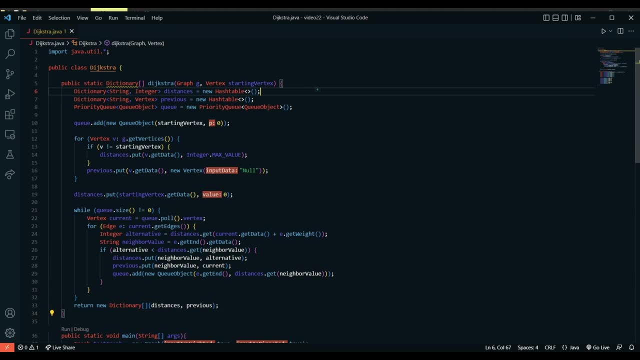 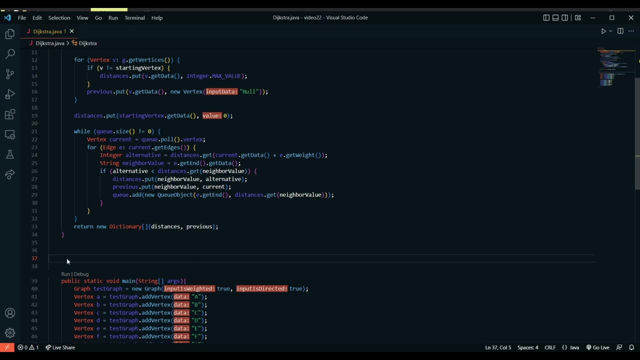 This is minimizing it so that you can see the entire thing. So this is the entire method for Dijkstra. Now we also have this helper method on this bottom, So I'm just going to paste this in. This is called the Dijkstra result printer method. 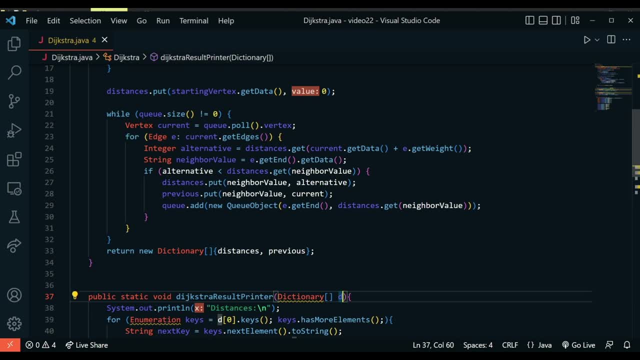 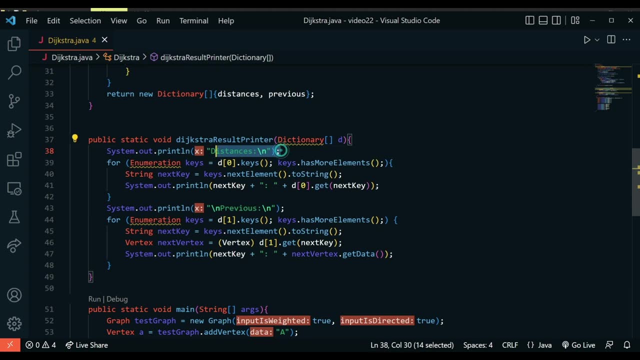 And what it accepts is an array of dictionaries. Wow, how convenient. We're just going to use this entire thing And it's just going to return it, And so we can pass it inside of this, And this will just actually print all the distances. 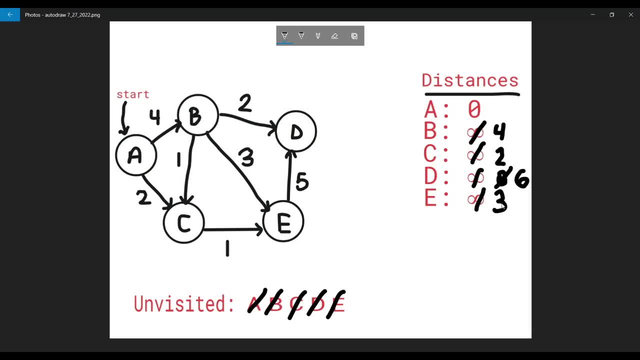 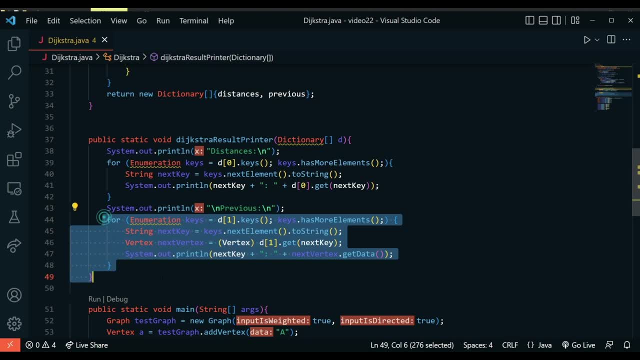 So what you can see over here. So it's going to print out the updated distances like this, And it's also going to print out the previous positions, So you're going to see that as well. So these both were dictionaries. We're going to use integration as keys to get the values of all of this. 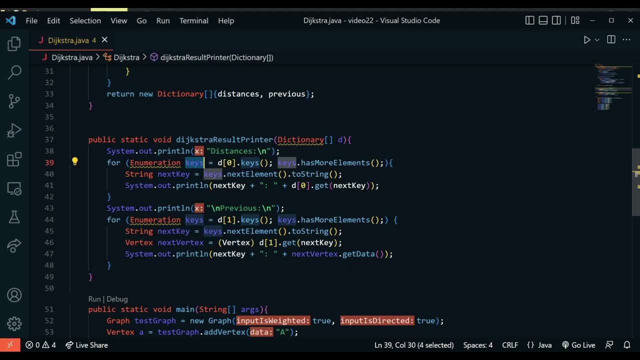 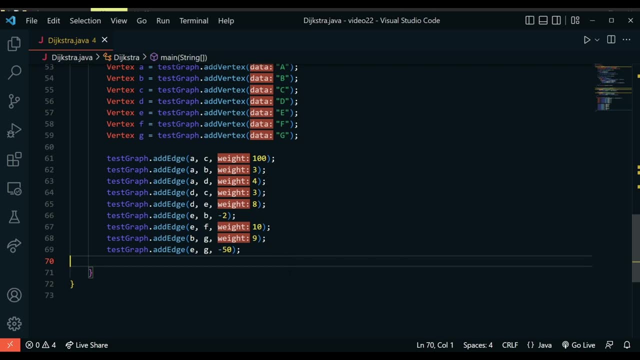 And it's just going to give us the key and value pairs And it's going to be pretty cool. So these both are going to be allowing us to print these structures, So we're going to add this process here, So let's just create this call. 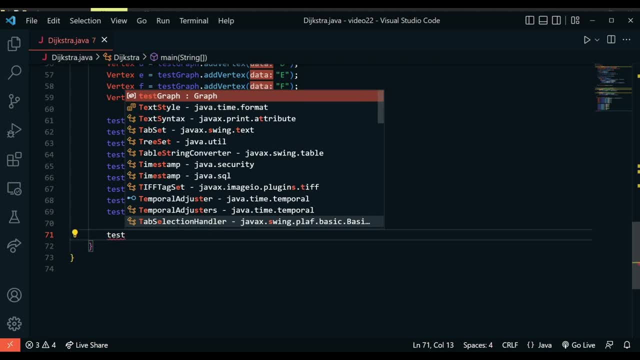 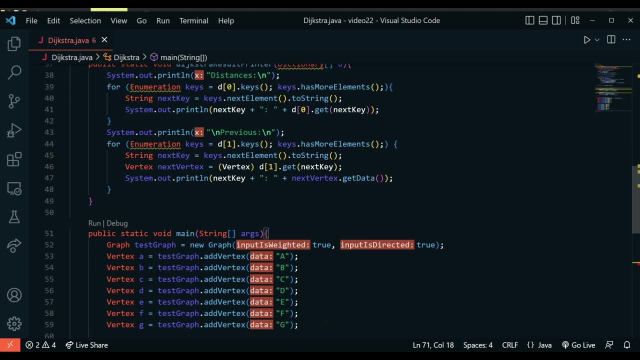 So we had this test graph And what we want to do is we want to use this method here, which is Dijkstra. So to use this, we have to pass that inside. So we're going to use Dijkstra here And we're going to pass in the test graph. 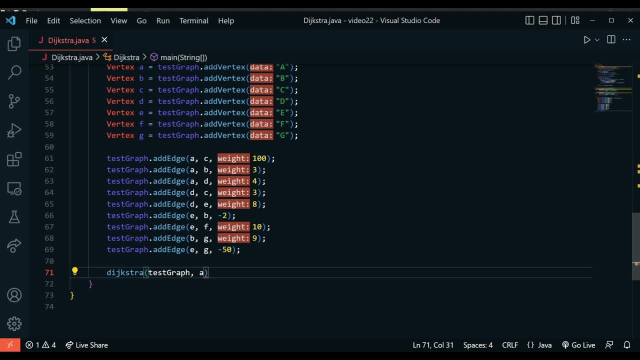 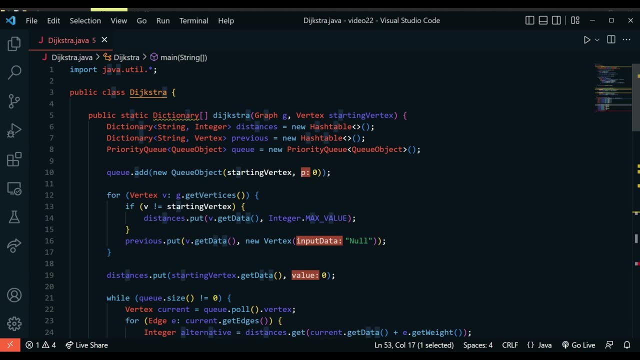 Also going to pass in the starting vertex, And that is A, because over here is the first vertex And that's going to be our starting vertex. You can set anything you want later on And then after that we're actually calling this inside of this method. 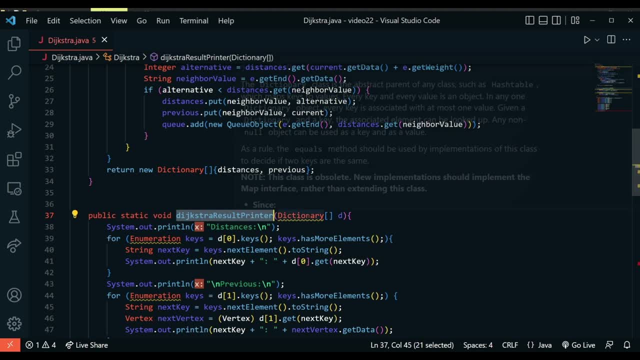 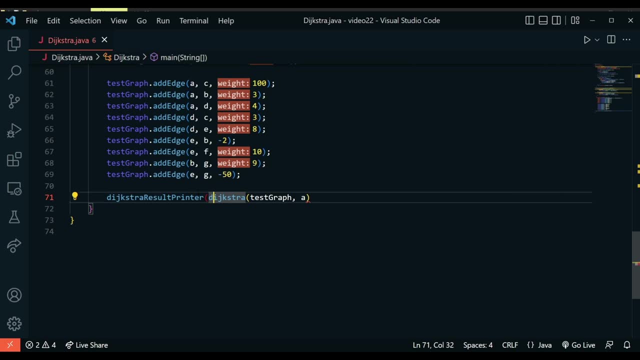 which is Dijkstra result printer, since it's accepting a dictionary array of D. So I'm going to paste this thing inside And we're going to wrap it around the Dijkstra. So there you go, And this will just print out the things. 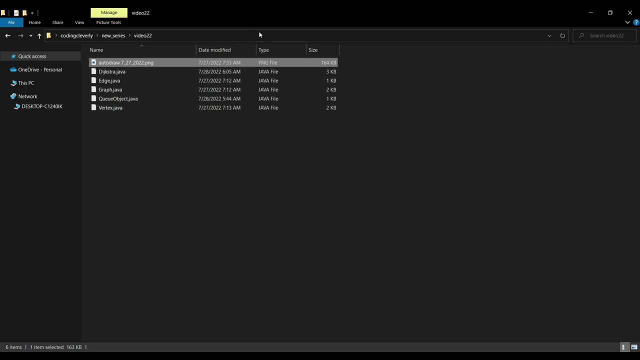 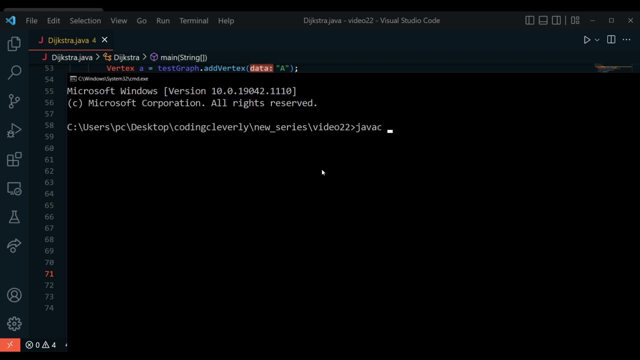 So cool. So now let's run this code. So let's go and add in CMD here And let's run this code So javacdijkstrajava, And then let's just run it using javakdijkstrajava, All right. 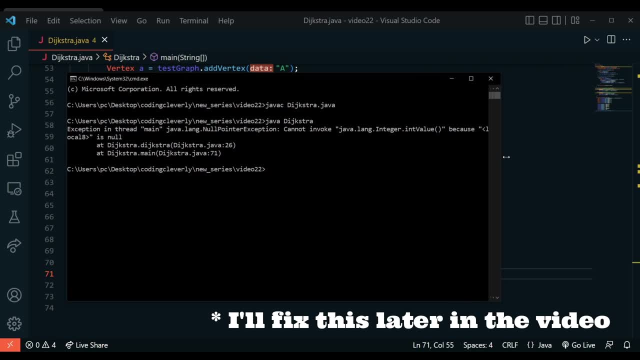 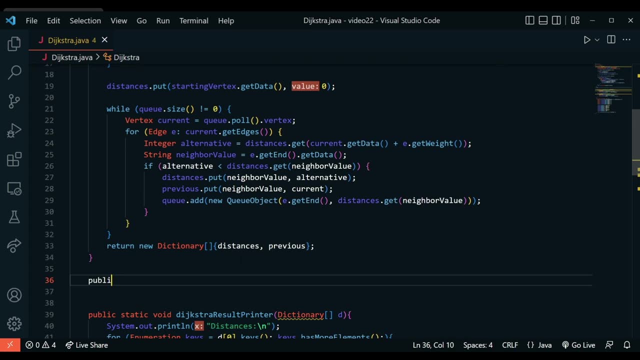 So we have an error here, something null pointer exception. OK, We want the shortest path between two vertices To calculate that. we'll just create a new method here And we'll call this as public static void And we'll call this as shortest path between. 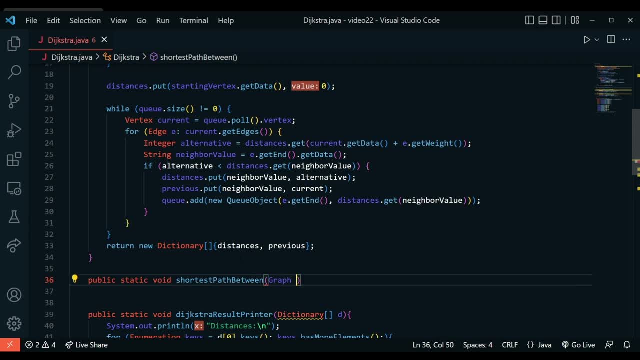 Inside here we'll have a graph DRAPH And we'll call it as graph G. We're also going to have the vertex And we're going to get the starting vertex And we also need the targeted vertex. So we're going to say target vertex here. 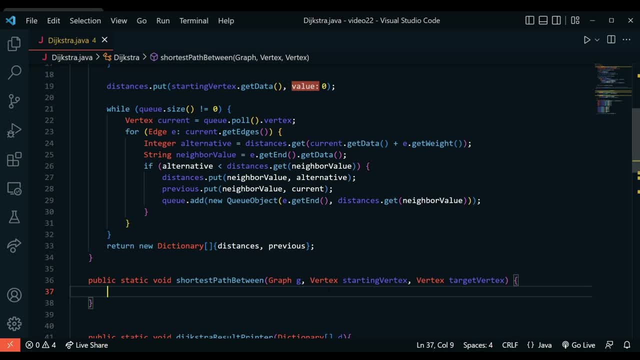 We have the shortest path between method in which we're going to input the graph, the starting vertex and the targeted vertex, Because we want the minimum distance between two vertices, so we're going to use this method. for that case, We're going to have the dictionary. 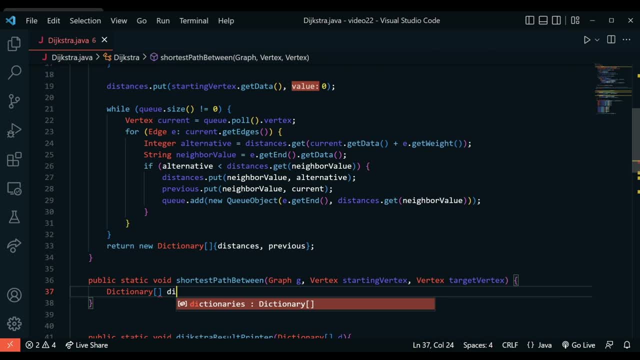 And we're going to call this array object here And we're going to call this as Dijkstra's dictionaries And that will be equal to the dictionaries. So we're going to call the Dijkstra method here. We're going to call it using the graph and the starting vertex. 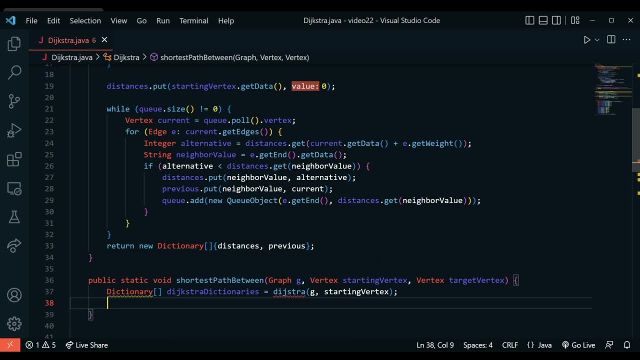 What actually it gives us is the distances and the previous dictionaries, And I'm getting an error here. It's actually DIJ. The method Dijkstra is undefined for the type Dijkstra, So the reason why I'm getting an error here is because I don't have a K. 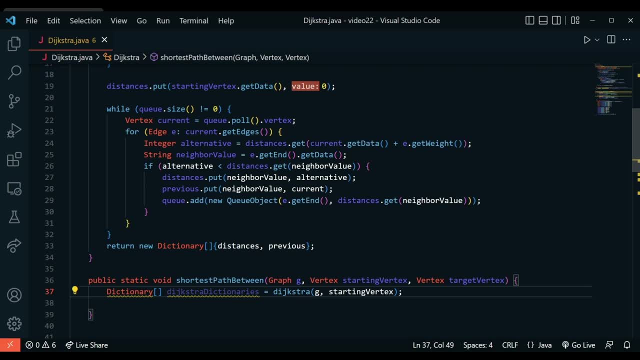 So DIJ K, And if I do that I'm all set. Now we want to put the distances and previous in their own variables, So we're going to have the scope for that. So I'm going to say distances dictionary. 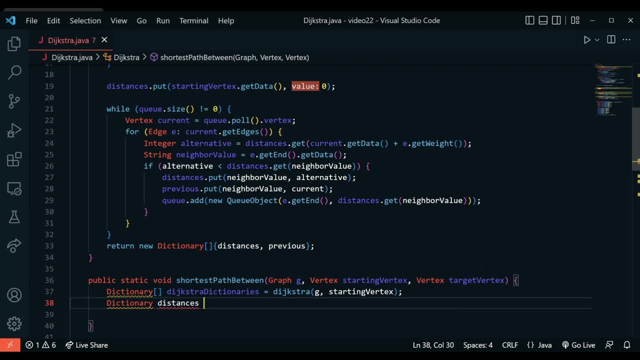 And it will contain all of the values which we had. And then we're going to manipulate this. So we're going to say dictionaries, So Dijkstra, DIJ K STRA, And we have Dijkstra dictionaries And we have this sub 0.. 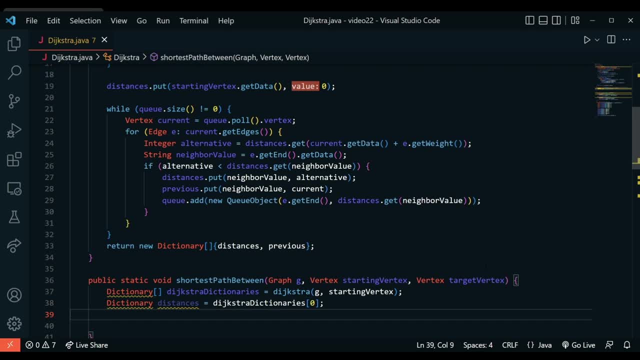 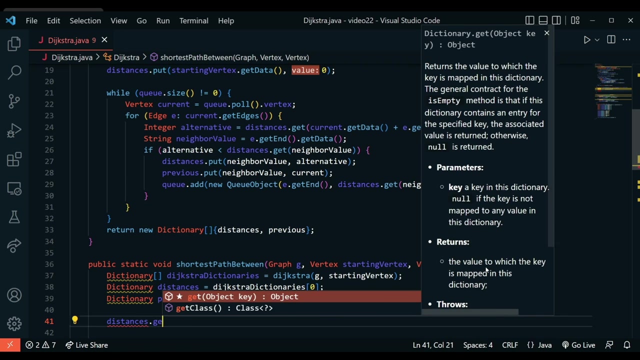 That will contain our distances, And for the second one, and for the second one we could have that as 1.. And that will be our previous Awesome. To get the distance of our target vertex, we could say distances dot get. 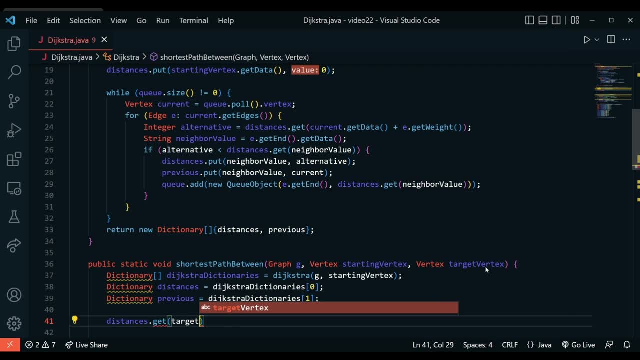 And we need to get the target vertex And we want the value for that. We could say: get data That will return a string And that will actually map us the value from our distances, which will be something like you know the value, what it will take for us. 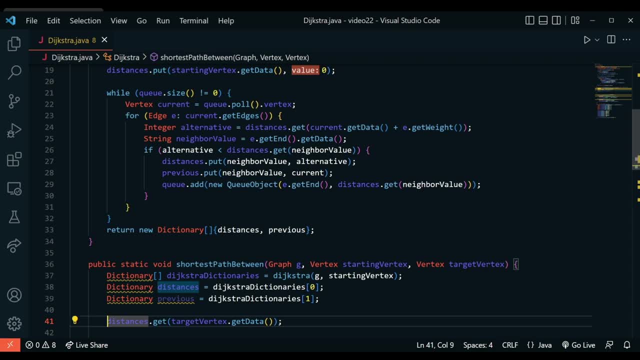 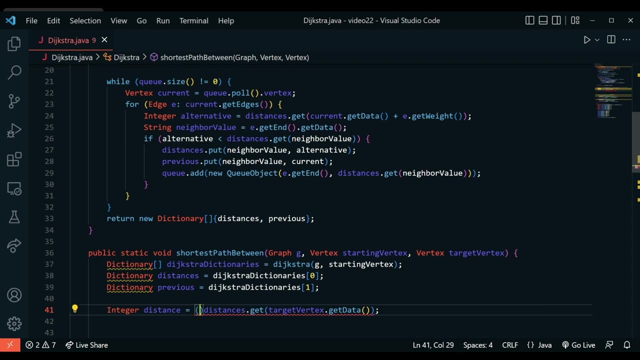 to reach from A to that point And that we could store in some variable called distance. So make sure you have the type set to integer here, And then that should go away. Now what we want to do here is we want a print screen. 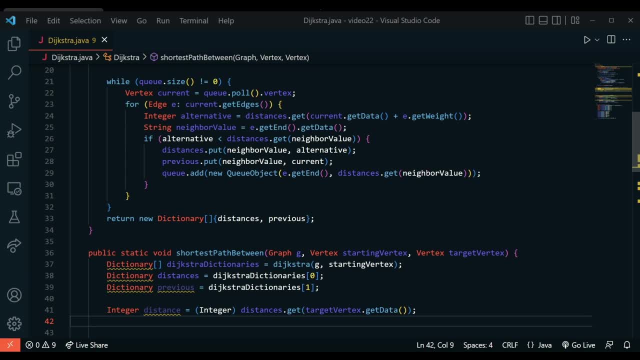 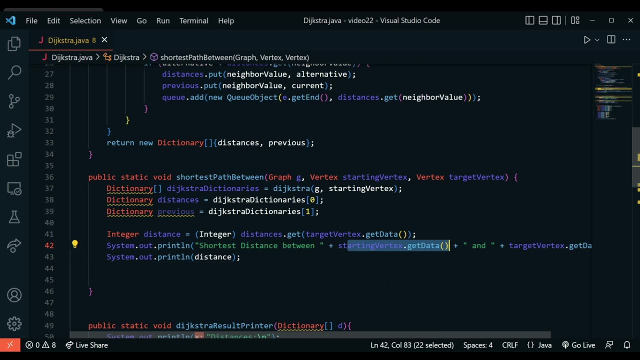 that will just show us the shortest distance path between those two. So what we could do is we could paste this in And this is just going to print out the shortest distance between the starting vertex get data and the target vertex dot get data. So just between the two vertex. 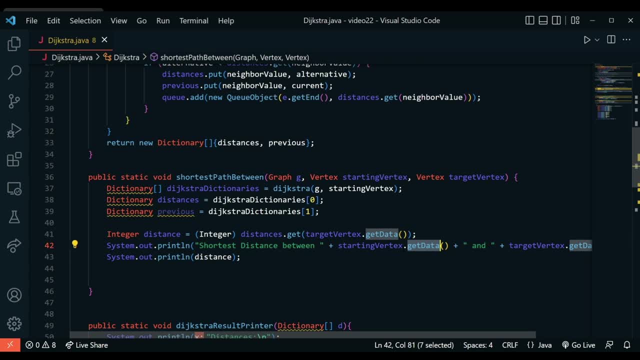 this is just going to give us the letters, you know the distance between A to whatever, And systemoutprintln will just print us the distance which was inside of the target vertex. Now we actually need the, the generated path that we should follow. 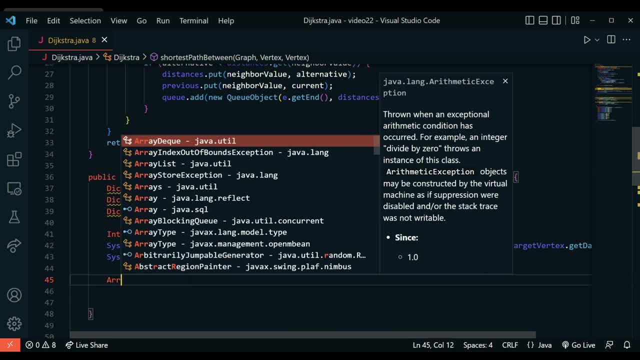 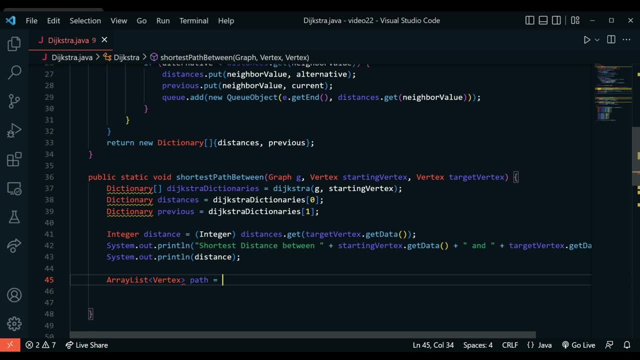 To create the path. we're going to create an array list for us And that would be a type vertex And we could call that as path. We initialized an array list to get the target vertex and assign it to a variable is very important here. 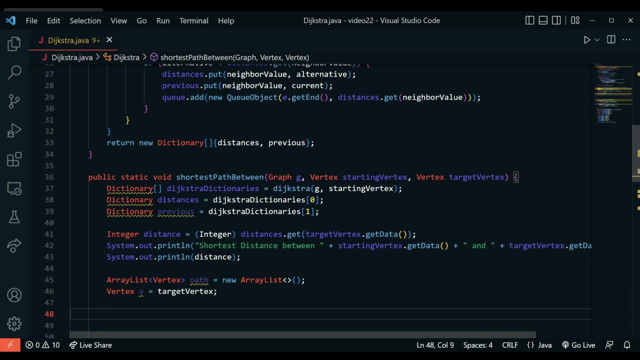 So we're going to have target vertex and assign it to a variable. So if we go from the target vertex to the starting vertex, it's a bit like the reverse link list. So we're going to use some kind of functionality like that. 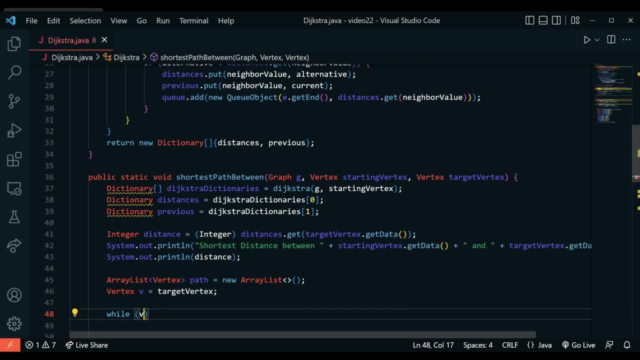 We're going to use a while loop and we say: while the V the vertex. So if the V is data and the get data will pass in a string and say if that is not null, because we know that the first one, which is the start will, is null. 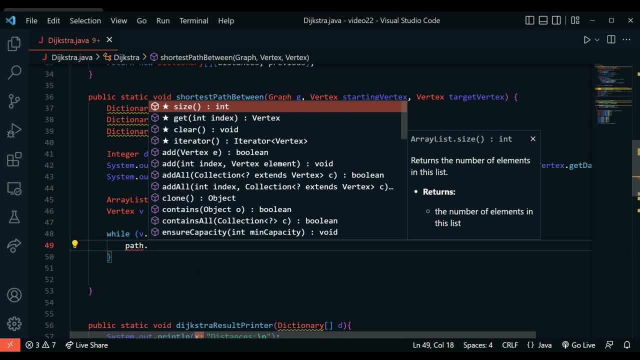 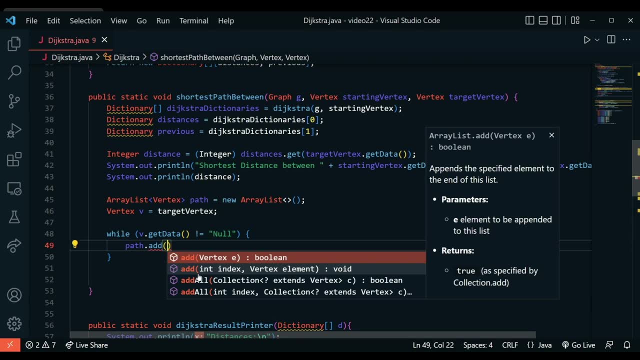 We're going to add the path, So the path is actually the array list. We're going to say the path dot add. We're going to add a zero here because the path is actually making us add something inside of this, So we're going to add in a zero. 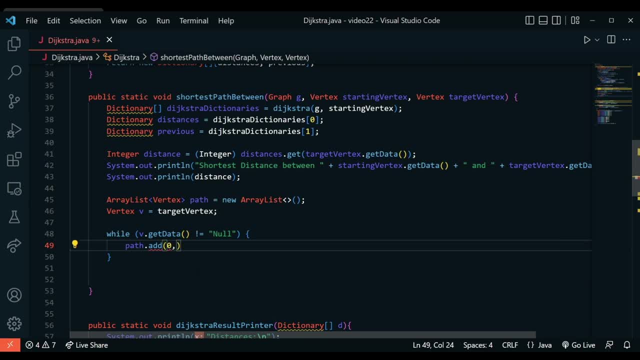 And this would mean that it will be popped in the forward direction. It's not going to go backwards, It's not going to queue there, But every time a new value exists, it will come in the beginning, Every time a new value is added. 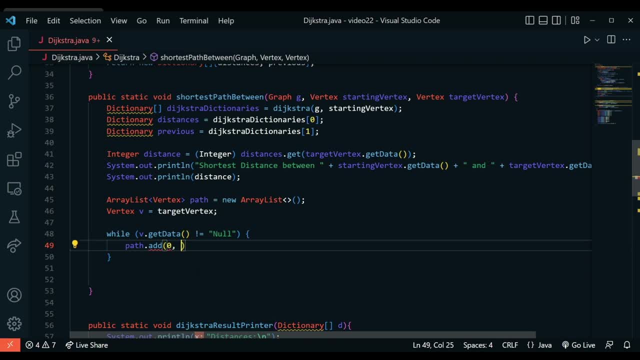 to this array list. it will be added in the beginning, So path dot add zero will be added. That value will be added to the beginning of the queue, not the end, And the other thing that we want to do is we want to pass in that V. 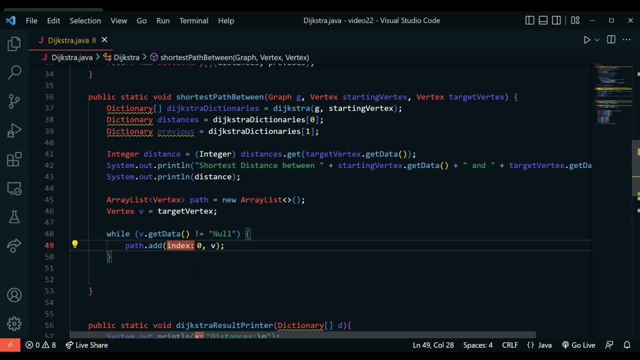 So that vertex that we set up will be also passed in here. And then the next step here is to get the previous instance here, So we can say previous structure, which is a dictionary, dot get, And what we need is the data here. 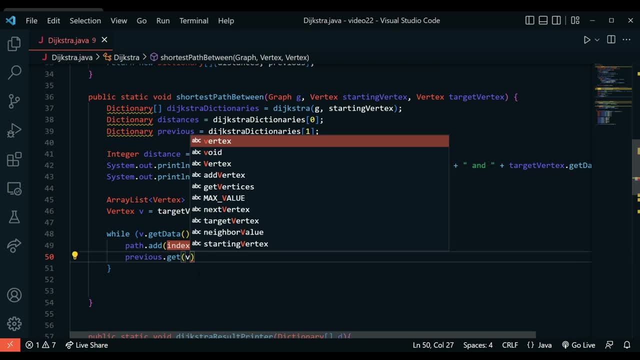 So we say V dot get, dot get, And then we're going to add a string here. So we say V dot get data, And that would give us a string- previous dot get- And we got the value over here And we're going to assign that. 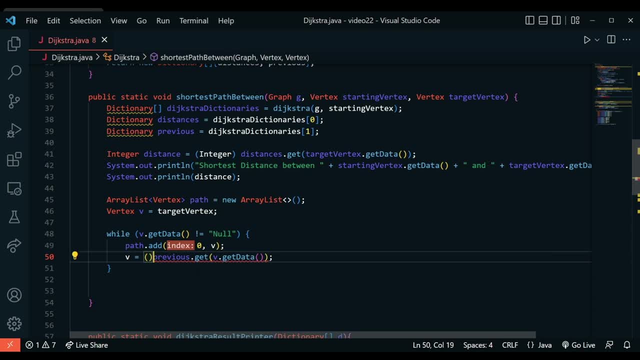 to the vertex. So since we have that get process here, we could actually need the vertex here And that will assign to the vertex. So it's just going to keep going like that And after this while loop we could just print out. 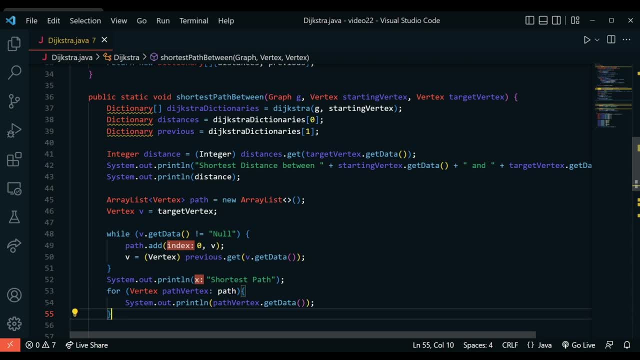 systemoutprintln the shortest path, And what we have now is the shortest path as well, So we could go from vertex path, vertex to from the path structure which is over here somewhere. So vertex path, vertex, So we have this path. 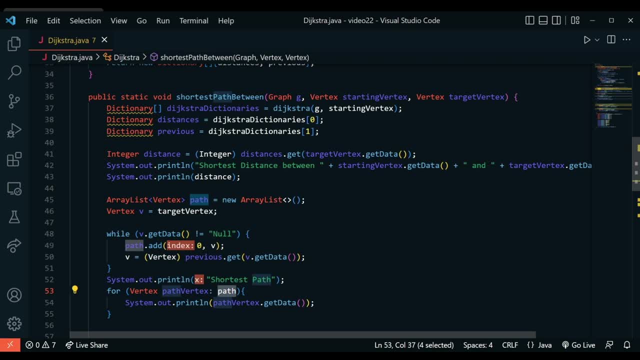 which is this entire array list that now contains all of the vertices for that directed path. Now all we're going to do is iterate through this. for every path vertex, We're going to print path vertex dot: get data And that's going to print us. 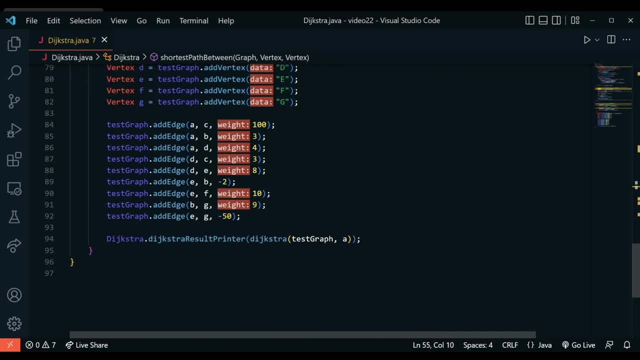 the letters of the corresponding path. Now, the only thing that I'm going to do now is, like I said, I called dykstra dot dykstra result printer and I passed in these two, So what happened here was that I was on an error. 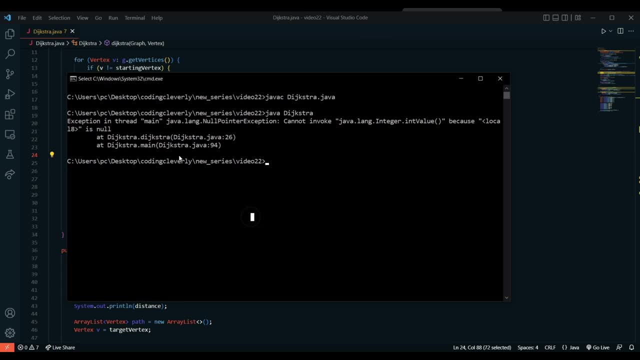 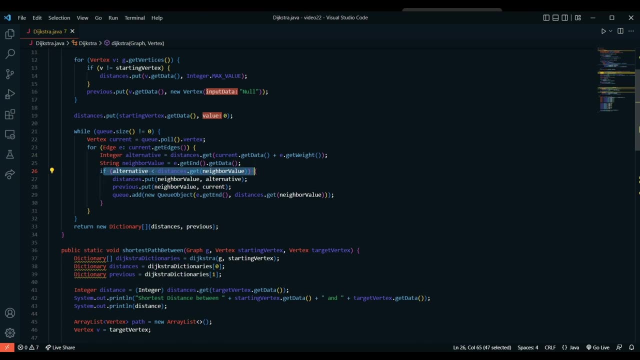 And whenever I was running this code I was getting this error over here at line number 26 and 94.. So over here at line number 26 and 94, it doesn't give me any clue of what's happening, because the alternative is less than. 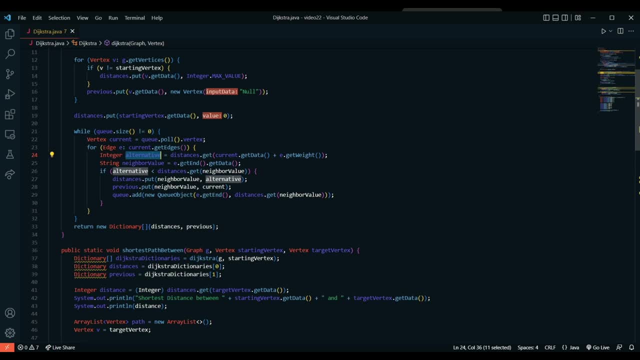 distances dot. get number value. So I was looking at the alternative value very carefully Here. I noticed that I did get an error while I was doing this, So this is actually a syntactical error. I was trying to get the alternative path- distance- and I was getting the value. 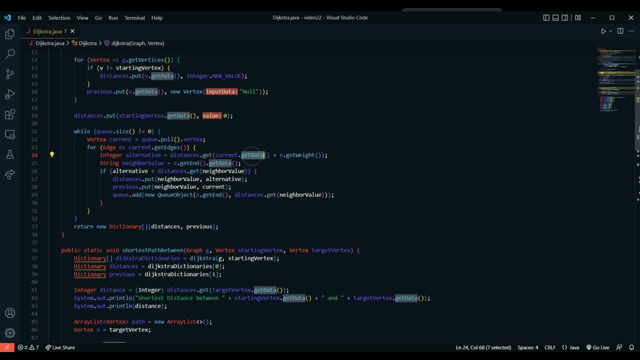 from the distances dictionary and I wanted to current dot get data And this was going to actually give us the value for this one. So I didn't need this parentheses over here, I just needed that closed here And now. it was just going to give us. 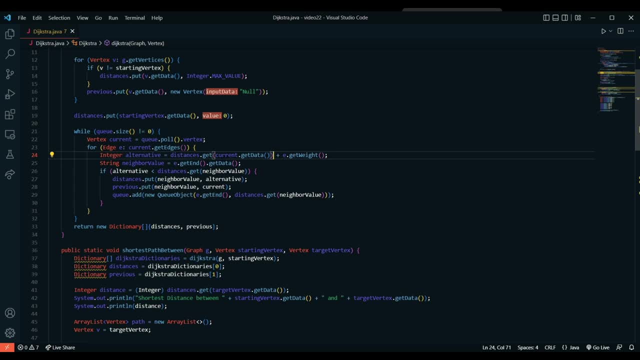 the value here, which was string, So it was going to give us the value of that current data. So it's just going to be an integer here. And then that was going to be added with the edge dot: get weight. So that will also be an int. 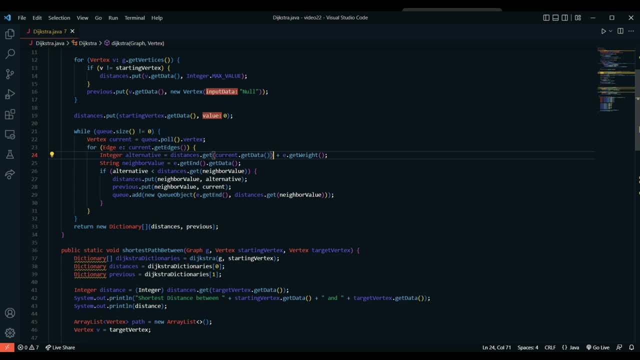 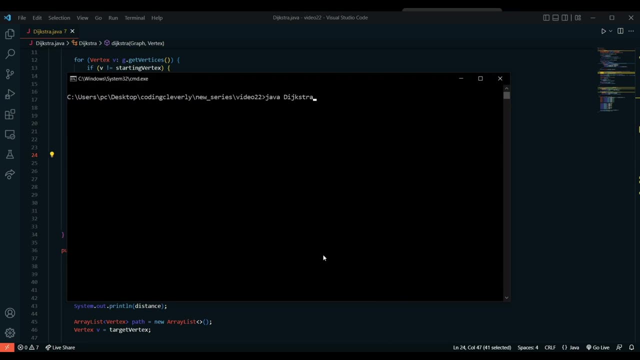 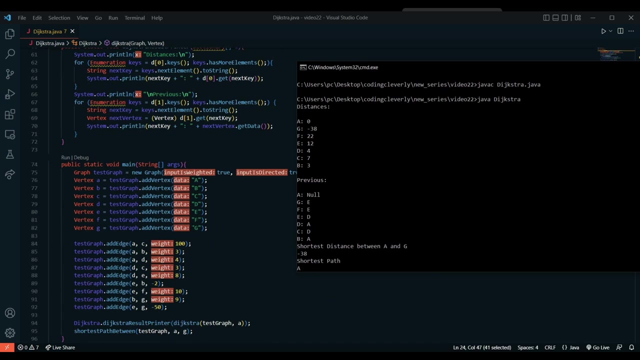 So both of these ints added will result in this alternative value. So now it's proper and if I run the code now, you can see now that this created it for me. So here what I had was these vertices: 1, 2, 3, 4,, 5, 6, 7.. 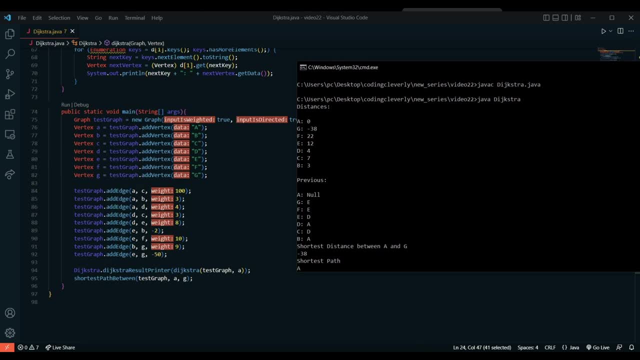 7 vertices and these were the connections to them. I just called the Dijkstra method passed in the test graph and put it in the starting vertex. After that I used the shortest path between method and this is all showing up Pretty cool. 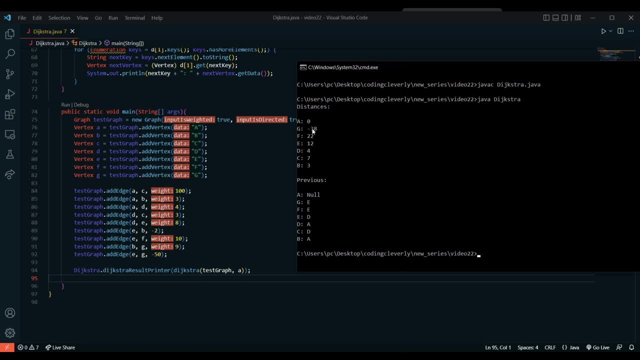 So now we can test it out and see over here that the distance is updated and it's according to what these vertices are. So these are, I believe, 7 vertices and over here we have the connections to them. So you can see A is connected to C. 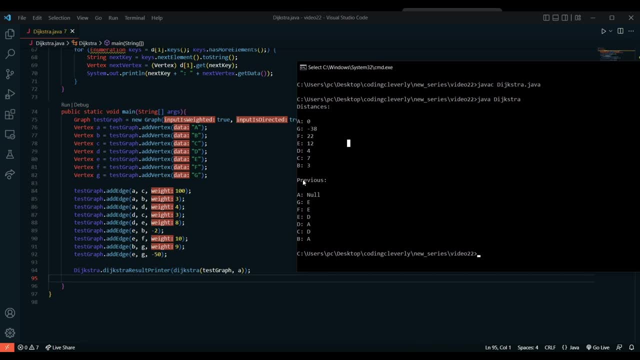 A is connected to B, A is connected to D, And what you can see over here is that the previous. here we have A as null and the rest, when I said, A is connected to B, D and C. if you look at B, D and C, 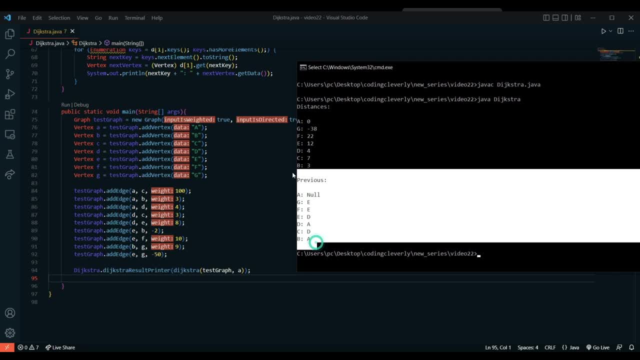 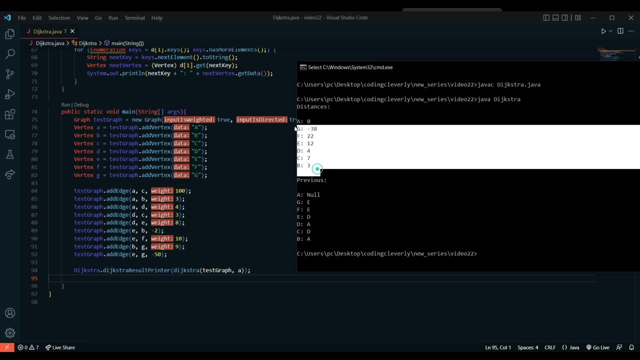 they're all connected to A, So D is connected to A. You can see that this is the structure here, where we have all these vertices and their corresponding values. So these are all the values that have been updated. So the distance from A to itself is 0,. 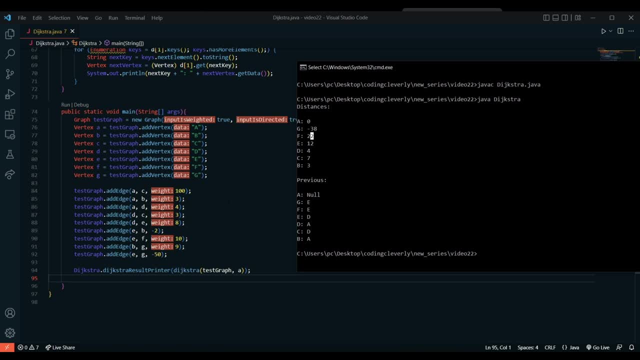 the distance from A to D is minus 38, the distance from A to F is 20.. So we just passed in these values here and it just allowed us to get the minimum distance from this graph. Just telling if the distance from A to B. 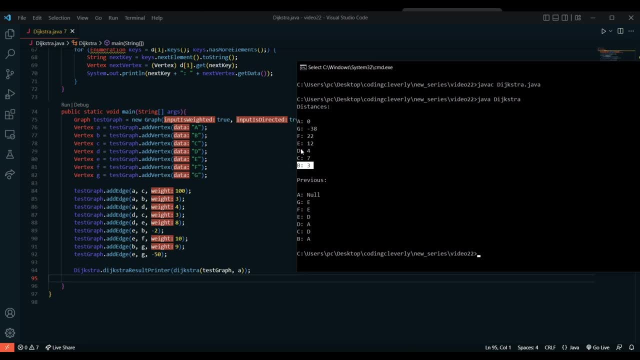 is so. the minimum distance from A to B is 3, the minimum distance from A to D is 4. over here in the previous we have: A has a previous of null, but the rest vertices show their previous vertex as well. For the last method that we created, 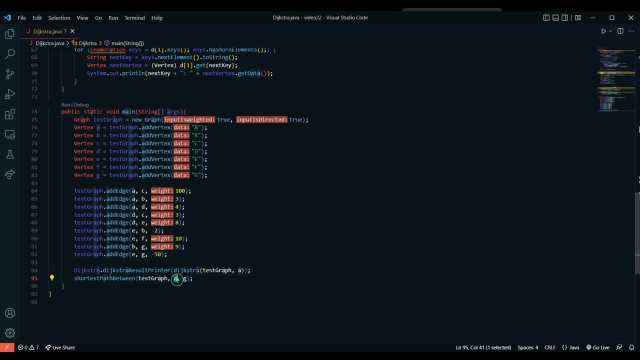 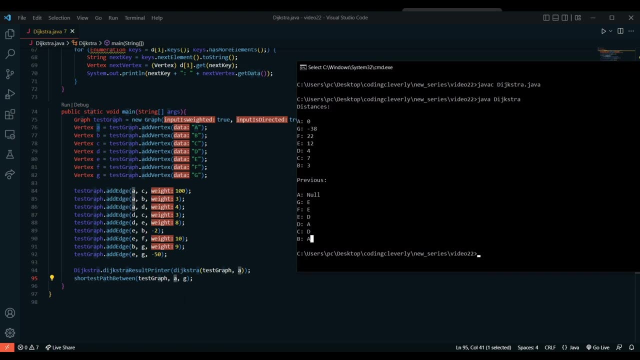 we want to call that shortest path between test graph and we then get the starting vertex and the target vertex. Now we want the path shown and also the shortest path. So what we could do is short pass, we pass in A and G and this is going to call: 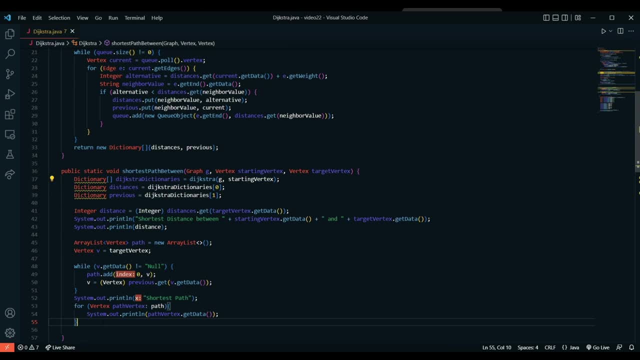 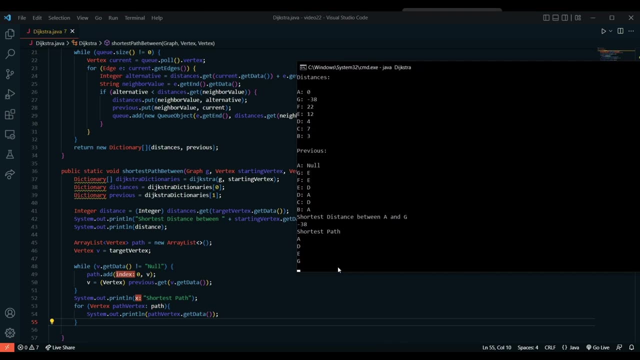 this method over here which is going to call that method, and it will return us some cool looking path. So we will clear the screen and then run it and then see the shortest path. Here we got the shortest distance from A to G, which is correct. We got A to G.